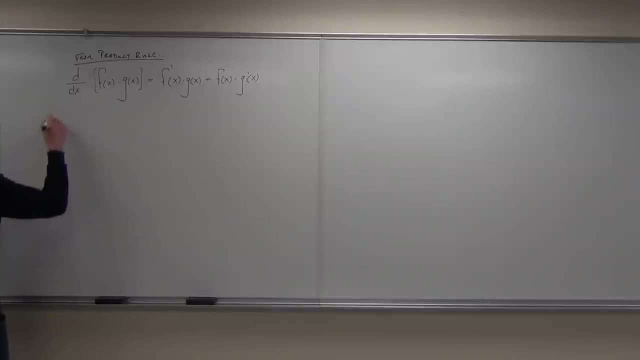 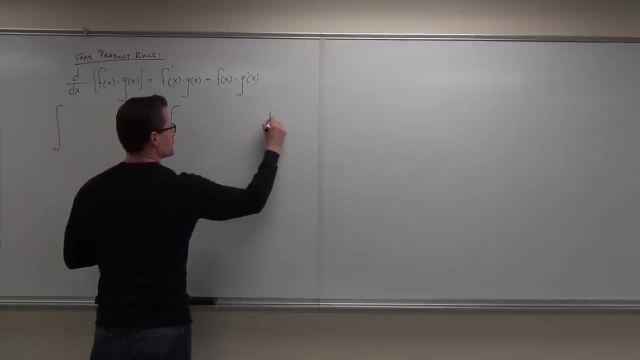 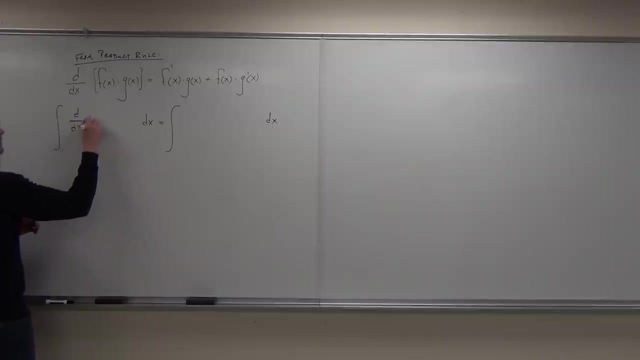 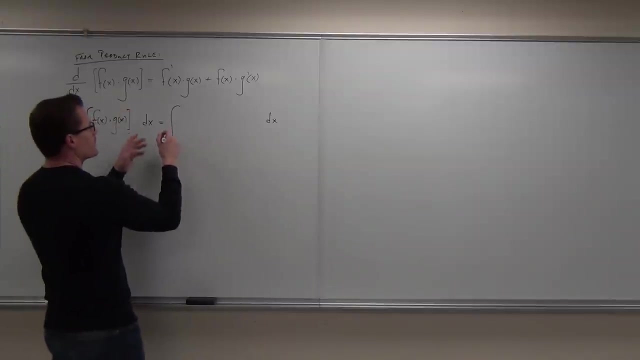 So if we integrate this dx and integrate this dx, then what we end up getting is the integral of the derivative of f of x times g of x dx. And over here we got the integral of f prime of x, g of x, plus f of x times g prime of x. 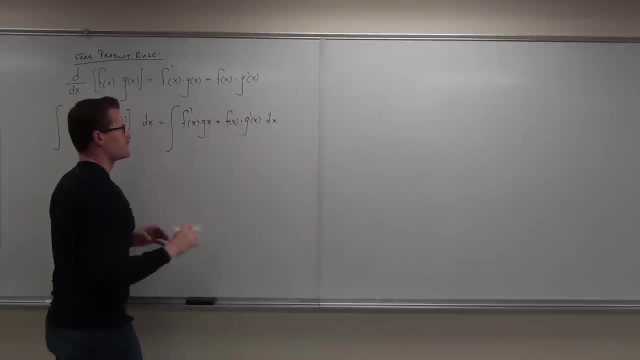 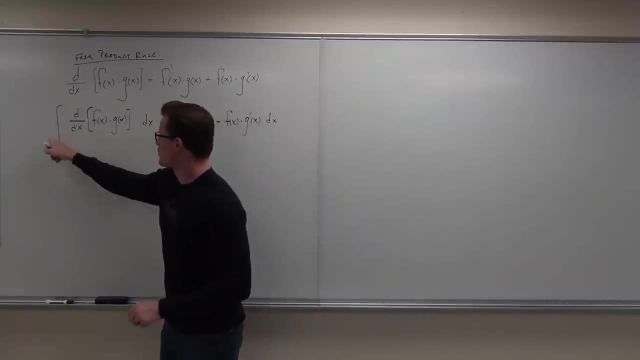 You guys okay with that so far? Yeah, Just taking an integral on both sides. Now let's see what happens here. What is going to happen here? if I take the integral of a derivative, It's going to do itself, Yeah. 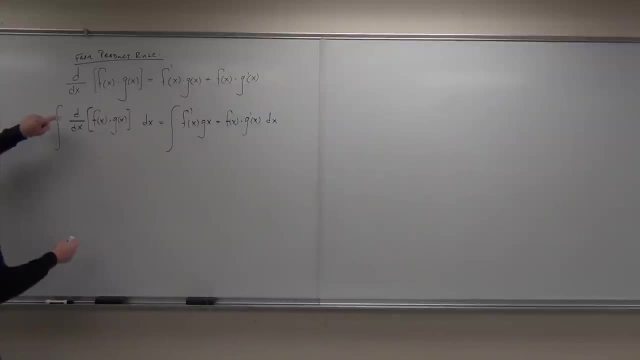 Calculus. Calculus tells us that They are inverses. So if I take the integral of a derivative, dx, dx, that's gone. All I'm going to have is f of x times g of x. Does that make sense to you? 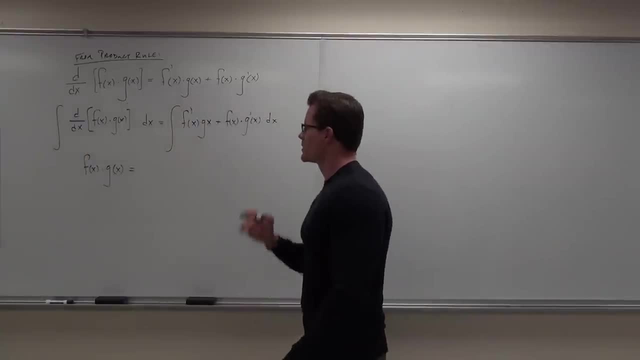 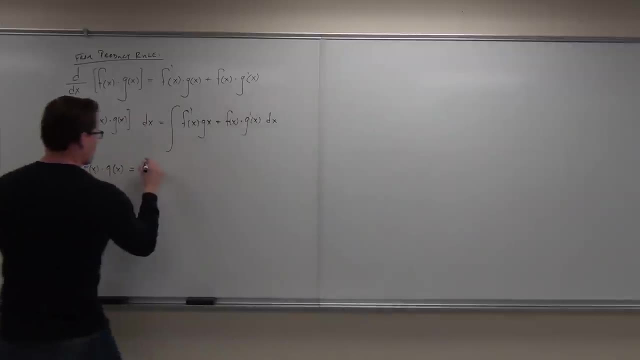 Yes, Are you sure? Yes, Now the next thing I'm going to do: I'm just going to separate this. Notice that with integrals, you can separate by addition or subtraction, So I'm going to do that. I'm going to have the integral of f, prime of x, g of x. 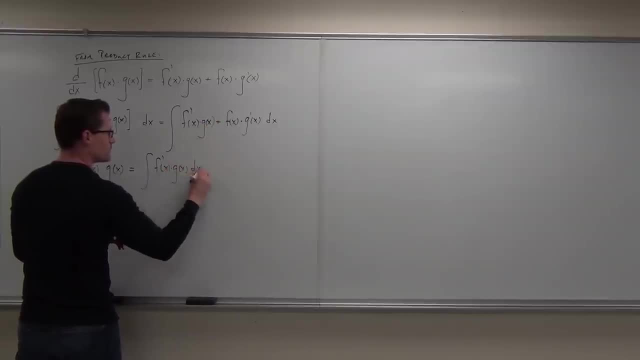 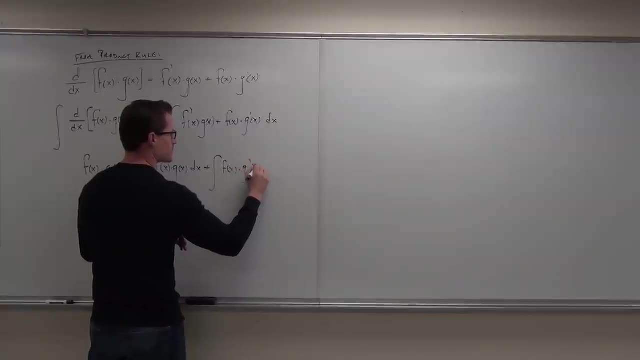 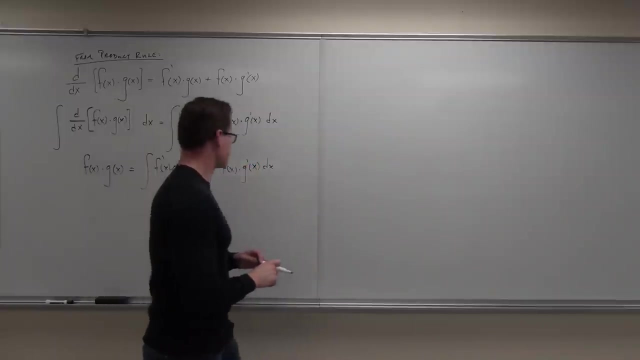 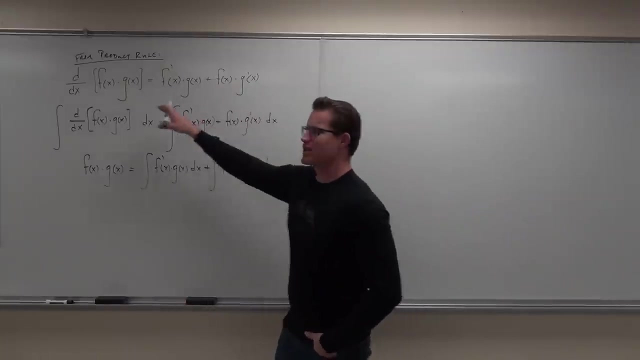 Yes, dx plus the integral of f of x times g. prime of x, dx. Yes, So we have product rule. I should take an integral on both sides. No big deal. Derivative is gone. Integral and derivative, they basically undo each other, They're inverses. 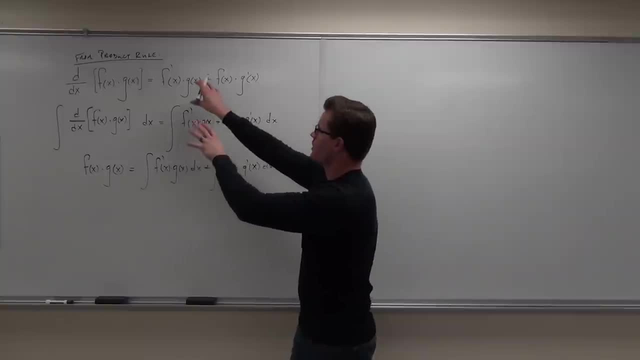 So we have just the functions themselves. f times g. Here we know this was a product rule. If we break up our integral after doing an integral, on both sides we have one integral. We've got two integrals. You guys with me. 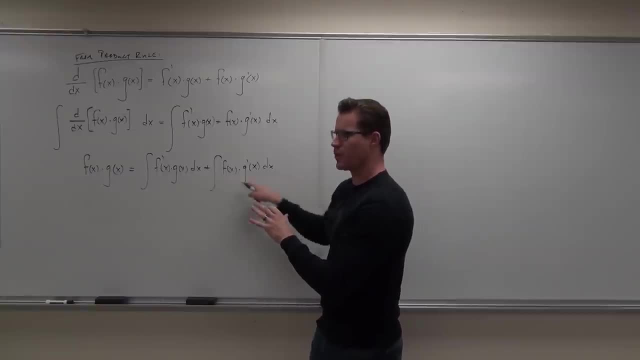 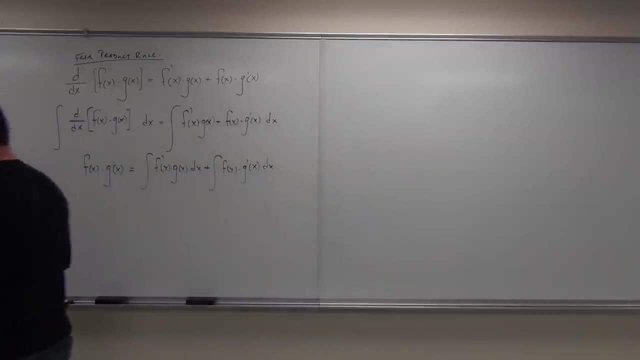 I'm going to solve for this one. I'm going to put this on one side. Basically I'm just going to subtract that guy. Does that make sense? Yes, Okay. So if I do, Then we've got integral of f of x times g, prime of x, dx equals. 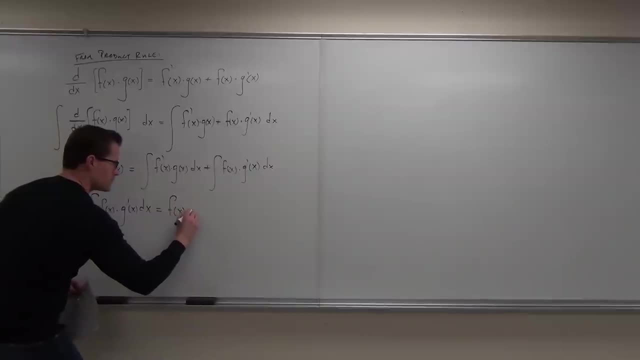 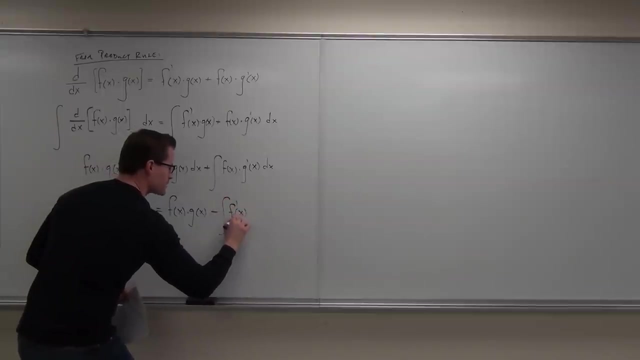 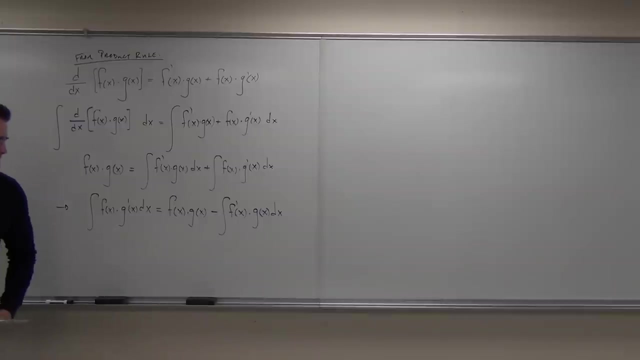 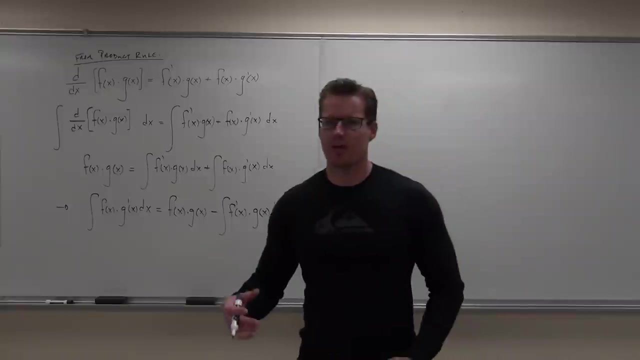 I'm going to keep this And if I have subtracted that I'll have f prime of x times g of x dx. Yes, Are you guys okay with the algebra? on that one I'm going slow. I want to make sure you really do follow it. 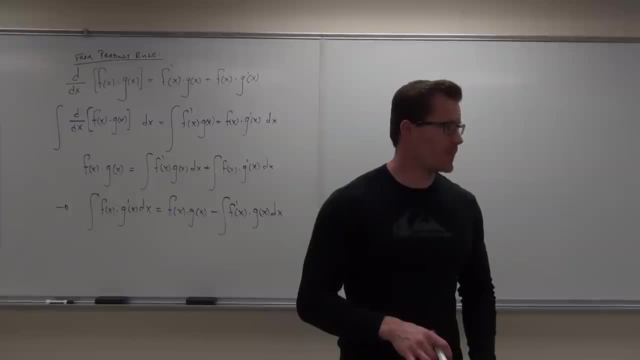 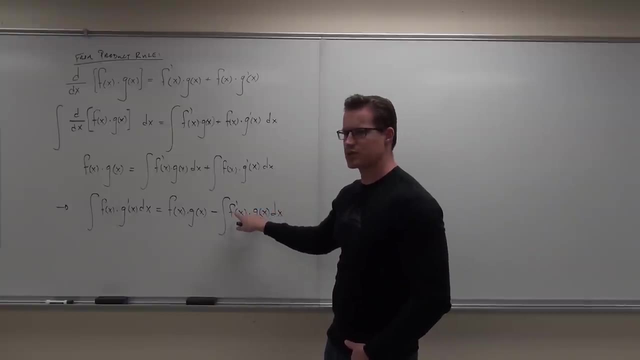 Do you follow it? There's only one more thing that I'm going to do. What I'm going to do right now, I'm just going to switch these two guys around. So, by the commutativity of multiplication, this is not a problem. 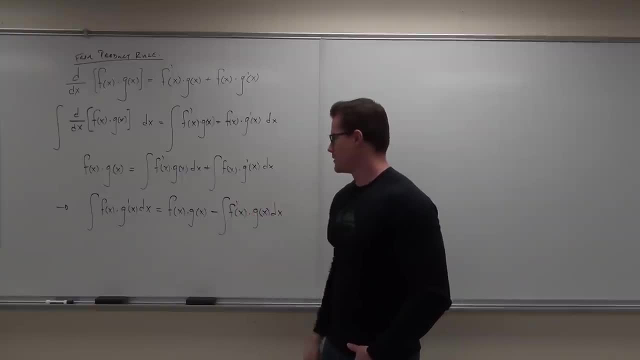 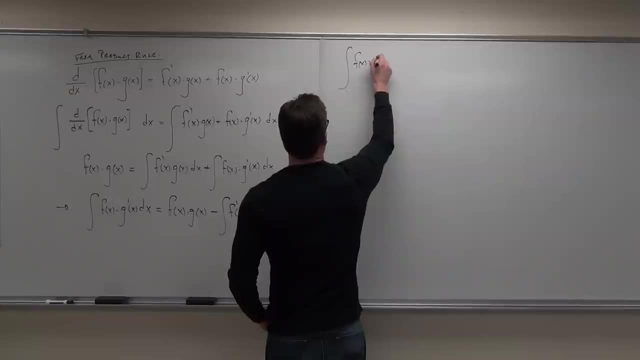 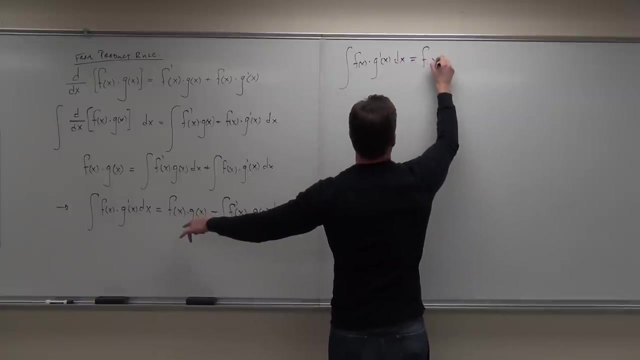 I'm going to put g of x before f prime of x. Are you okay with that one? Okay So, Okay So. integral of f of x times g prime of x: dx equals. Let's see f of x. 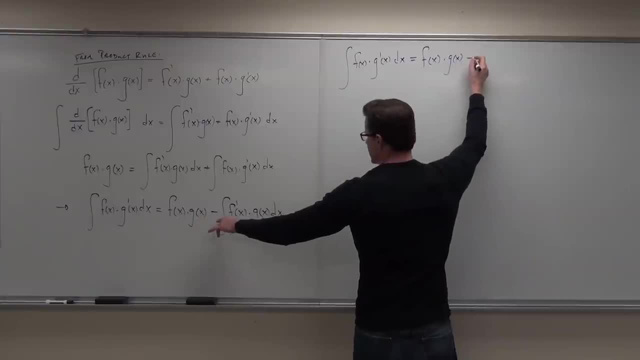 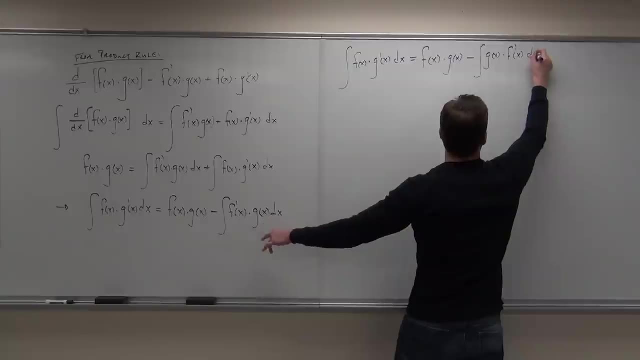 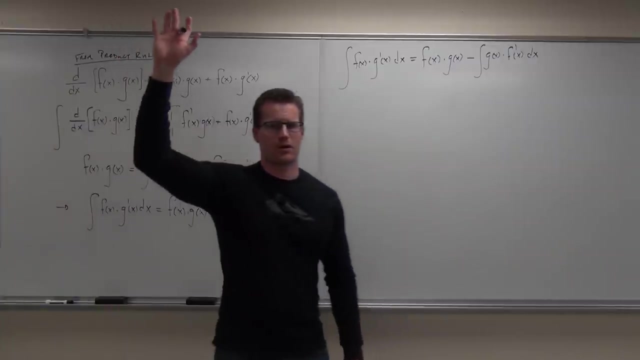 Got that Times g of x, No problem. Minus integral of g of x times f, prime of x, dx. Okay, I want to show if you guys feel okay with that so far. Now that's just some algebra after doing a little bit of calculus. 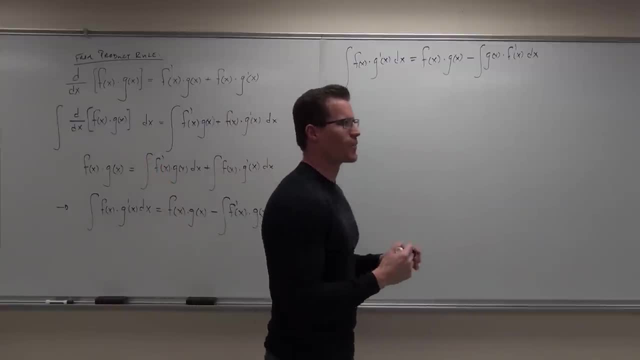 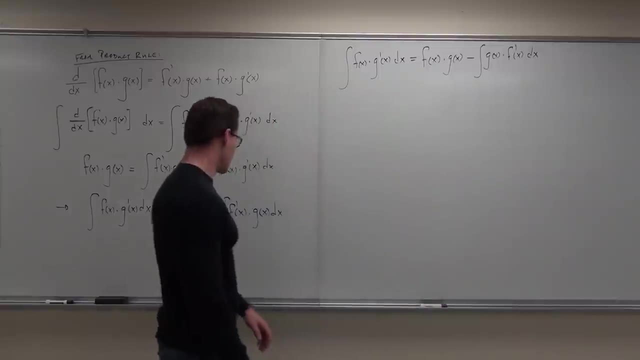 All we did was doing integration on both sides. What in the world does it all mean? Well, I'm going to show you, because right now it's a little hard to understand. We're going to use some symbols right now to represent some of these functions. 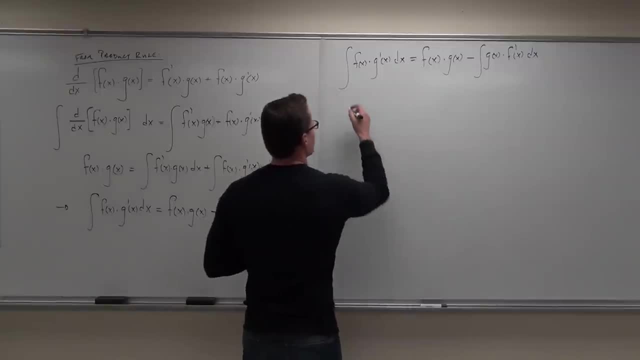 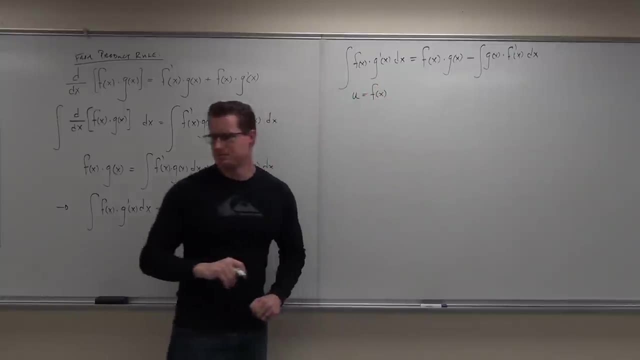 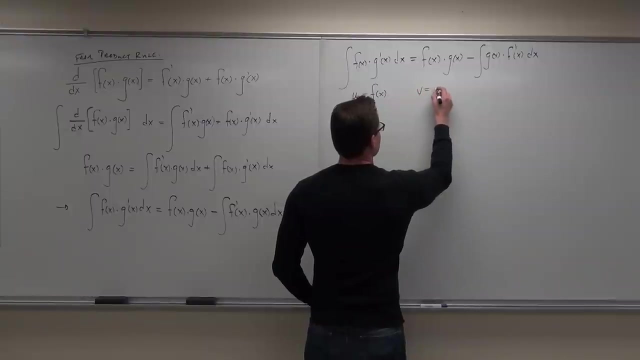 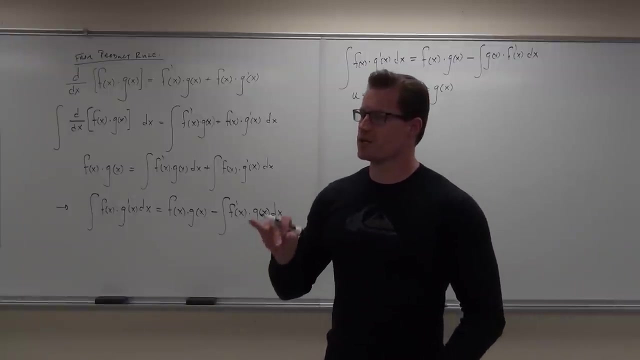 So what we're going to do is we're going to call u, We're going to call f of x u And we're going to call g of x v. Please keep in mind: u and v are going to represent functions in your integral right now. 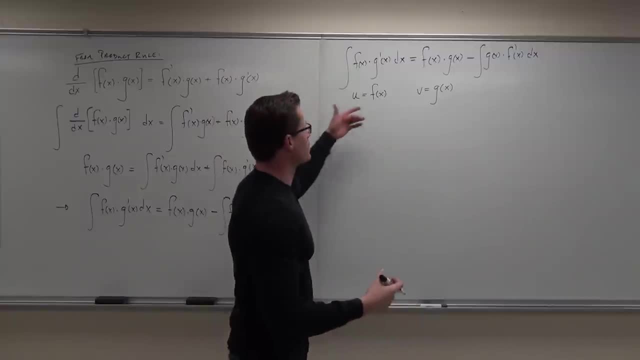 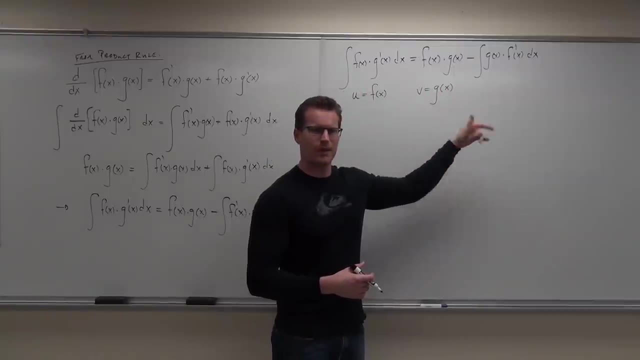 They're going to represent some functions here, So we're letting u represent the function of x, v represent the function g of x, a function of x. You guys? okay with that so far? Yeah, Now we got some other things besides just f of x and g of x, don't we? 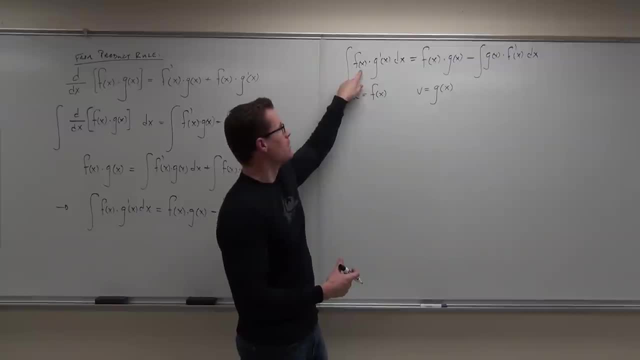 I mean, we could change this to a u right now. Are you with me? We could change this to a u. We could change this to a v. We could change that to a v. You with me, Mm-hmm. 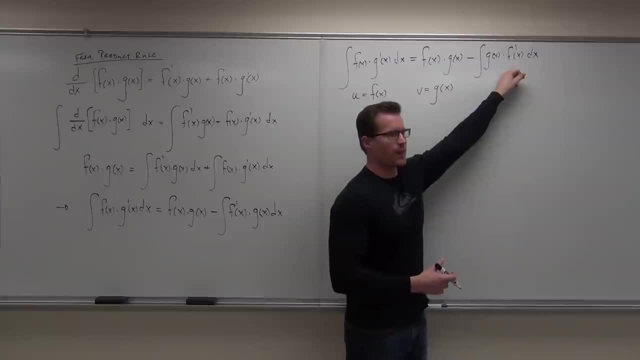 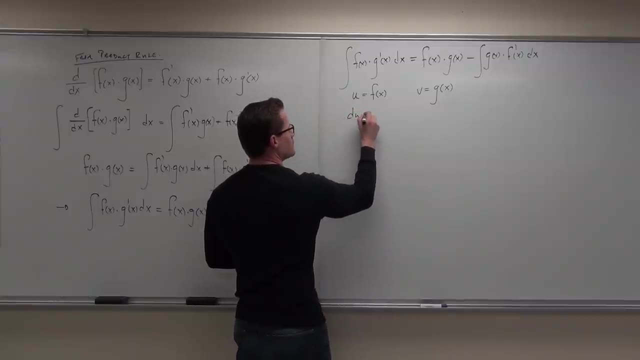 However, we've got an f prime and we've got a g prime, So what we're going to do is go, okay, cool. Well, I'll tell you what. Let's just do like a du, Let's do a derivative on both sides. 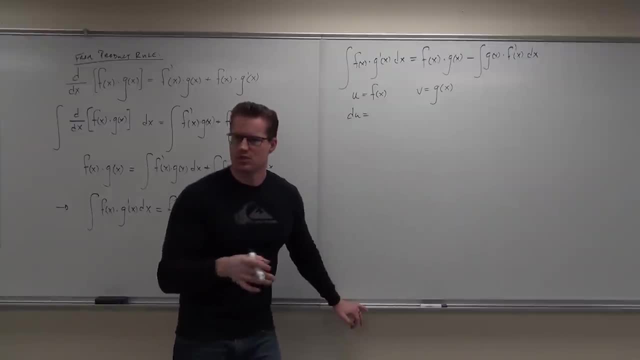 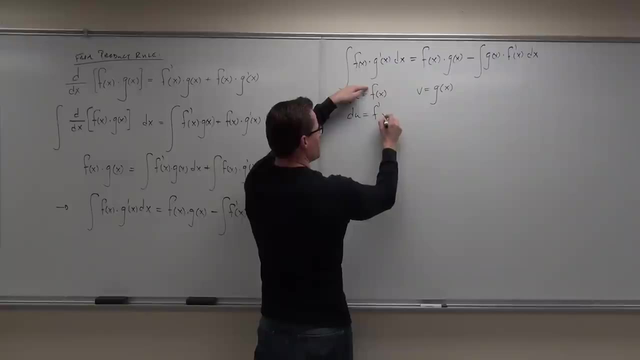 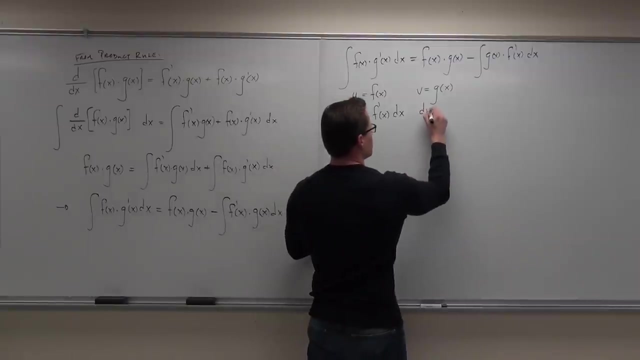 If I do this, just like your substitutions do, sorry, derivative of u is our du. Derivative of f is f. prime of x dx. Ah, dx. Do you ever do that? Yeah, Just like a substitution. Well, here we'll get dv and we'll get g. prime of x, dx. 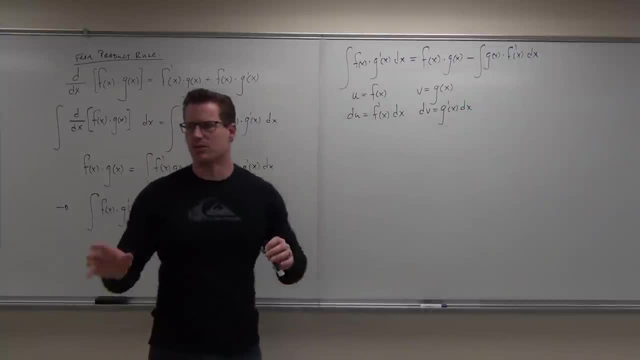 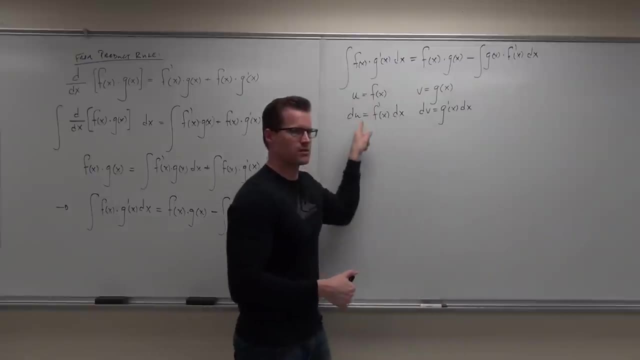 Mm-hmm, You still okay with it? Yes, Now look, Every one of these pieces is now part of this little box of knowledge. Let's do a substitution. Instead of f of x, what are we calling it? U? 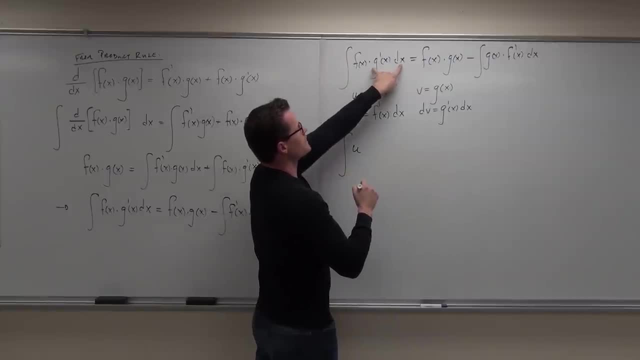 No, f of x is just u, U. What is this piece? g, prime of x, dv, dv. That's our dv, So this is dv. F of x. was u g prime of x, dx, dv, dv. 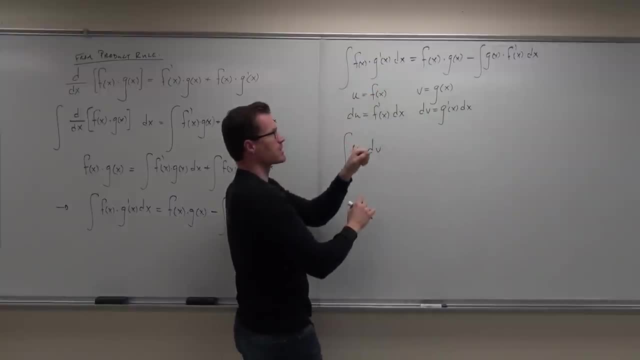 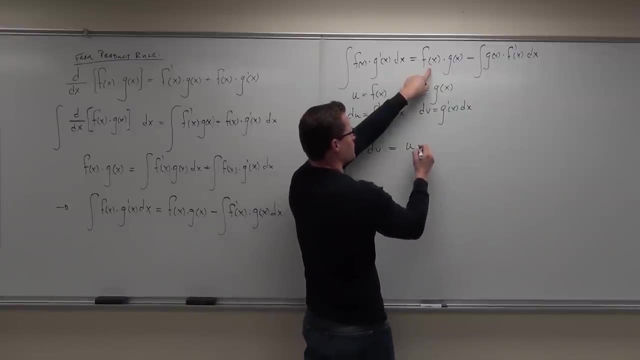 You guys okay with that so far. Yeah, Yeah, Equals, Equals. What's our f of x? again, u? u. What's our v? v? So f of x is u times, g of x is v v. 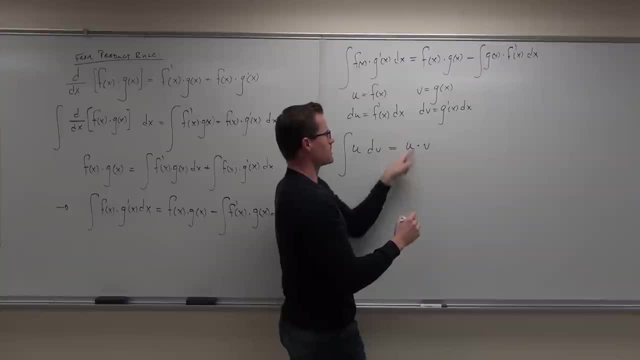 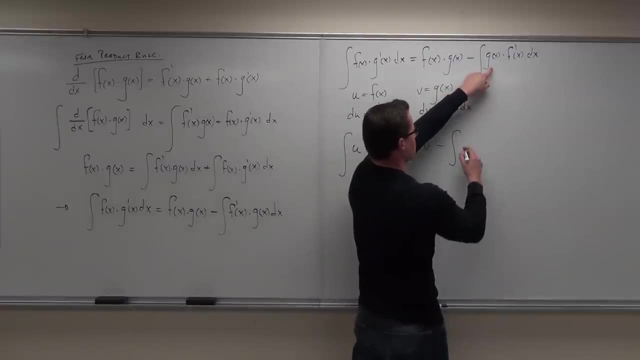 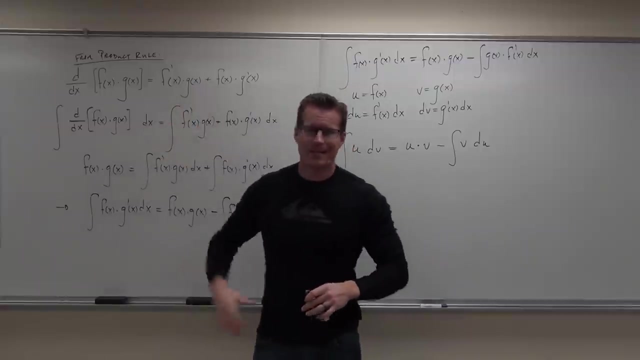 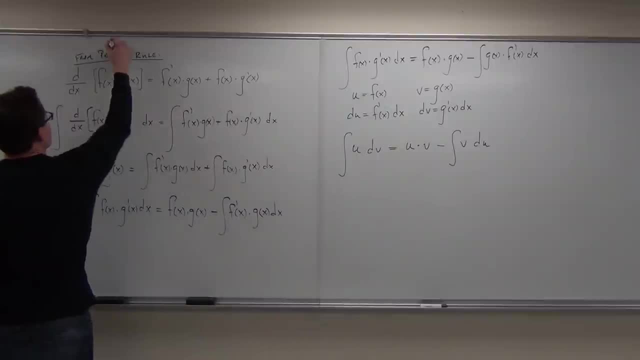 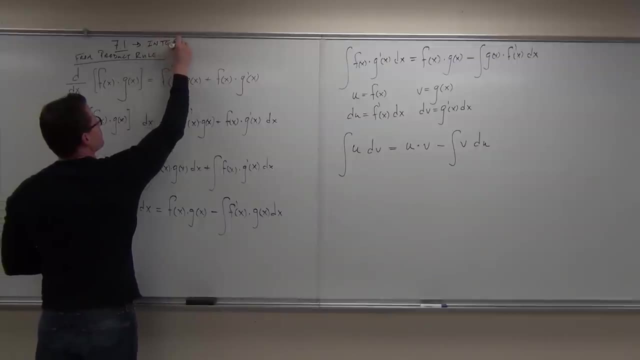 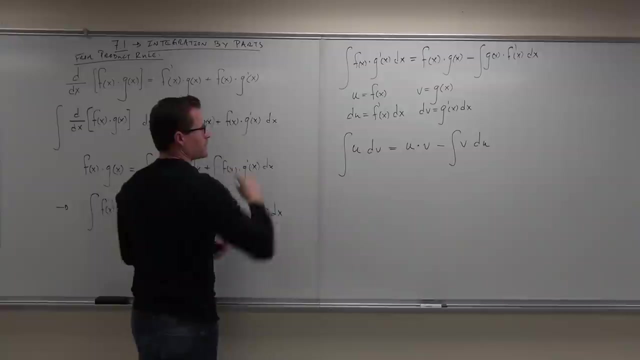 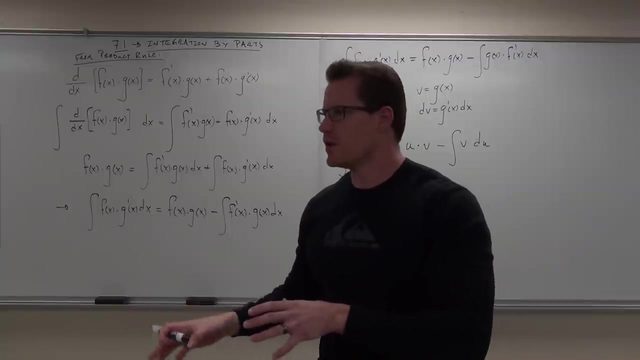 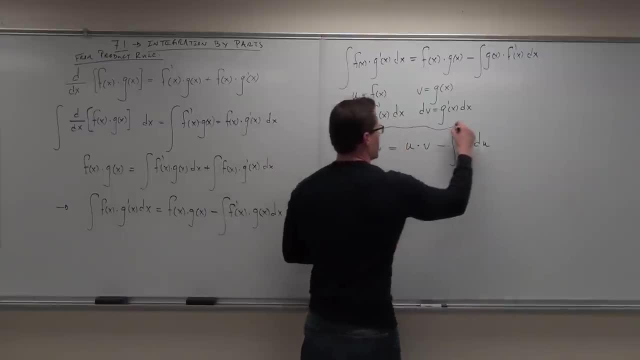 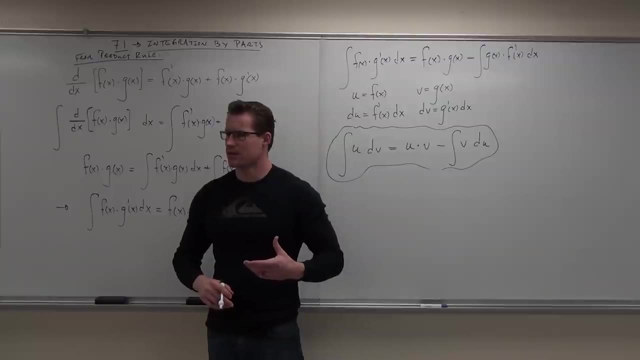 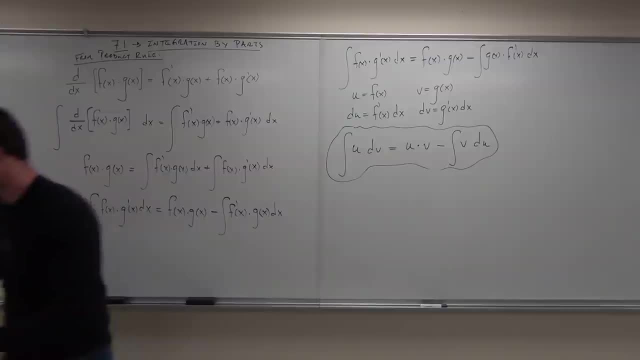 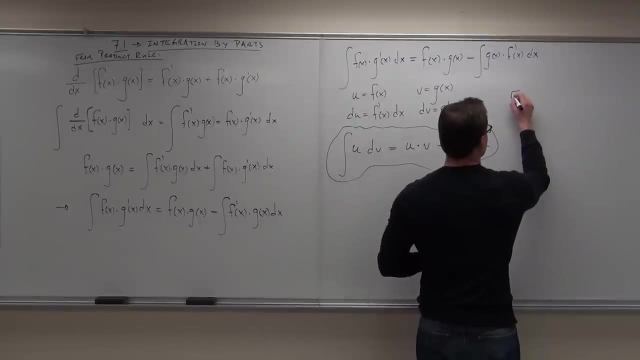 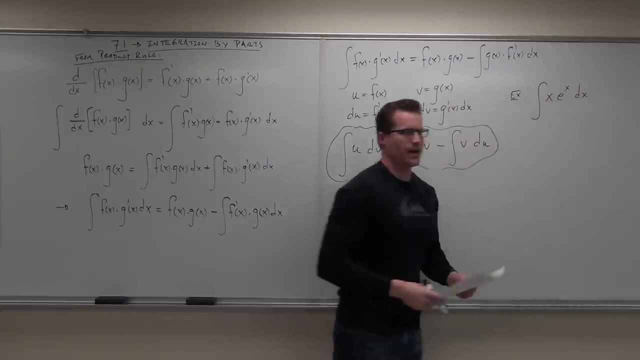 This stems from the product rule. It's an easy proof, but that stems from the product rule. Let me show you why we do this. So: integral of x times e to the x dx. So this right here. what's this called again? 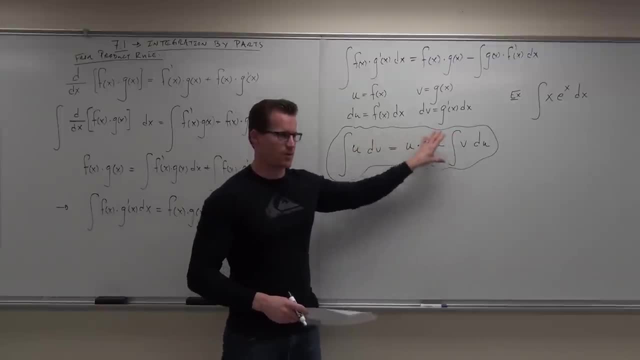 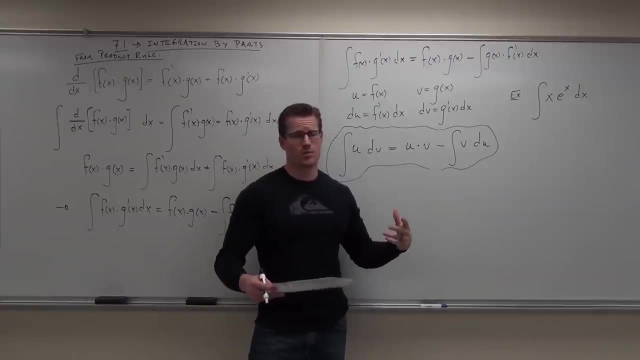 Integration, Maybe write that This is integration by parts. So when I say do integration by parts, or when the book says, do integration by parts, or your best friend says at one of your parties, hey, can I do some integration by parts? 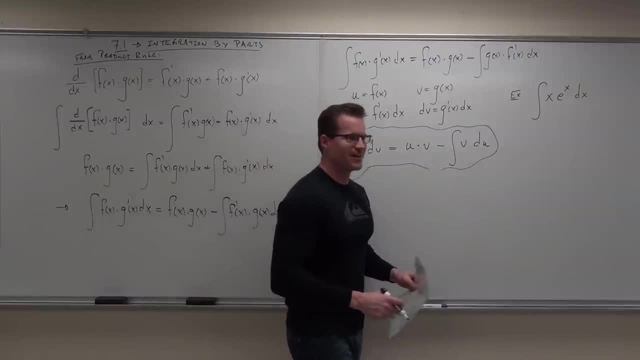 You're like, uh, yeah, Duh, I know what that means. That would be the best party ever, by the way. So my kind of party. So let's look at this for a second. Think through all the things you know about integrals. 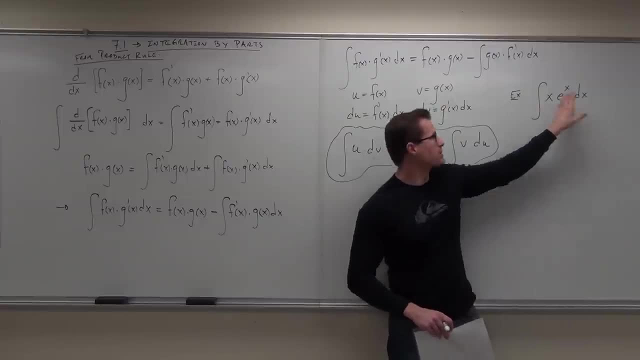 Does that fit your integration table the way it is? No, This would. That would be easy. That would This. Can you use a substitution? No, If you take this to be u, the derivative is 1.. Does that get rid of the x? 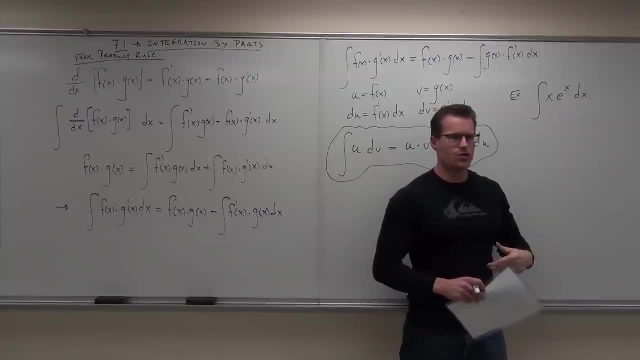 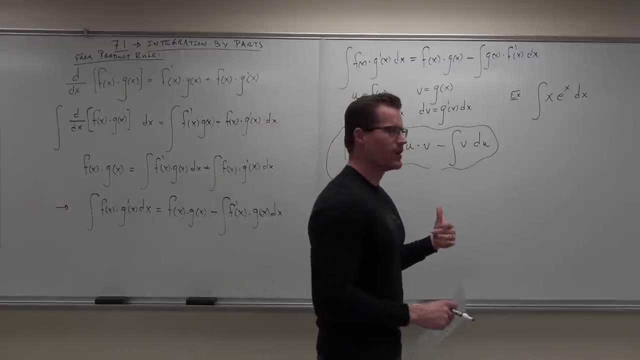 No, That's a problem. So, will a substitution work here? No, There's no way to do this integral for us right now. We had to create something new that would take care of it, and this is what we have. You see, when you have a product here, we use the product rule. 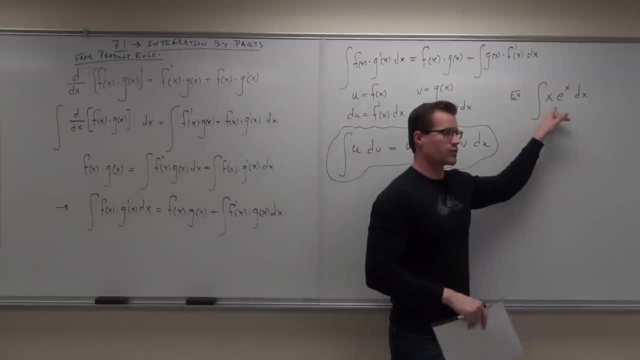 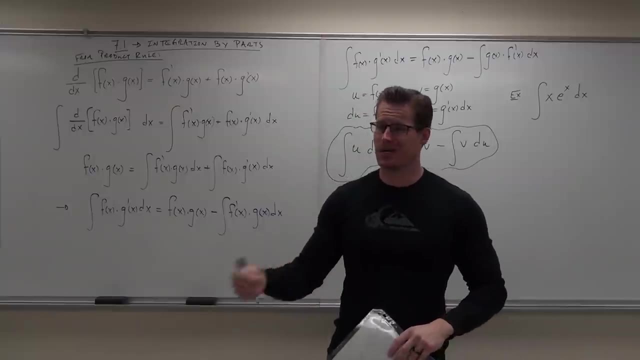 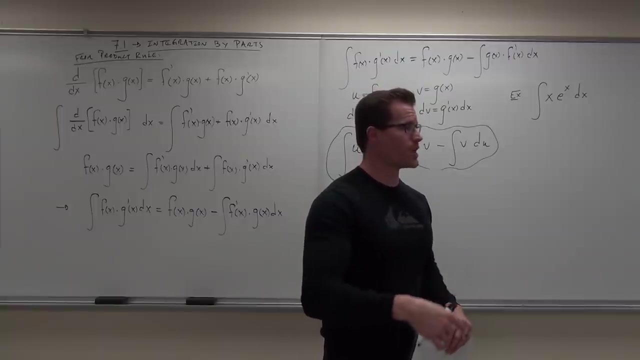 Sometimes, when we have products here, we can use for integrals, integration by parts, which is really really cool. Let me show you how this works and let me show you what you should be picking for u and for v. By the way, it should be really apparent whether you picked the correct thing or not within about the first step or two. 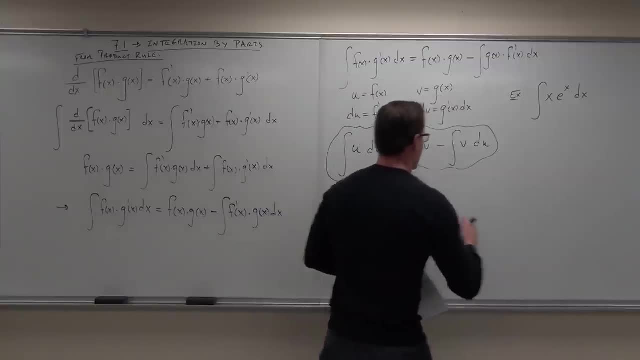 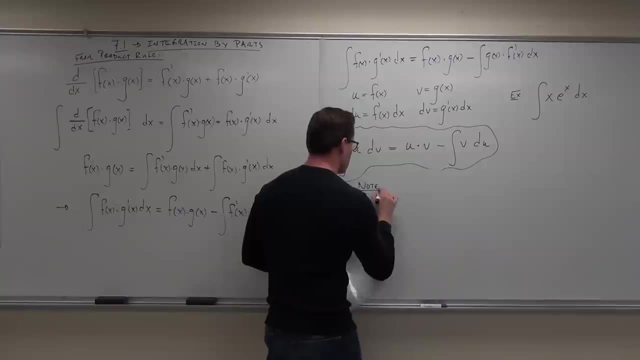 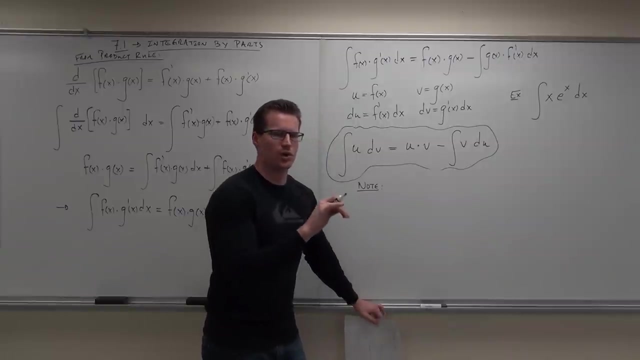 All right. So here's how, in general, you choose your u and how you choose your v. So a couple little notes. I want you to choose u so that you can take the integral of whatever v is basically the integral of the rest. 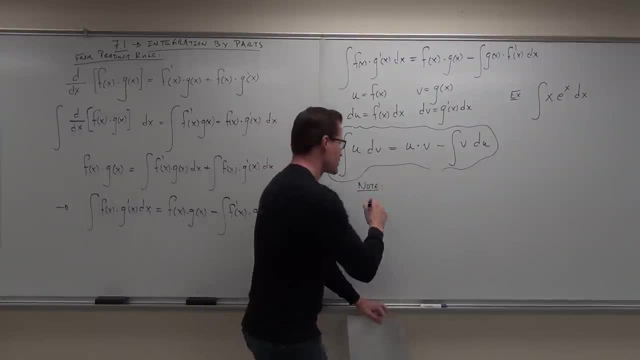 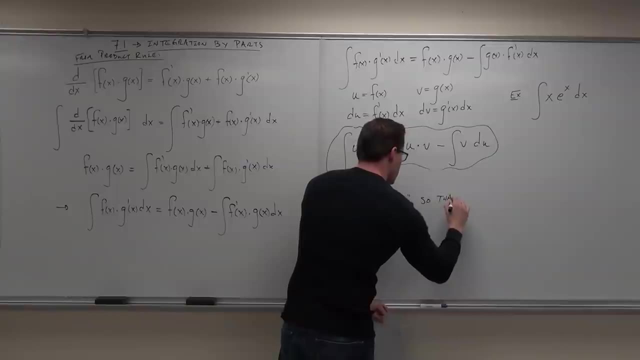 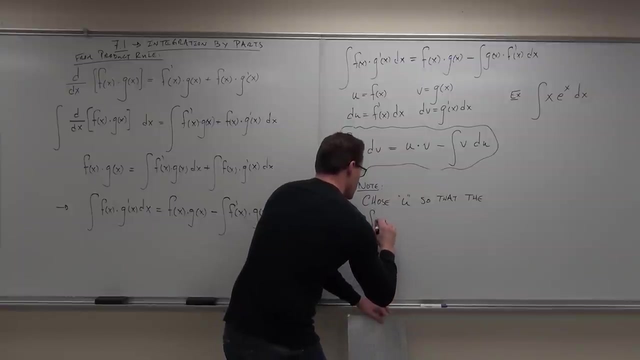 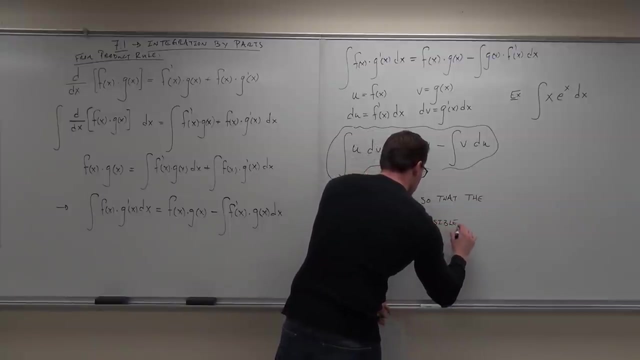 It'll make sense in just a second. I'm going to write out the notes right now. I'll write them down and I'll explain it. So choose u such that or so that the integral of v is actually possible. All right, And try to pick u. 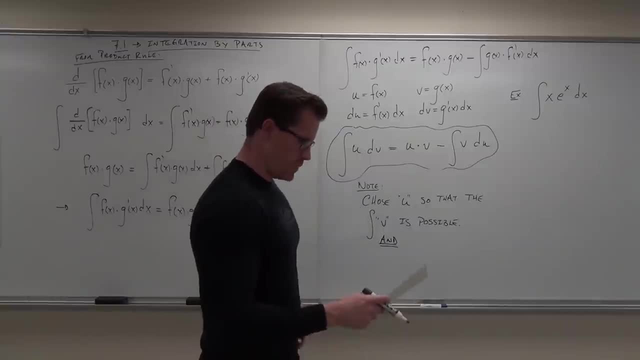 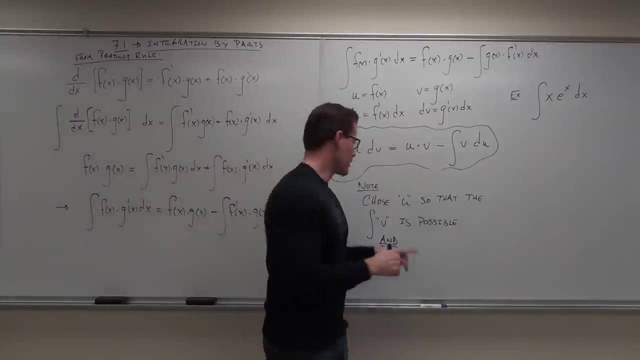 This doesn't always work, but this is a good indication. Try to pick u so that the derivative of u is better, so that it's smaller or easier to work with. So choose u so that the integral of v, firstly, is possible, because you're going to have to take the integral of v. 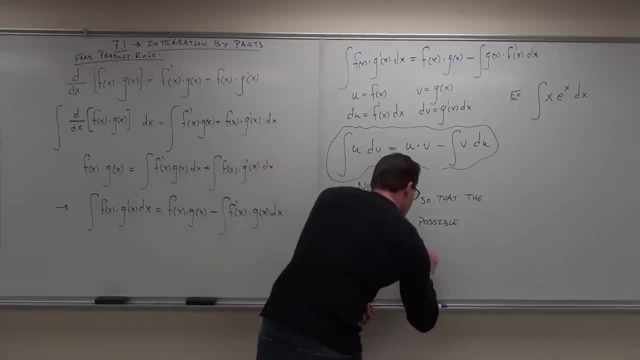 Also again, try to pick u And so that the derivative of u is better- I know that's not mathematical, but better as in: you reduce the power, It becomes smaller, It goes away completely, something like that. So here we go. 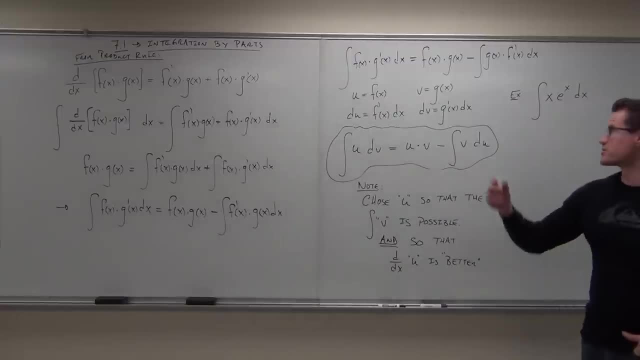 I want you to look at this integral with me. There's two parts to this. There's an x part and there's an e to the x part. You with me? OK, If I pick u to be e to the x, is the derivative of e to the x better? 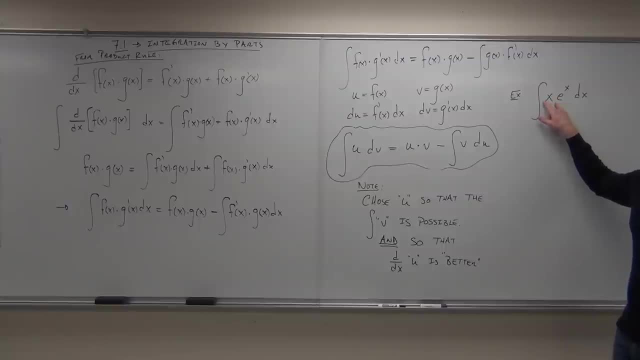 No, No, it's still e to the x. I could take the integral of x, That's OK, But if I pick x, what's the derivative of x, 1. Is that better? Yes, Yes, 1 is better than x, isn't it? 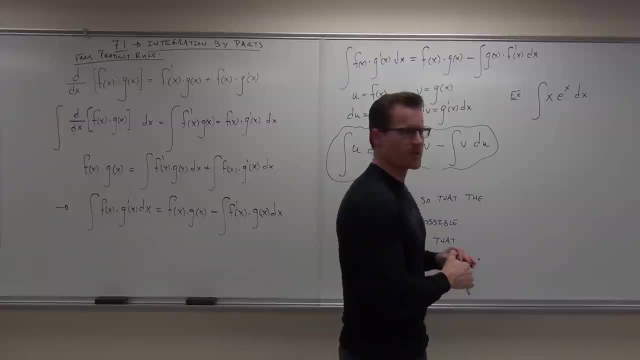 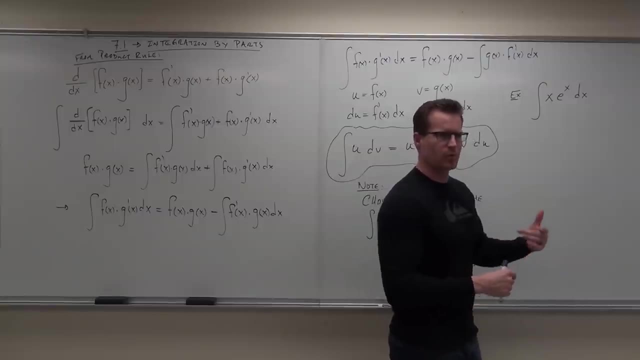 I think so. I think so. I'd rather work with 1 than x. It seems better. Also, can you do the integral of e to the x? Yes, Let's pick our appropriate choice for u. So here's how we do this. 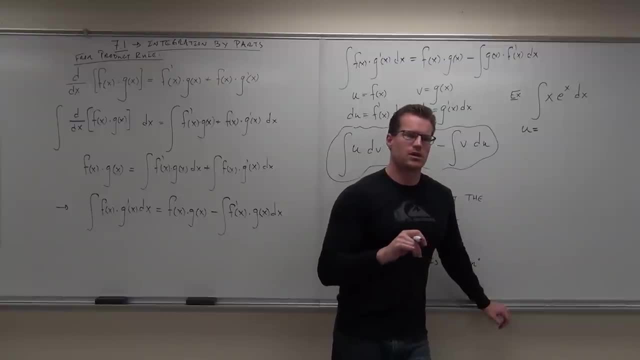 It's going to take some getting used to, but here's how it works. Pick u so that you can take the integral of the rest, your b, and pick u so that, hopefully, the derivative of u is going to be better, easier to work with. 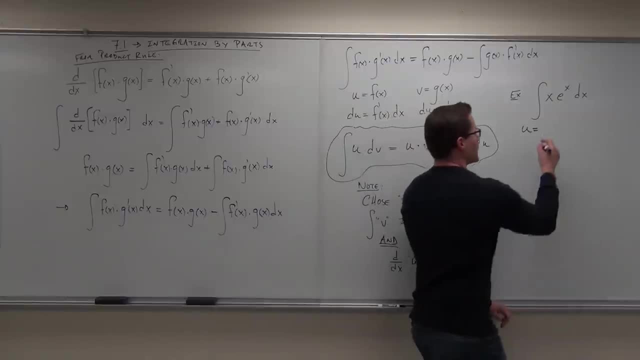 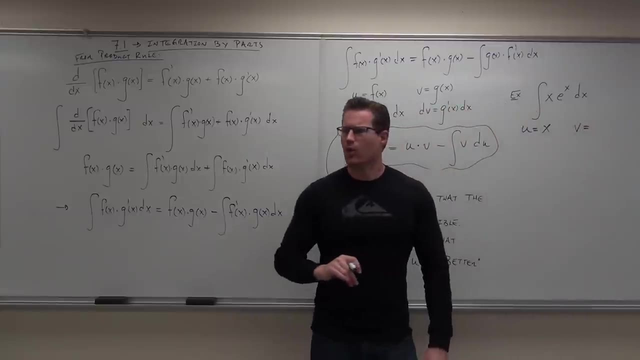 Do you follow that? So in our case we're going to pick: u equals x. Here's what b equals. It's really easy to find. There's an easy way to do it. Once you're u cover that up with your hand. 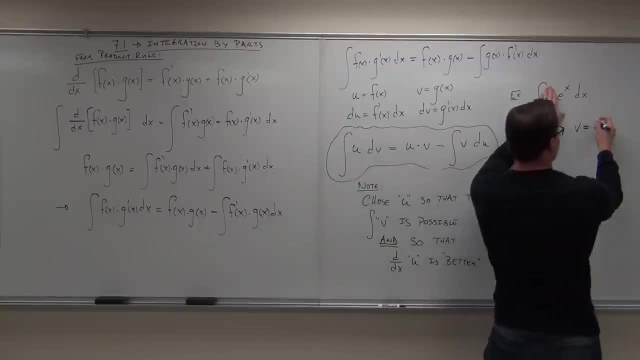 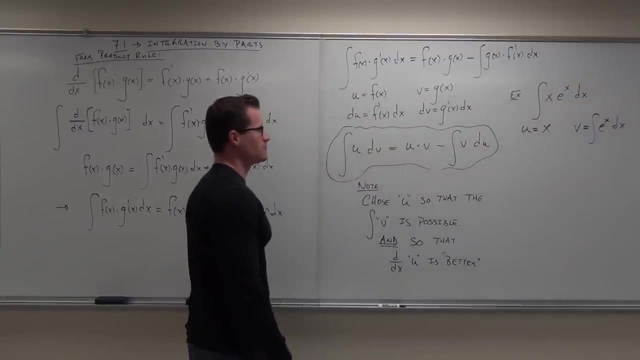 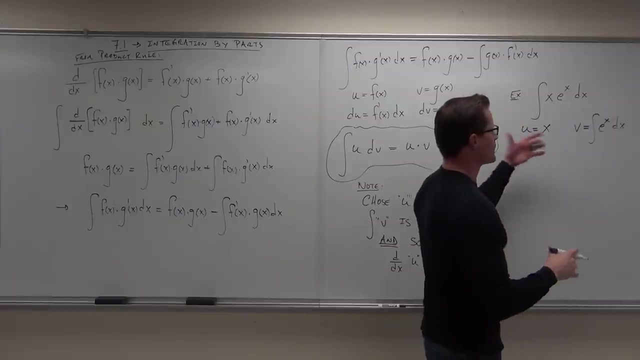 v is all the rest of it. So v is the integral of e to the x dx. The reason why we have that is because we're going to have to deal with the integral at some point. We have to have. our v equals the integral of the rest. 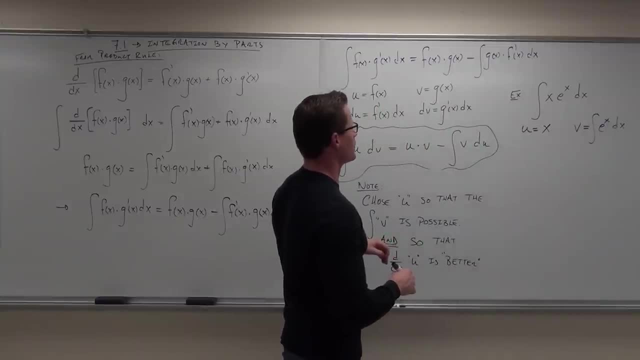 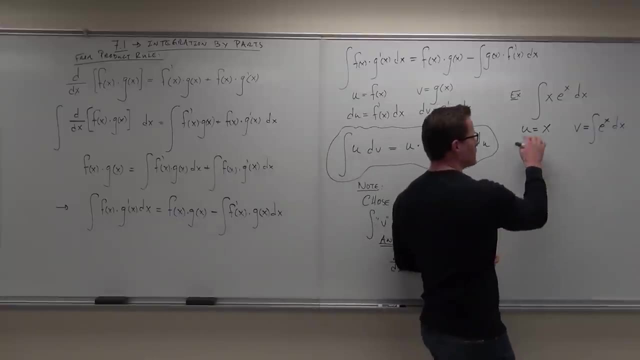 We need to be getting. let's see what are we trying to get there. We want to be able to find our v for this guy. We've got to have that. So can you do your just like you're doing a substitution? can you do your du? 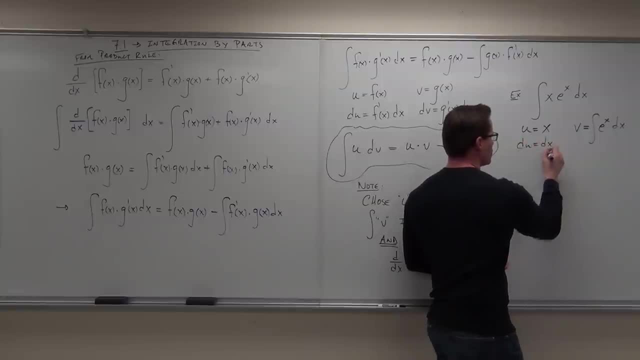 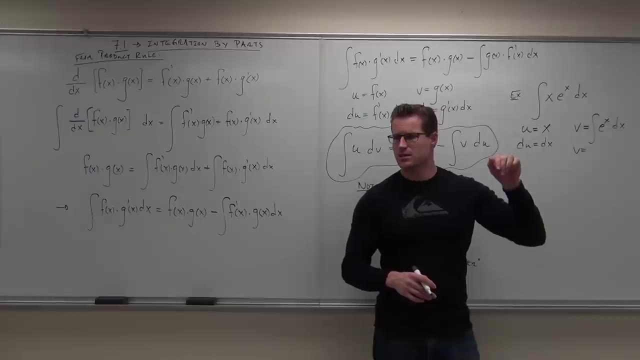 Yes, How much is your du equal? Yes, Okay, v was the integral of the rest. Can you do the integral of e to the x? Yes, How much is it? e to the x? Don't worry about the plus c right now. 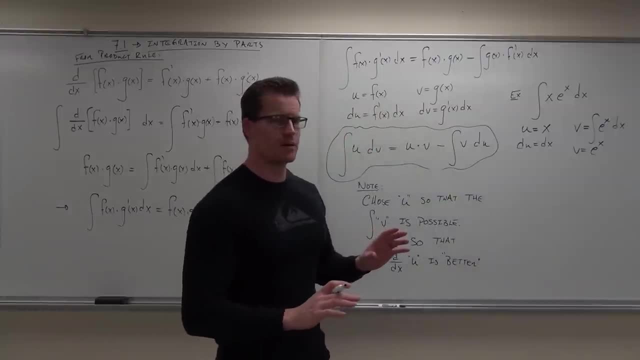 Don't worry about the plus c. right now We're going to deal with the say what Oh v? No, we're just right here. we're not doing a derivative. We're saying v is the integral of the rest. 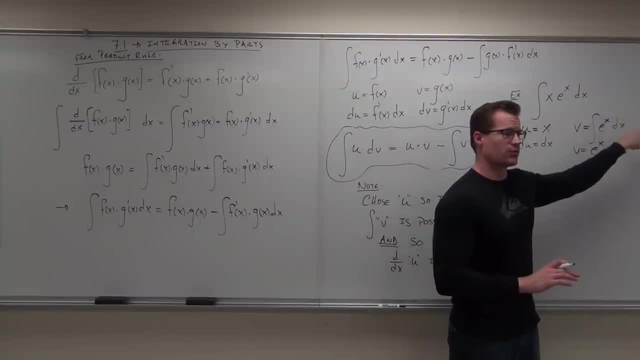 Okay, we're not doing derivatives here, We're actually doing the integral of this thing. So v is the integral of the rest. That's what v is. So, okay, do the integral of that. v is now e to the x. 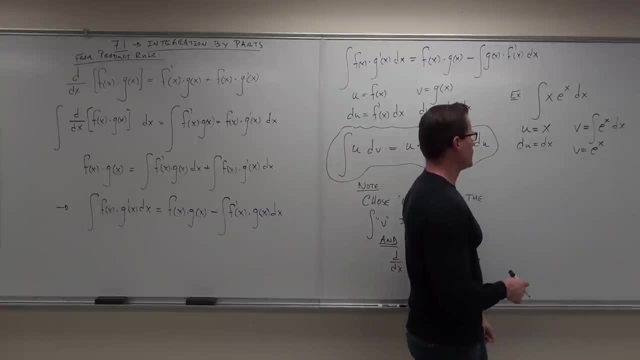 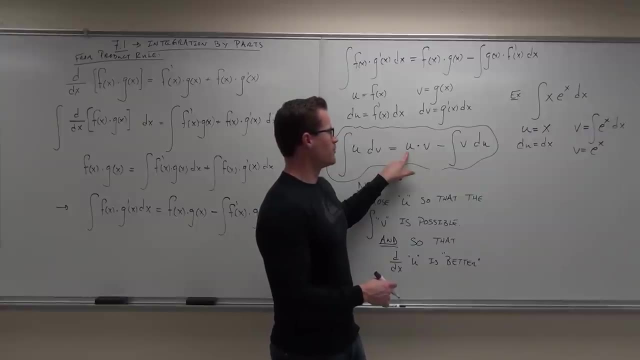 You with me? Yes, Okay, cool Man. do we have the parts? Do we have what u equals? No. Do we have what v equals No. Do we have what v equals The same thing? Yes. Do we have what du equals? 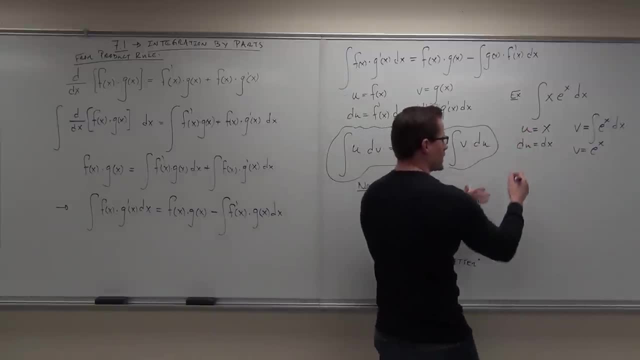 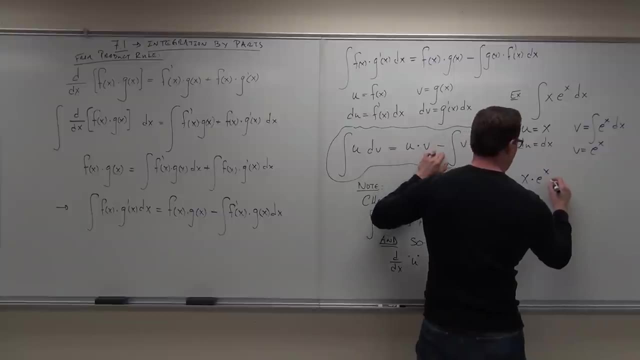 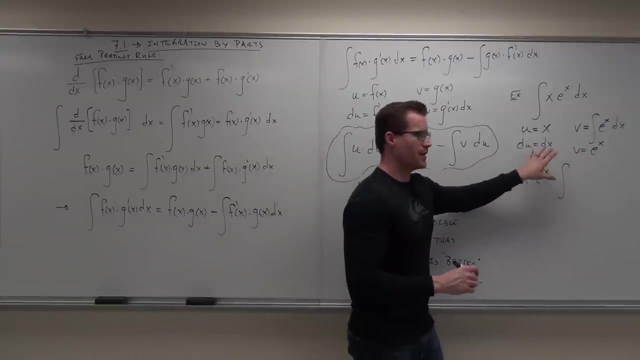 Yes, Put it in the formula. So what our integral is then is u times v, minus the integral. Notice there's another integral. You do integration twice here, One to find the v, and then again in your formula, e to the x. 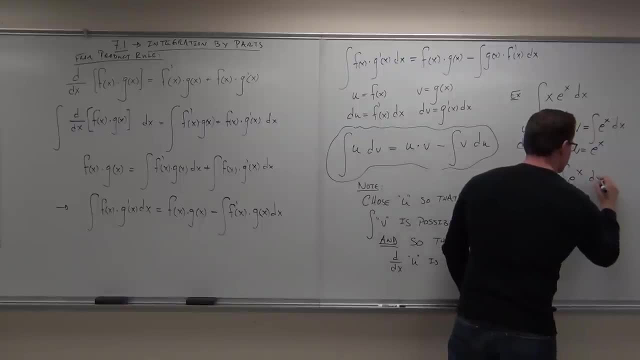 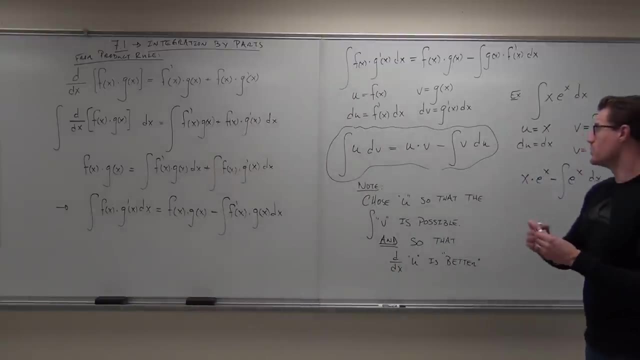 So what was the du dx? That's the idea. I need to make sure this makes sense to you. So we're picking u so that the derivative becomes easier and you can do the integral of the rest. The easy way to do this: identify what your u is, cover it up with your hand. v equals. 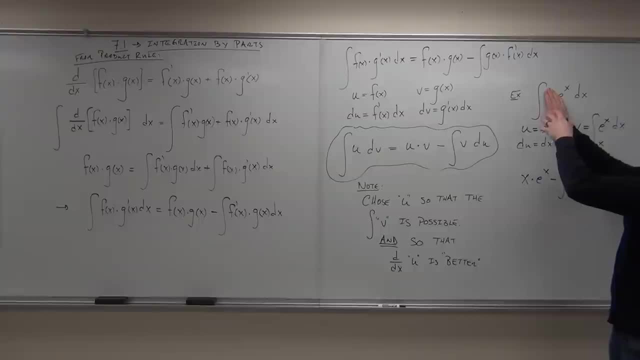 the integral of the rest. That's what v is for us. That's the easy way to do it. After that, well, find the derivative of u, derivative of x. du equals dx in this case is a really easy one. Do the integral of whatever you had left over. 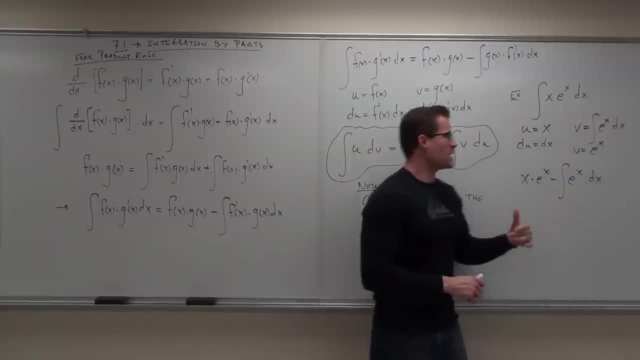 So that's e to the x. Now put it in the formula: Integration by parts says: integral of u- dv equals u times v, minus the integral of v du dx in this case. Now can you do that integral? Yes, How much is it? 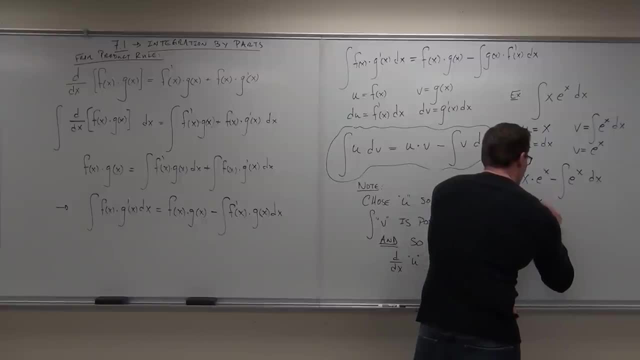 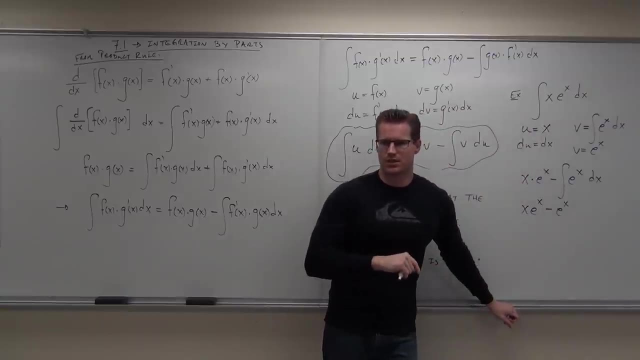 e to the x. So we get x times: e to the x minus. what e to the x minus, e to the x. This when you finish that last integral. that's where you do the plus c. You see you could get a constant here. 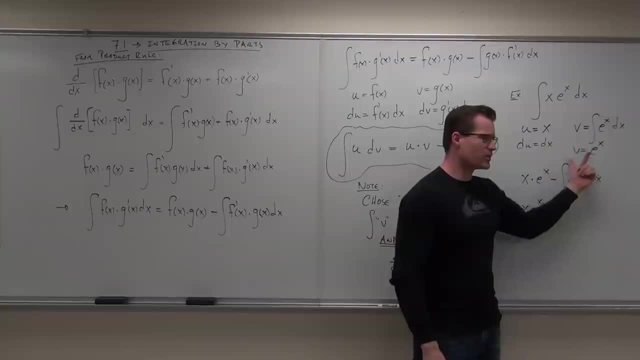 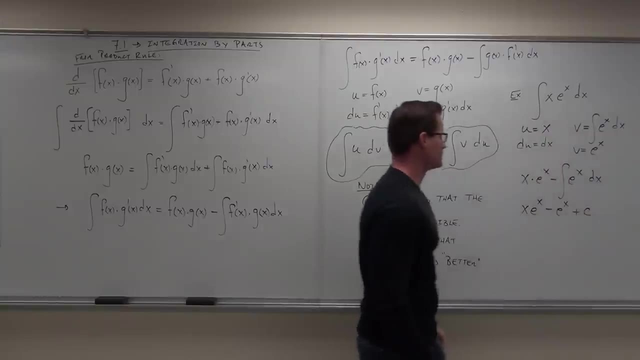 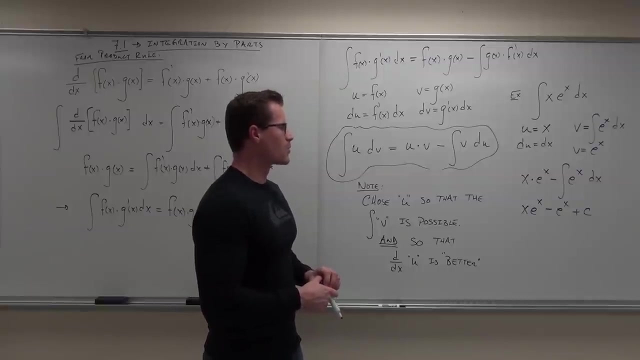 You could, But we don't need to, because you're saying: integral of a constant plus a constant would just be another constant. So we have a plus c here. You guys? all right with that one. Tell me one more thing that we could do. 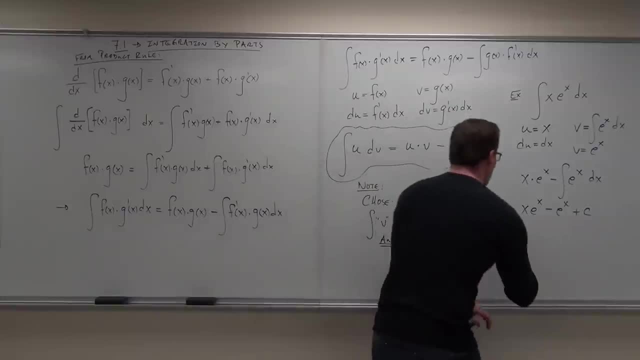 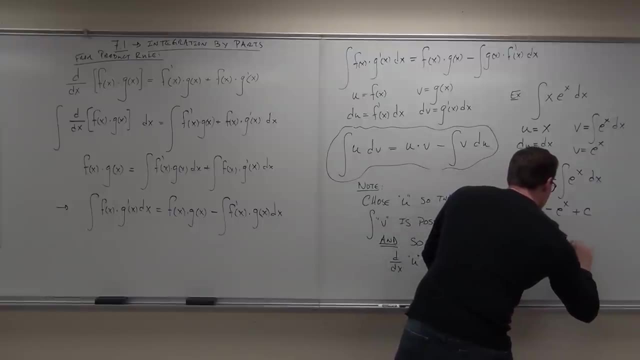 We could factor in e to the x if you want. A lot of times, with e to the x, you can factor in e to the x. So what we know is the integral of x e to the x, dx actually equals x? e to the x minus. 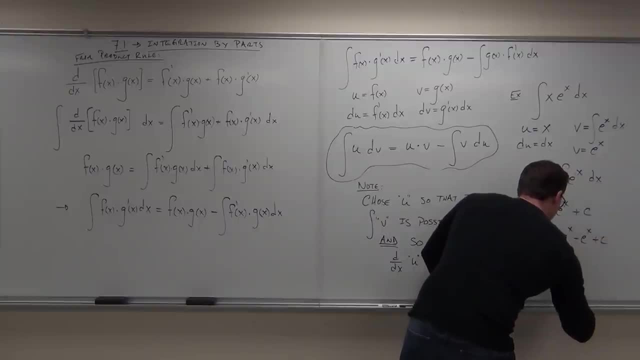 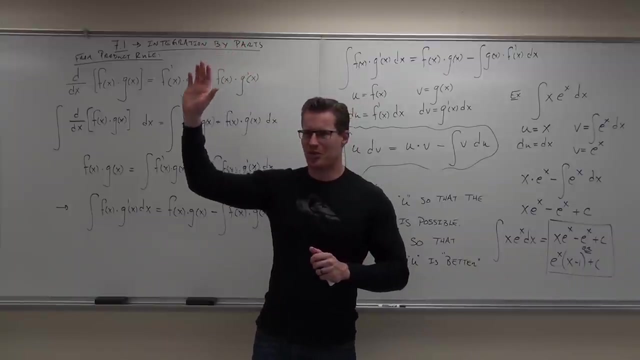 e to the x plus c or e to the x times x minus 1 plus c. Either one of those things Show of hands. if you can follow that one, You're probably going to need some more practice, right, Yeah, Okay. 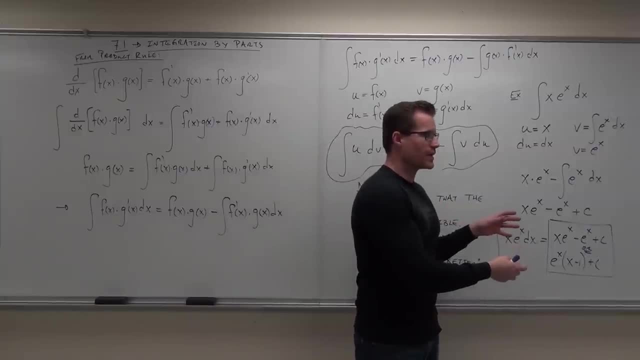 So we're going to do this one now. This is the first. This is about the easiest that we can do. They get a lot more intense. I should say. Not really any different idea, It's the same idea If you can't do a substitute. by the way, when you're doing integrals, don't jump immediately. 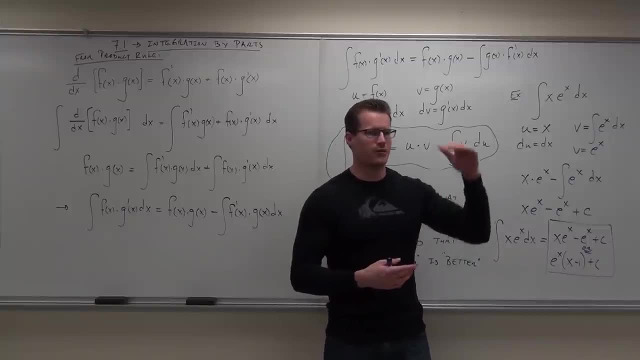 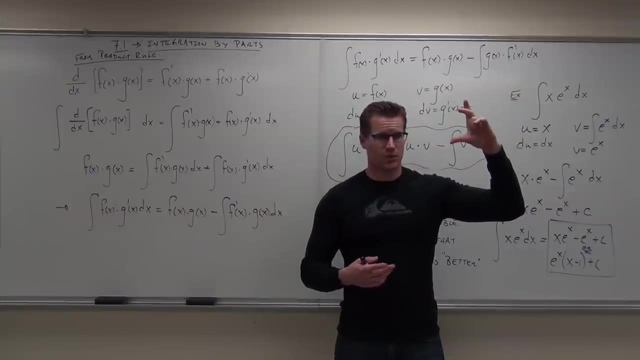 to integration by parts. Go through your list. If it's integration table, that's the easiest and you just do it. If it doesn't, you try what? first Substitution? Please try a substitution, because if you can do a substitution, that will be easier. 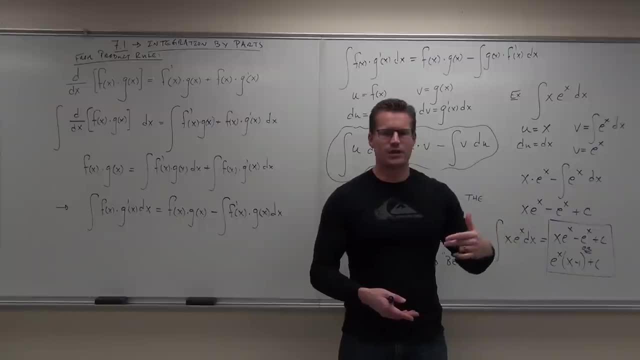 After that, then you try something else. After that, then you try stuff like integration by parts, Then you try trig, sub trigonometric substitution, which we haven't covered yet. We're going to cover that in this chapter, but that's later on. 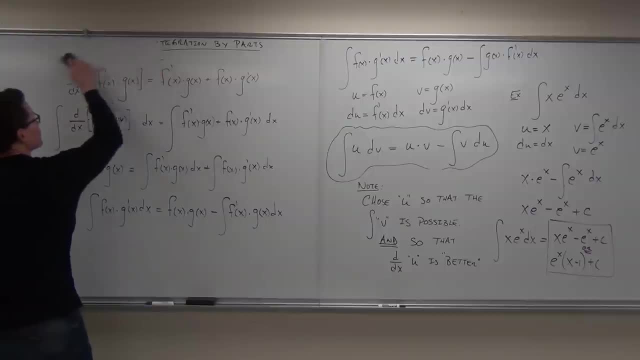 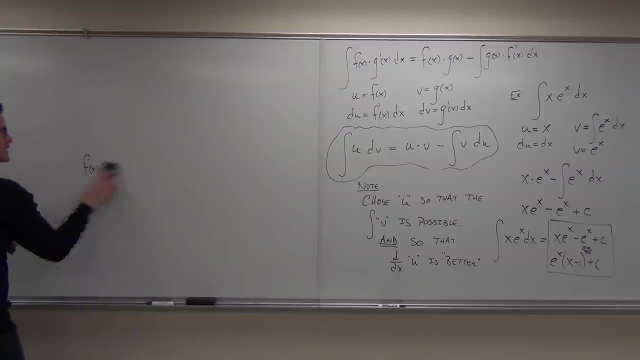 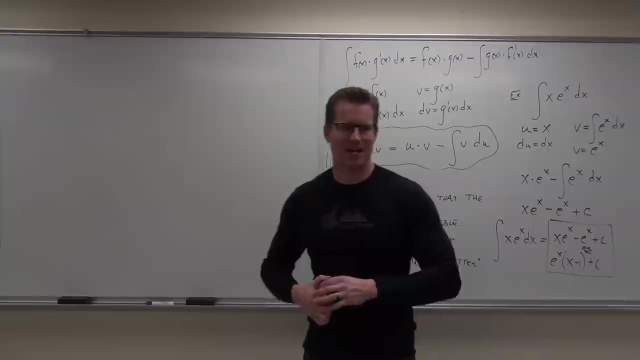 So let's try a few more examples. We're going to start building these up to more and more intensity. That way you get used to doing some of these problems I don't want to give you just like spoon, feed you and then, on your test, just hammer you. 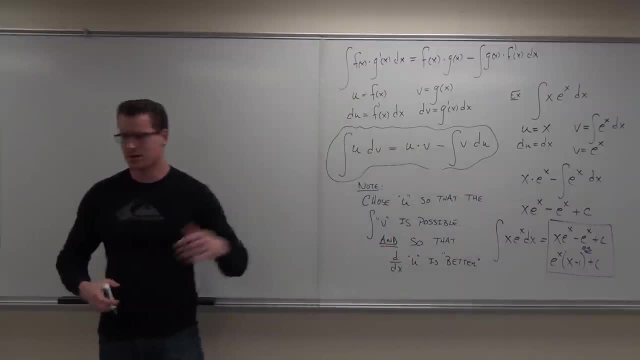 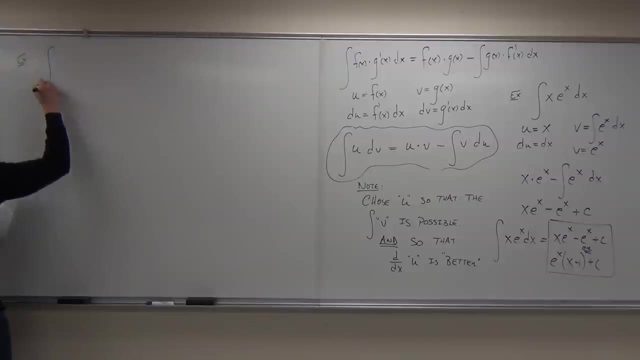 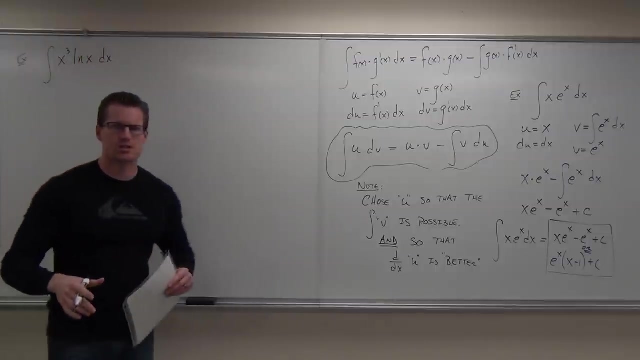 with some hard ones. So we're going to do some hard ones here in a little while, but I want to get you used to this first. How about I'm also going to try to make some mistakes? That way you can see the appropriate choices and when you will realize that you've made? 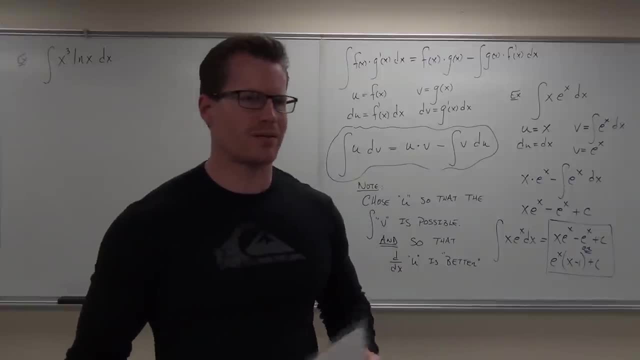 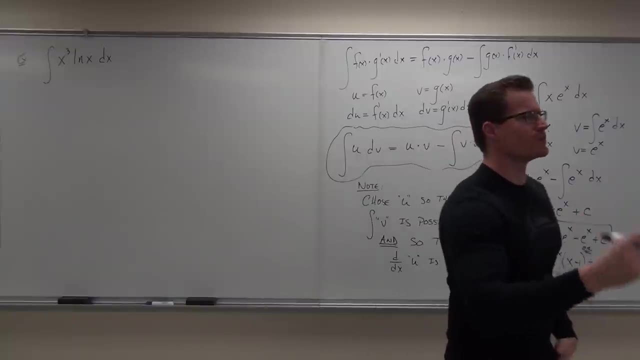 the wrong choice. Does that make sense to you? You're going to go. oh man, that's what happens when you make the wrong choice here. Take a look at it. The first thing we always check for what is it when we check integrals? 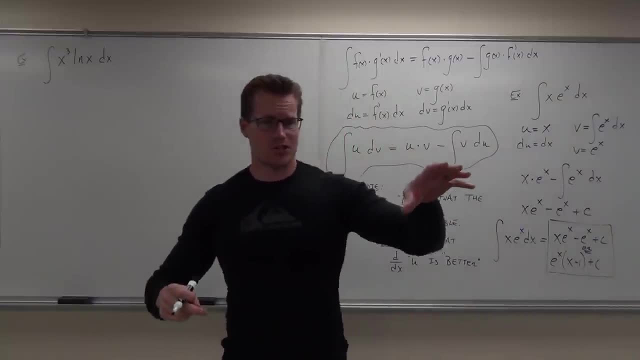 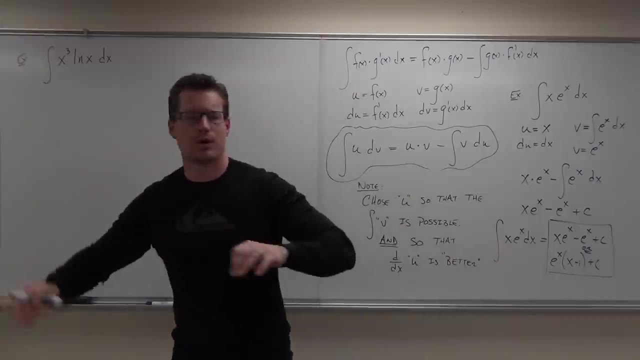 What do we check for User? We check to see if it's actually in the table first. Is that in your table? Heck, no, most of them aren't gonna be okay, otherwise it'd be really easy. After it's not in your table, what do you try to do? 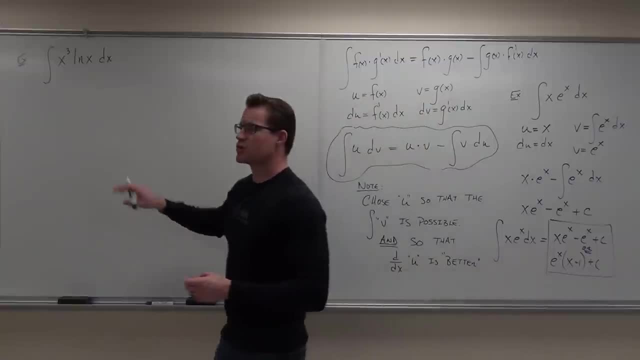 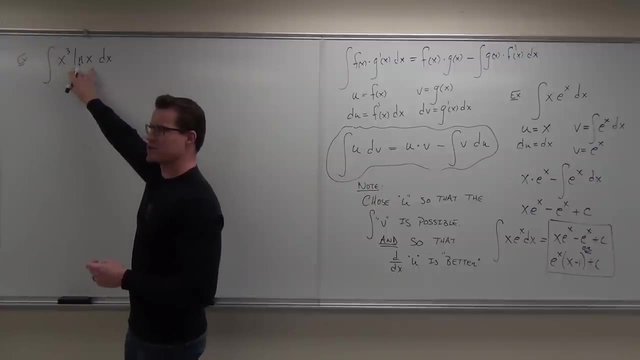 Now you try to do u sub. Is a u substitution gonna work here? If I pick this, the derivative is x squared. Do you see an x squared anywhere? No, If I pick this, that's one over x. Do you see a one over x anywhere? 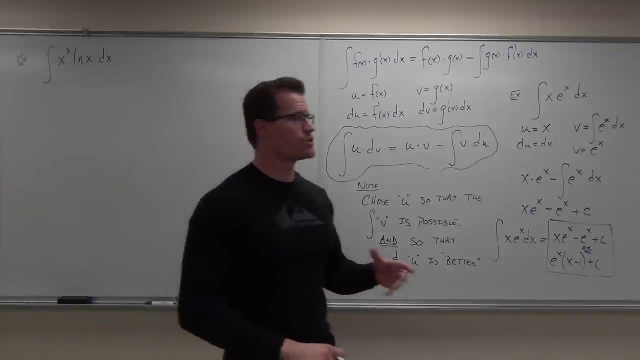 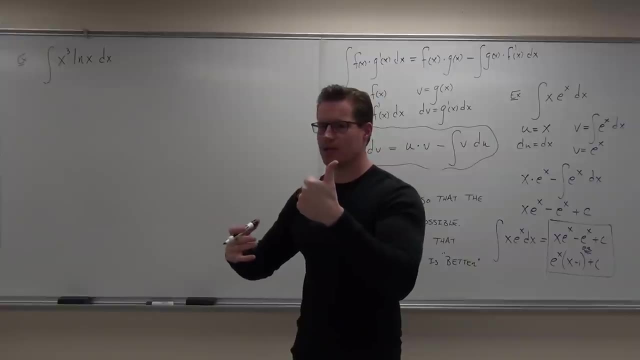 No, The substitution is not gonna work, Okay. well, if a substitution doesn't work, our next go-to. this is the model of thinking: you do, okay, Does it fit the table? If it does, awesome, If it doesn't, okay, substitution. 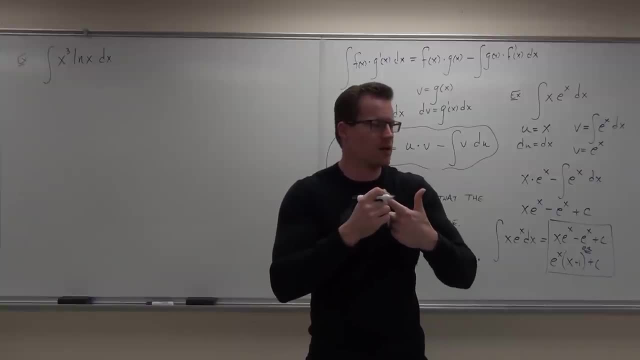 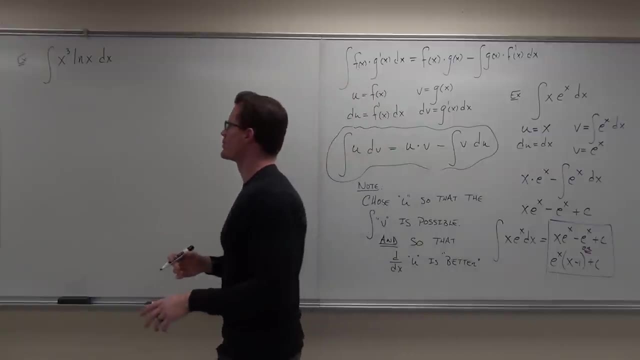 Does it fit substitution? If yes, cool, that's pretty easy. If not, dang it, then we got integration by parts. It'll still work. it's just a little bit more work, So go through and try to pick the appropriate thing. 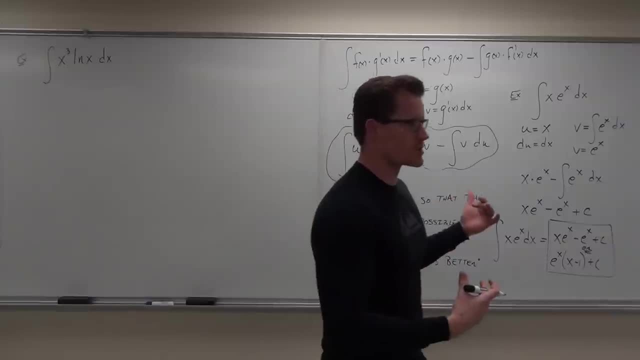 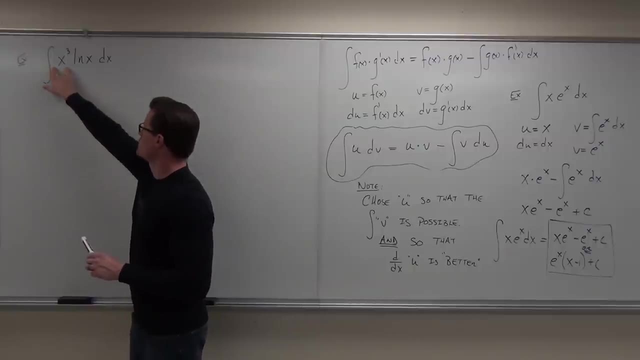 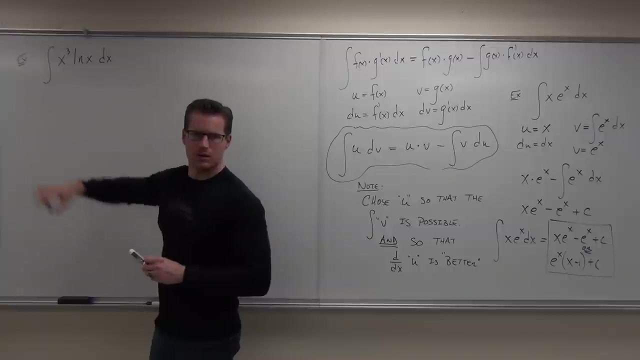 the appropriate factor for your integration by parts. So we got two choices again for our u. Our u could either be x cubed or it could be ln x. What would you pick for your u? Three x to the third, ln x. 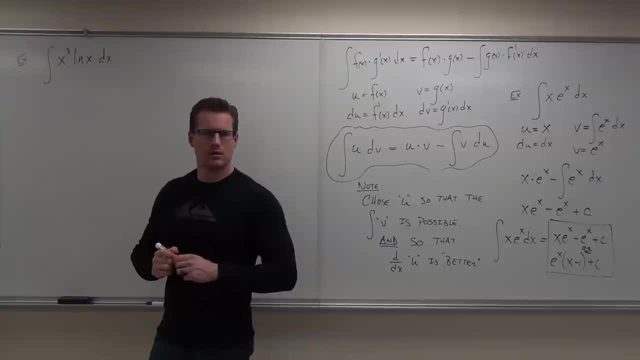 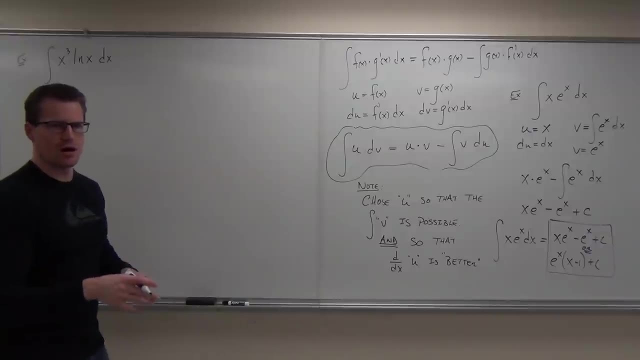 Why not x cubed? Let's think about it. I want to show you, though. check this out. Let's say that I picked. you can write this down or not, I don't really care. Let's say you picked, u equals x cubed. 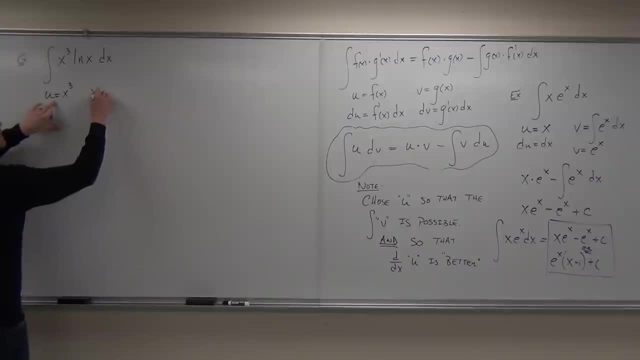 You with me. If you picked u equals x cubed, can you please tell me what your v would be? Oh, is that ln x? No, it's not just ln x. It's not just ln x, It's dx. 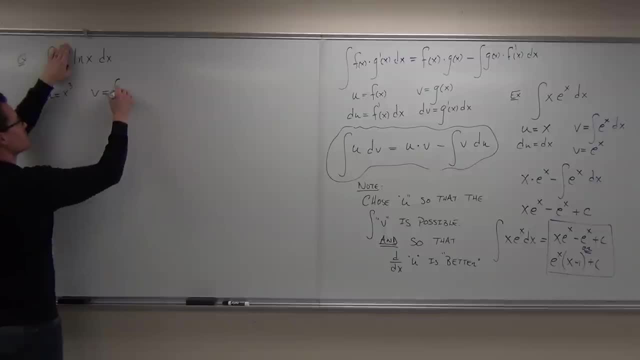 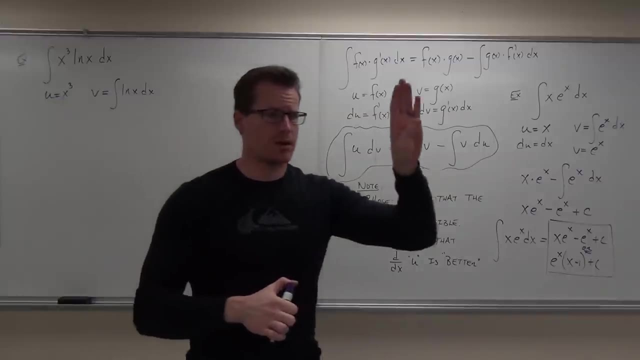 Don't forget that integral. My goodness, don't forget that. It's the integral of ln, x, dx. It's all of the rest of the stuff. Does that make sense? You're basically just covering up the? u, The? u is one part. 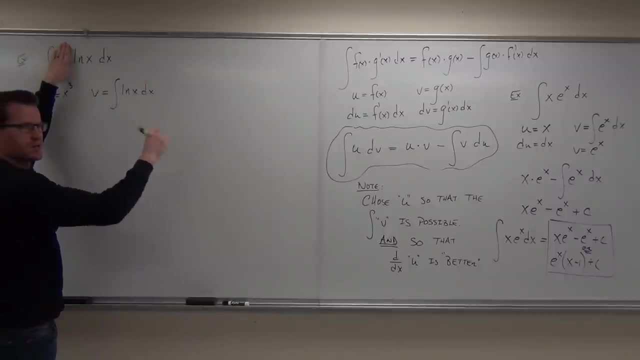 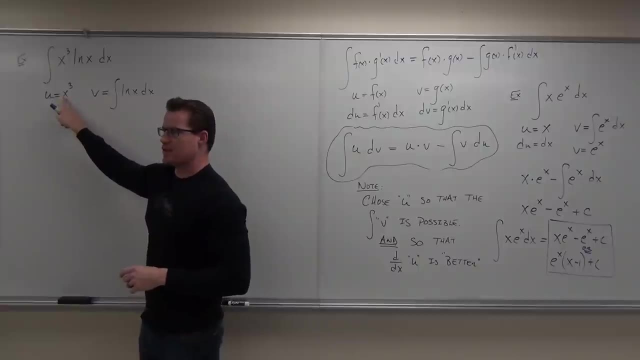 This is your u. V equals all of the rest of the stuff. So v equals quote, unquote the rest. So if you feel okay with that, it's a big deal, All right. Now could you take the derivative of this? 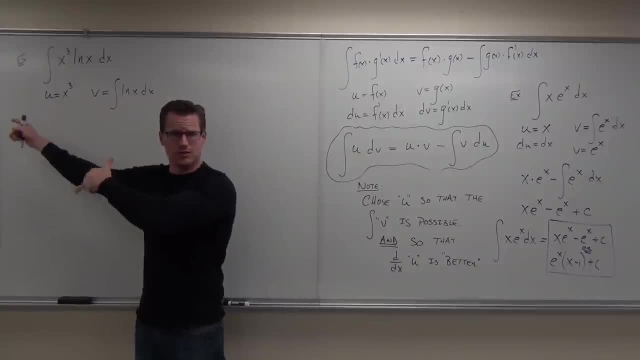 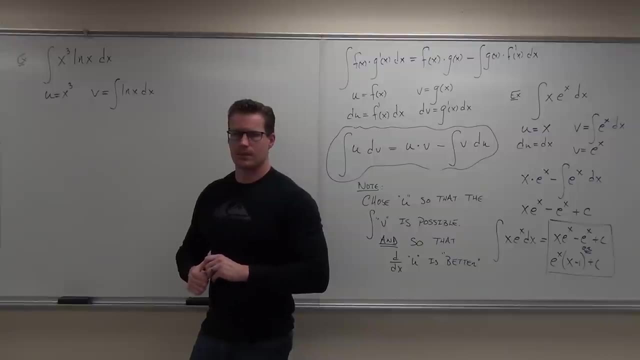 Yeah, We can take the derivative of darn near anything, And that actually makes it easier for this one. Can you take the integral of ln x? You can. What is it? The one over u, The one over u? Okay, I'm not asking for the derivative. 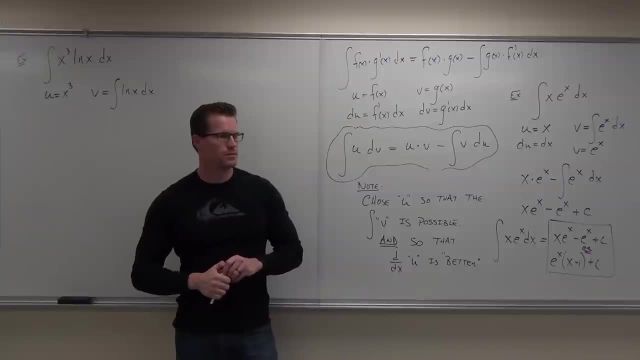 I'm asking for the integral One over x. The derivative of ln x is one over x. What's the integral of ln x E? No, it's not E, O. Well, I don't know What is it. 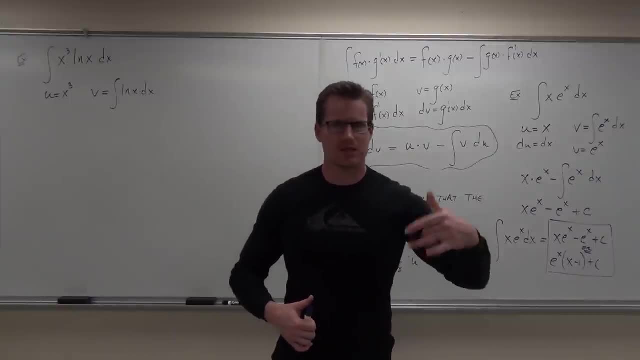 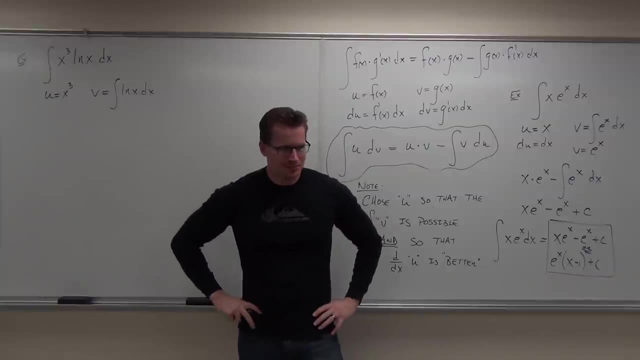 Can you do it? No, You can't, actually, I don't want to, I don't know You can't. You can't actually, I don't know, I don't know, You can't, You can't do it. 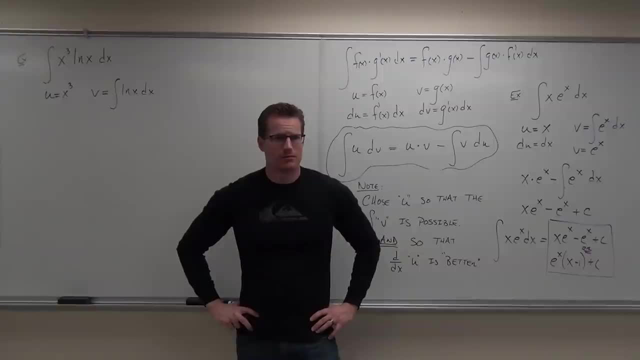 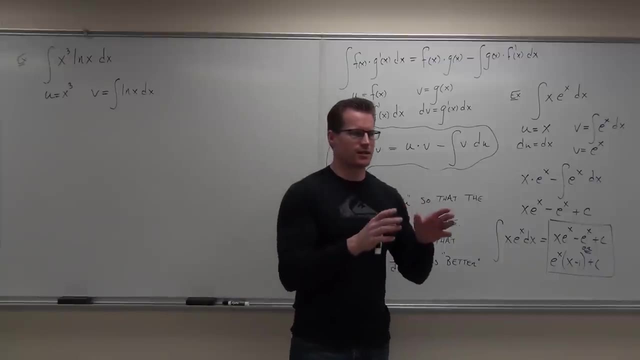 I don't know, I don't know, I don't know. Can you do it? Well then, if you can't do it, then we've picked the wrong thing. Does that make sense? Yeah, You need to pick. listen, listen, listen. this is not a trivial point here. 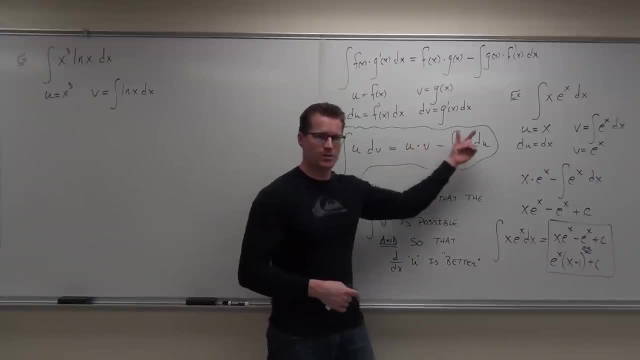 You need to pick u so that hopefully the u becomes better, the du makes it better, But if not, okay, the main thing here is that you can actually do the integral of v, Because if you can't, then you're stuck. 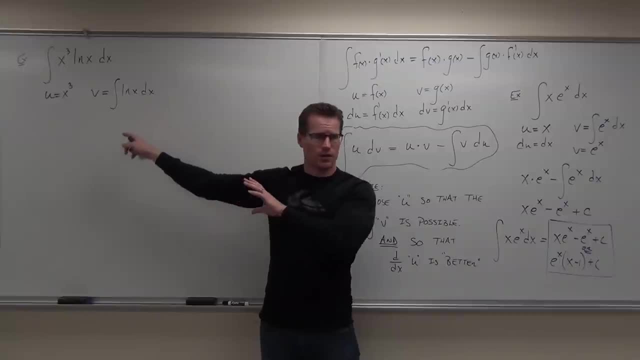 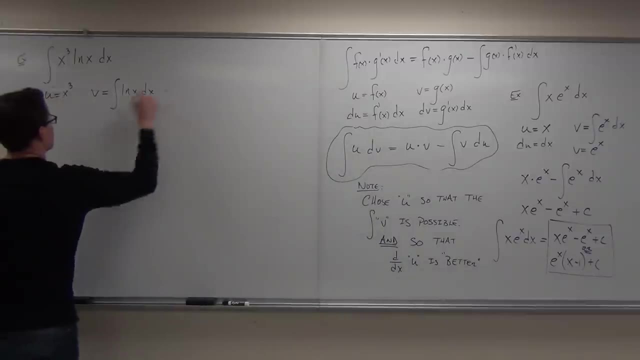 None of you right now, unless you've had this class before, know what that integral is. Do you know what the integral of ln x is? No, you don't. So we made the wrong choice. This is a bad choice? Well, if that's the bad choice, don't beat yourself up over it. 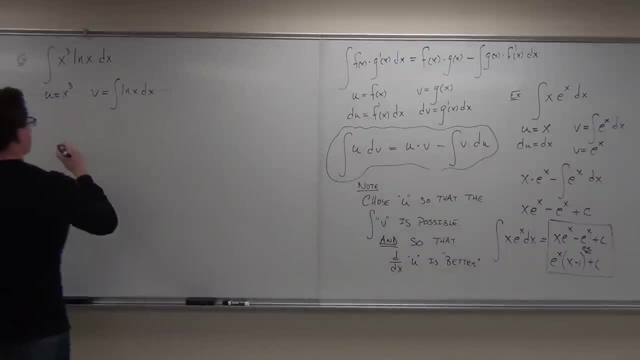 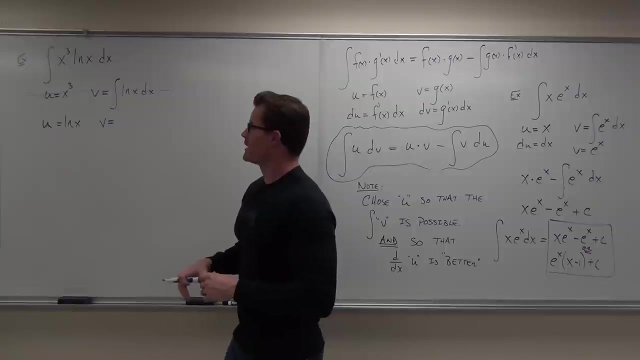 Just erase the problem and pick the different thing. What should our u actually be? Okay, cool What you said all along genius. So if u equals ln x, can you please write down what the v is going to equal? Well, that would be 3x squared. 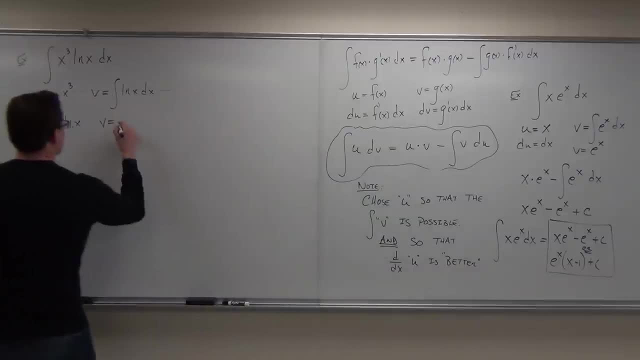 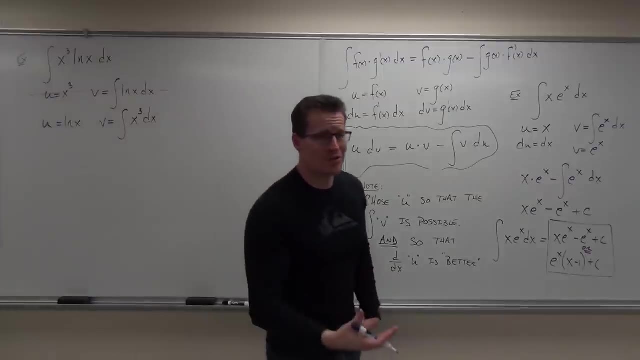 No, it wouldn't be 3x squared. No, it wouldn't be 3x squared. We still got an integral, don't we Listen? I'm not lying to you. All you do is cover this up. Sorry, cover that up your u and write the rest. 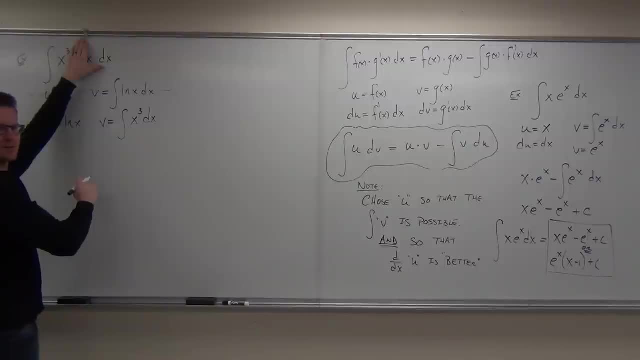 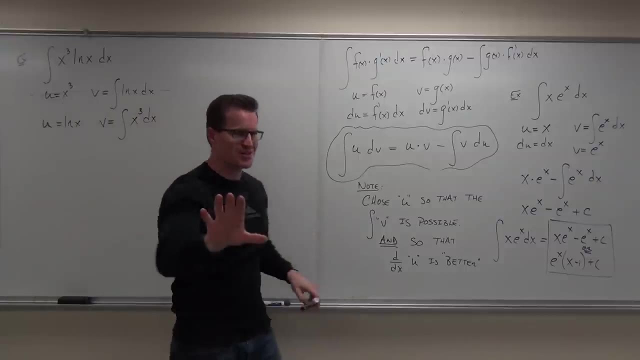 Whatever you see, that's what goes for your v. It even rhymes. Don't you love rules that rhyme? Whatever you see is what goes for your v. I'm not going to. You can watch me go. I'm not going to. 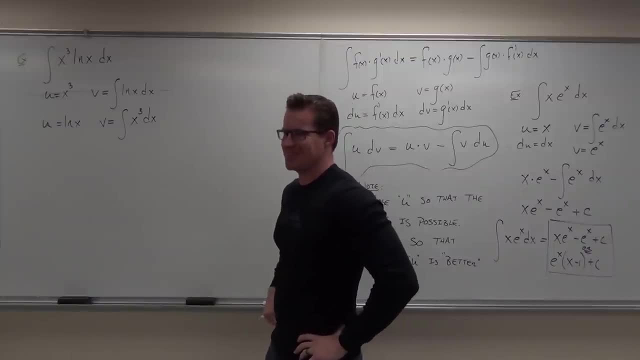 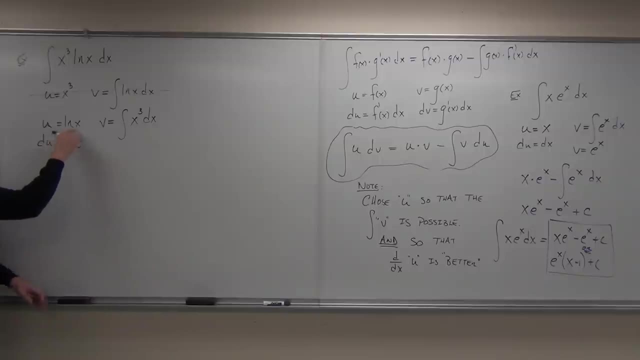 I'm not going to, I'm not going to, And then, And then. Yeah, I feel victorious right now. Can you take the derivative of this guy? Okay, what's the derivative of ln x? One over x? Hey. 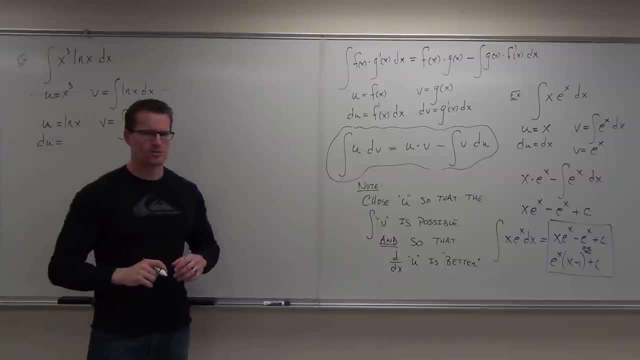 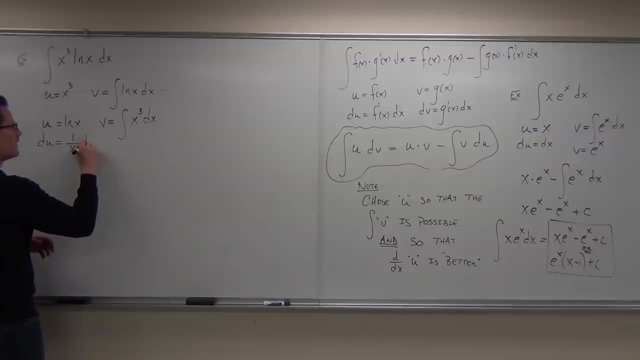 The only thing where the derivative equals the integral is when you're dealing with e to the x. okay, That's it. ln, x is different, So we get one over x. Ah, good, Now with v, we're not doing derivative here. 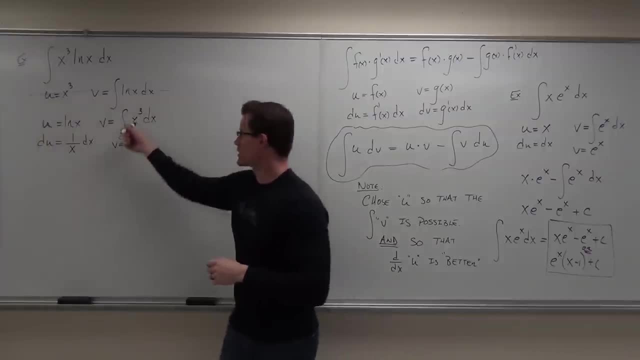 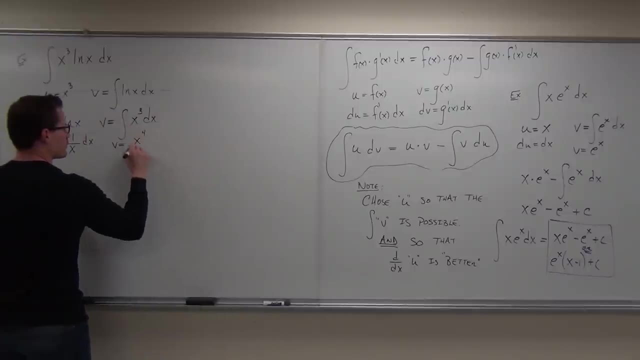 we're actually solving this integral. Can you do the integral of x to the 3rd? Then we've picked the correct choice here. okay, The other choice didn't work. This choice: we get x to the 4th over 4,. 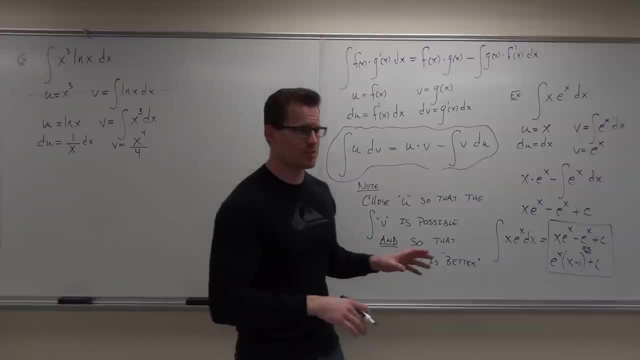 or 1- 4th, x to the 4th, I don't care how you put that. We don't need a plus c because we're just using this in our formula right now. We'll have the plus c at the very, very end. 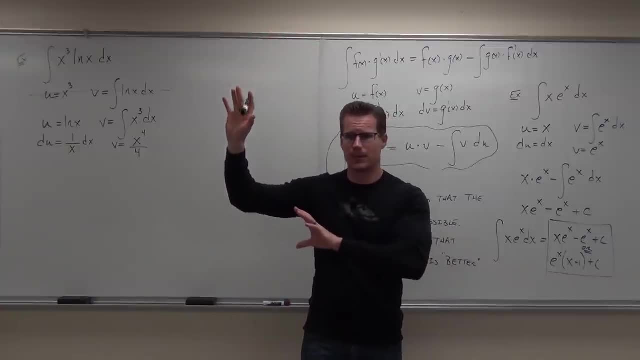 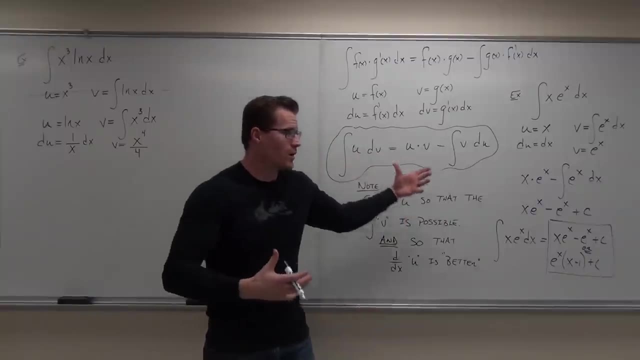 So, if you guys feel okay with that one and do you understand why we picked the? u the way we did, Good, that's important. That's the hardest part of this is picking the? u correctly, Honestly it is. The rest of it is a formula which you know how to do. 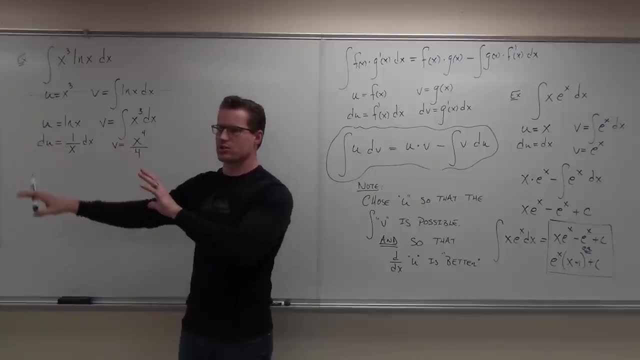 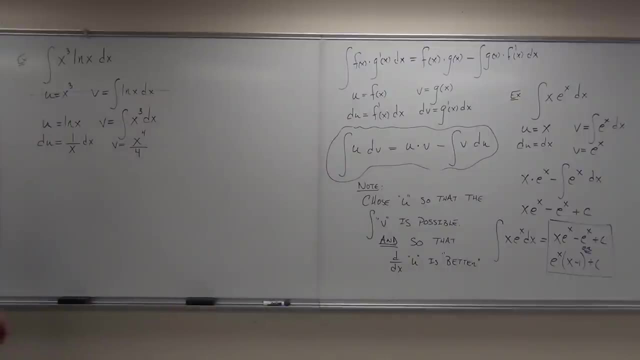 You know how to do easy integrals. You know how to do all sorts of derivatives. You're good to go, Just use the formula. So what the formula says is that the integral of u- dv equals u times v minus the integral of v- du. 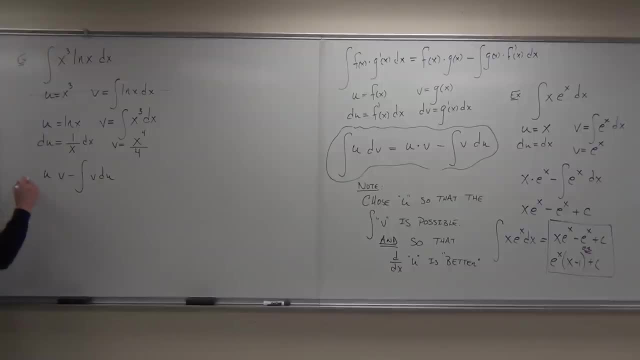 Just plug in the pieces. Watch this real careful, though. Make sure you plug in the pieces correctly. Can you please tell me what the? u is Good right here? That's our, That's our? u times, our v. Do the v that you actually solved for. 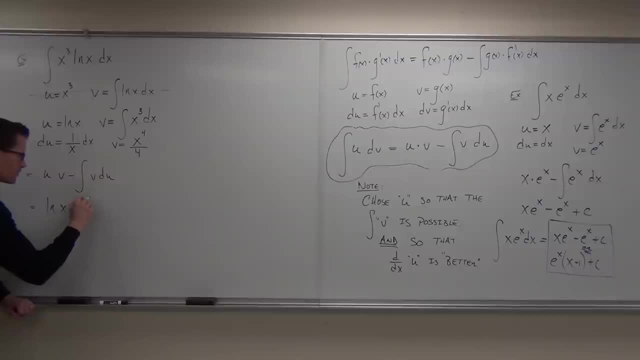 Go with the integral again. What's the v? You guys? okay, on the? u times the v. We got a minus sign. Put a minus sign. We got an integral sign. Put an integral sign. Put the v. here again, The v goes in two spots. 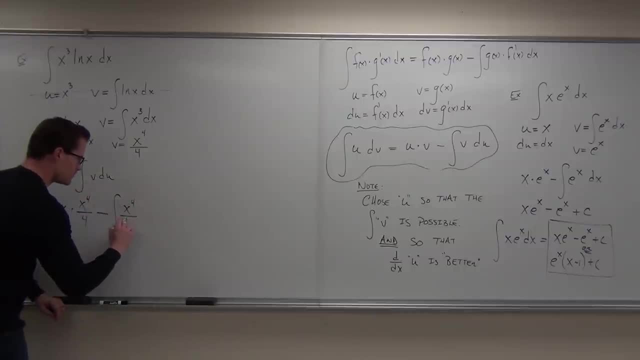 v goes here. v goes here. Now stick with me. ln x x to the fourth over 4, minus sign. Got it? So ln x x to the fourth over 4, minus sign. Integral integral x to the fourth over 4 again. 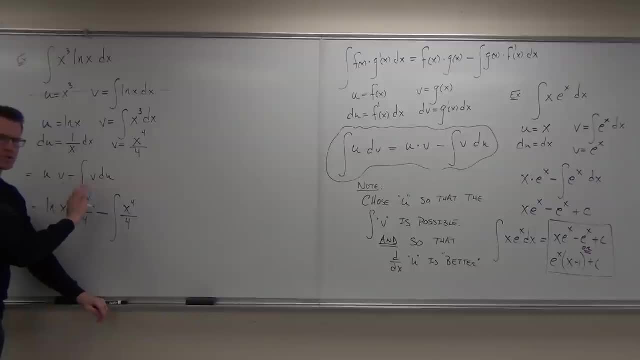 That's our v. Now look at your du. Your du is not always dx. Your du depends on what you picked for your u. What's your du? 1 over x dx. So we need 1 over x dx. It's different than substitution. 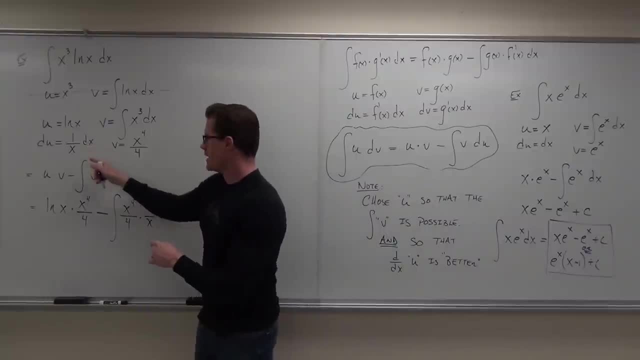 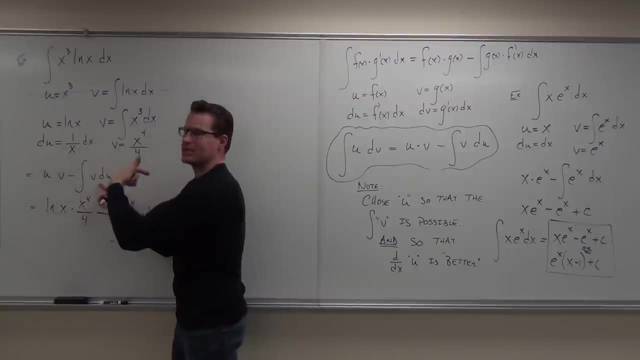 It's different. You don't start solving for the dx here. The formula says you're going to take this and put this whole thing where this is. You don't start solving for that like some people do, like I do, for substitutions. So if your u is ln x, put that. 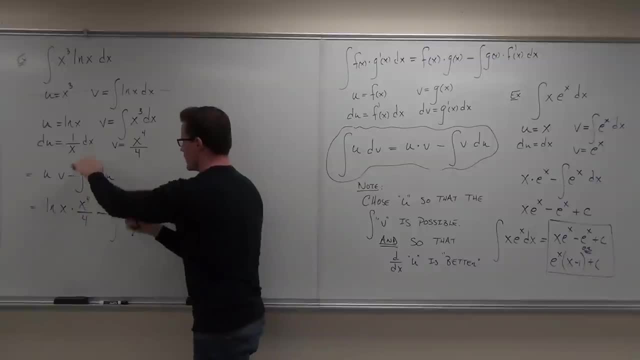 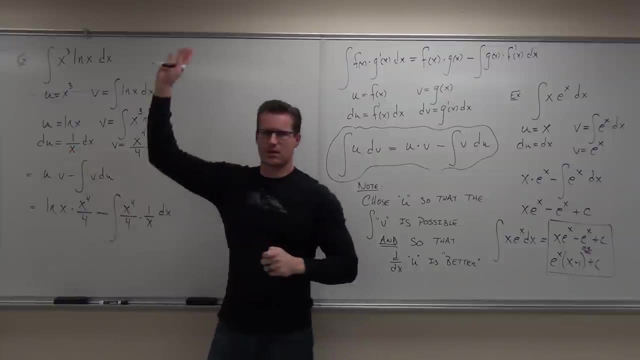 If your v is x to the fourth over 4, put that Minus no problem. Integral, no problem. v is x to the fourth over 4, put that du is 1 over x. dx Show of hands. if you understand the concept. 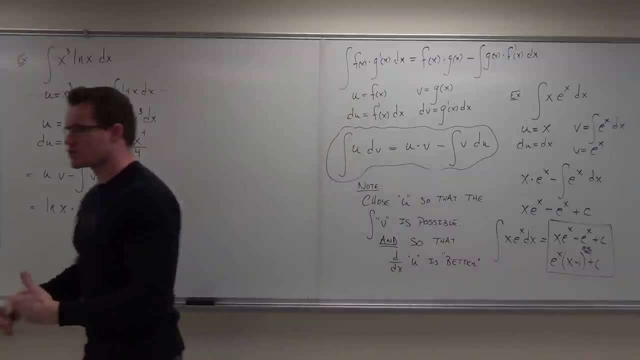 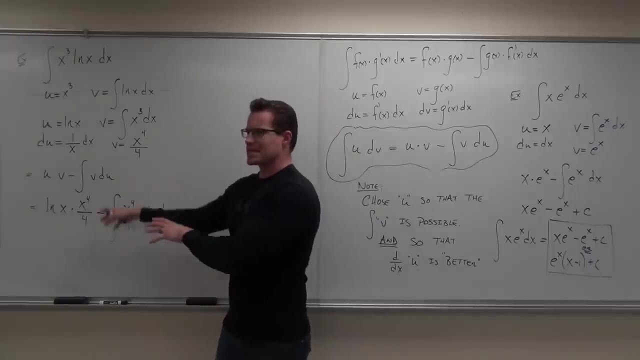 Good, Now simplify it, Solve it. This should be solvable. If it's not solvable, listen carefully, please. If this isn't solvable, it's the only piece of calculus you have left right. If that's not solvable for you, if you can't do that, try a substitution. 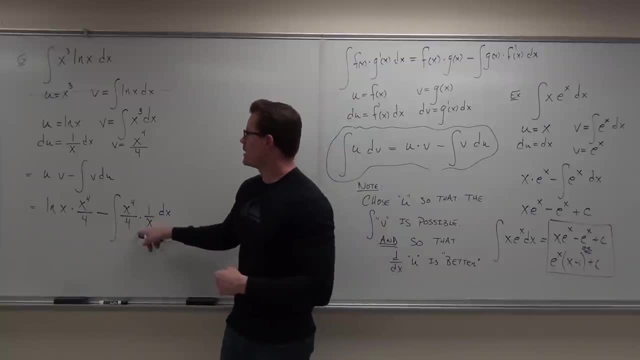 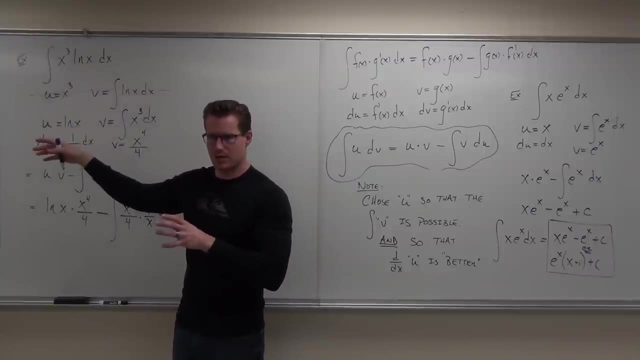 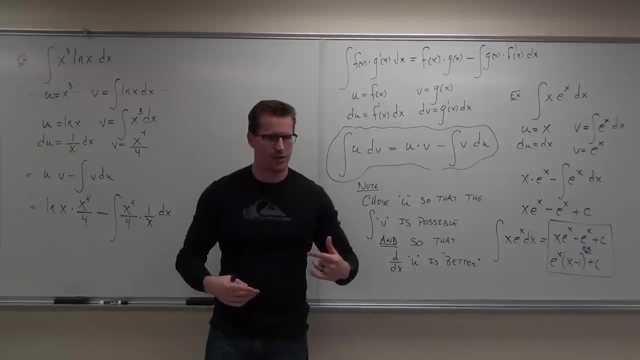 Or try another: integration by parts. If this thing explodes way bigger than this thing, then you've picked the wrong choice and tried the other u So you shouldn't be making these way way worse. They should start getting better. Smaller powers and things like that. 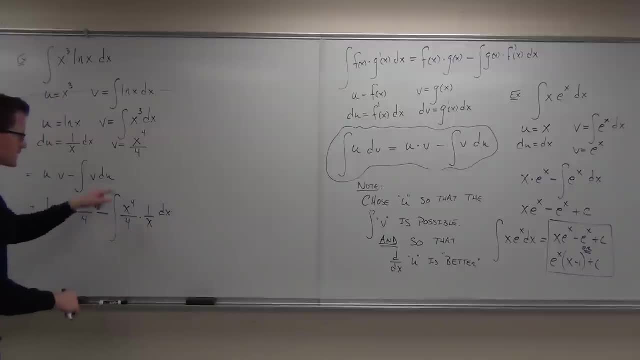 Or a doable integral. This will actually get the same power back, but we can do the integral. So in our case we got ln x times x to the fourth over 4, minus the integral. What are you going to do with all this stuff? 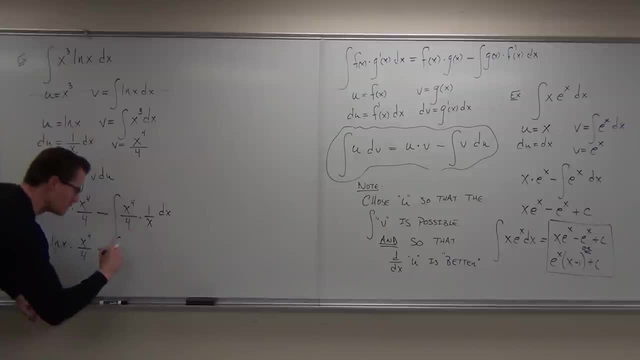 Tell me something you can do: Combine, Combine. How much did we get? x to the fourth over 4.. Not x to the fourth, No. x to the third. x to the third, yes, And then we can also do what. 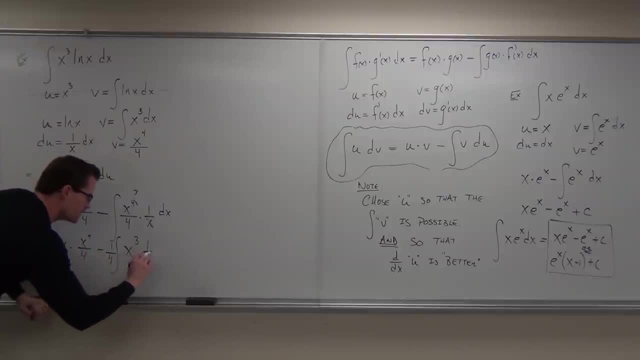 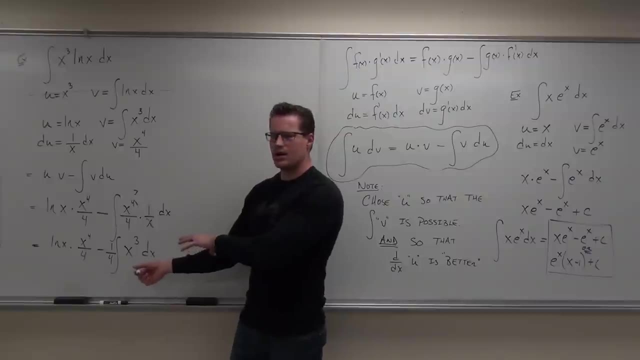 Bring the fourth, one-fourth out. Maybe one-fourth out front would be a good idea. Hey, does that look like something you can do? Yeah, I sure hope to goodness that you can. I mean, that should be an easy one. 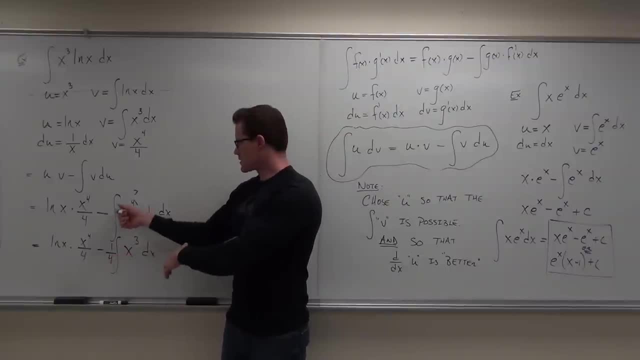 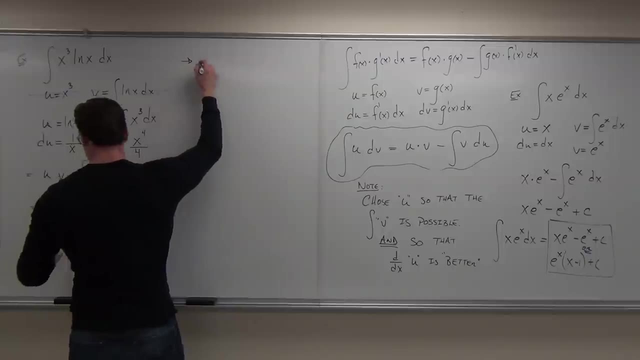 You guys? okay with the algebra on that one. Yeah, One-fourth comes out x to the fourth. You should know how to simplify here. Yeah, So let's keep after it. This one. I'm going to write a little bit different because I don't like having my ln x first. 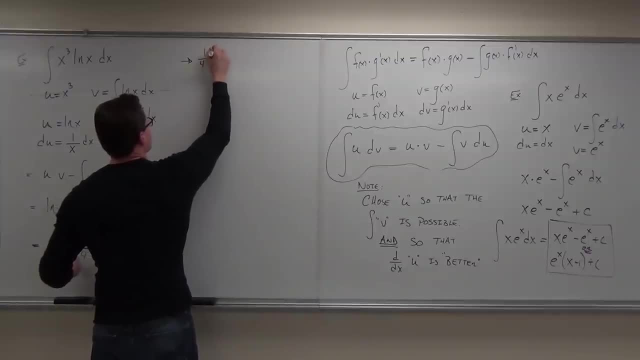 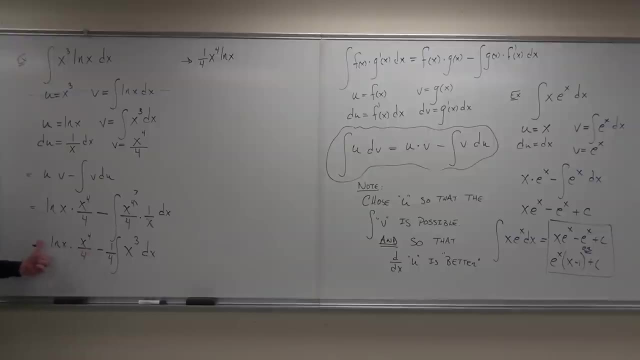 So I'm going to write one-fourth x to the fourth ln x. You all okay that that's the same thing: One-fourth x to the fourth ln x Minus one-fourth. Hey, look at that. Now we can do an integral of something that's really really, really easy. 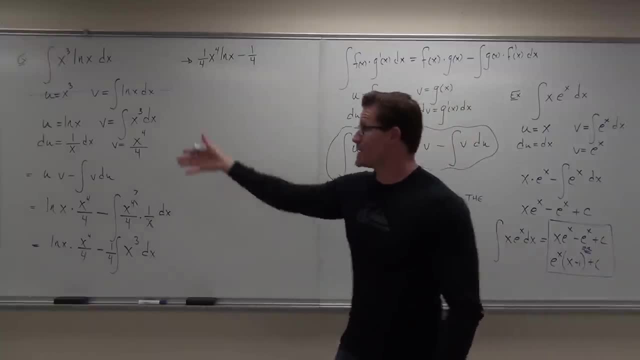 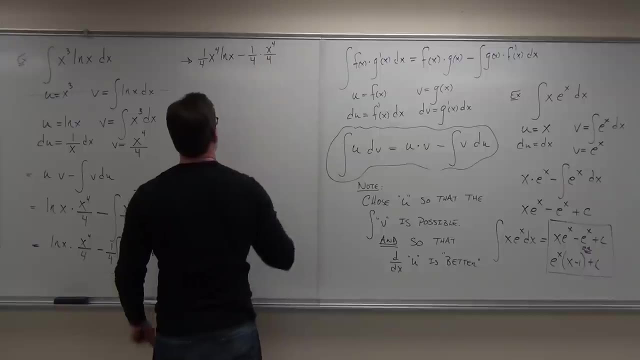 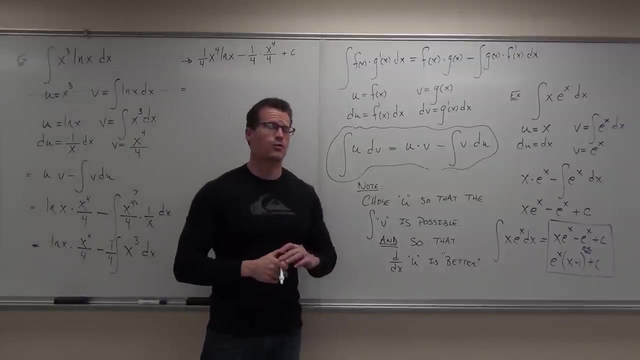 What's the integral of x to the third? One-fourth, In fact, we already did it, Yeah, One-fourth. Now is where you put your plus c. Yeah, Is the plus c important? Yes, Yes, Don't forget it. 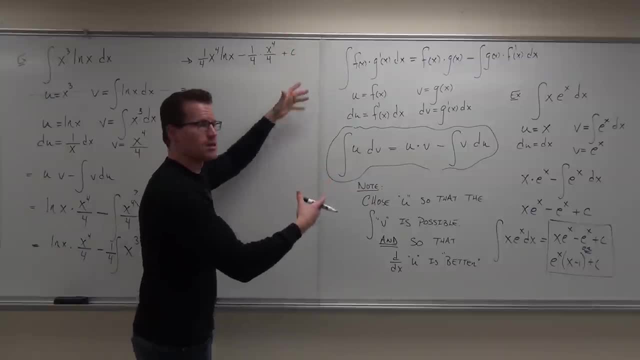 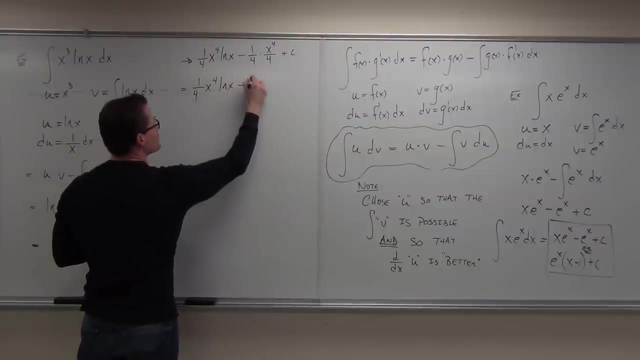 Okay, So don't do all this work and then go I'm done. No, you're not done. Put the plus c. Let us know that that happens. So one-fourth x to the fourth ln x, No problem, Minus one-sixteenth. 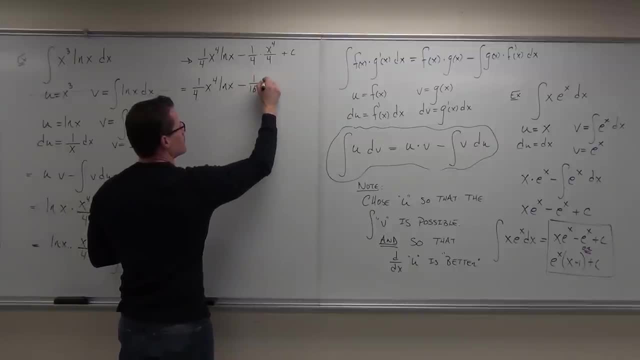 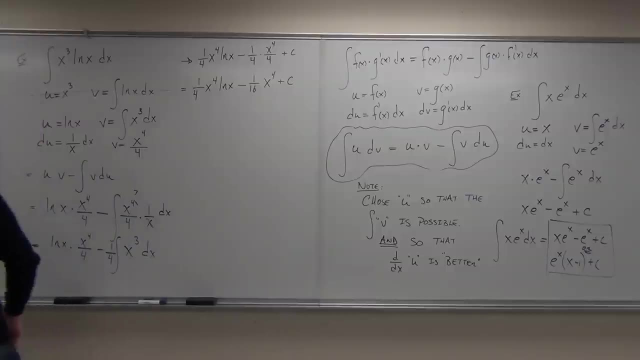 See where that comes from. Yeah, Yes, No, Everybody. Yeah. x to the fourth, x to the fourth. Let's see, Could you do something like that? Yeah, Yeah, Yeah, Yeah. Could you do some other things with it? 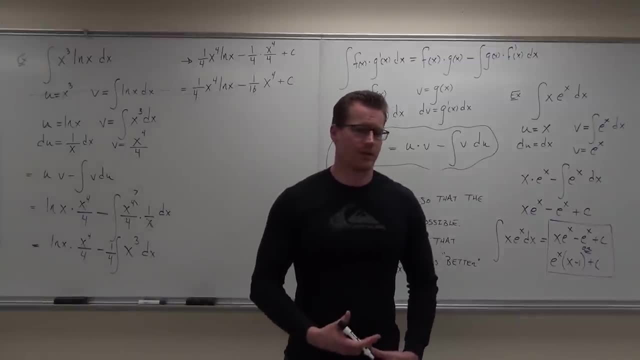 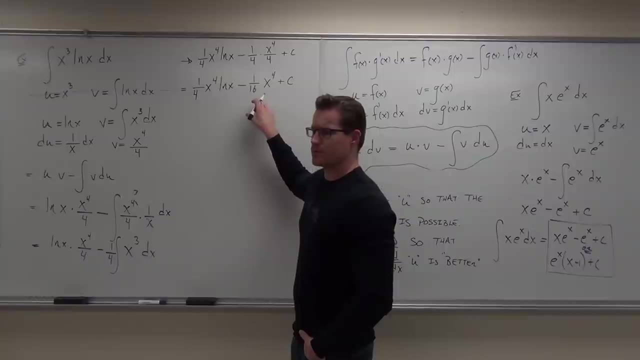 Factor out x to the fourth. Factor out x to the fourth. You can do a lot of things with this, okay. Factor out x to the fourth. You could factor out x to the fourth. You could actually force this thing to factor out a one-sixteenth or a one-fourth or a sixteenth. 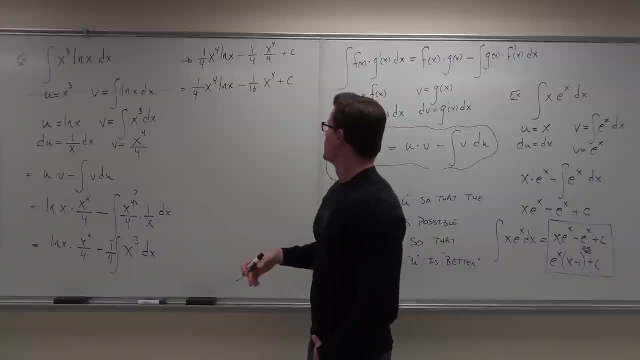 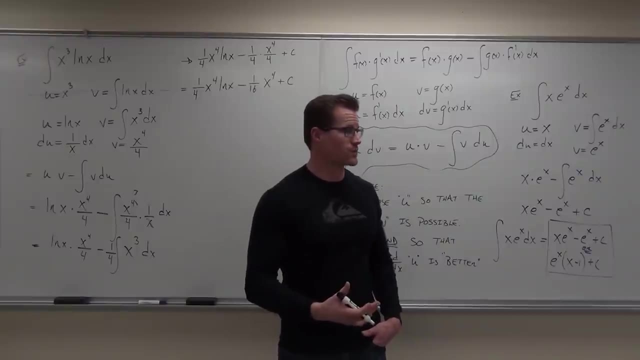 You could factor out a lot of stuff here. So if you did, it's going to look a little different. So keep in mind when you look in the back of your book, if it looks different, they might have just started factoring things. 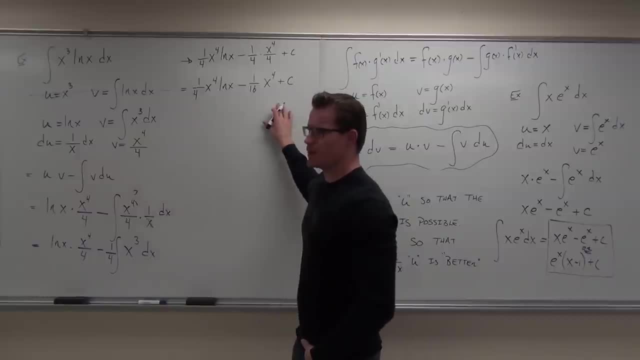 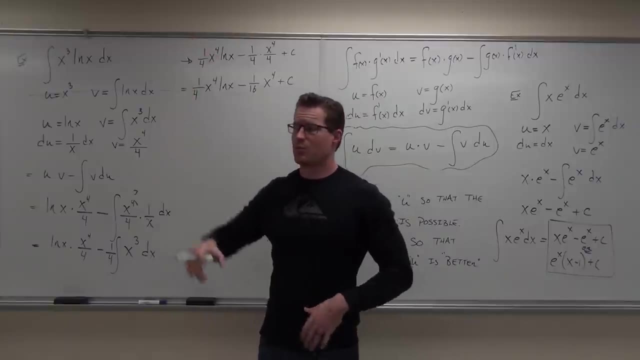 So don't give up on it. If you're a man, I think I'm right. Start factoring something. See if you can see a common factor that they have. Okie-dokie, Should I feel okay with that one, Can we build it up just a little bit? 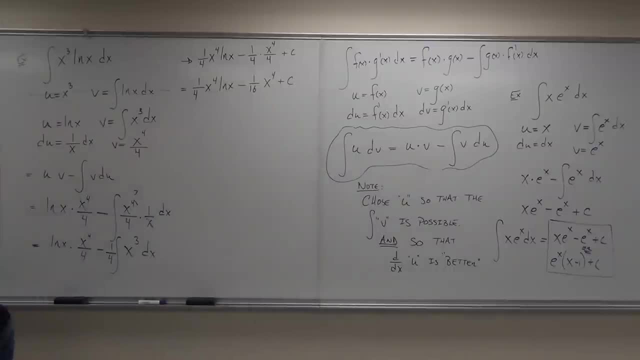 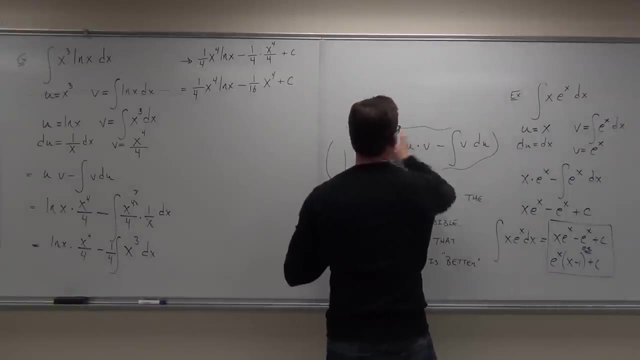 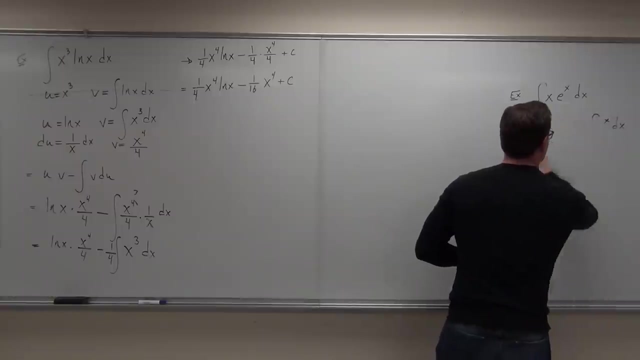 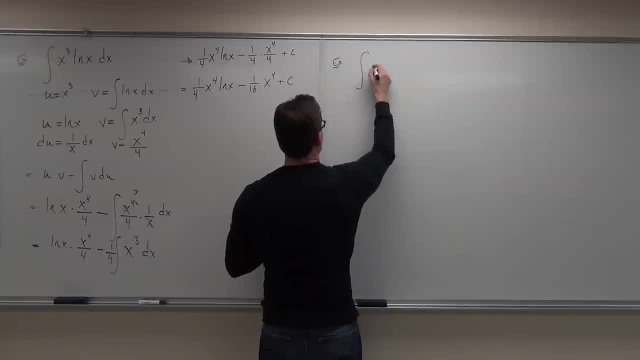 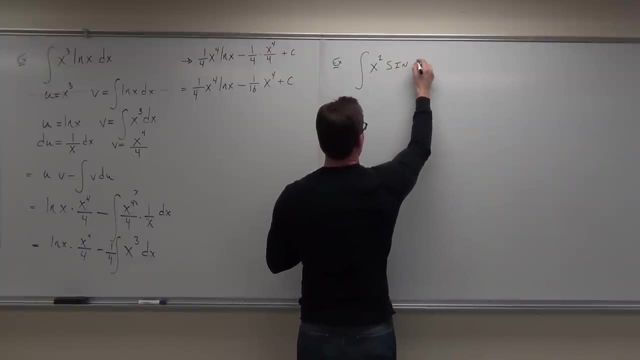 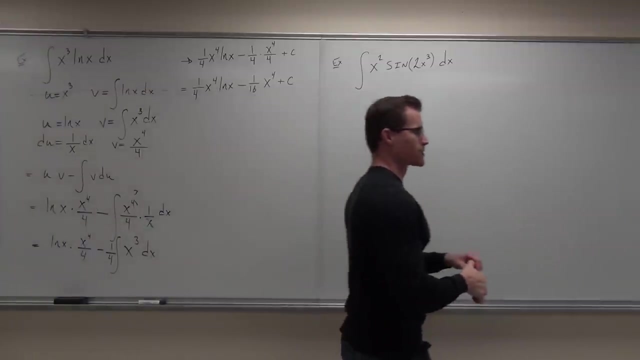 Okay, Okay, Okay. I'm going to change these problems slightly in just a moment, But I want to ask you a question first. What do you check first What you're doing In your tables? In your tables? Ok, Just a table. 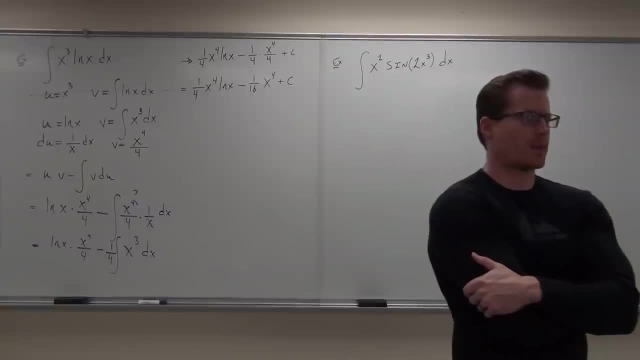 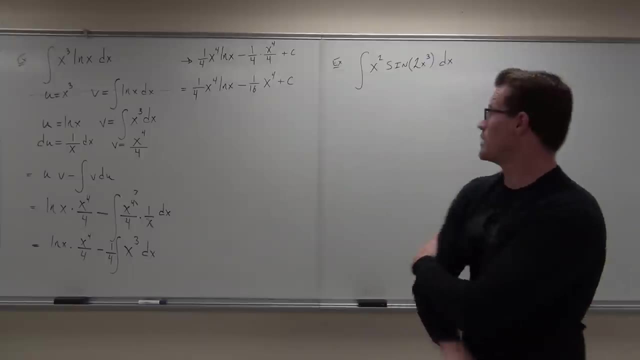 Okay, does it fit your table? No, Next you check for: will a substitution work here? No. Look again, Will a substitution work here? Absolutely, Because the derivative of this is 6x squared. do you see it? Your x's are gone. 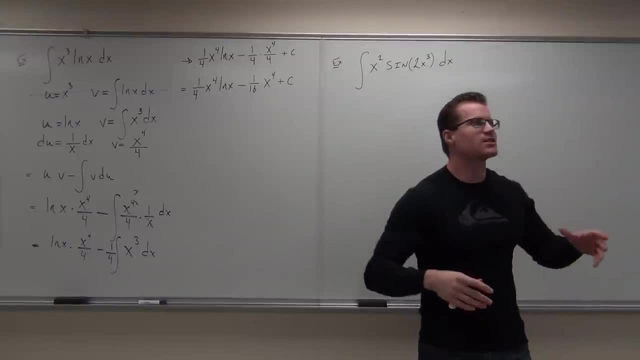 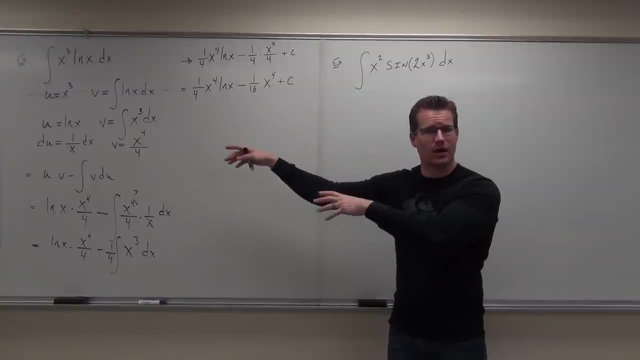 So if I gave you this problem, this is my whole point, which some of you obviously didn't listen to. my whole point is: do not jump automatically to that. that's silly. okay, Try a substitution, if it'll work Here. don't do this problem. I told you I'm going to change it in a minute. 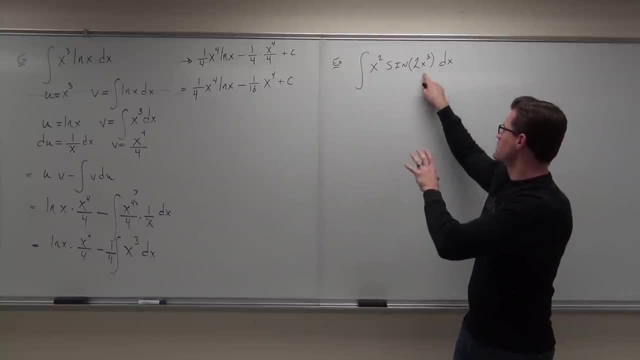 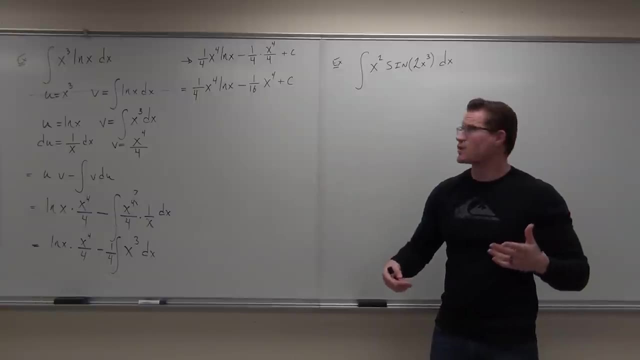 So this: this would be great for u sub. u equals this derivative of 6x squared. x squared are gone. you pull out a 1 sixth. you're basically done. You're going to get negative cosine 1 sixth, negative cosine of 2x cubed, if I'm right. 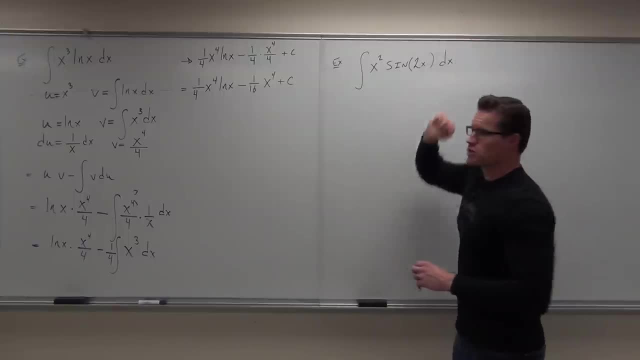 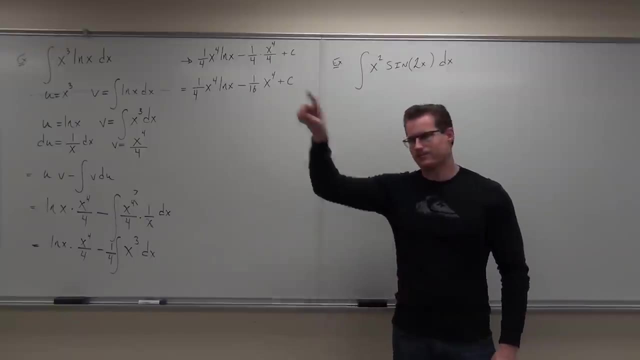 plus c, Done easy. Will a substitution work now? No, No, No. So what are we going to do? Parts, Parts- The next one. You always check a substitution before you check integration by parts. I hope that I'm getting this right. 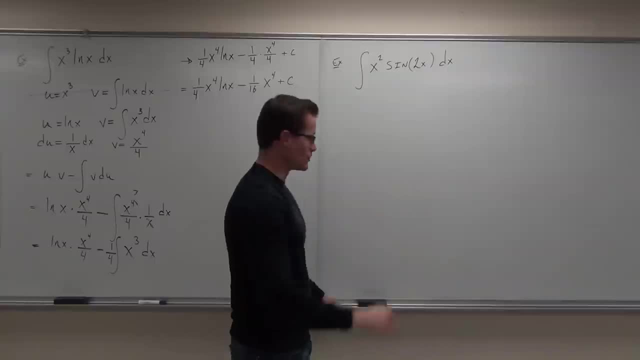 I'm getting through to you right now. I'm getting through to you right now: Always check that, because it'll make it easier if it'll work. So, oh man, let's see here What's a good choice. What do you think? 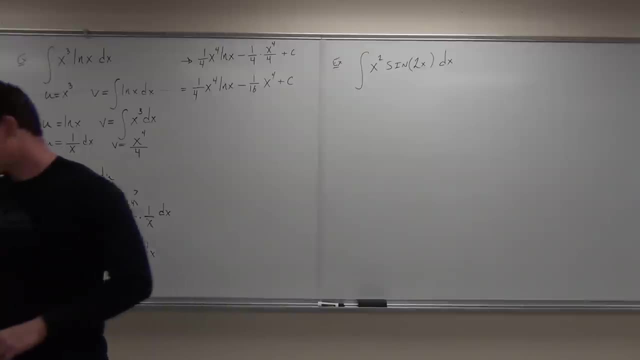 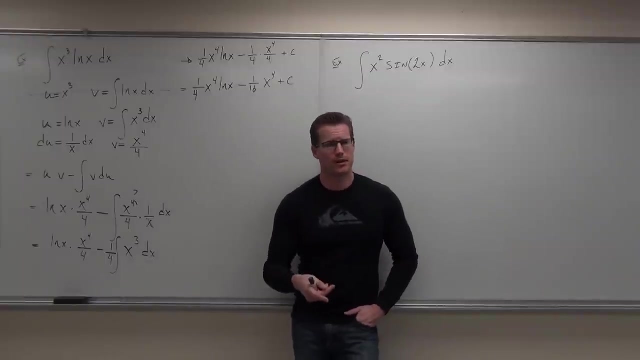 Sine, Sine 2x, Sine 2x. well, 2x, If we pick, Say what now 2x? If we pick sine 2x, as your u, does the derivative get better? No, 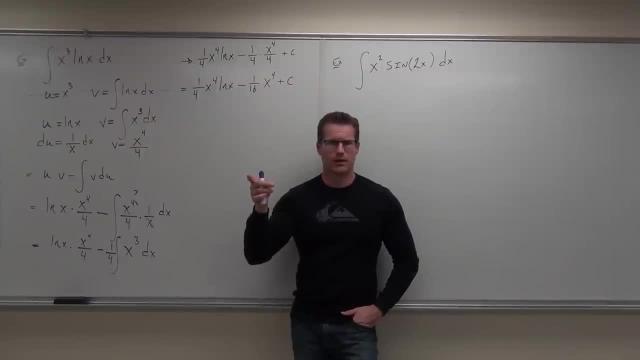 No, No, No. And the integral grows right. Square root of u has to be a third. okay, So in your next process You would have, You'd have a cosine somewhere and you'd have an extra third. Your integral's going to explode a little bit. 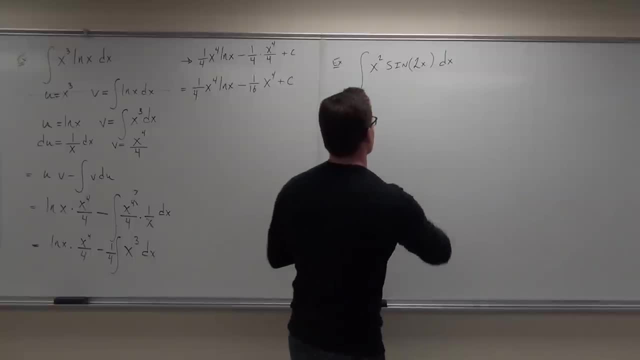 Does that make sense? I'll show you if you want. I think we have time for this. If you did, Don't. Don't write this in the law. I'm going to leave it up here, but You can if you want, I guess. 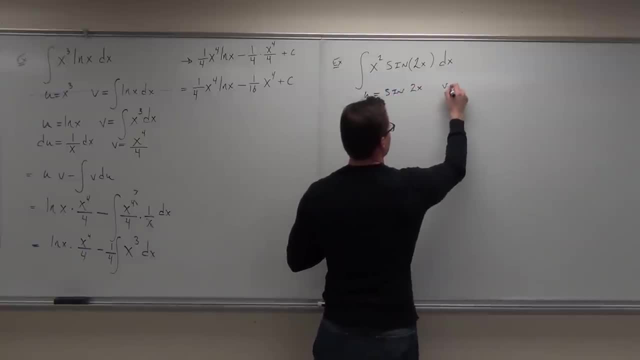 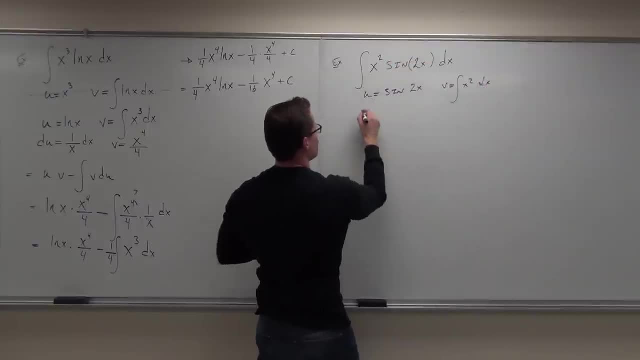 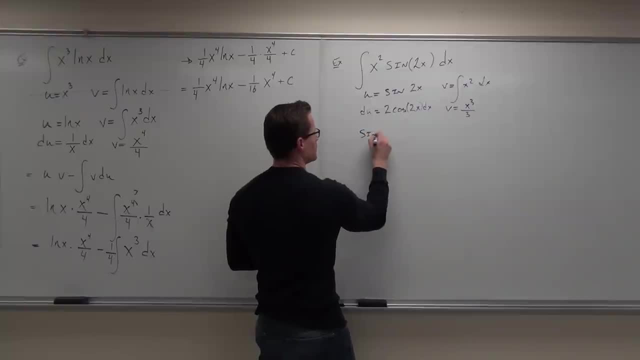 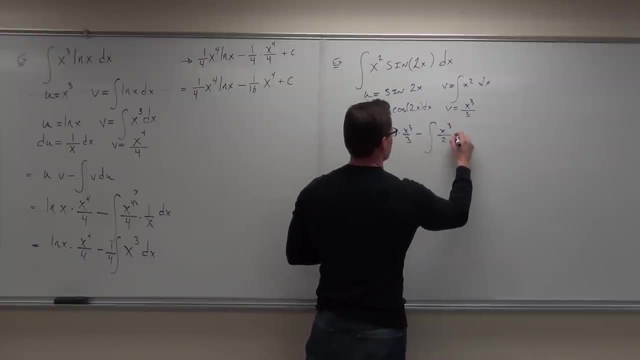 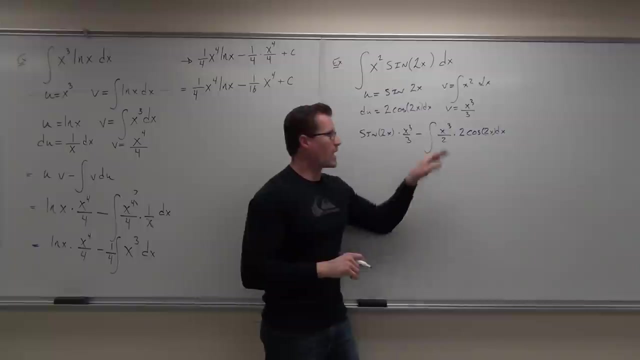 Then I have uv minus integral of v du. This is my du. Do you see what I'm talking about? Right, when you do this, You should give up. Okay, not calculus, all right, but right when I see this, look what happened. look, look it honestly, look. 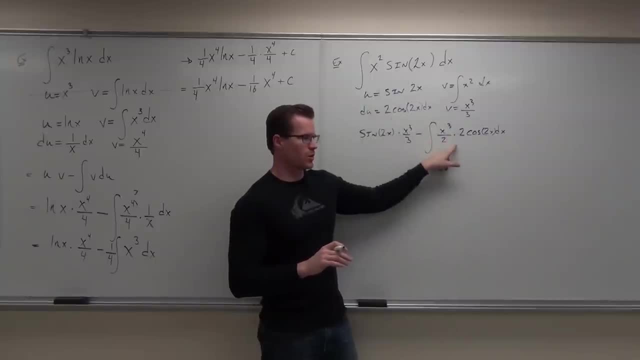 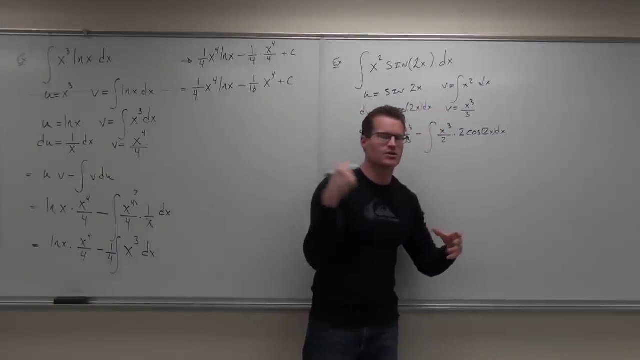 This is basically the same thing, but my power grew. It didn't get smaller, it grew. Is that a good thing? No, Then this is the wrong thing to do, So don't try to manhandle this problem and pound it into submission. 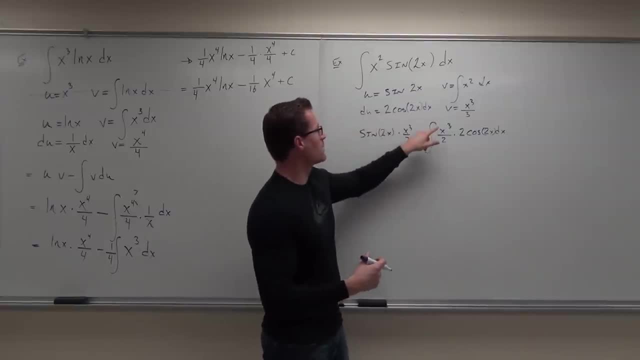 because it's gonna kick your butt. all right, This thing's gonna get worse If you pick this again. well then that's gonna go to a four, And then that's silly. so we don't wanna do that. So this is a bad choice. 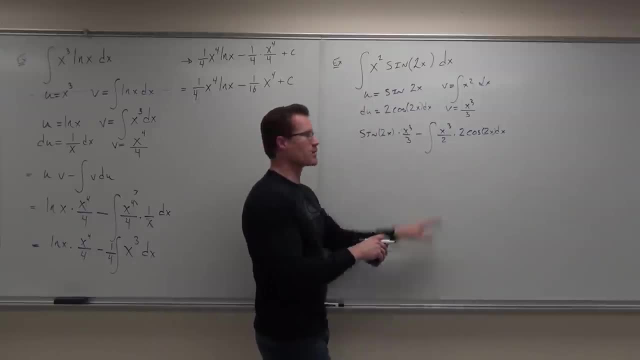 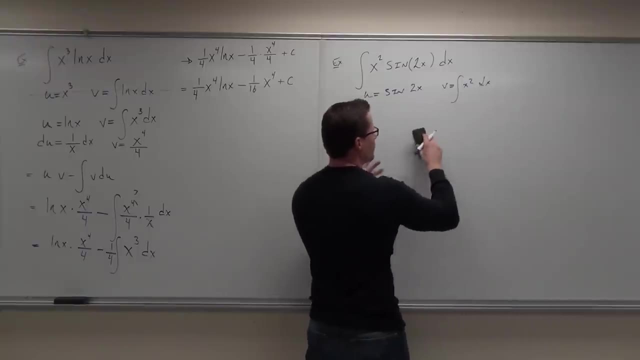 You understand why it's a bad choice. The integral got worse, not better. Even though you could do the integral of this one, this derivative didn't look better. You want both. really, you want the derivative to be better and you wanna be able to do the integral. 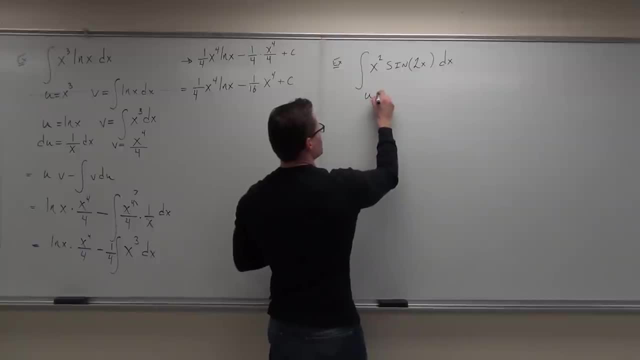 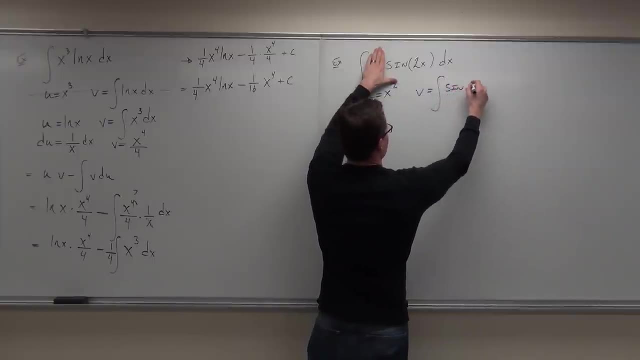 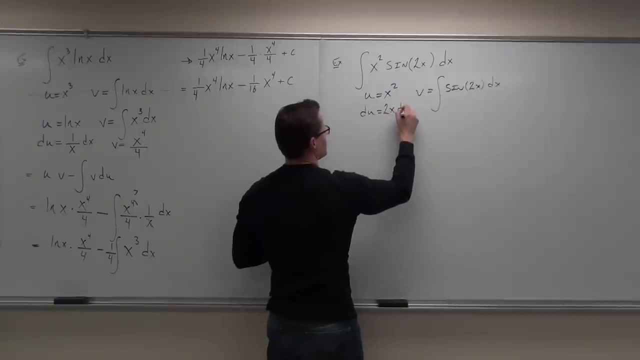 So let's try the other one. Instead of this being u, let's pick that one being u. Then v equals: cover it. integral of the rest. du equals- this is easy. or du equals 2dx, You guys, okay with the. du equals 2dx. 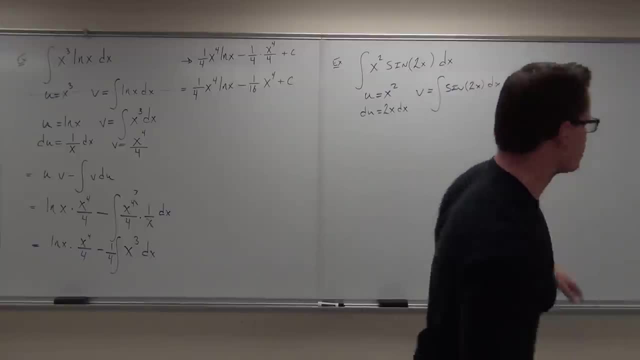 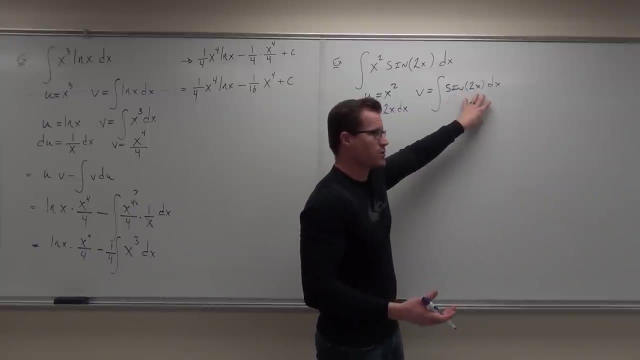 Yeah, Now listen, you should be able to do this other thing, this other integral. Can you do this integral? Yeah, You might have a u substitution in there. So if you do a simple u sub, I wouldn't pick u. 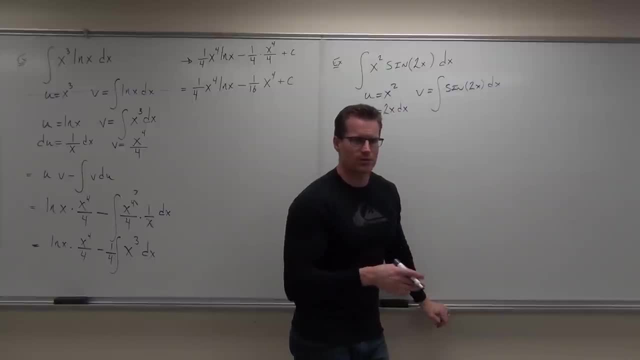 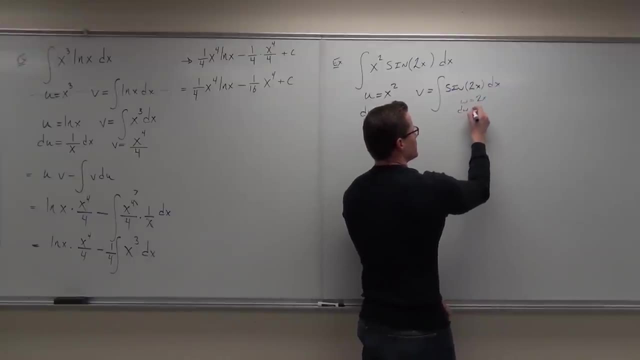 because you already have a u. I'd pick, like a w or whatever you want, anything that you want besides x, v and u right now. So if you picked a w, substitution equals 2dx. dw equals 2dx. dw over 2 equals dx. 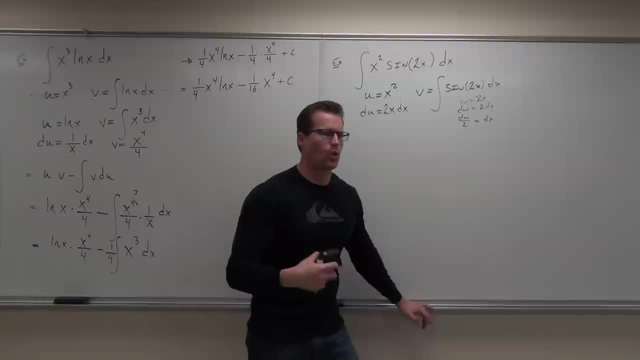 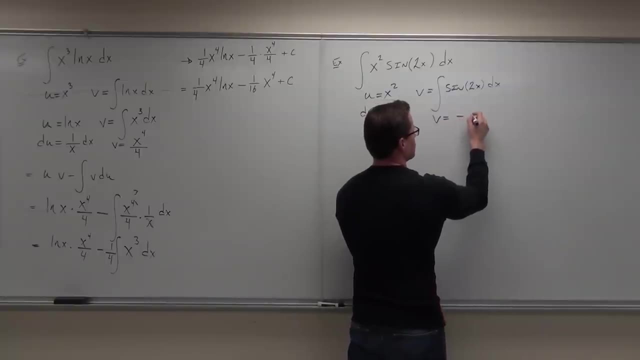 And then do your substitution. What you're gonna end up with after you do this- a whole lot- is you're gonna understand that, really, what this v's gonna be is negative cosine 2x over 2 is what that's going to be. 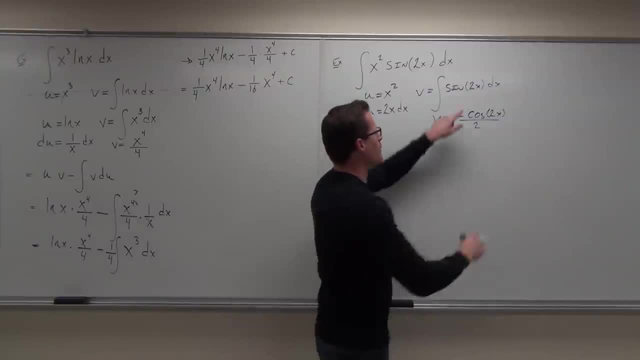 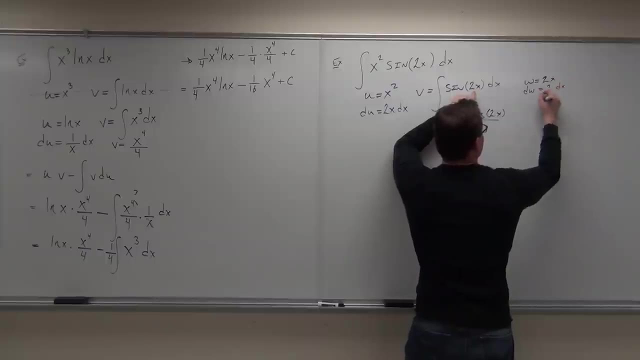 Do you guys see where the over 2's coming from? Yes, Where's the over 2's coming from When you have your u? well, w equals 2x dw, equals 2dx dw. oh, look at that, over 2.. 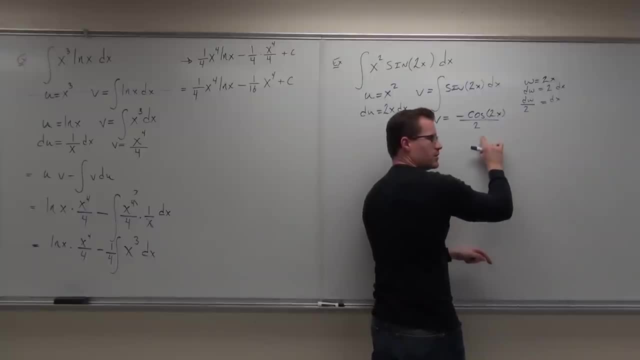 That's where the over 2 is coming from. No, Yes, You didn't blow your minds. Did you follow that? Yes, Do I need to do the whole thing for you? No, No, Okay, No, All right. 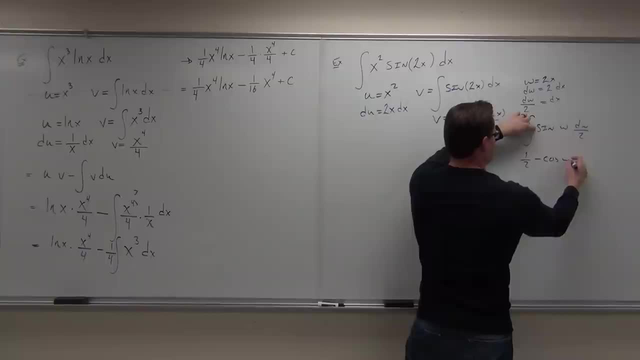 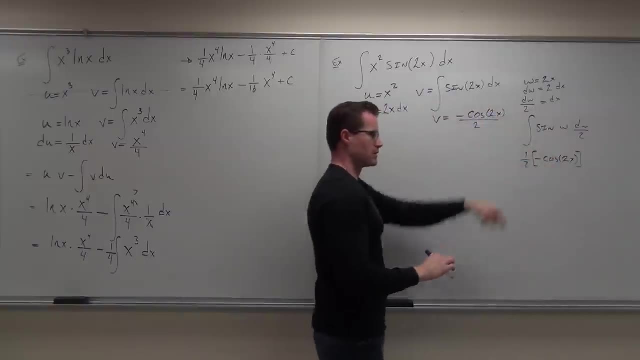 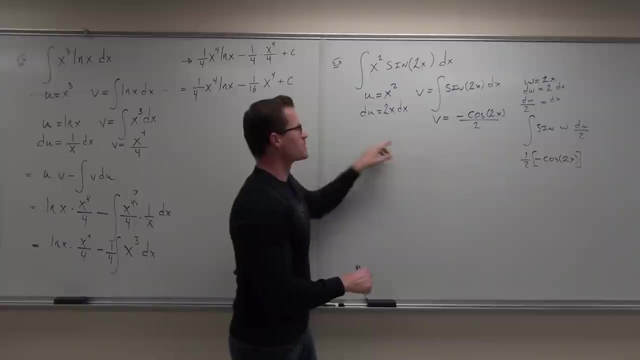 One half Negative cosine, w. ah, w is 2x. That's that. That's all there. Okay, now we don't need it. So we've done our u, we've done our v. Let's put this thing together in the formula: 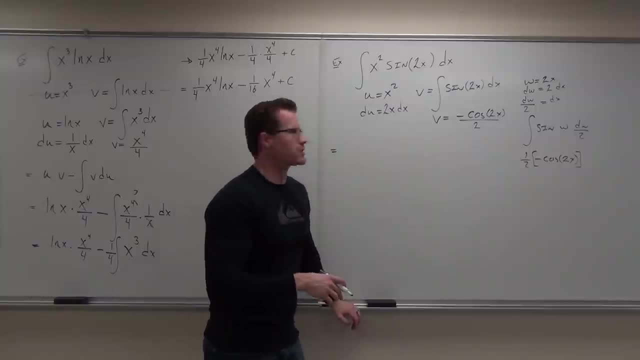 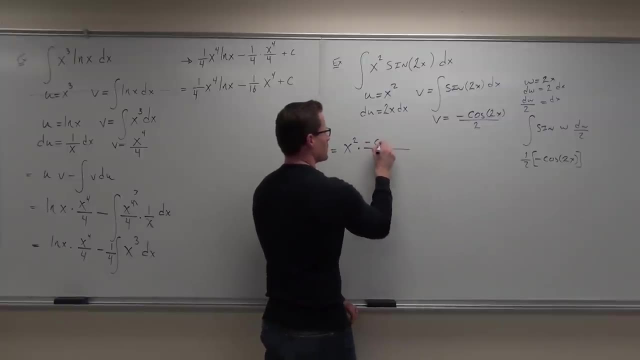 The formula should look. you tell me what's the first thing I should write here: X squared, X squared Good. X squared times Times. Negative cosine V. Negative cosine 2x over 2. 2x. 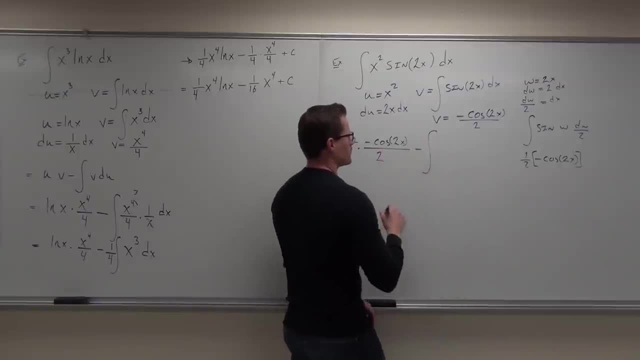 Minus the n-th, Minus the n-th, Minus the n-th. Oh V Negative cosine 2x over 2.. Times, 2x, Times, what? 2xdx, 2xdx, 2xdx. 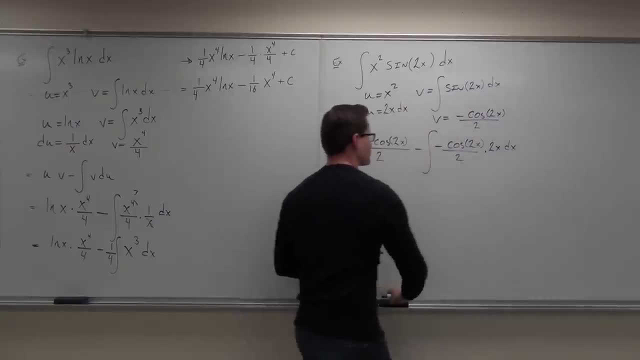 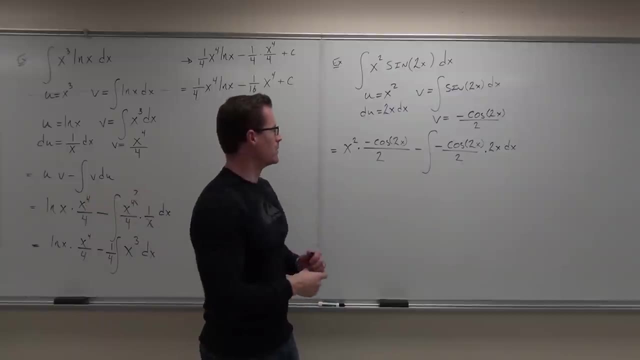 I'm gonna erase this. Yeah, should I be okay with that one so far. Yes, Yes, You guys in the middle. Oh yeah, Let's clean it up before we go any further. That's nasty, all right, All right. 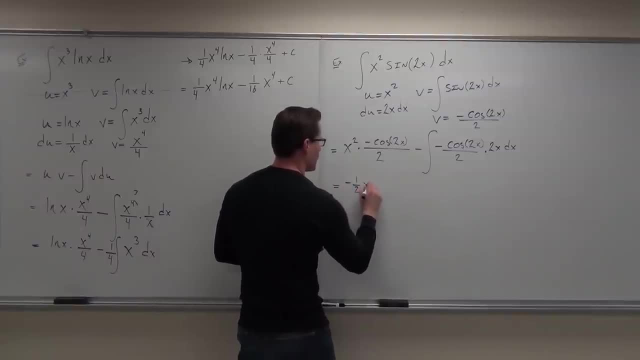 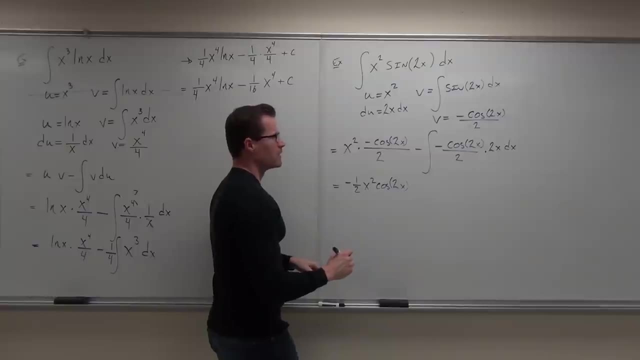 Let's make this negative: 1 half x squared cosine 2x. Negative: 1 half x squared cosine 2x. Let's do a couple things here. Let's pull out this negative and make that a plus. Let's pull out this 2 and simplify it with this 2.. 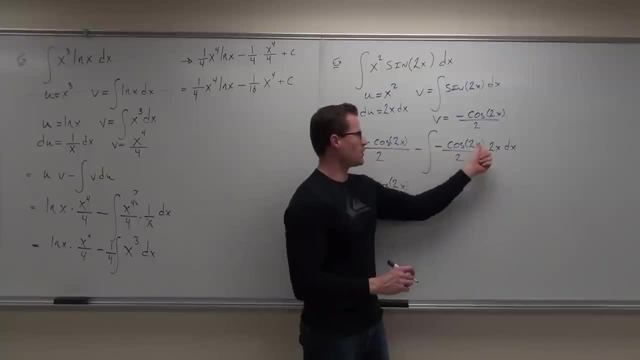 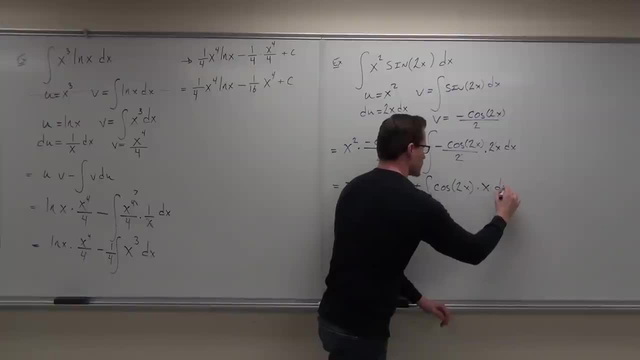 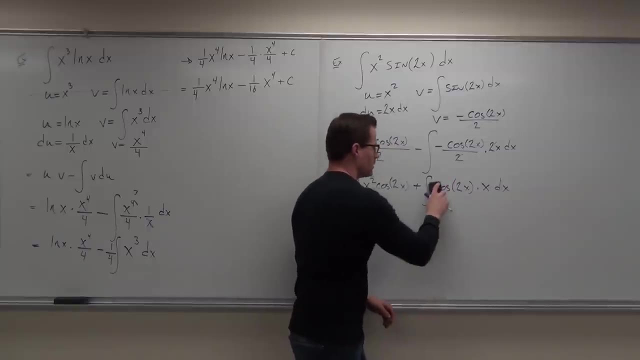 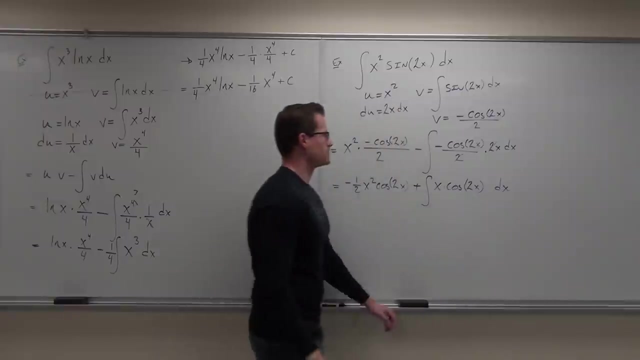 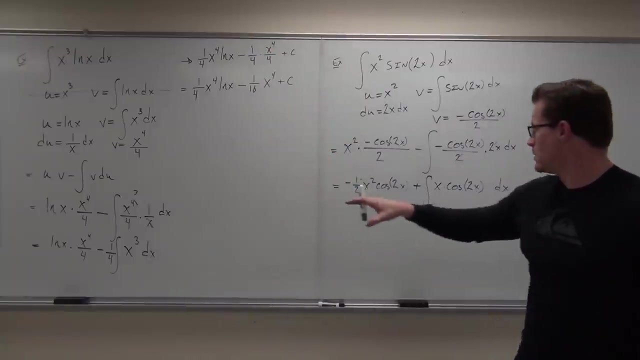 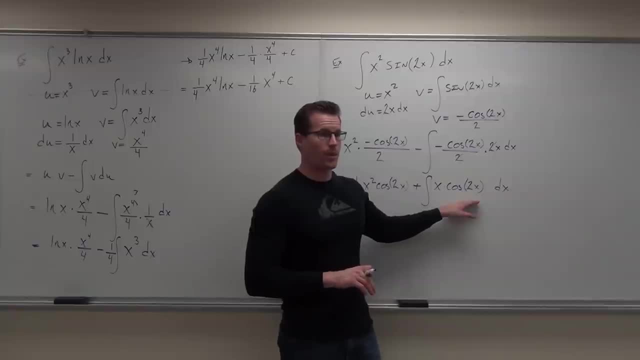 Yeah, you can. Is it an integration table? No, Hmm, No. Is a substitution going to work? Yeah, Yes, Okay, What's the derivative of 2x, Two, Two? So you need another part? I mean x. 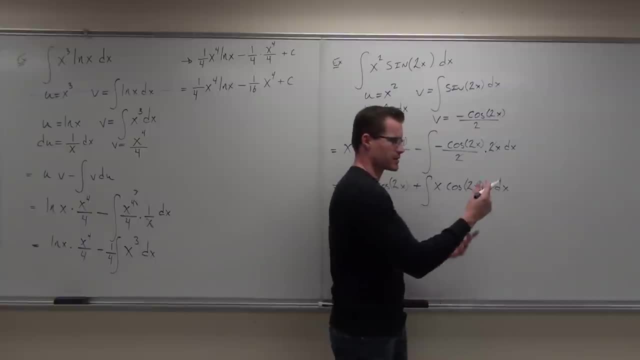 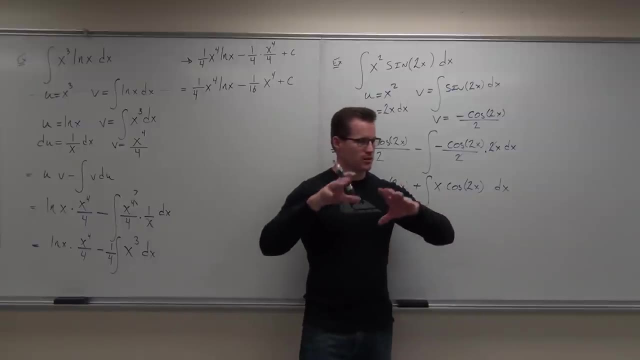 You need an x, right? Would this work? Yes, if it's a square, Is a substitution going to work here? No, No, Another part, Oh my God. Well, okay, So we did. Is it in the table? 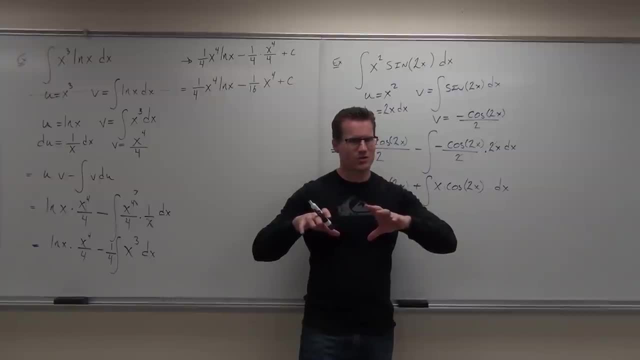 No, No. Will a substitution work? No, What's your next choice Parts? No, You can do it again. I didn't do that. Now, don't screw this up. Pick the same thing for you that you did here. 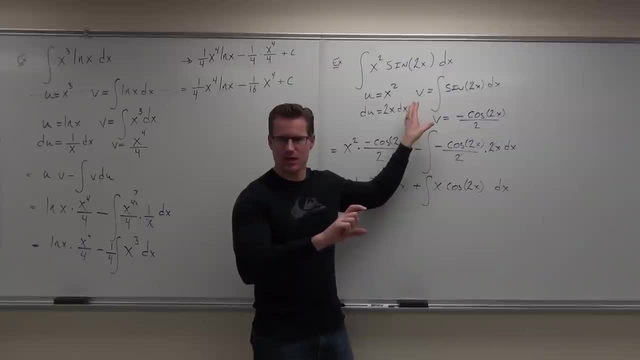 The same thing. It should be reduced by a power. Do you see that? Yeah, This is basically the same, except it's an x squared again of x. That's how you know you've done it right. Okay, This should at least go down a power. 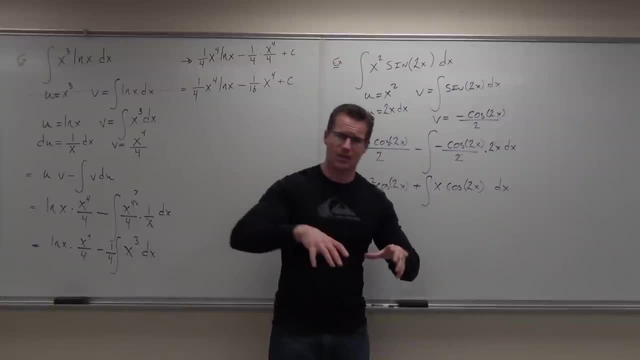 If it goes up a power, you picked the wrong choice. If it goes down a power, you picked the wrong choice. If it goes down a power, you picked the right choice. You just got to do it again. So let's do it again. 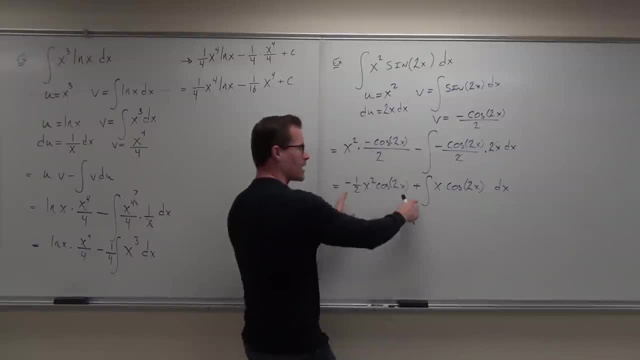 Lots of practice. So we're going to hang on to this. okay, We're going to look just right here. What's the? We've got to move quickly. What's the appropriate? u X. Check this out When that's x. see how, when we take a derivative. 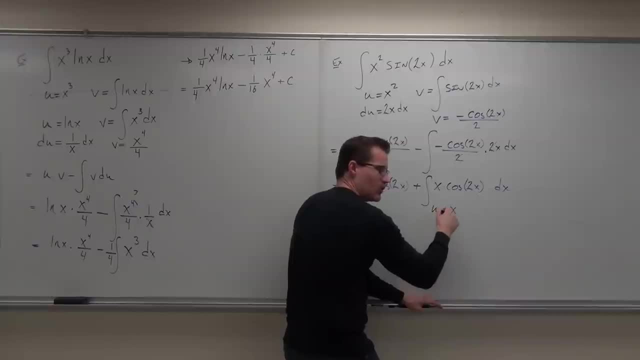 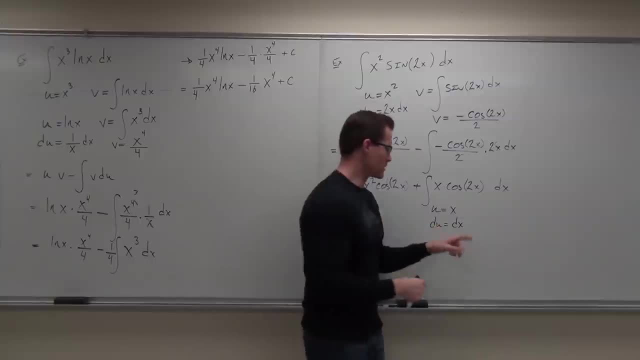 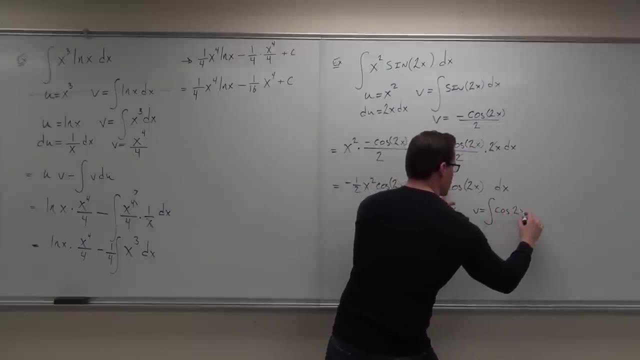 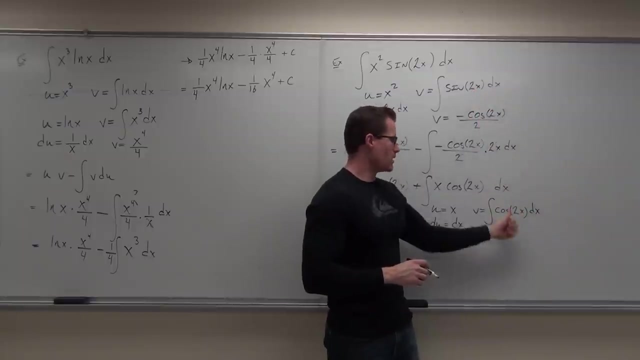 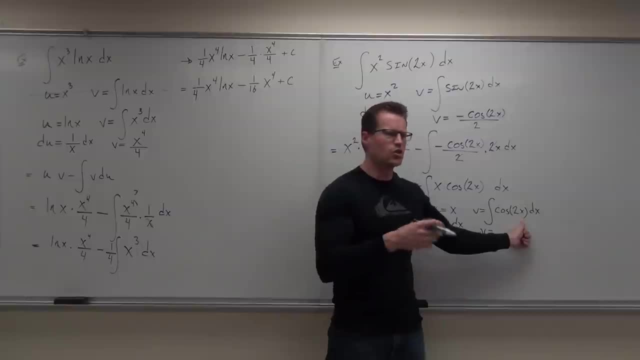 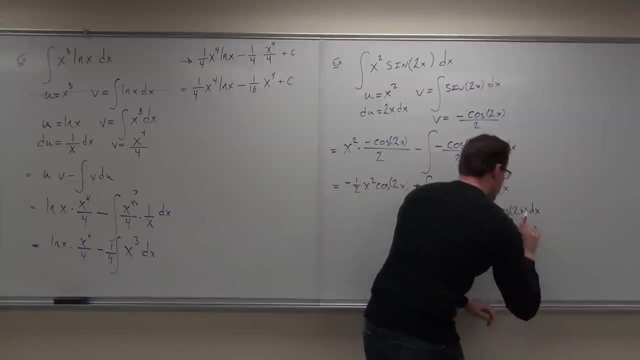 Do you see that you're going to have another substitution here. U or w or whatever, is going to be 2x. That means dw is going to be 1, half dx. That means we're going to get an over 2.. So this would be sine of 2x over 2.. 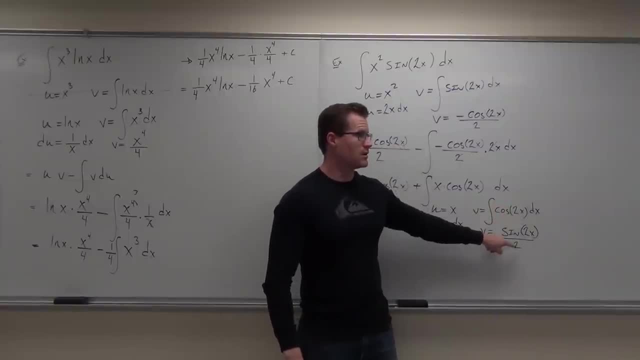 Can you verify that for me? Yes, Sine 2x with an over 2 by the Substitution Substitution. Okay, So I would not write this again right now. I'm just going to hang onto it, I'm just going to focus right here. 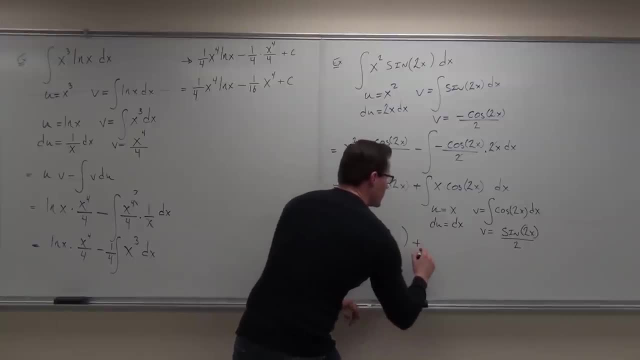 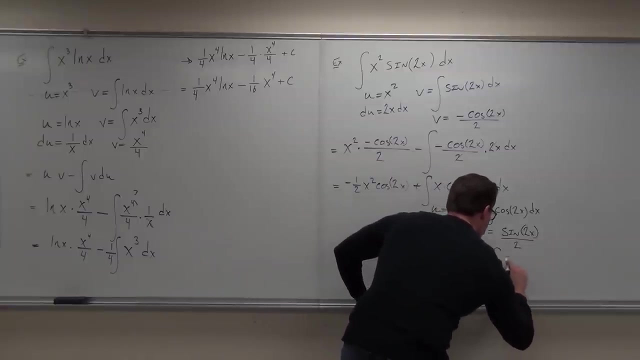 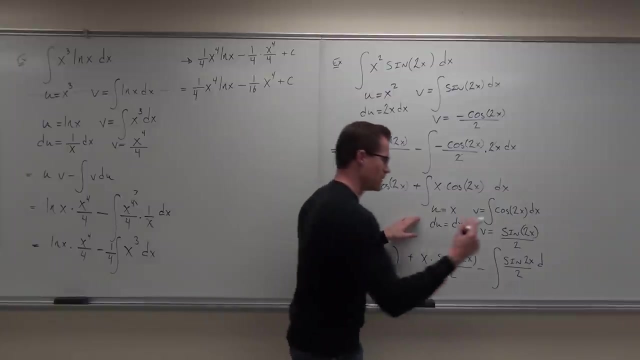 So I'm going to have a plus big old stuff. plus Well, we're going to have u times v, U times v Right, U times v Right, minus the integral of v du. Now, what's our du in this case? 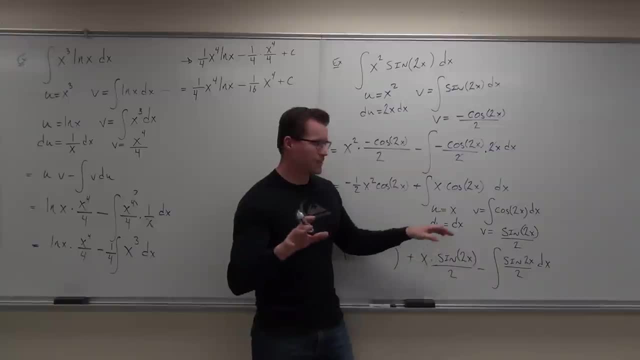 That's nice. That means that we're not gonna have any extra work to do. I want you to see if you're okay with this one. I know I'm going about a minute or two over, but this is kind of important for us. 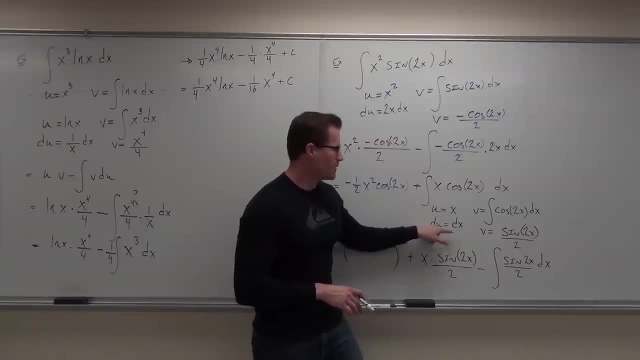 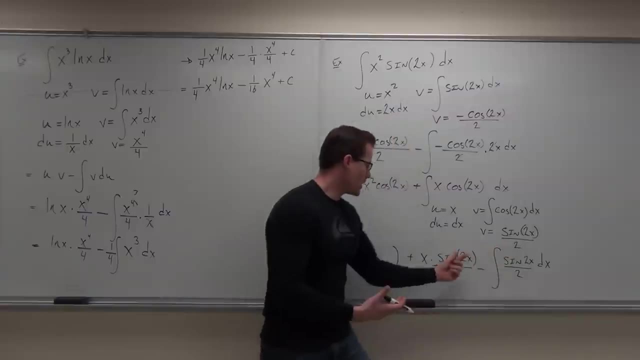 You okay with the u, Du, it's dx. now You okay with the v? V's the integral of the rest, Pretty easy integral. You need to be able to take these integrals, otherwise you'll make the wrong choice. Now we got u times v minus the integral of v. 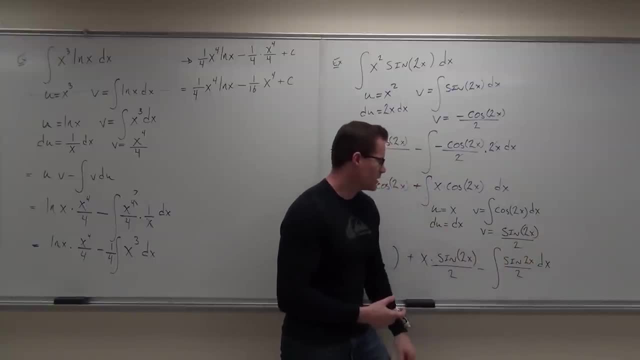 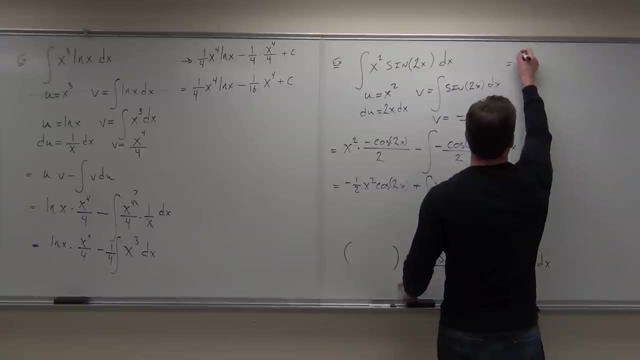 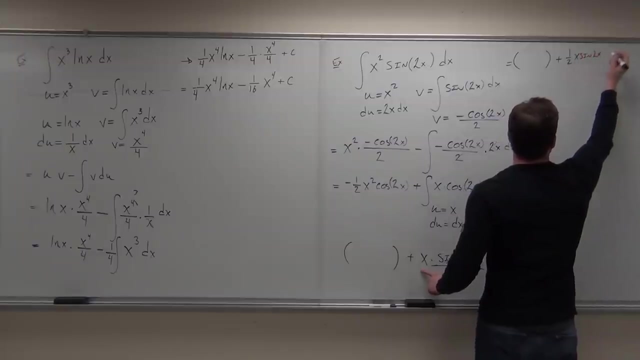 and then du, Du is dx. Make that substitution again. Tell me something we're gonna do with this One half. Okay, so if we do that we get some stuff plus one half x sine two x minus the integral. Oh yeah, 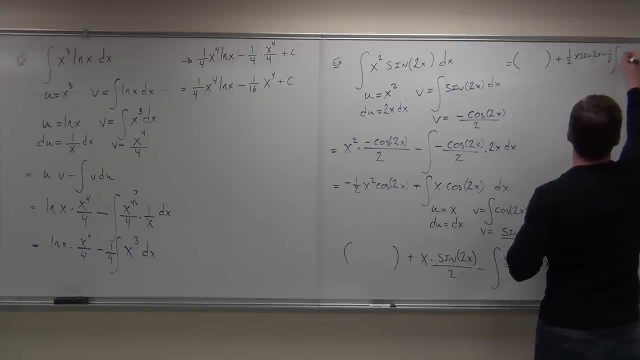 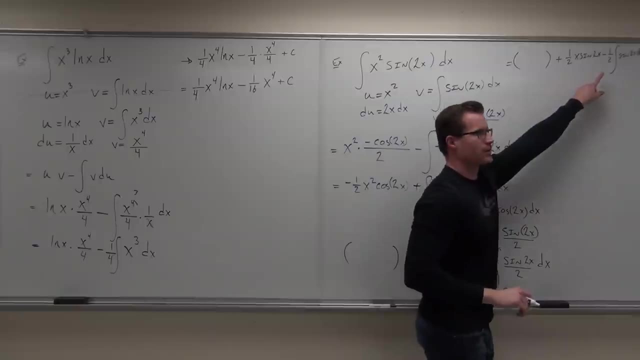 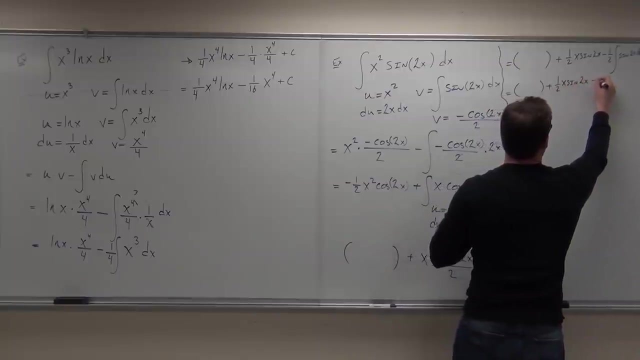 One half integral sine two x, dx Only. we've already basically done that one. Look at this: This integral is that integral? So just look back at your table. We've already done it. So we have all the same stuff Minus one half. 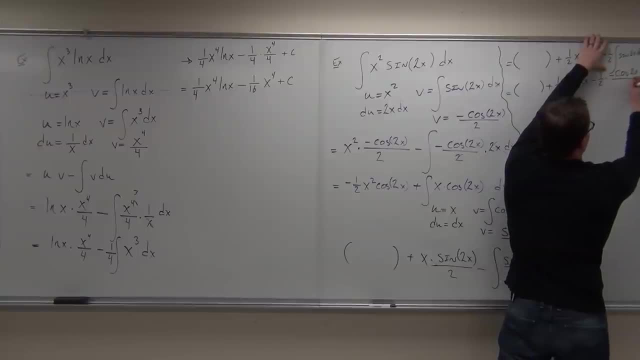 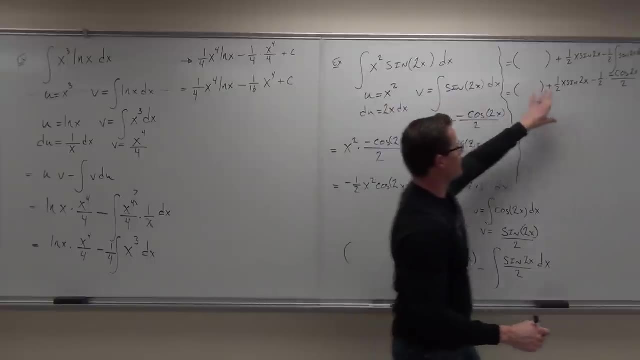 N was negative cosine two x over two, Exactly what we have here. This integral is the same as this one, So negative cosine two x over two. So we can just be okay with that one. Now, we're just gonna clean it up. 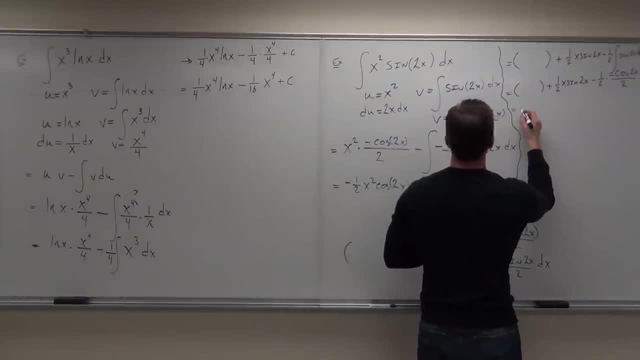 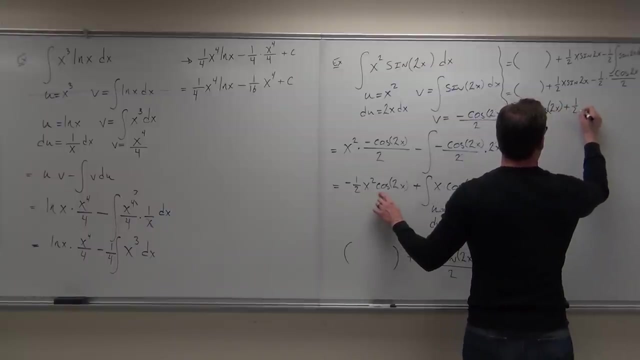 Okay, just cleaning this thing up. We've got all that nasty stuff. was negative: one half x squared cosine two x Plus one half x sine two x. What happens here? Two's cancel out. Two's do not cancel out here. Oh sorry. 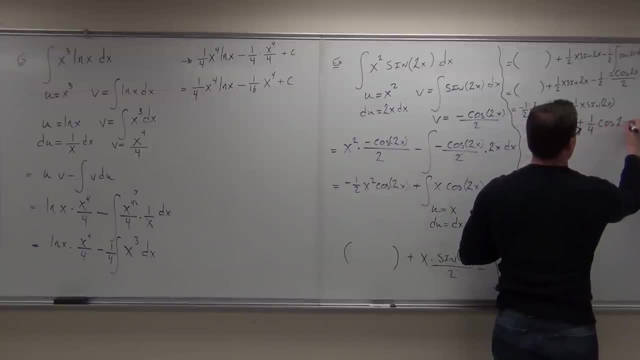 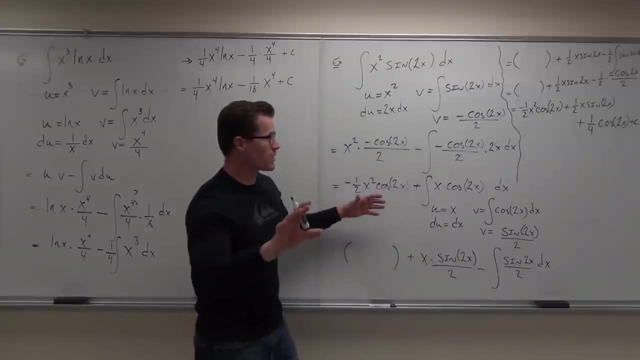 Plus one, fourth cosine, two x And last one. Okay, I wanna make sure you're clear before I let you go. This is the first little part. It's right there, Do you guys? okay on that one? Yeah, This is the first integration by parts. 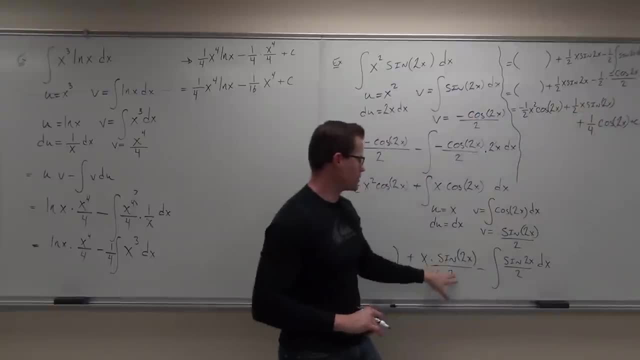 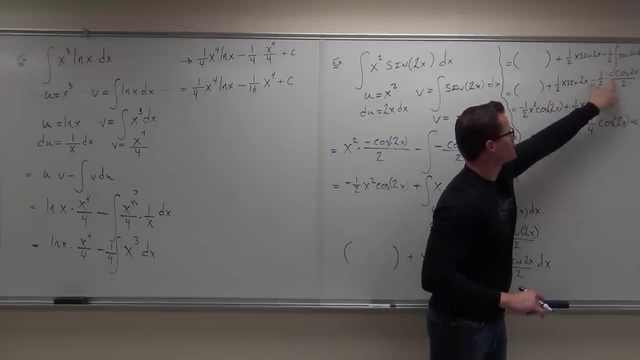 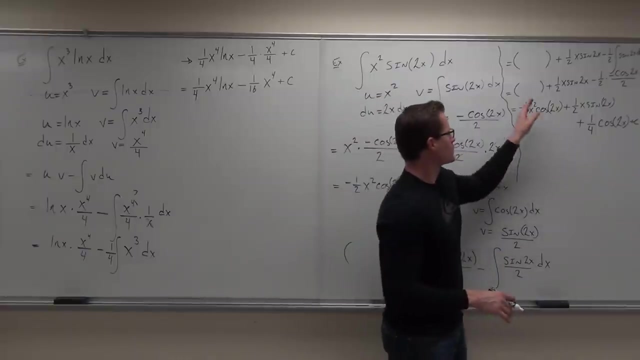 This was the first part of our second integration by parts. The? u times v. This little piece, this plus, comes from when we do our last, integral Minus and negative becomes a plus one. fourth cosine: two x plus c. Oh my gosh, look what happens to the powers. 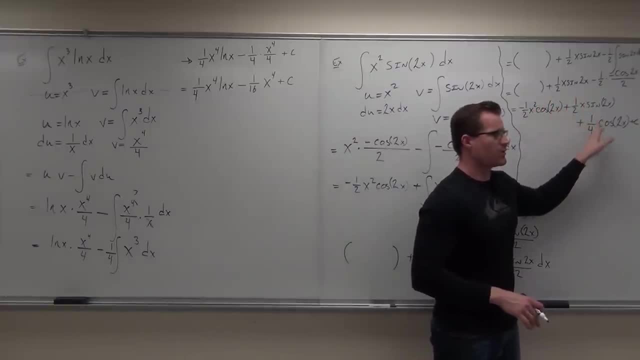 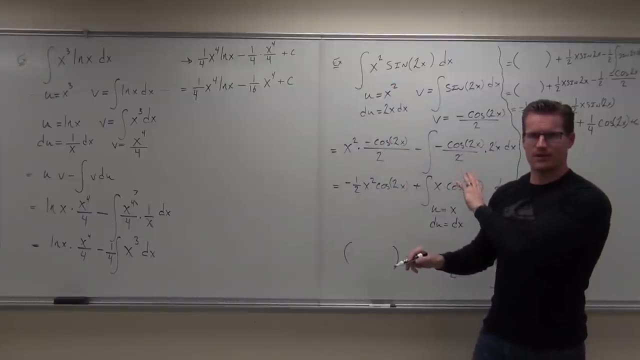 Square to the first power. No x at all. That happens a lot when you have this. If you add x to the third power, you'd have to do that one more time. If you add x to the fourth power, you'd have to do it one more time. 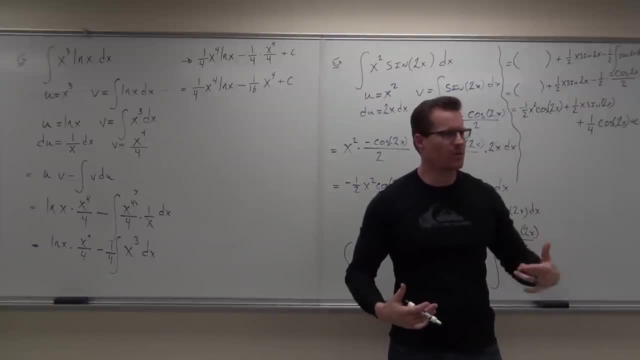 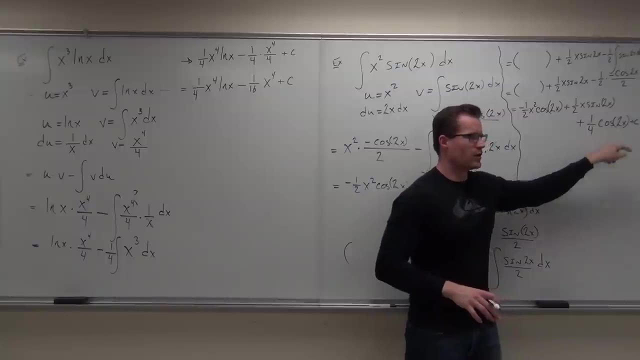 Ultimately, we're gonna find a reduction formula for that. We're gonna create our own formula for this. What I wanna know is if that actually made. I know this is kind of sloppy, I didn't have room over here, but do you understand that this is the plus one? fourth, 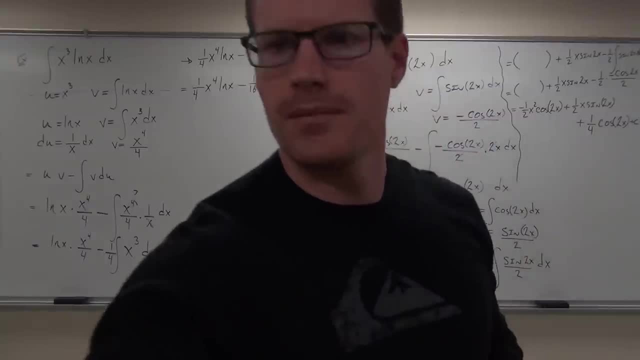 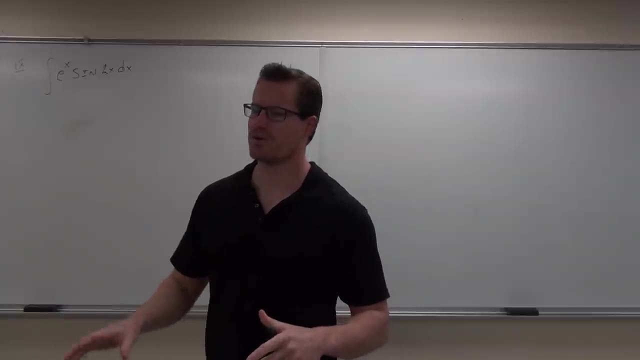 Yeah, Show of hands. if this made sense to you, Good, All right. so for our day today, we're gonna practice more integration by parts. So if you don't remember from last time, though, we've got a weekend in between this. 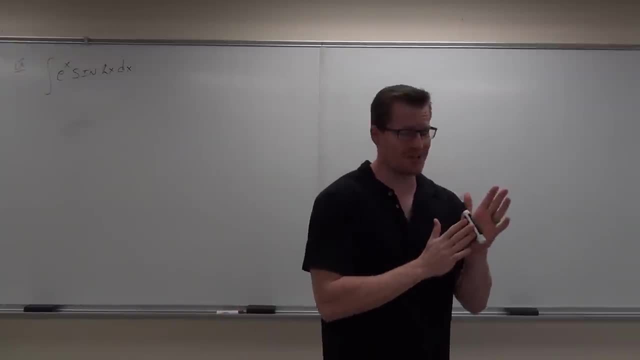 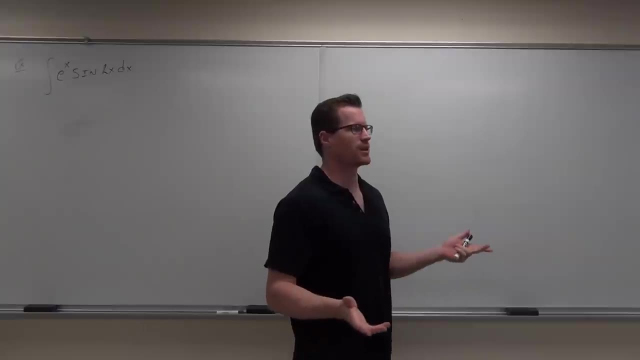 Except for people watching online, they have like five seconds in between this. So for us, though, what we're talking about is integration by parts, And the way we do integrals is. first thing we check for is: do we have something that's in the integration table? 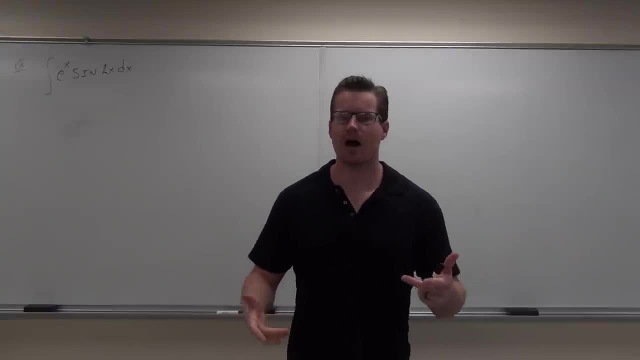 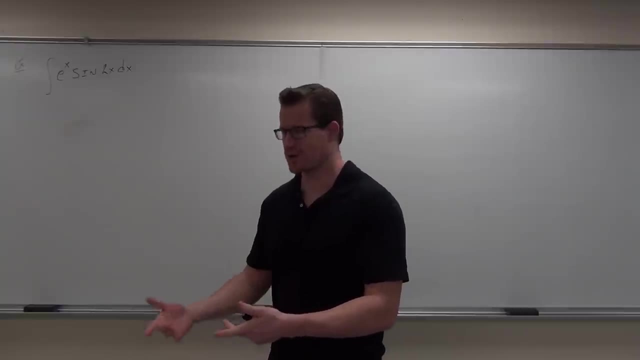 If we do, it's really easy. It's in the table. If it's not, then we try a substitution. Once we try a substitution, well, hopefully we can do one. If we can't, we can do it because it's easier. 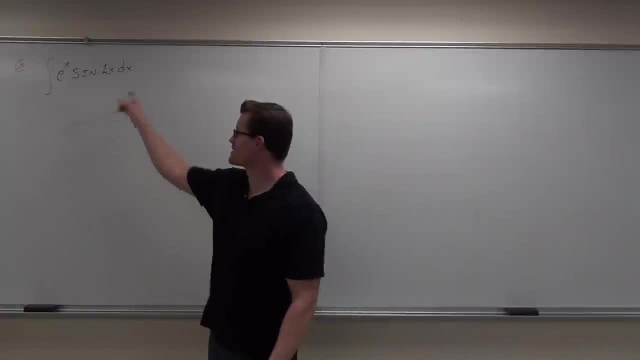 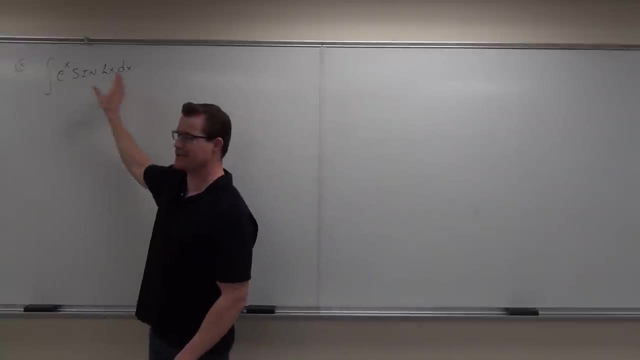 If we can't, then we have now integration by parts. So we check this. Is this in an integration table for us? No, Of course not. Will a substitution work? No, No, if I substitute this part, there's no other e to the x in there. 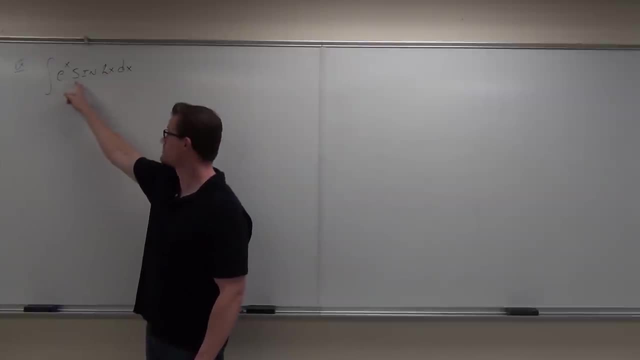 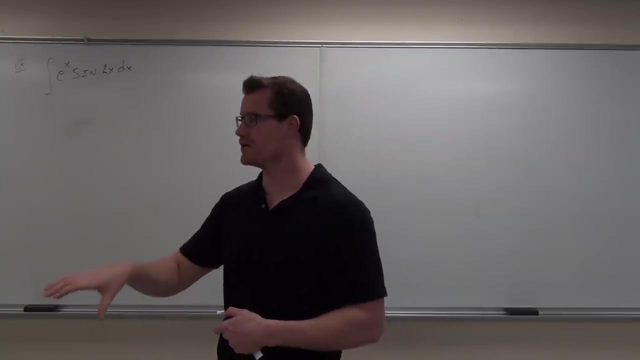 If I substitute this, well, there's no, it's not gonna take care of the e to the x. If I do sine, there's no cosine up there. Remember, with substitutions, the derivative of your u has to be somewhere in your integral. 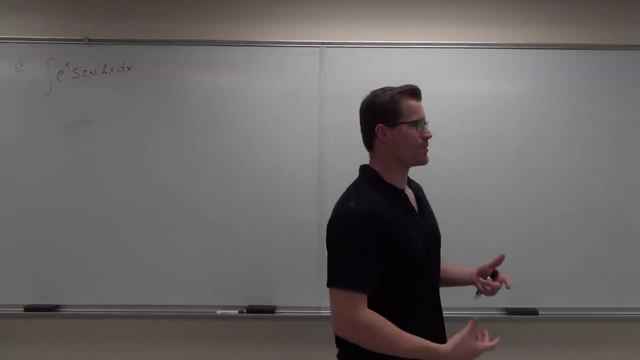 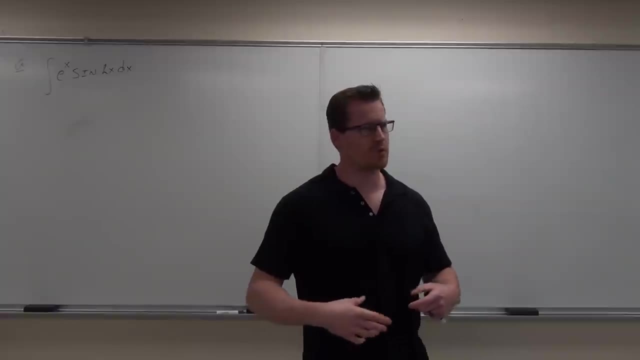 That doesn't happen here, So what we're left with is an integration by parts. Now, these last four examples that we're gonna do today. they are like the more difficult concepts, the more difficult ideas, the ones that are like: wow, I didn't know you could actually do that. 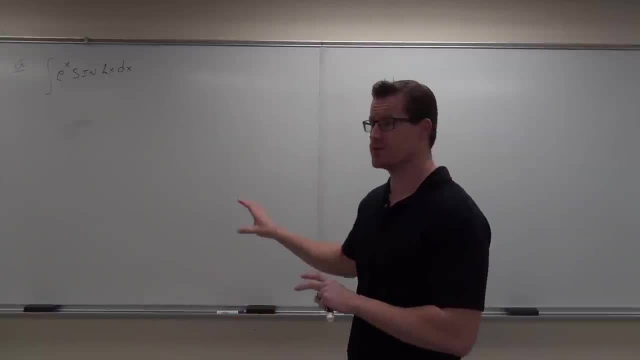 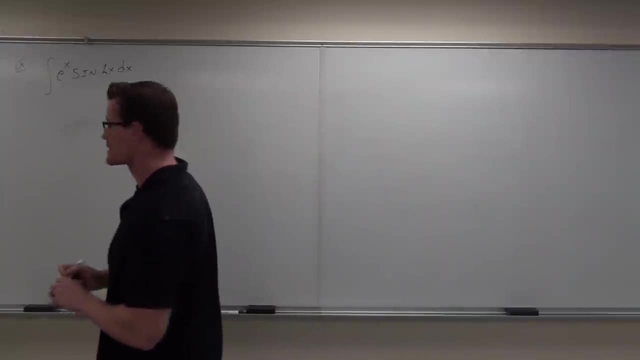 with this stuff. I'm gonna show you some cool, interesting things that you can do with integration by parts. Are you ready for it? Yeah, So here's what I'm gonna do. I'm gonna pick u to be sine x, sine two x. 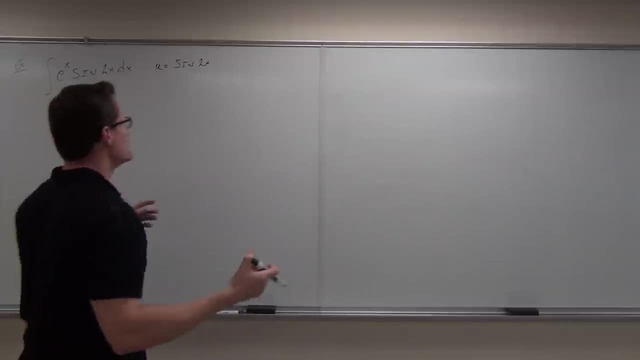 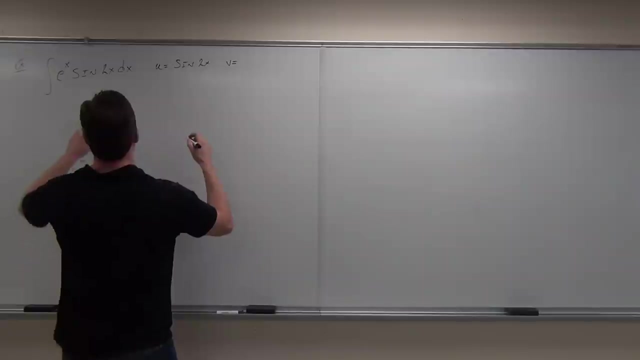 Now, as soon as you pick u what's v, So I pick u. we've gotta be able to be pretty good about finding out what v is. What's v. Everything Very good, everything else. So you just cover this up with your hand, right? 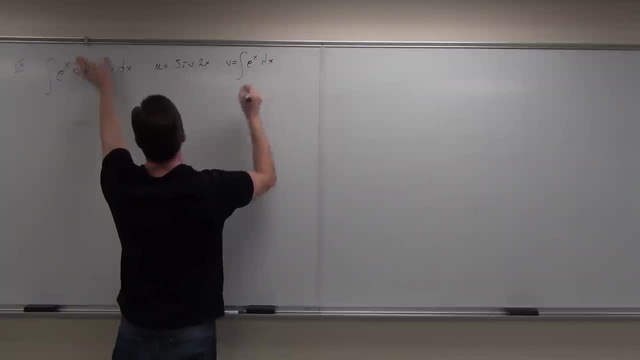 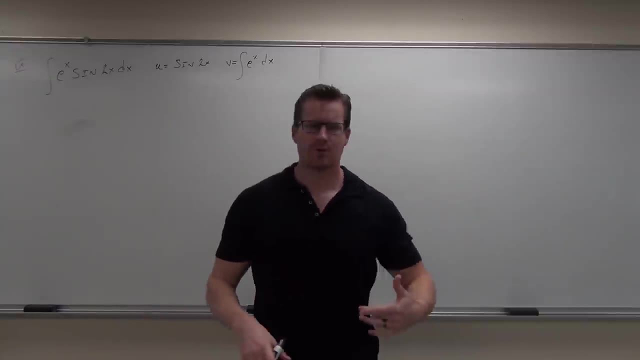 Exactly what's left over, In this case, integral of e to the x, dx. Quick head nod if you're okay with that one. So this is coming back to you, I hope right Now the way that we pick u is typically u becomes easier. 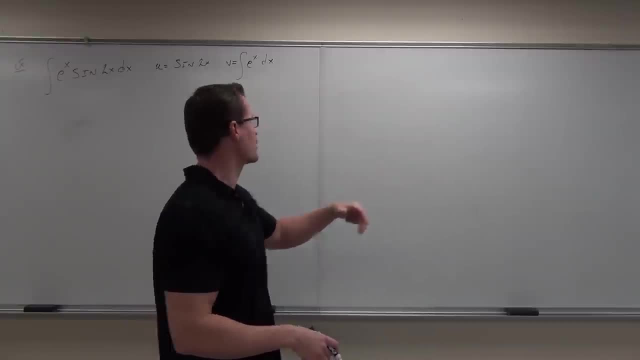 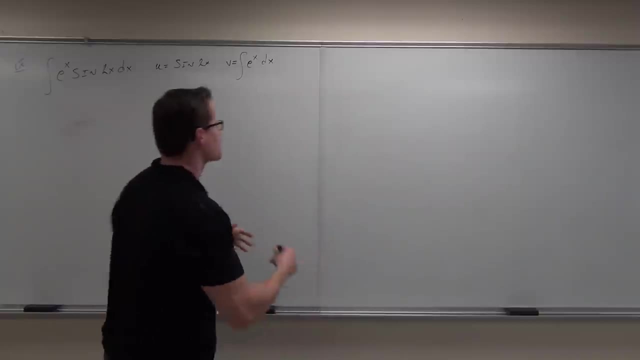 and you can do the integral of the v. Well, in our case, this integral should be really easy, isn't it? This one doesn't get any better, but you're gonna see something really unique that happens on these types of problems, where we get when you think about it. 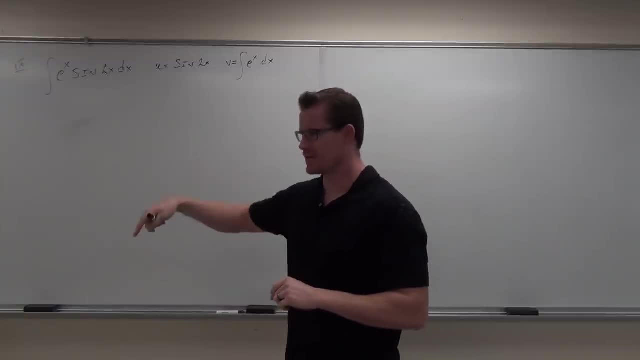 we're gonna get repetitiveness here, aren't we? The integral of e to the x is e to the x. The integral or the derivative of sine x is cosine x and the derivative of that one is sine x. We're gonna get things back again, no matter what we choose. 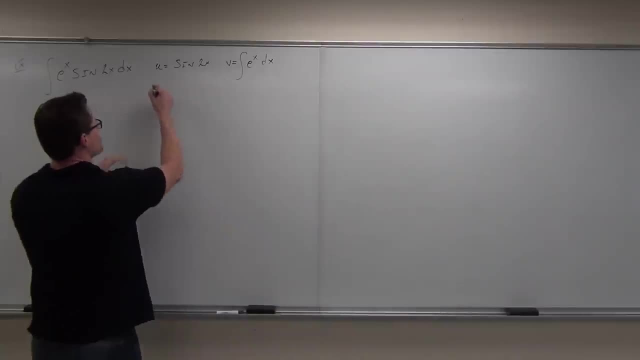 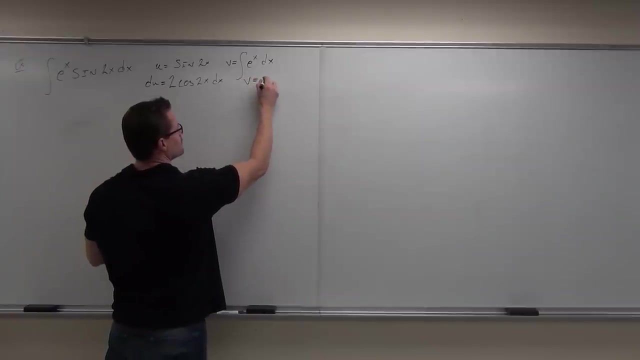 Does that make sense to you? So watch what can happen here. If we do this, then du equals two cosine, two x, dx. Can you please explain to me where this two comes from? V, Hey, And v equals e to the x. 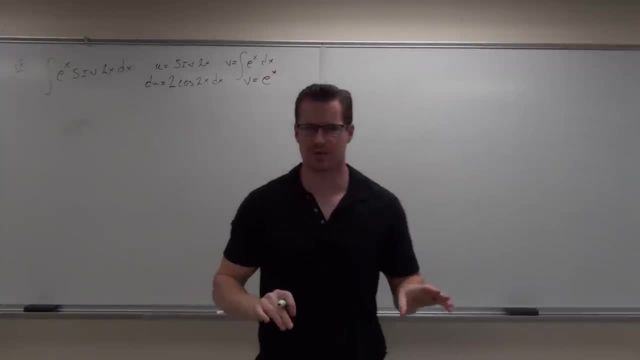 Do I need a plus c right now? No, No, we're gonna wait to the very end to put a plus c. Quick head nod if you're okay with that one. Quick head nod if you're okay with that one. Now, what we do with our integration by parts. 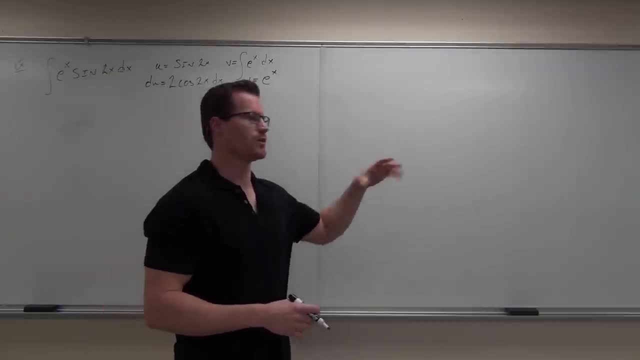 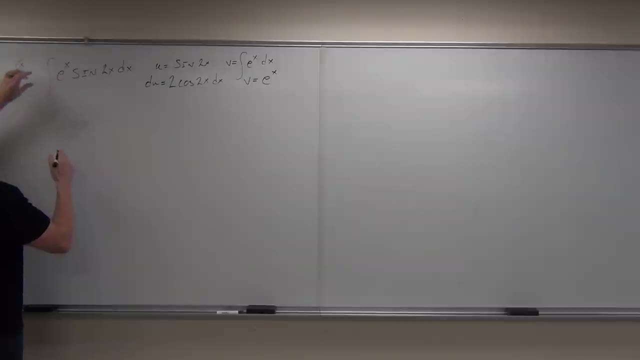 is: we pick our u, we do a derivative, we pick our v, we do the integral of whatever's left over. The v is the rest. Then we do integral of v. du equals u times v. so in our case our integral is going to equal u. 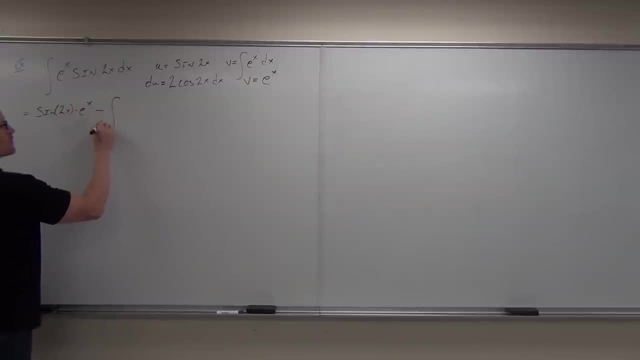 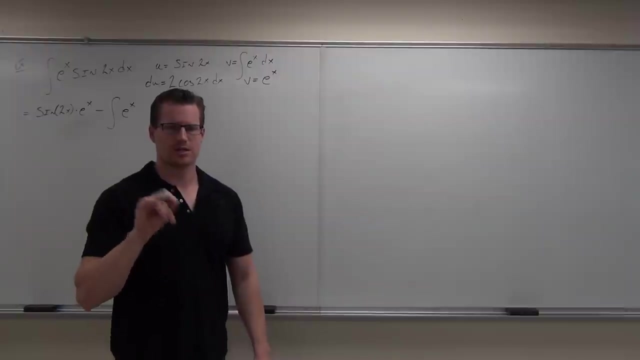 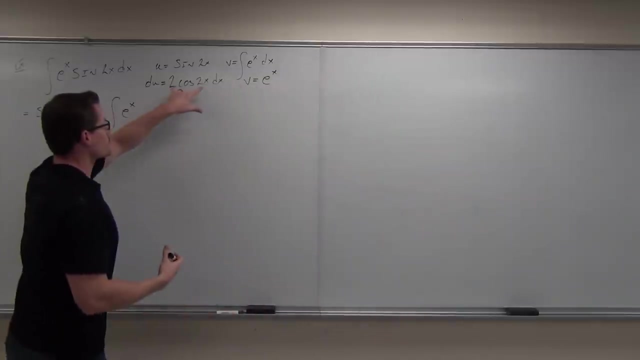 times v minus the integral of v, minus the integral of v, minus the integral of v- Now this is what's interesting- Minus the integral of v. but then we gotta have du. How much is our du in this case? So we need this whole thing right here. 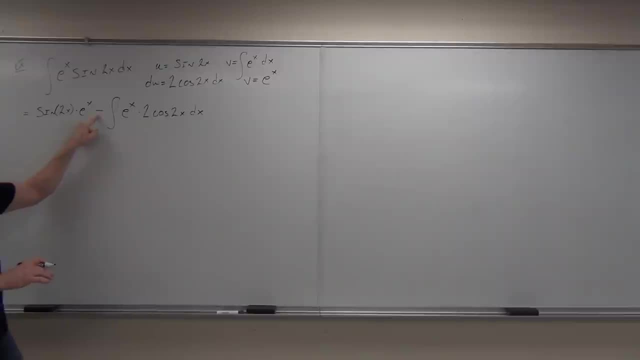 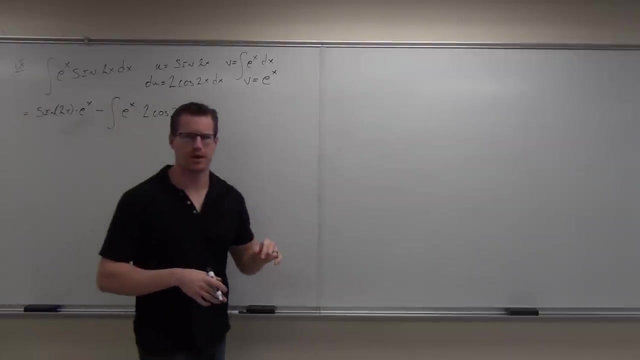 Okay, so let's make sure you guys got it. U times v. u times v minus. okay. integral of v. integral of v: du U. is this whole piece Quick head nod. if you're okay with that one, Now check it. 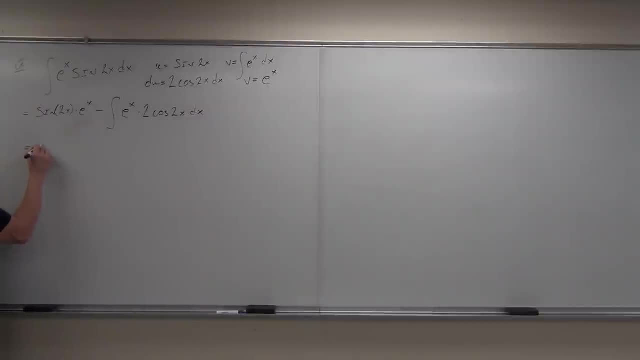 We did this last time. We saw something similar to this last time. I'm gonna move my e to the x- to the front, by the way, So e to the x sine two x. The last example that we did, by the way. what else can I do here? 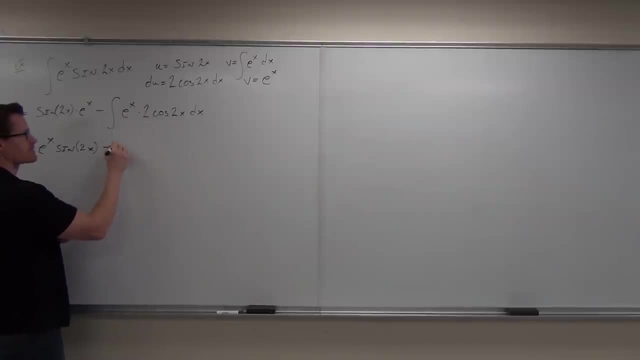 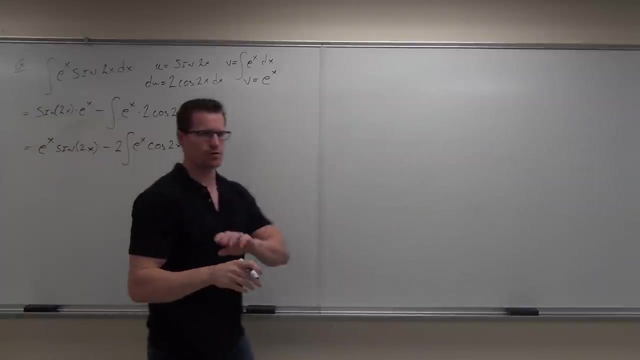 Two out. Yeah, we're gonna take that two out because it is a constant being multiplied: E to the x cosine, two x dx. If you think back, if you watch back on the video for the last example that we did, 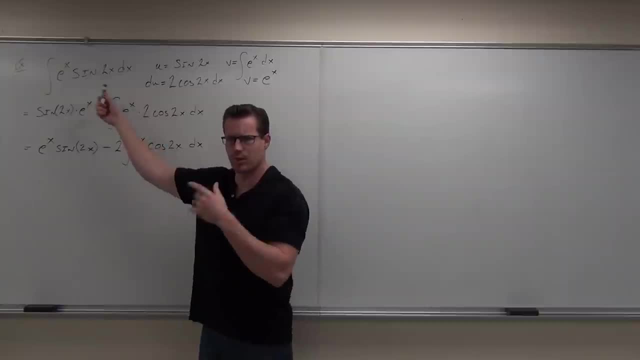 do you remember the last one that we did? We had something kind of similar to this one. We worked it down, except instead of sine two x and e to the x, it was like an x squared, remember that. And we had to do integration by parts twice. 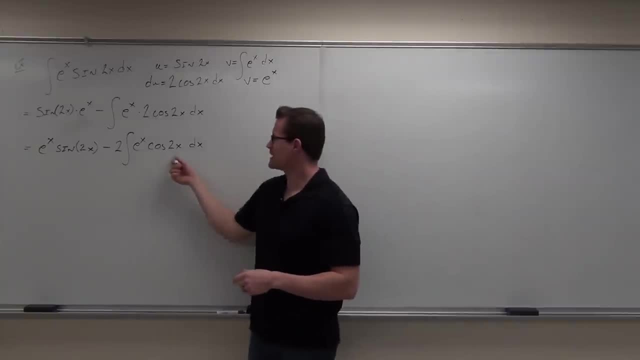 Do you recall that example? Well, look at this one. Doesn't that look almost exactly the same as that, Except if it says sine, we're gonna have cosine. Could we do integration by parts again? Yeah, Let's do it again. 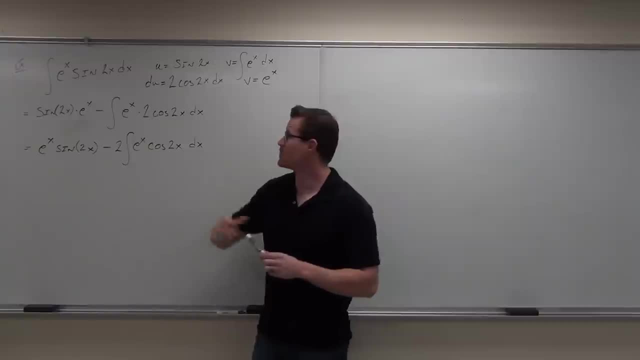 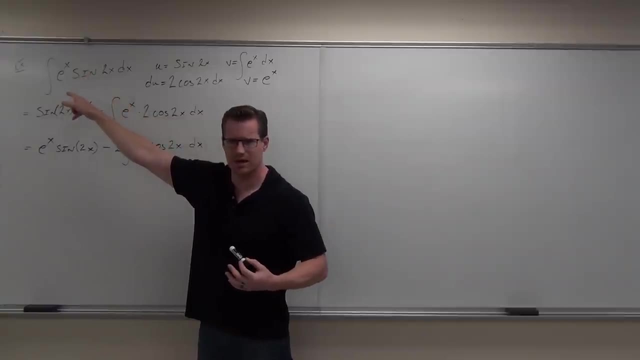 Now, if you're thinking, wait, a minute, wait, If I do integration by parts here and it gets this plus something that looks almost exactly the same as that, why are we doing that And aren't I gonna get something like this? 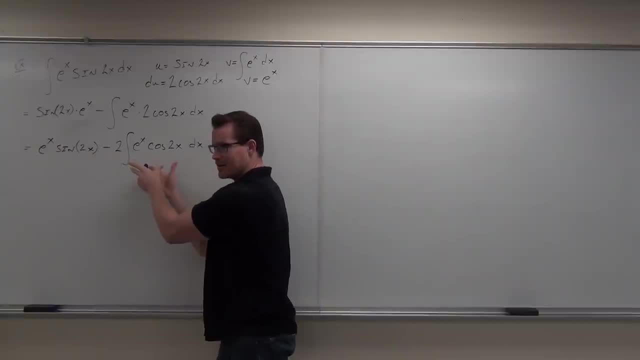 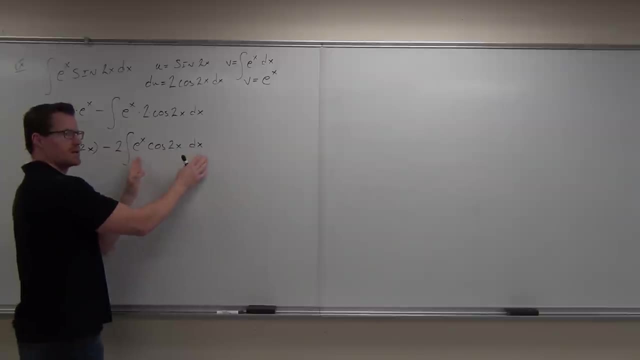 but something that looks just like this again. Yeah, but that's the whole point, and I wanna show you why. So we're gonna leave this thing alone and we're gonna look right here. Here's the whole thing. If you pick u equals sine of two x. 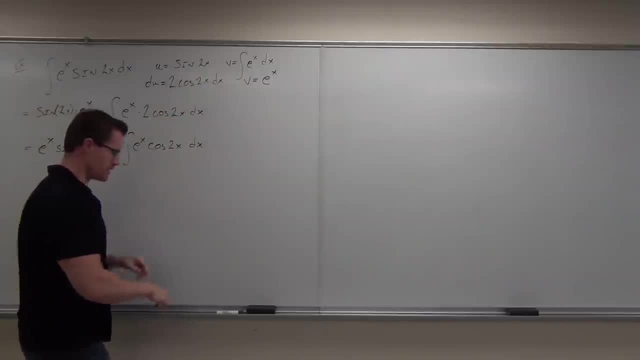 what are you gonna pick for u here? Pick the same thing. So now u equals cosine two x. I'm sorry, not the exact same thing, but pick the same part that you picked. So if you picked sine of two x for this one, 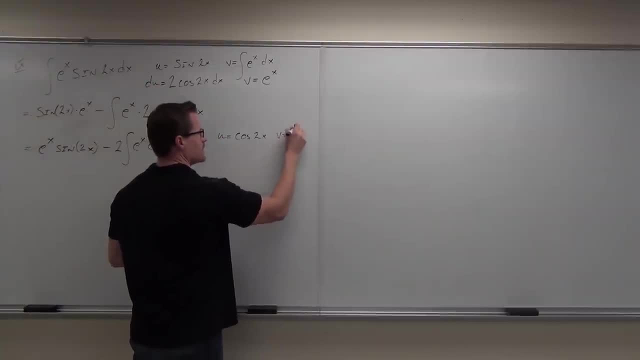 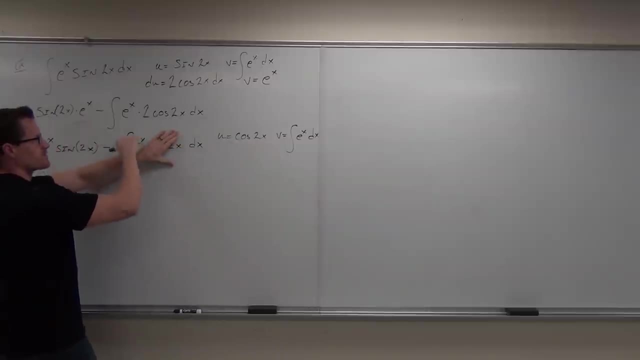 pick cosine of two x for this one. V again is the integral of e to the x dx. That's pretty easy. So u cosine two x, no problem. V is just the integral of the rest. Help me out with the du. 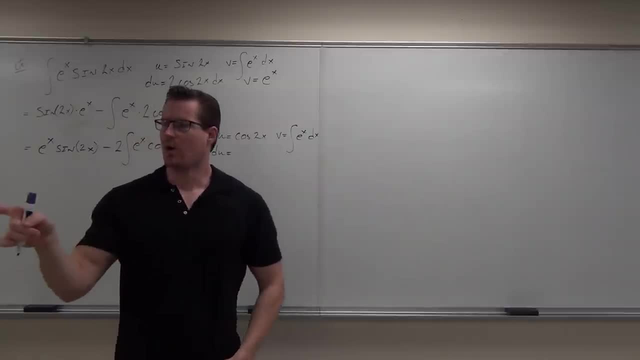 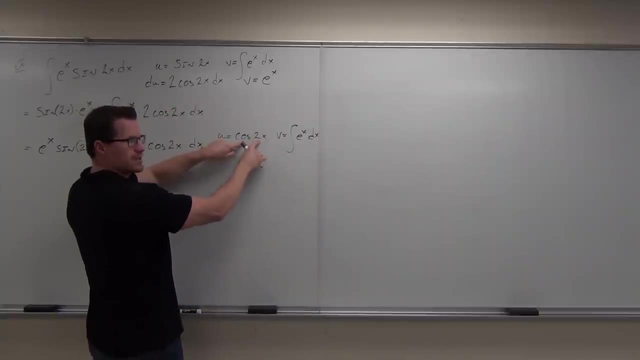 What's the du going to be Negative two sine, Because the derivative of cosine is negative. Good, negative sine. So this is gonna give us a negative sine. The chain rule is gonna give us a two, so we're gonna have negative two sine two x. 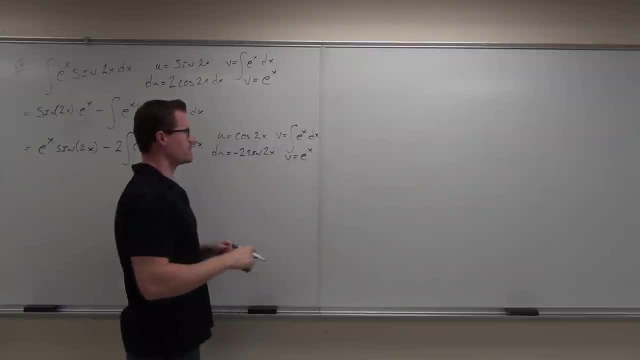 and v is going to equal. well, that's pretty easy. The integral of e to the x is e to the x. Show of hands, if you're okay with that one. so far, Good deal. Now we're gonna wrap this thing up. 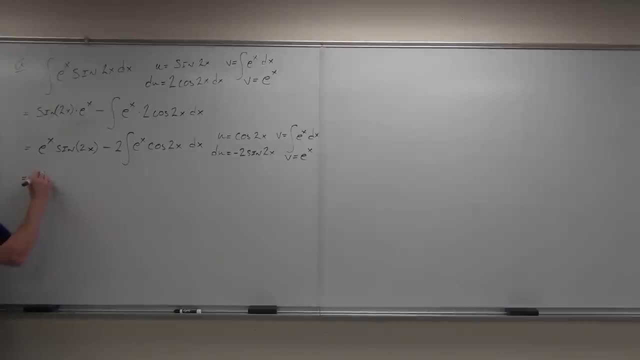 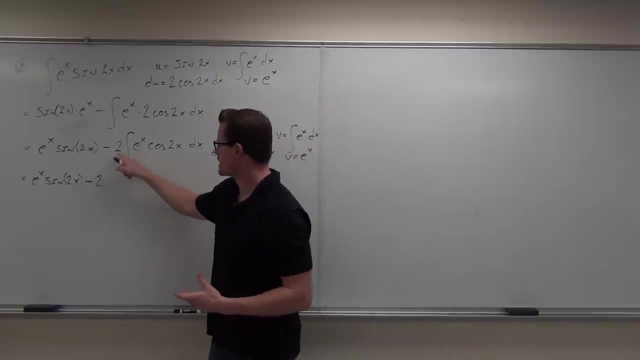 So here we go. We got e to the x. We got sine two x. We got minus two, We got minus two. You guys, okay with that so far. Now, please watch carefully When you're doing this integral. this is minus two times this whole thing, isn't it? 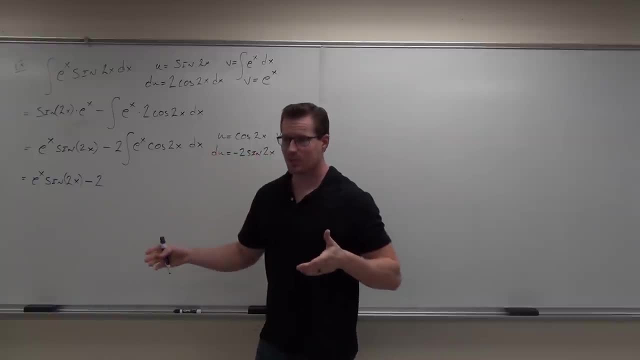 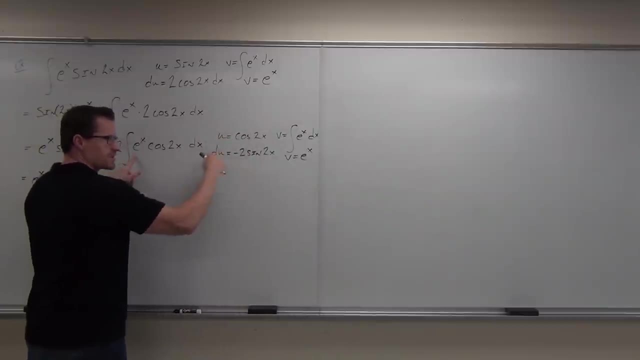 Yeah. So if we just start writing out stuff willy-nilly, we're probably gonna make some sign errors here. So what we're gonna do is: hey, if this integral is gonna be u times v minus integral of v to u. 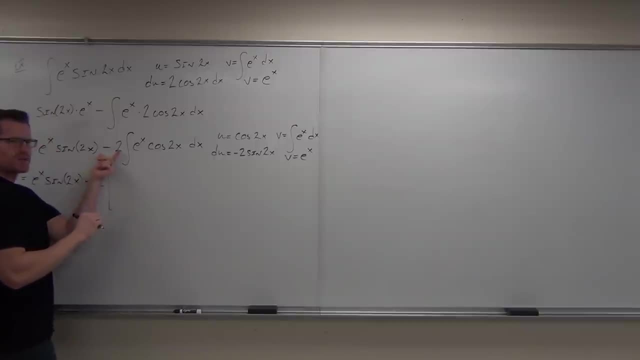 put a bracket here, because what's gonna happen is we're gonna be distributing that negative two throughout this problem. Does that make sense? Yeah, Okay, So minus two, no problem. Now our integral. What are we gonna write first? 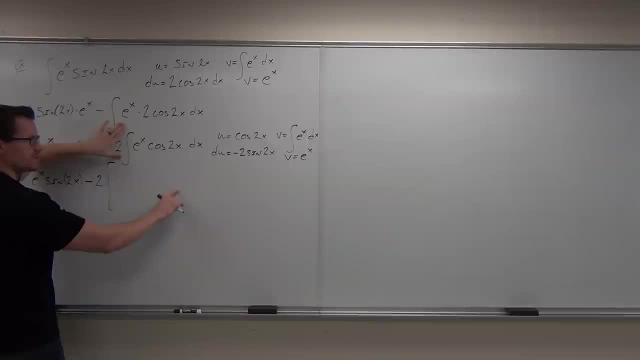 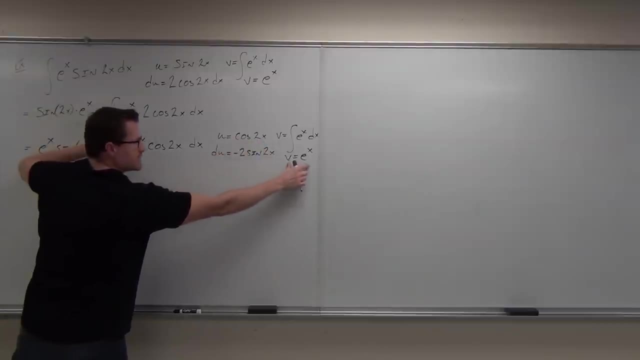 e to the x? u times v. So yeah, you could write cosine two x times e to the x or e to the x times cosine two x, It doesn't matter, It's u times v. So I'm gonna write e to the x, cosine two x. 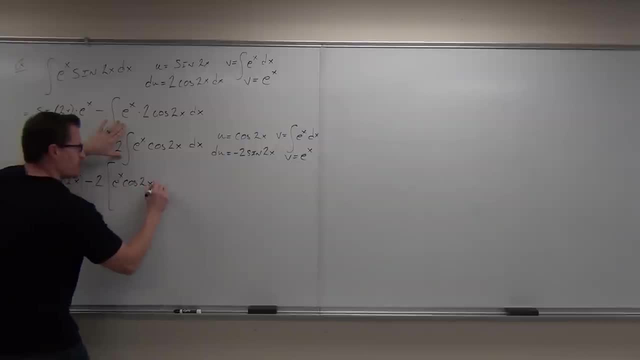 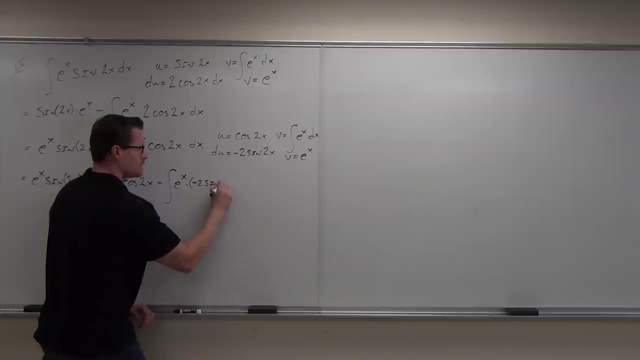 u times v. We just have it in backwards order, Minus the integral of what's going in here v. That's our v, Okay, And then o v du. So negative two times, two x Times. negative two sine two x. 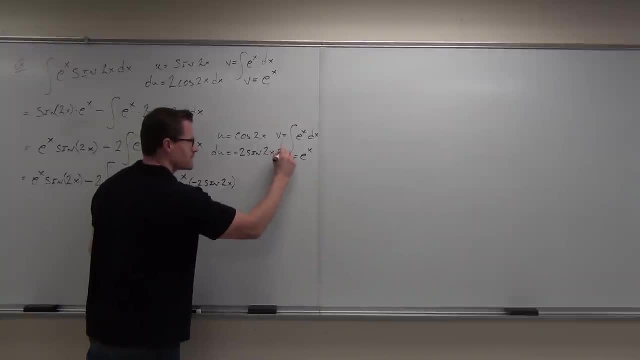 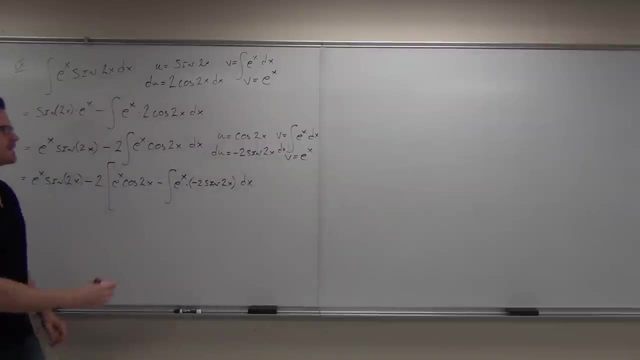 Oh, I forgot something. Do you see what I forgot? Oh, my dx, dx. Sorry, I forgot my dx. Let's double check to see if I'm right, We'll go like a ten second recap to make sure that you guys got it. 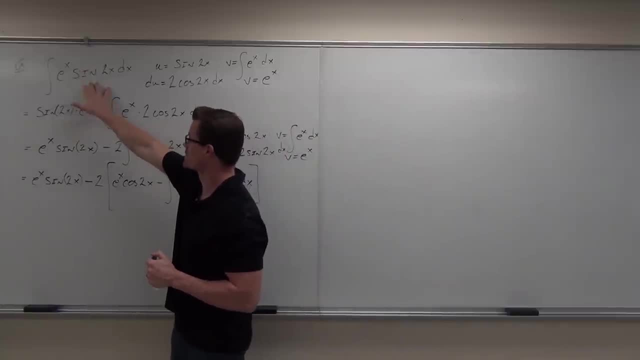 So we're looking here. It doesn't fit our table. We can't do a substitution. We're gonna try integration by parts. We pick something, All right, cool, We'll pick this one. u v is the rest. 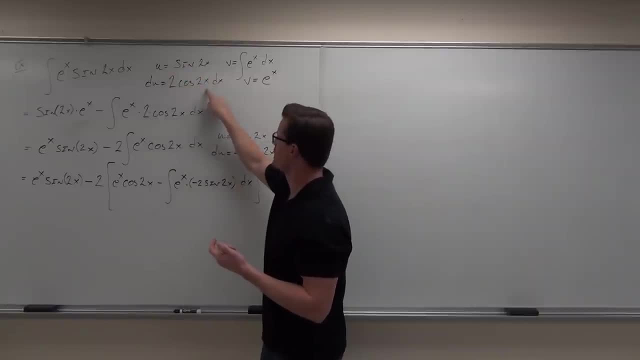 Derivative of u: is this guy by chain rule? Integral of v: is this guy? No problem, We do u times v minus the integral of v, du And we start over again. We simplify, See if we can move anything outside of our integral. 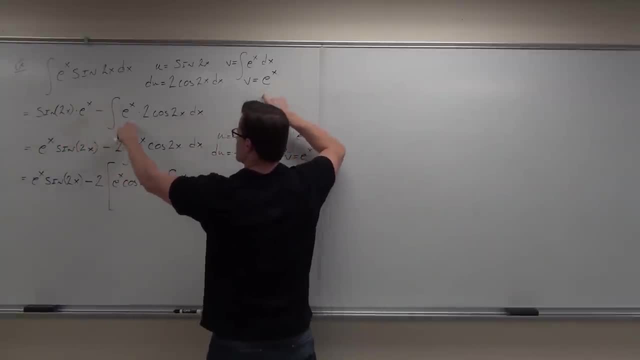 This part, calculus is done. This part minus two integral. Okay, We get something real similar. Well, let's pick the same type of idea here. Let's pick cosine two. x is our u. Okay, v times v. Let's do that. 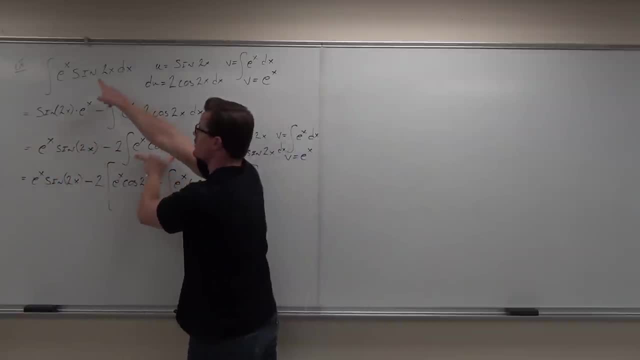 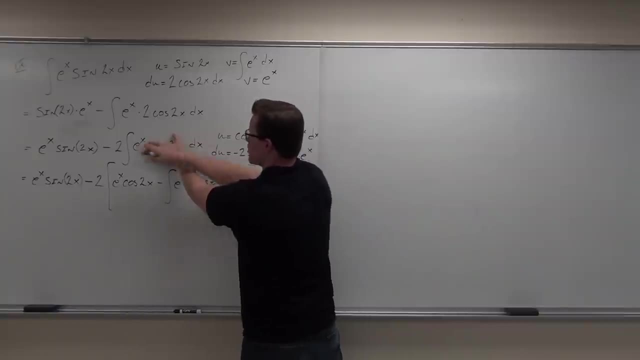 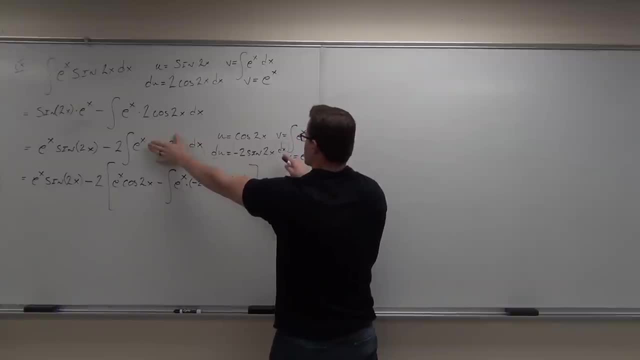 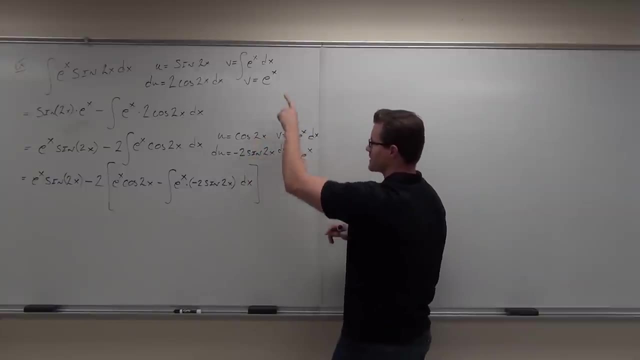 That's outside of our integral. v equals integral of e to the x dx. Okay, Derivative of cosine two x. We can do that Negative two by the chain rule, Sine two x- dx. v is exactly the same as it was before. 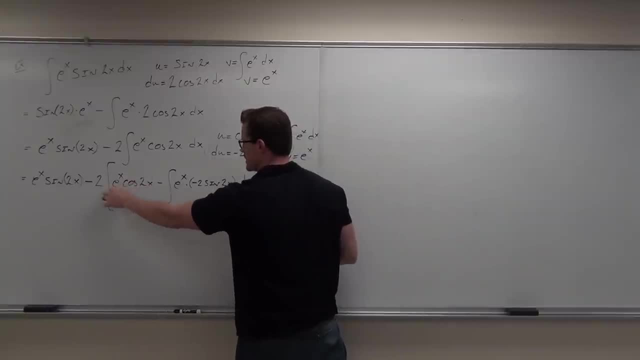 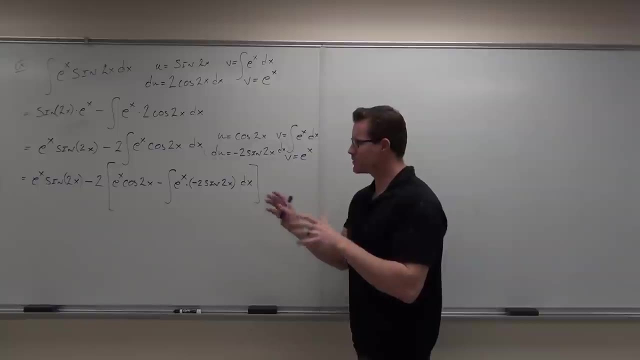 So again we have it. We have u times v minus the integral of v and then another du. You guys, okay with that one. Let's simplify some of this stuff. Let's see what's going on. So what can I do here? 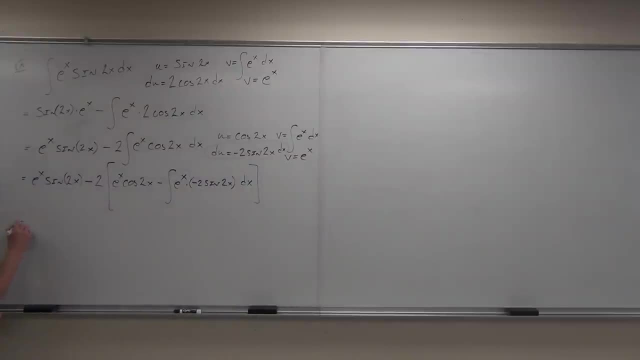 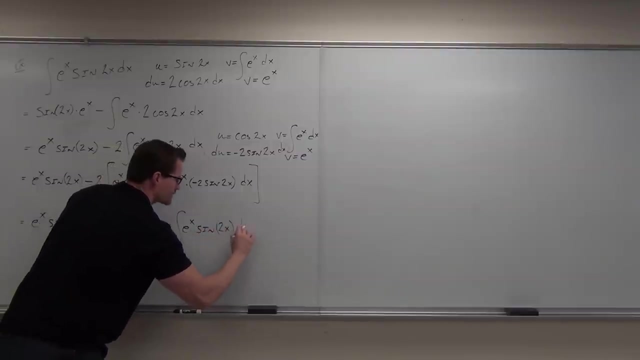 Let's do that. So I'm going to get e to the x sine two x minus two big old bracket. I'm going to get e to the x cosine two x plus two integral e to the x sine two x dx, lots of x. 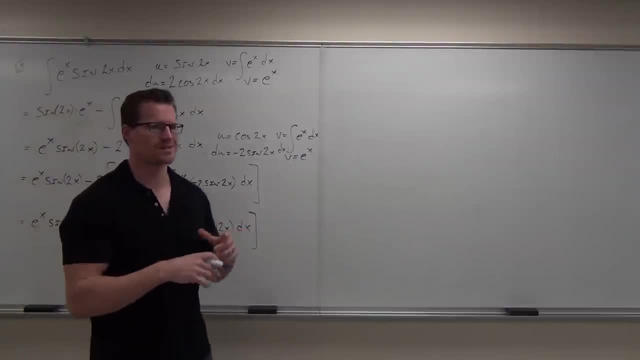 By the way, I like to go slow on this If I do these ones, because the worst thing you can do here is mess the sign up. That would really screw this problem up. Does it make sense to you? So don't mess the signs up here. 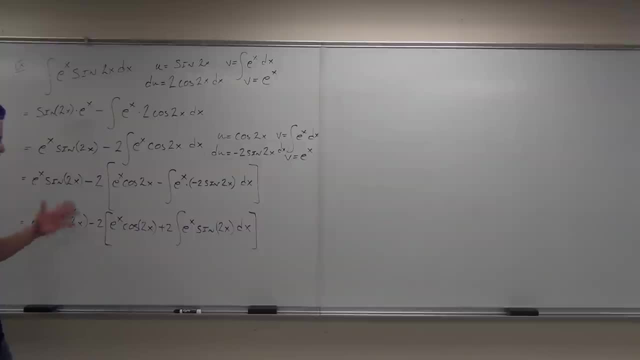 So we're going to go slow, We're going to make sure this is right. What else can I do here? I don't want to factor things. I want to get rid of these brackets. How do I do that? If I do that, if I distribute that, then what we end up getting is something really long. 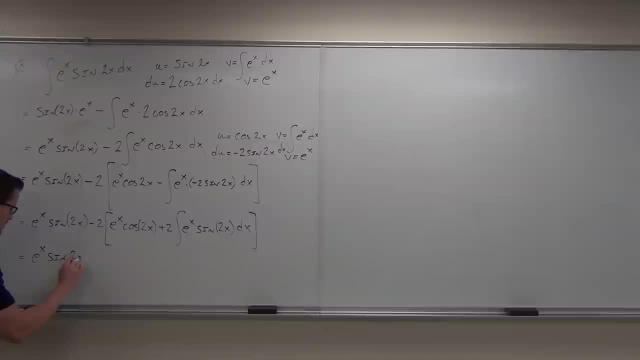 E to the x Sine two x V, Let's see minus 2,. e to the x cosine 2x. Yeah, minus 4, that's very good, because we're going to distribute Minus 4, integral e to the x sine 2x dx. no more brackets. 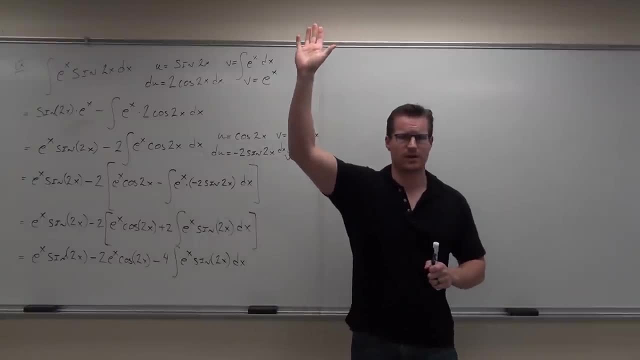 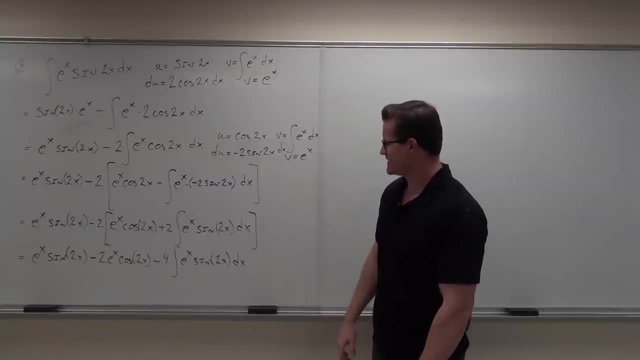 I want to know if, mathematically, you can make it there in your head. if you feel okay with that, we'll show it to you Now. did we do anything great on this problem? What it looks like is that. do you see what happened? 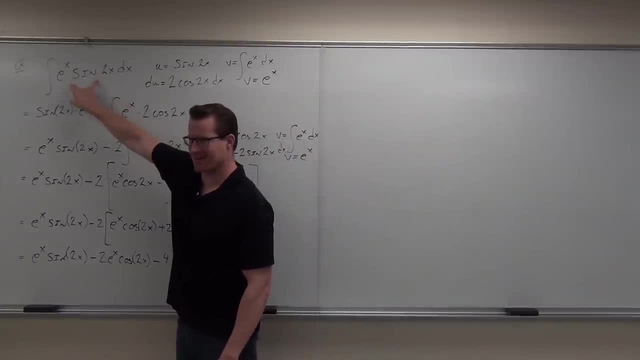 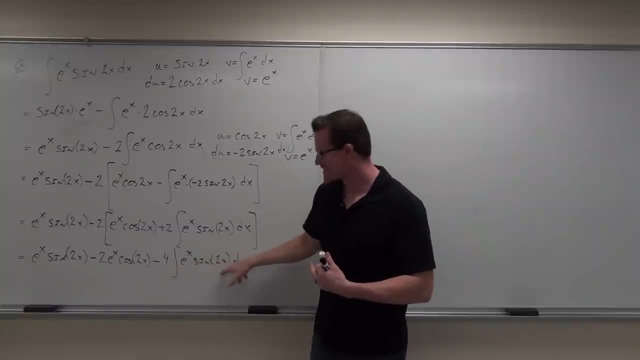 Do you see this? We started here right. We started there. We did all this junk. In fact, we did the junk twice And we got down here and this is exactly like what we started with. So you go: dang, what are we going to do? 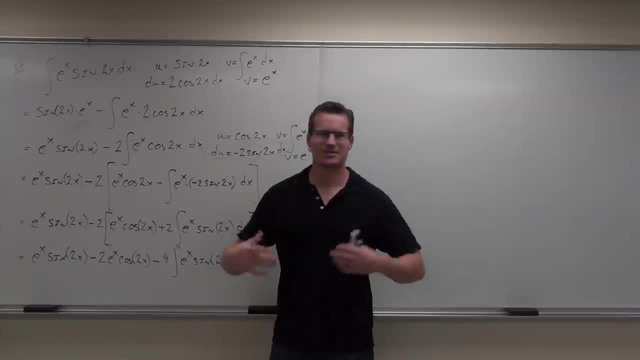 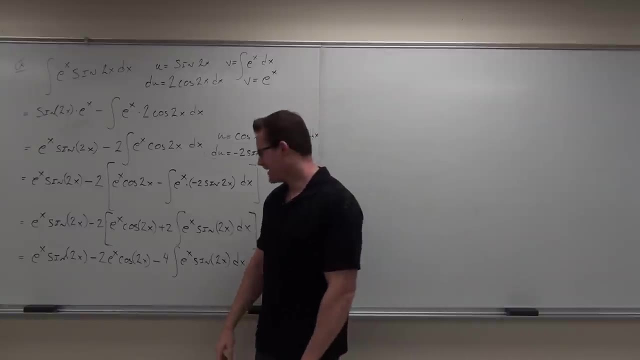 We can do it again If we do it again. that's Einstein's definition of insanity, or something like that. I don't know who it was, but it's the same thing over and over again, expecting a different result If we do this again. unless your math was. 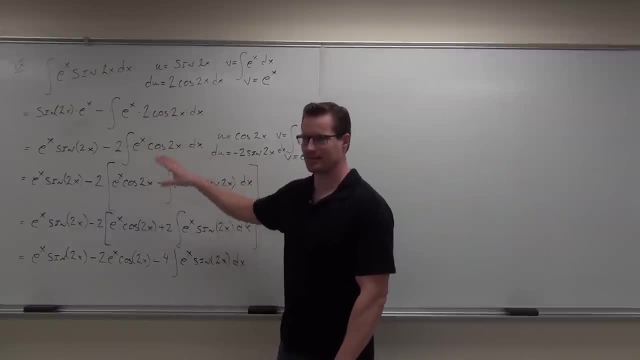 it's completely wrong. you're probably going to get the same thing again and again and again. Does that make sense to you? So this is a problem. So what are you going to do about it? We're going to be smart about it. 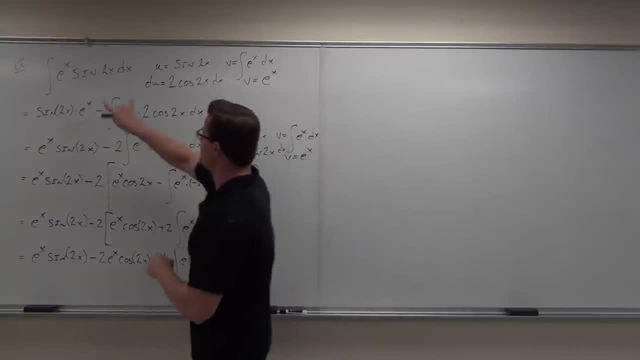 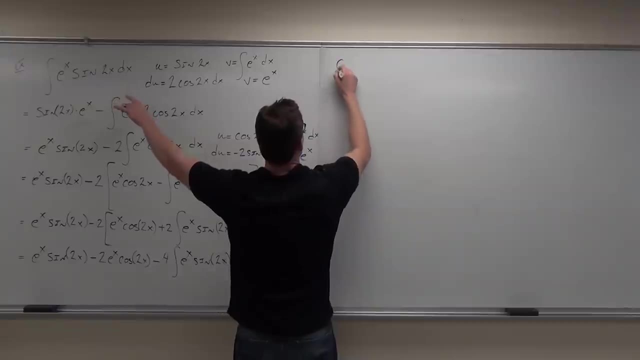 Check this out. Here's what we know. We know that this, this integral, equals this part. Do you believe that? Yeah, Check this out. So what we know is that the integral- don't lose me here- this is the important part. 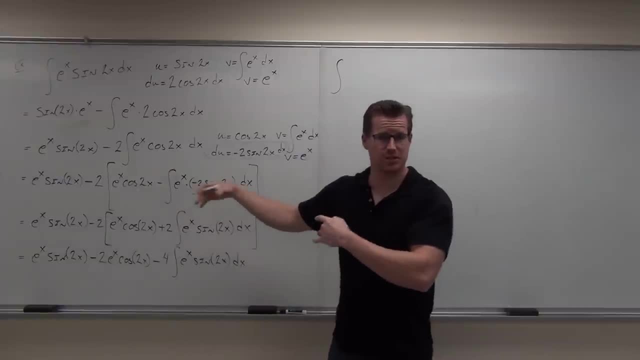 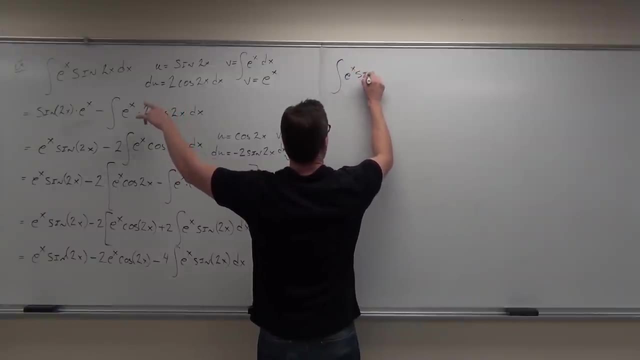 This is easy. You can do this. Everybody can do this right now. This is the interesting part. This is why we're doing this problem right now. So we've got integral e to the x. It's going to be sine 2x. I'm so excited. I'm a little shaky. it's going to be so much fun. 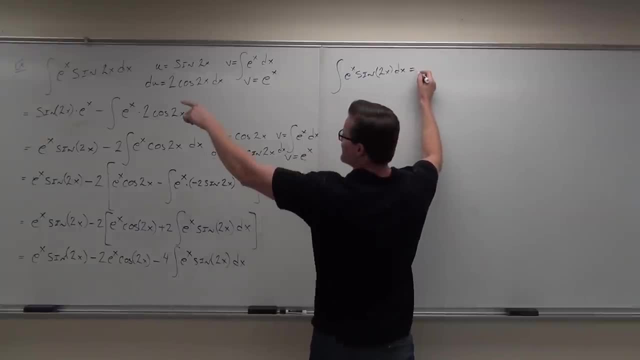 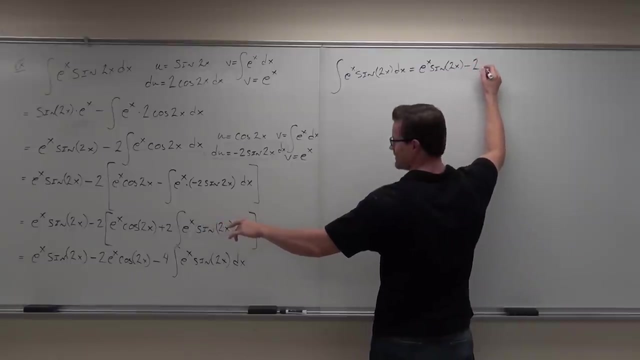 Not really, but it's going to be fun. I'm not shaking. you know, This thing equals- we had equals the whole way down- equals this whole enormous piece of junk. You know, you've been recorded right, All right. 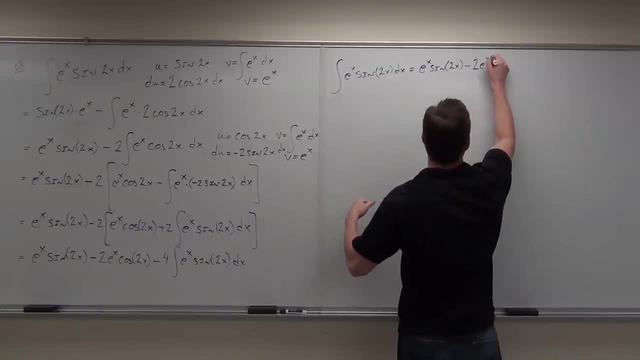 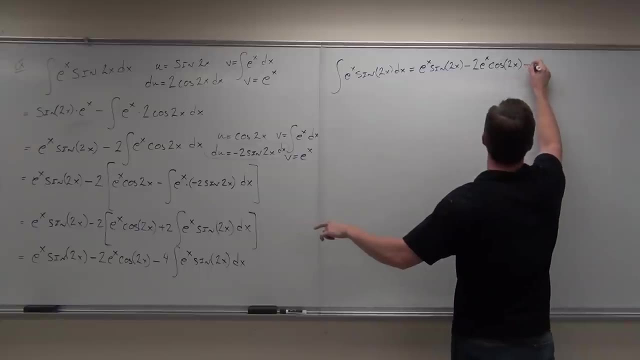 It's okay, You should apologize. You should apologize to the people. They care, I care. Maybe they'll get excited too. He's a fan of India. You're fanning my people in India. Okay, That's long enough. 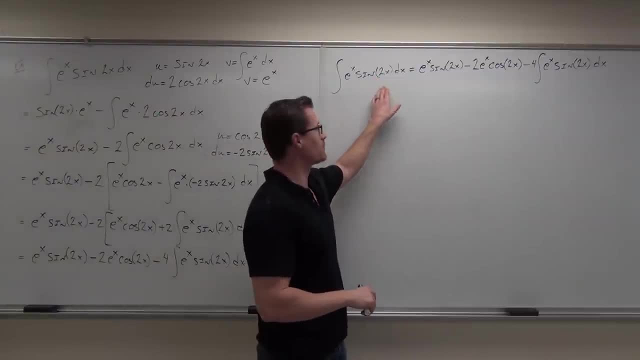 What I want to know is: do you understand this is true, We did the integral of this. It equaled this whole mess of Let's make sure I didn't miss anything. Do I have all the numbers and stuff right? Pretty sure. 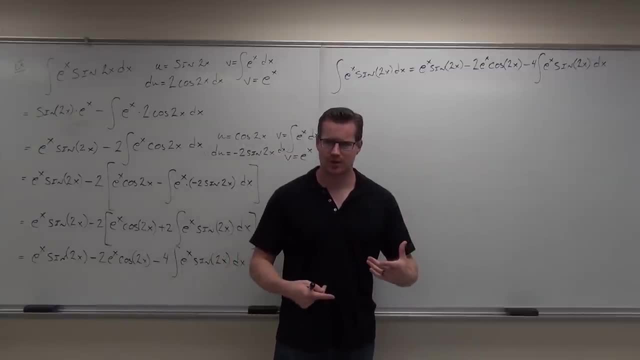 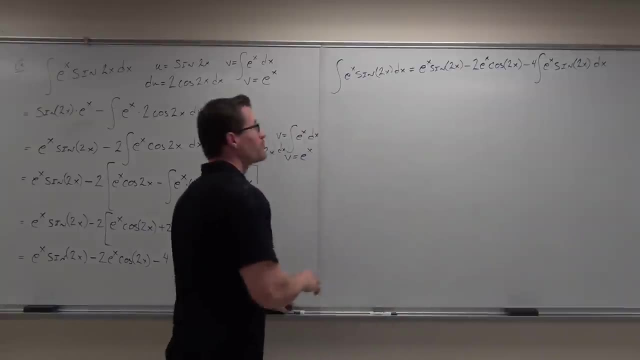 Okay. Do you believe that we have an equation here? Do you believe that you can do anything you want to as long as you do it to the other side? Then what if we do this? We go, wait a second. This part looks great to me. 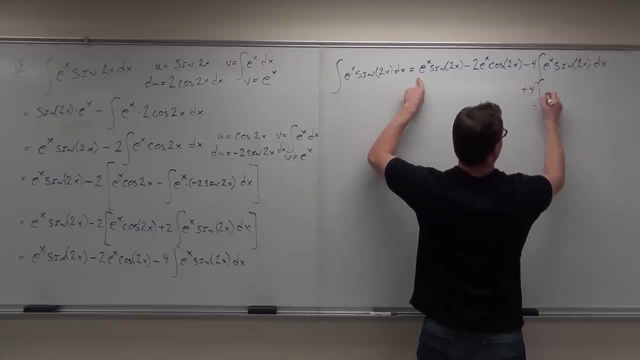 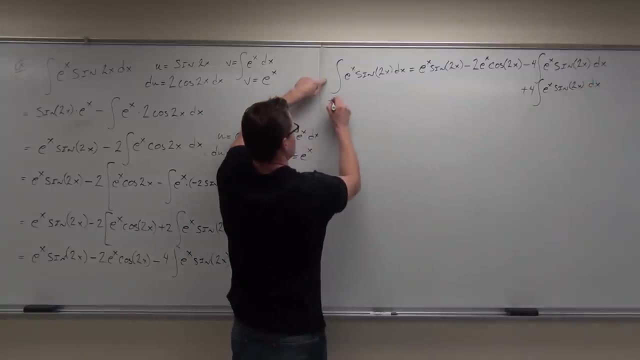 This part looks not so much. but what if I were just to take that and add that: Oh, Oh man, I know right. Oh my God, Here's the whole cool part about this. If you get a piece of your integral back again, like the same thing, 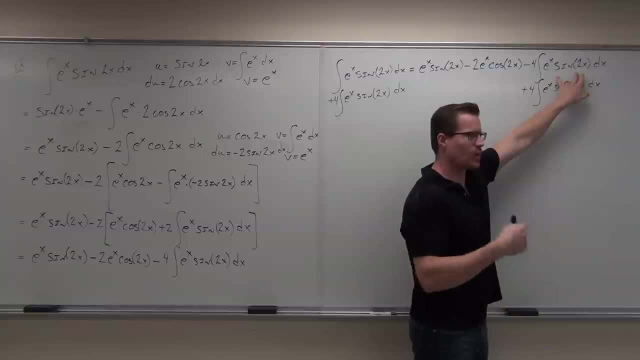 Do you guys see how we get the same exact thing back again. What can we do? Shoot, just add it to both sides. That's going to get rid of that integral. So let's see, We have one of them here. 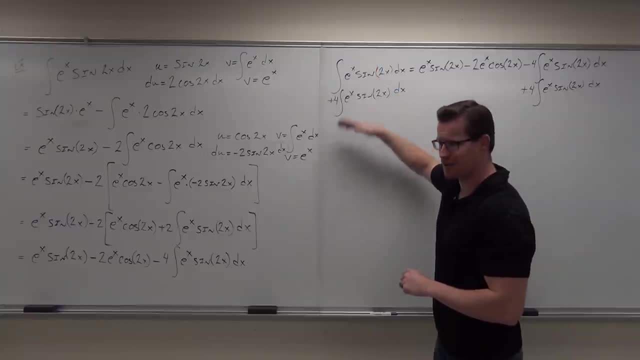 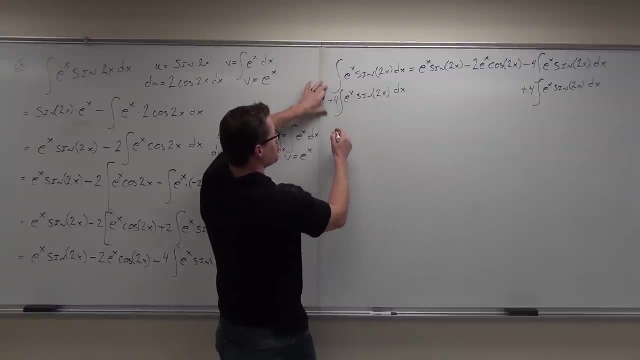 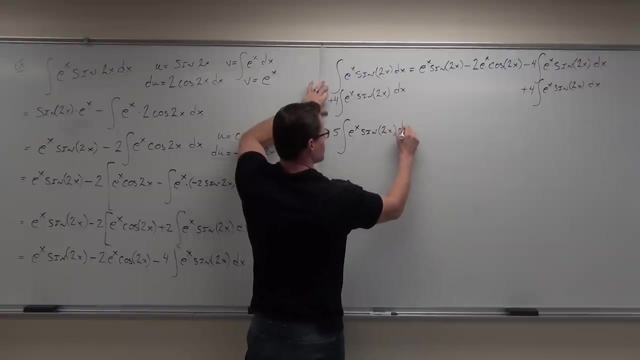 I just added four of them. How much do I have Five? I have five of them, So we're treating this thing like the equation that it actually is. So one plus four equals five times the integral e to the x. sine 2x dx equals. 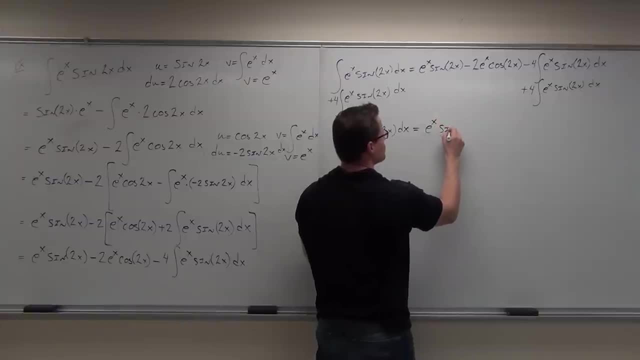 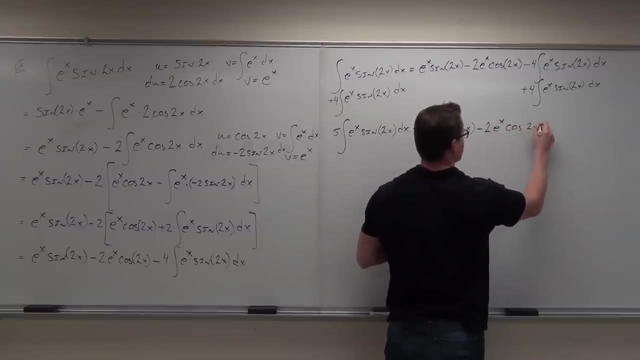 Well, this is awesome. I have e to the x, I've got sine 2x minus 2. e to the x, cosine 2x. What happened to this Gone? I added it over, Completely gone. So the whole idea here is this. 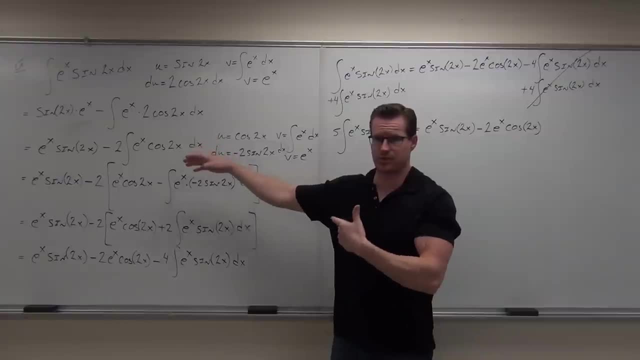 Well, maybe you're not on the wrong track. Maybe you're actually on the completely right track. You just get the same exact thing back. You go wait a minute, Man, I blew this thing up. No, no, You did it right. 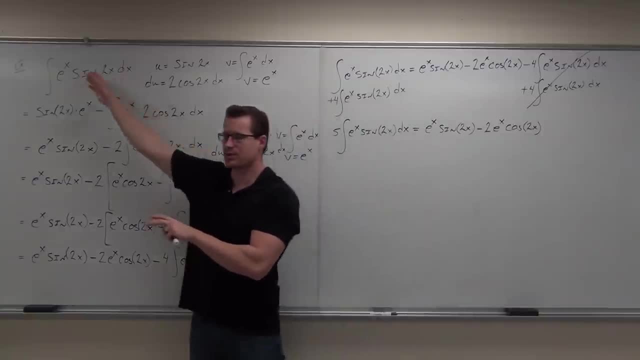 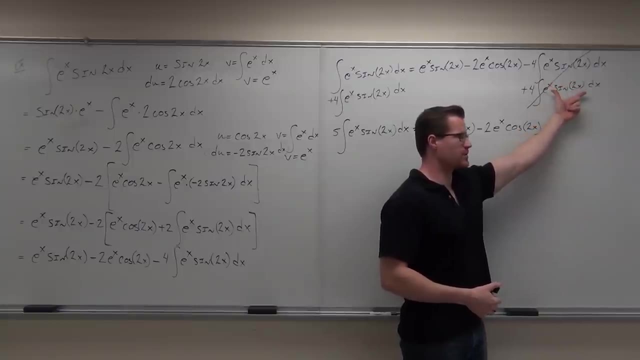 So if we have all but the last integral- and the last integral is exactly what we started with- just add it to both sides like this: Shoot: hey, We have minus four, Just add four, Add four times the integral of this whole thing. 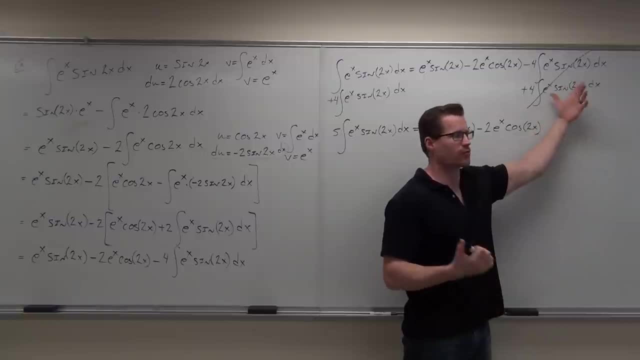 It's going to get rid of it, Just like if you had minus 4x and you add 4x, Hello, it's gone. Add it to both sides. Here's five. We only have to do one more thing. We've got to get rid of this five. 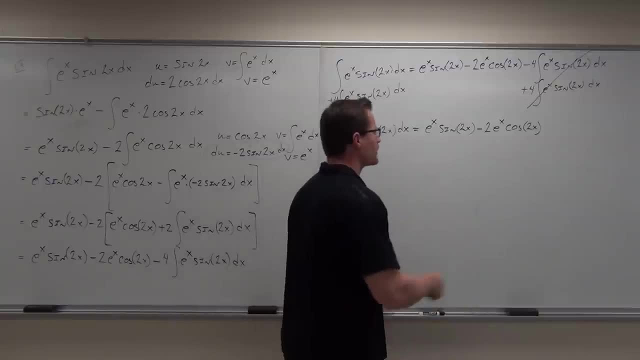 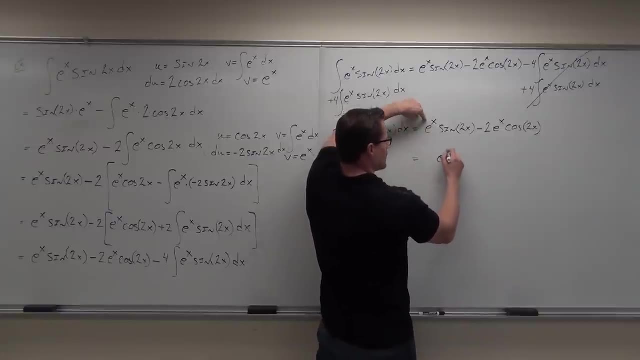 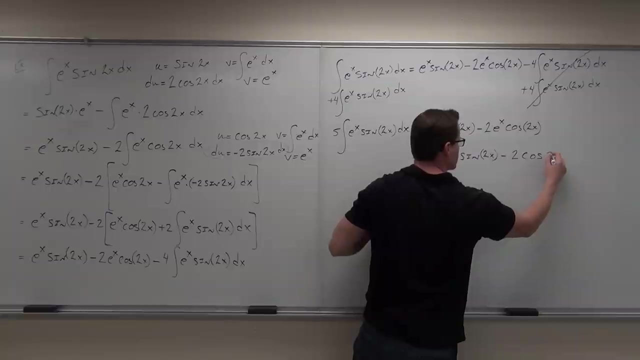 How do you do it? Five by five? So I'm going to do a couple things right now. First thing I'm going to do is factor out my e to the x, so that's possible. So over here, if I factor that out, I've got e to the x, sine 2x minus 2, cosine 2x. 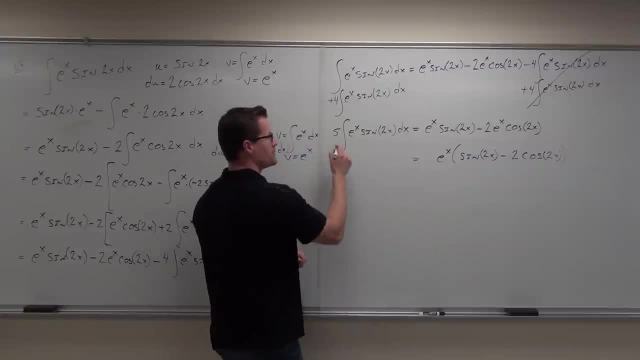 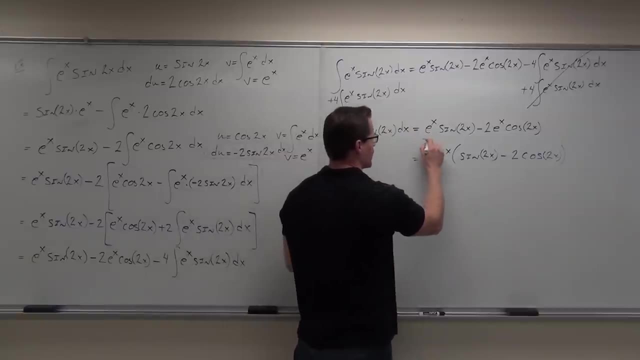 So I've just factored out my e to the x, And then, if I wanted to get the, if I wanted to get the 5 over there, I do what now? Divide by 5.. If I divide by 5,, I divide by 5, then I end up getting 1 5th. 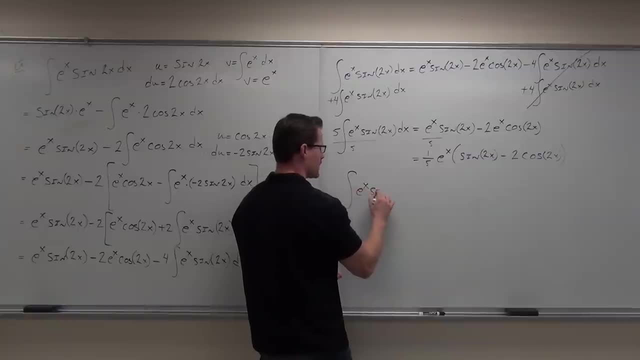 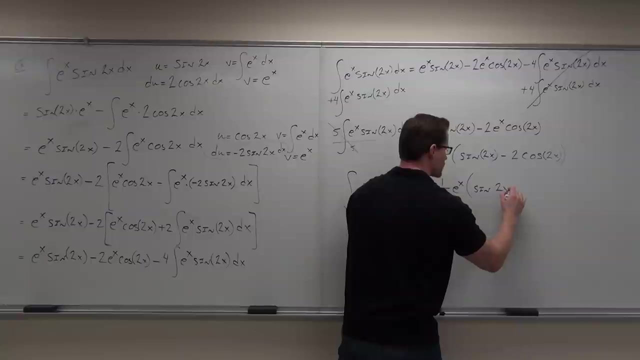 So our integral of e to the x sine 2x dx, What we wanted to find out, we know. since we divided by 5, this is gone. We get 1, 5th over here. 1, 5th e to the x sine 2x minus 2x. 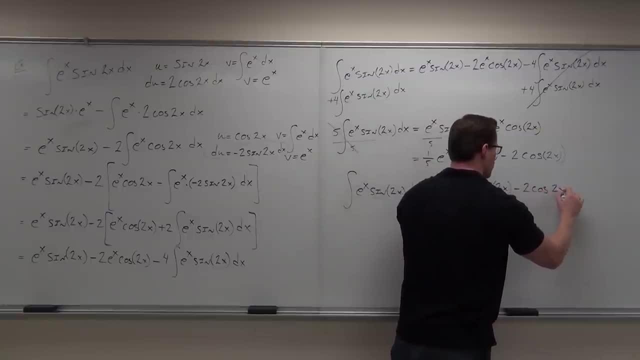 That's 1, 5th e to the x. So we get 1, 5th e to the x: sine 2x minus 2x, 2 cosine 2x. One thing I'm missing. What am I missing? 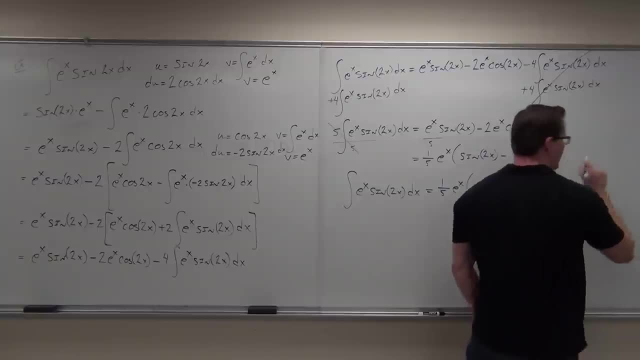 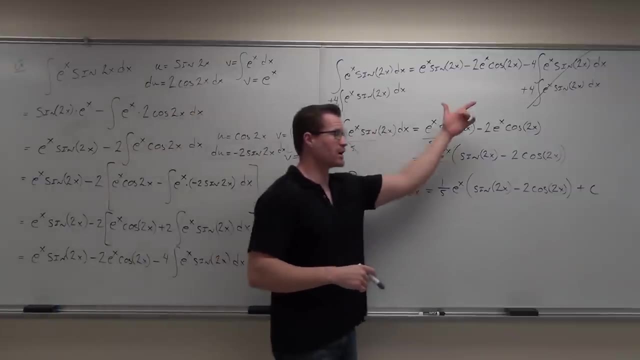 Plus C. Do the plus C. Oh my gosh. Well, isn't that cool, Isn't that kind of exciting? It's interesting, isn't it? How are we going to do it? Well, if you get the same thing back, you can add it to both sides. 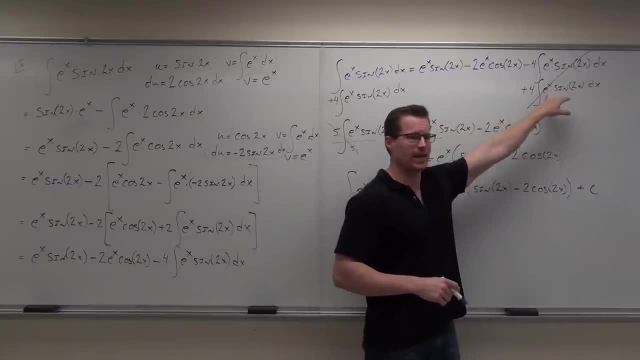 Then all you have to do is divide. This addition gets rid of the. that you can't do. You can't do that by itself, You've got to do it this way. So if you just add to both sides, you're done. 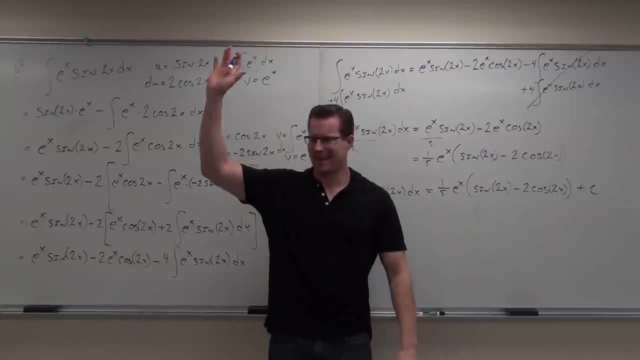 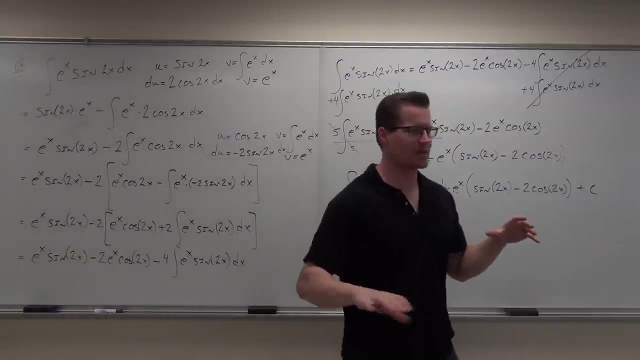 Just divide by 5, and we're good to go. So you guys feel okay with that one. Isn't that kind of interesting? Yeah, it's cool, right Cool, thank you. Any questions or comments? I've got to erase this whole thing right now because these problems, besides the next one, 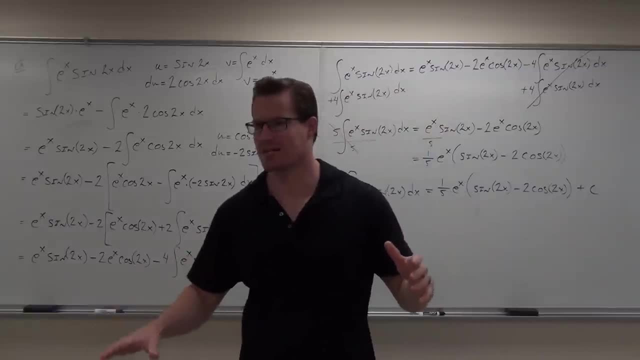 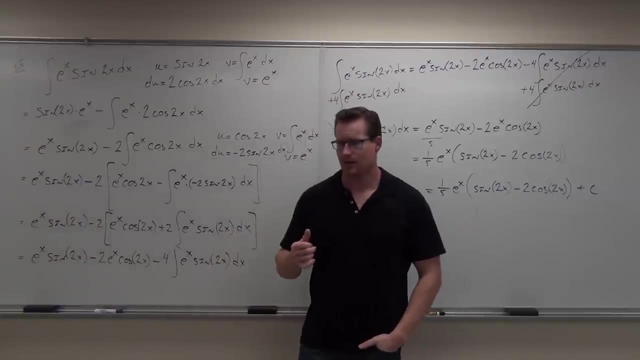 are going to take up the entire board every time. The next one might even take up more than the entire board Question. So the only time you would do that like add an integral to the other side, is when you get the same thing back twice and you do parts twice. 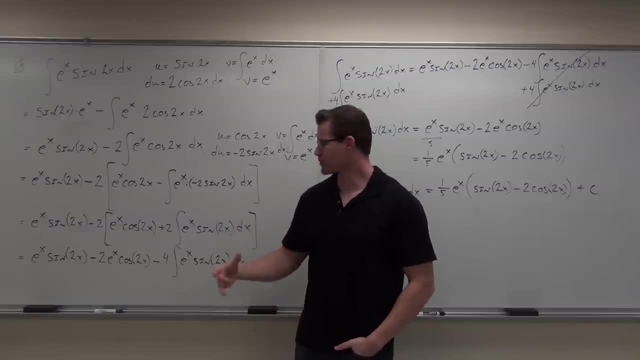 I don't know if it's twice, but if you get it back again and there's one integral and it's exactly like what you started with, why wouldn't you do that? If it's exactly the same, you go, wait a minute, I just got back the same thing. 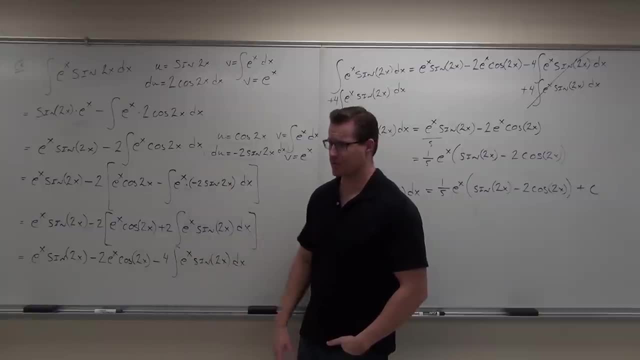 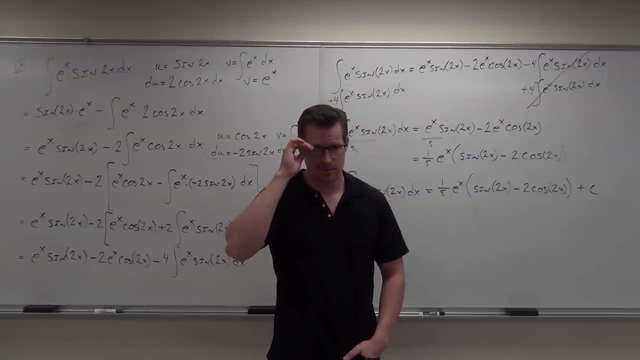 Either I did it completely wrong or it's just perfect, because I'm just going to add that to both sides and divide by whatever the constant is the coefficient, Because you have two looping terms. would it matter if you switch the e to the x and the cosine? 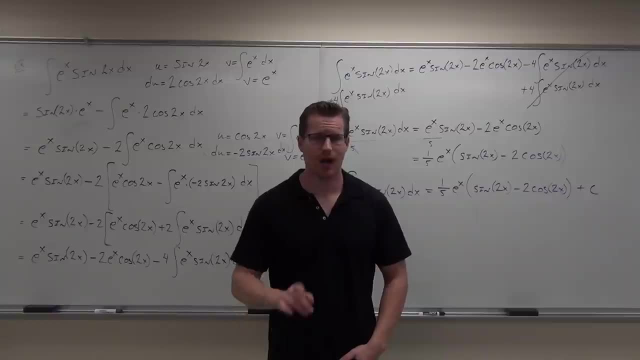 I don't think so, and I haven't done it. I think I did it a long time ago. I don't think it matters. My point here was: just pick the same thing, though. Pick sine x, pick cosine x. If you did e to the x, you could do the integral with sine 2x, no problem. 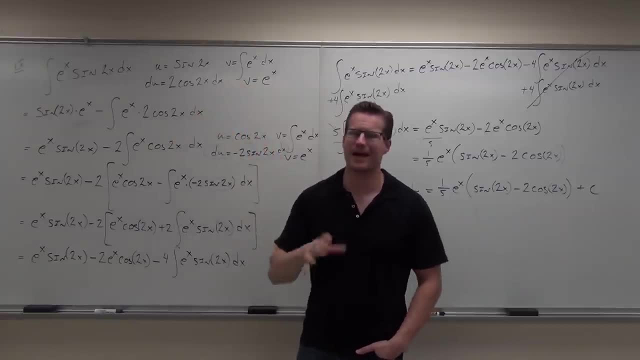 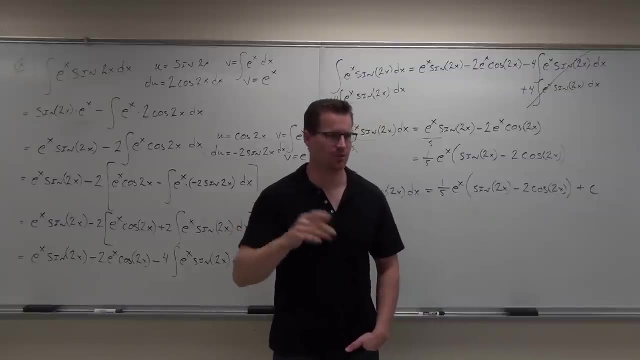 You just have to pick that again. I think this is a better way, but I haven't done it the other way. I like it this way because it worked out really nice. I didn't have to worry about integrals. That's why I picked it, because the integral of e to the x is very easy. 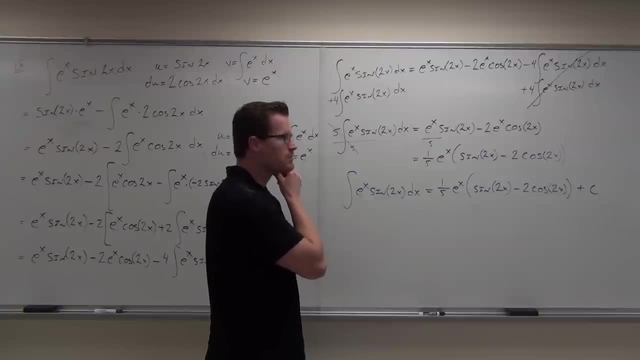 Question: If this was on, if this was a homework problem, is that what our answer would look like? That is your answer. Okay, Other questions? All right, can we try another one? Yeah, I asked you a while back when we were doing one of these things. 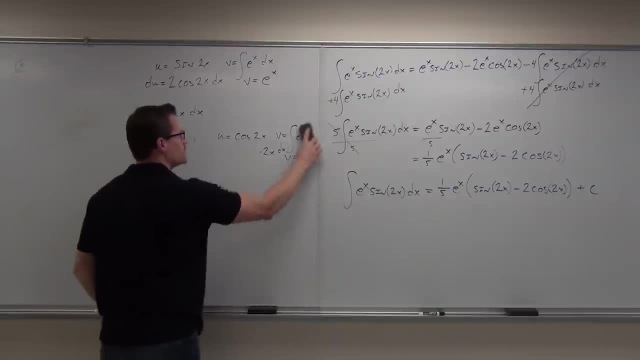 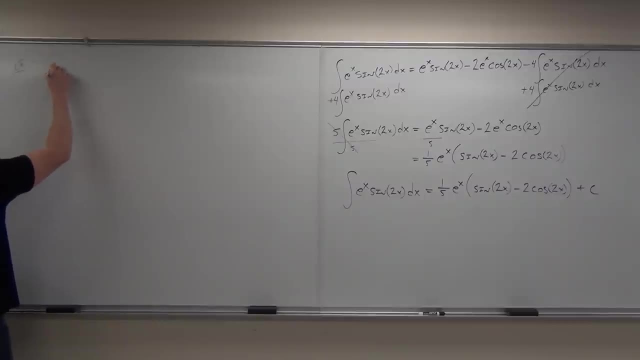 it was integration by point. I said: hey, what are you going to do if I give you a problem like? I don't remember what it was? I think it was something like xlnx or something like this. Remember that. So what are we going to pick? 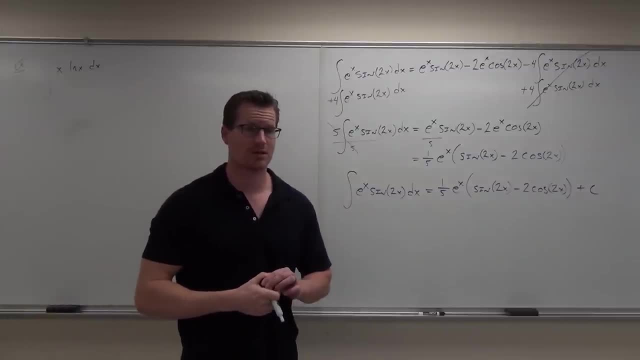 And some of you guys said, well, let's pick. u equals lnx. I said, really, So, oh sorry, u equals x and v would equal the integral of lnx. I said, well, do you know what the integral of lnx actually is? 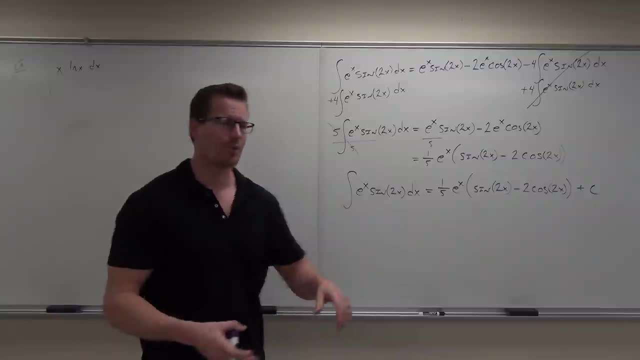 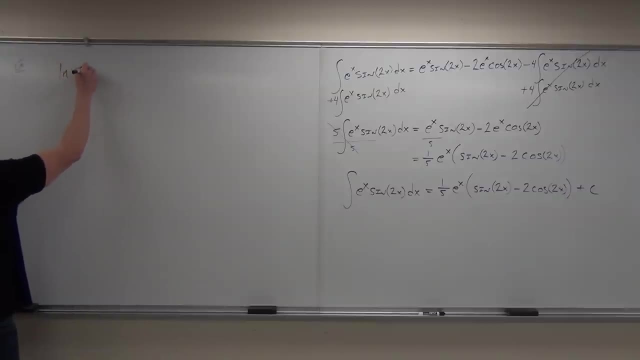 Do you know what the integral of lnx is? No, we don't. Well, now, what I'm going to do is, instead of asking you this problem or something similar, I'm going to ask you this problem: What is the integral of lnx? 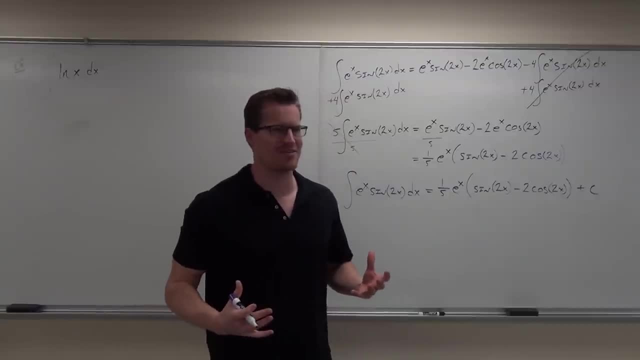 I'm asking for integrals, not derivatives. Ah, Hulk angry, Just joking. I'm wearing a black shirt, Yeah, and jeans. So do you know what the integral of lnx is? Do you know what the derivative of lnx is? 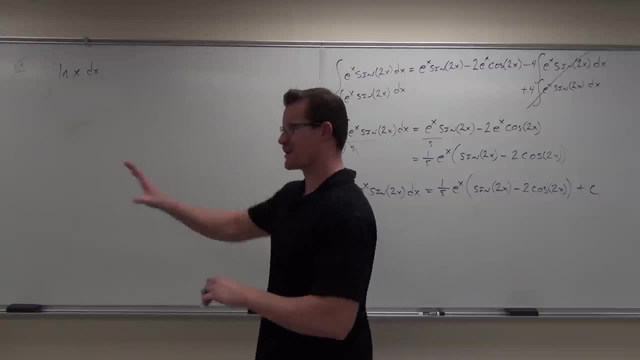 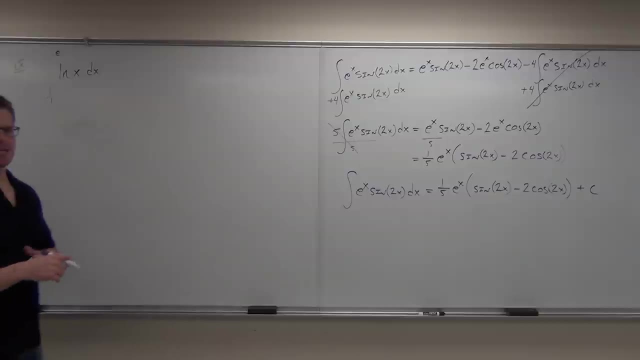 Yes, That's 1 over x. So here's what we're going to do. We're going to get a little bit more interesting too. I'm going to ask you, how much is this from 1 to e? Now, of course, the 1 to e part. that's really easy. 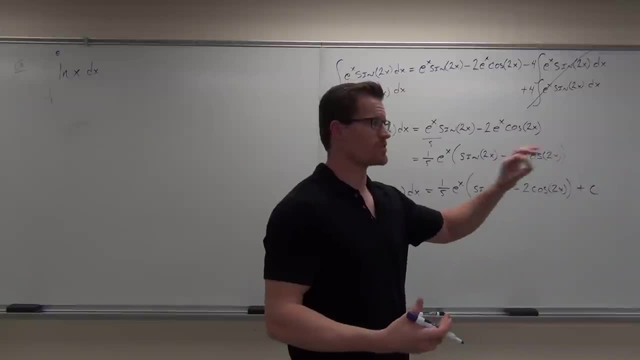 We're just going to take care of that at the very end, okay. So when we're going through integration by parts, though, I really want to figure out what's the integral of lnx. Okay, well, let's start picking, let's start going through our process. 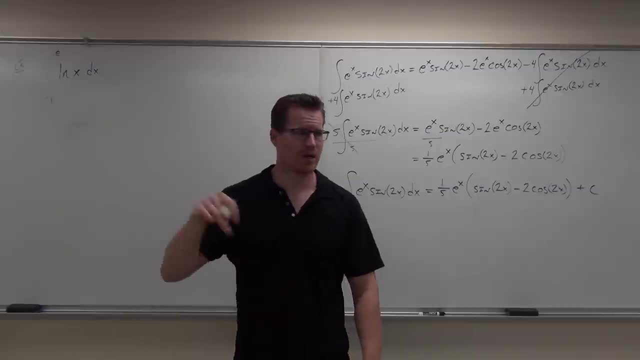 Is that part of our integration table? No, It's about to be. Is it right now? No, Will a substitution work? If we do a substitution of u equals lnx, the derivative is 1 over x. Do you see 1 over x anywhere up there? 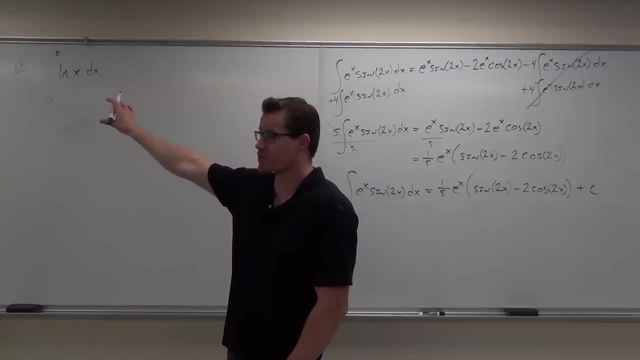 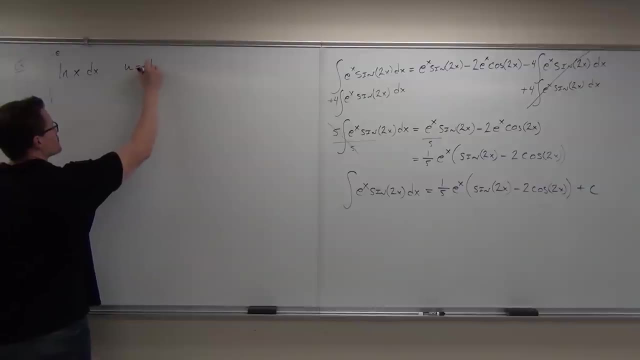 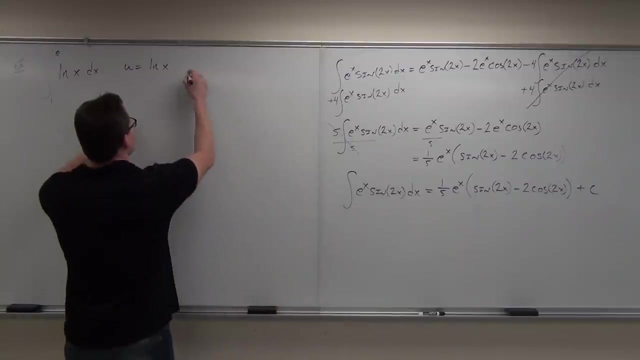 No, Substitution won't work. The only thing we have left is integration by parts. The only thing we can pick is what? lnx? Okay, so u equals lnx. Now if u equals lnx. see if you guys are thinking outside the box here. 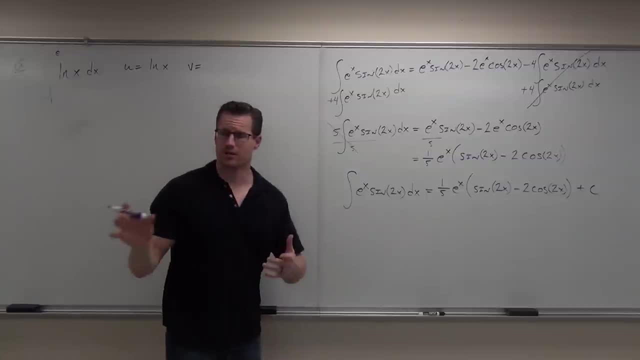 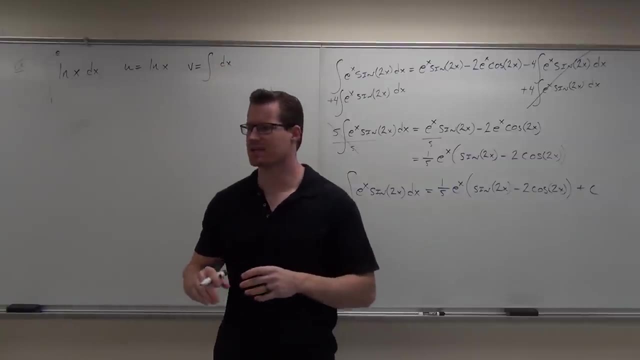 dx. How much is v dx? It's got to have an integral 1 dx, Integral dx. If you don't know what integral dx means, integral dx means integral of 1 dx, So remember how x is 1x. 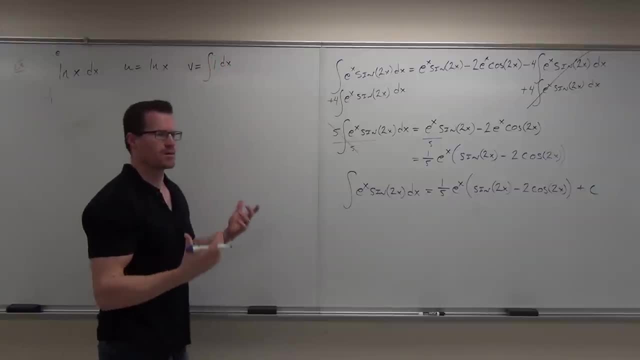 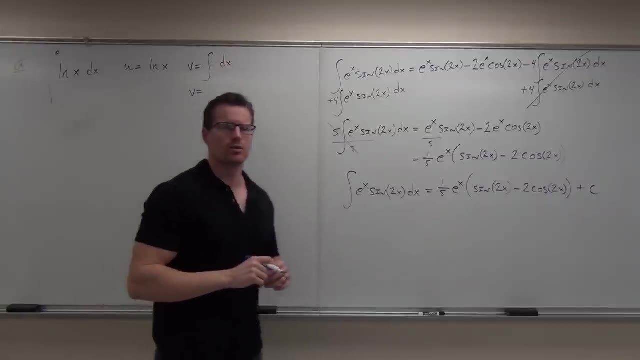 Integral dx is really integral 1 dx. A lot of people don't write the 1, but it's there, So let's see. Let's just start with a v. How much is the integral of dx or 1 dx x? 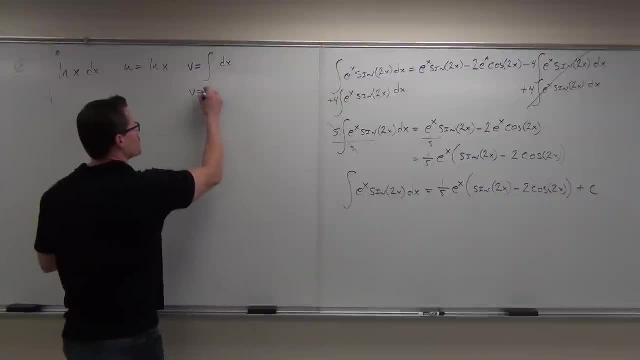 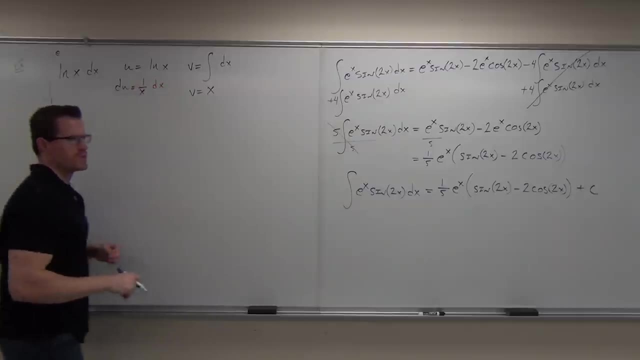 It's x. Yeah, the integral of 1 is just x. You guys? okay with that one. Yeah, We know that du equals 1 over x dx. That's actually pretty easy. We know what the derivative of lnx is: 1 over x dx. 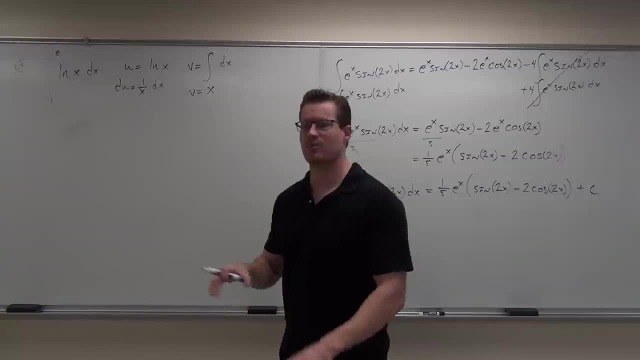 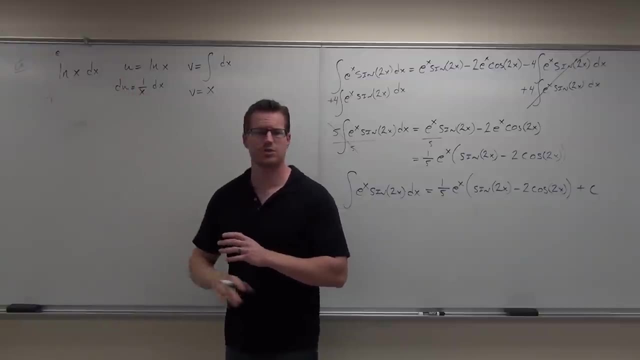 Show of hands. if you're okay with that so far, Let's start putting this thing together. By the way, you don't start evaluating this right now. You wait to the very end to evaluate from 1 to e. okay, You don't have to change bounds in this, because if you think back to integration by parts, 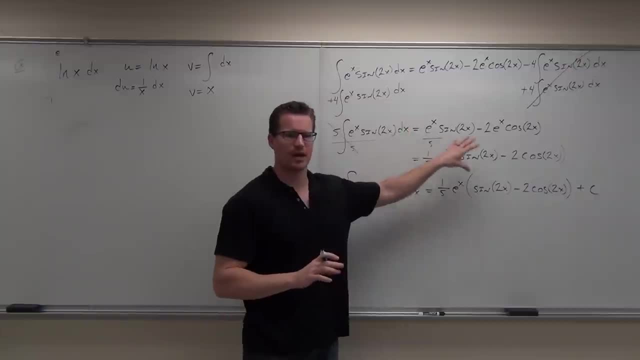 well, what happens is you're using u times v that are already in terms of x. You don't have to do a substitution here. So don't worry about Change of bounds, Don't worry about that stuff. You just evaluate at the very, very end. 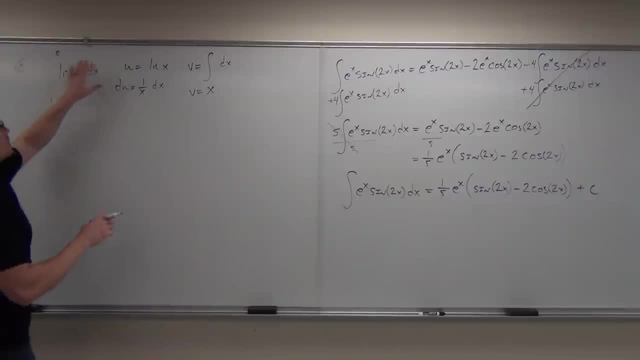 Does that make sense to you? Okay, so we know that we pick u. The only thing we have to pick is lnx. The rest of it is integral of dx, That's x. So v equals x. We're going to do u times v minus the integral of v du. 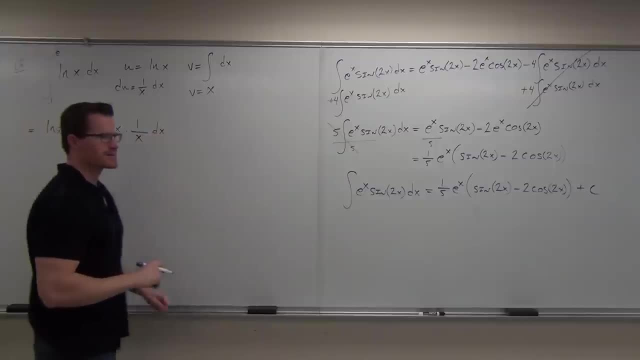 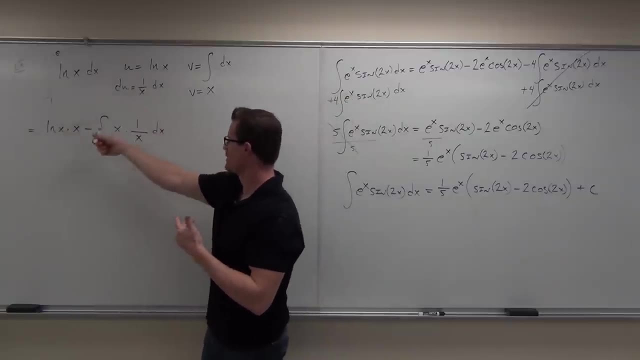 Only du is 1 over x dx. Now that's kind of interesting, You guys, okay with what we've done so far. u? u v, got it minus the integral of v, no problem. So u times v minus integral of v and this part is our du. 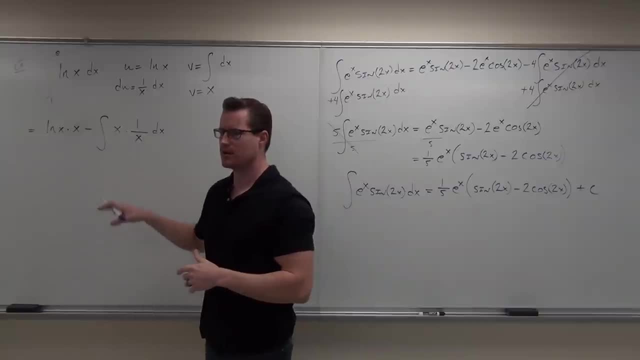 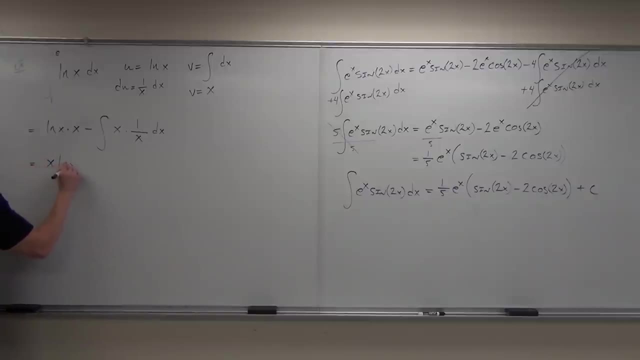 Look at what happens in this integral. What's going to happen? What am I having there? 1.. So I'm going to reverse these because it looks a little funny. So I'm going to have x, lnx minus the integral of hello 1, or just dx again. 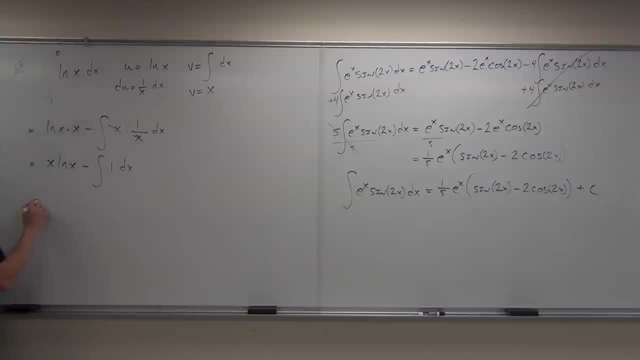 Can you do that? Can you do that integral? Yes, It's actually really easy. That's x, lnx minus hello. Now, if I didn't have my 1 to e, you'd put a plus c. If I didn't have my 1 to e, you'd put a plus c. 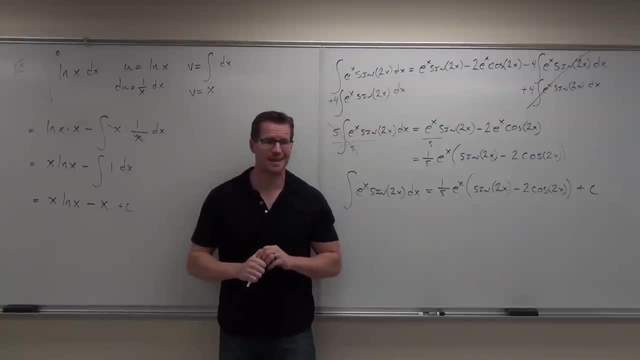 That's actually the integral of lnx. The integral of lnx is x lnx minus x or x times lnx minus 1, if you wanted to factor that, That is the integral. We actually just did it. It's really easy. 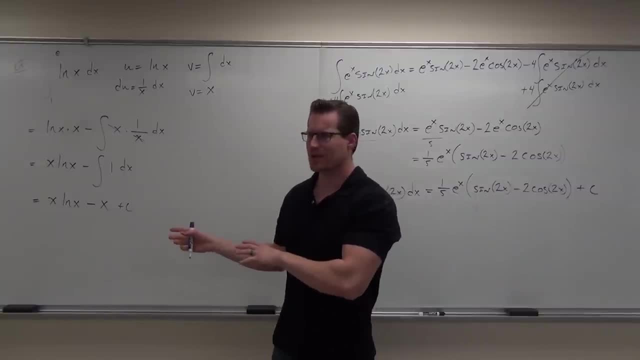 It's really easy if you do integration by parts. It's kind of cool, though, right, We can invent our own integration tables with some of this stuff, like with integral of lnx. So if I'm asking you to go from 1 to e, I don't have a plus c, because now it's a definite integral. 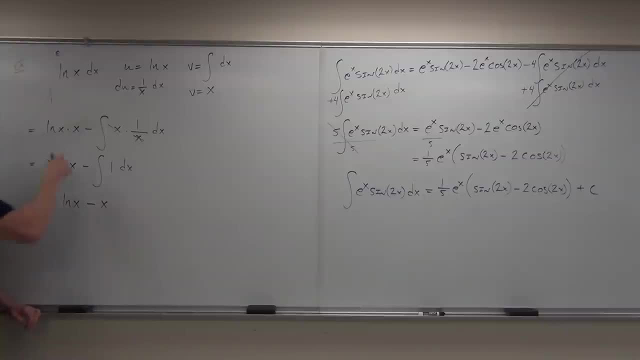 How you write this. you don't continue to write your integral because you actually just did your integral correct. This would be silly to write. You've done it. How you write the evaluation is you either put a bracket like this or the line, or even a bracket. 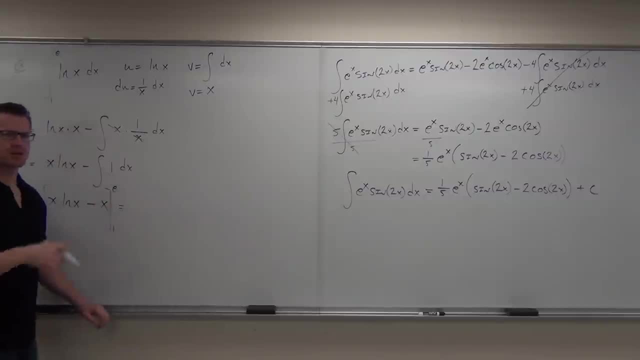 and we go 1 to e and then we just plug it in. So here we have e ln e minus e minus 1 times ln of 1 minus 1.. Let's see what happens here. Most of this stuff should be kind of nice. 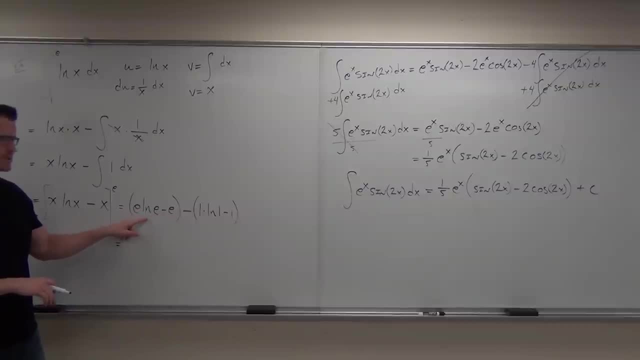 How much is ln e 1.. This is 1.. So we have e minus e e times 1 minus e minus. okay, how about ln 1? 0.. This is 0.. 0 minus 1.. 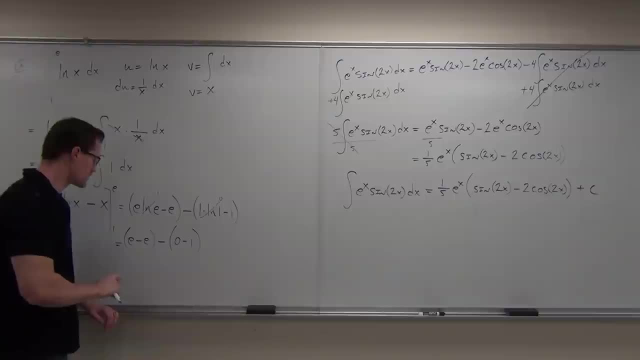 That's still there. You don't just get 0's everywhere when you plug in 0, or when you sorry, when you get 1, 0.. So this is 1, e times 1 is e minus. e okay, big ol' minus ln, 1 is 0.. 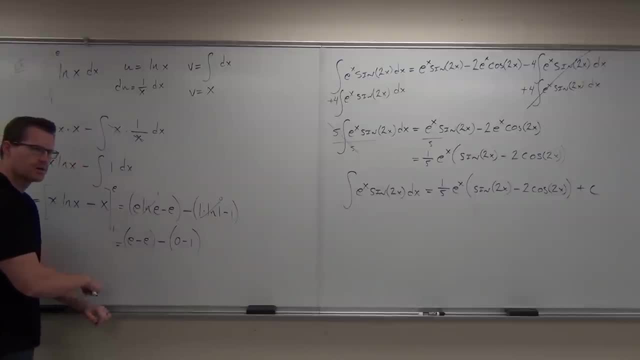 So 1 times 0 is 0 minus 1.. How much is 1?? It's 1.. How much is this whole thing? 1. It's 1. Now, that's interesting. I think that's really interesting. 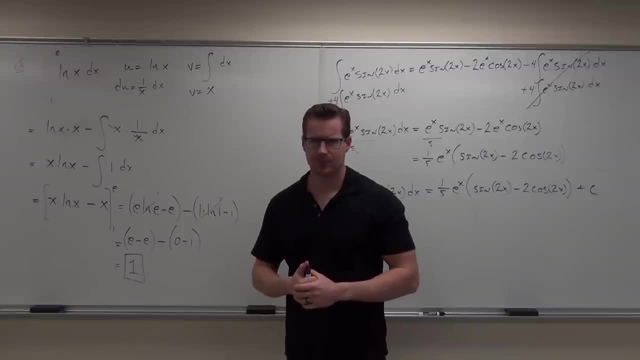 Do you remember what integrals actually mean? A reverse derivative? It is an antiderivative. Well, what I mean is a derivative is a rate of change or the slope of a curve at a point. Do you remember that? Yeah, 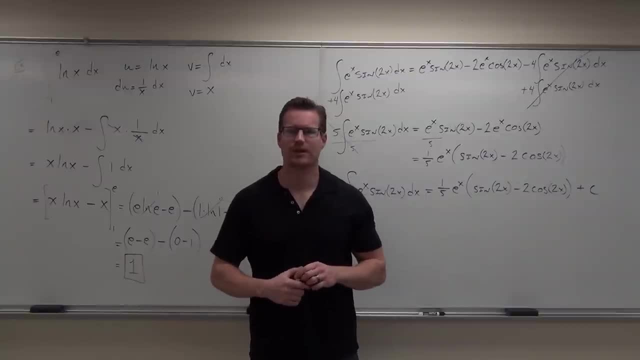 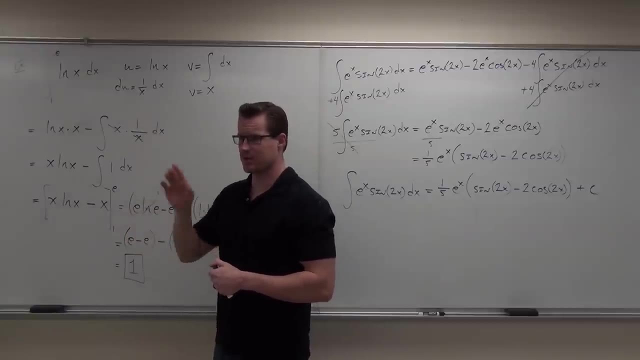 That's what a derivative is. What's an integral? Area under a curve? That's right. So a definite integral is the area under a curve between two points, The area under the curve ln, x Between 1 and 1.. And e. 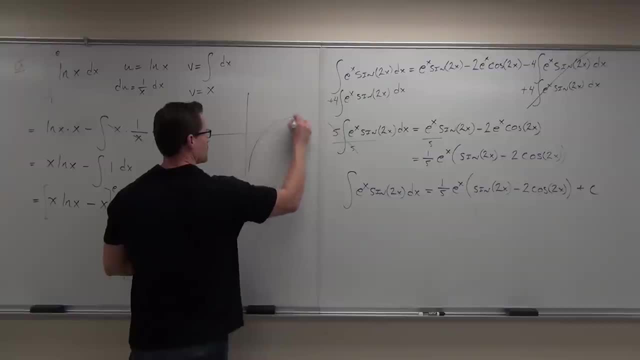 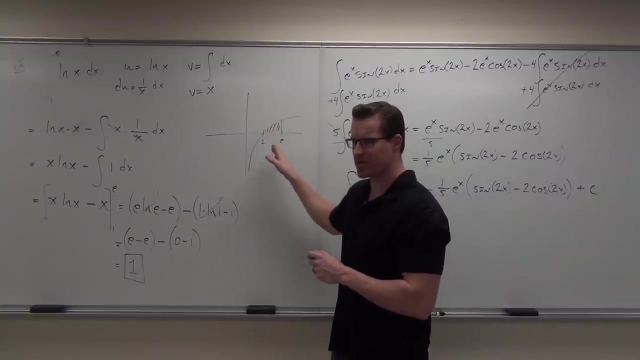 If you know what ln x looks like, it looks like this: It crosses at the point 1.. Here would be the point e. The area under this curve is exactly 1.. Is that not weird? So the area under ln x between 1 and an irrational number, e 2.7, blah, blah, blah, blah, blah, blah. 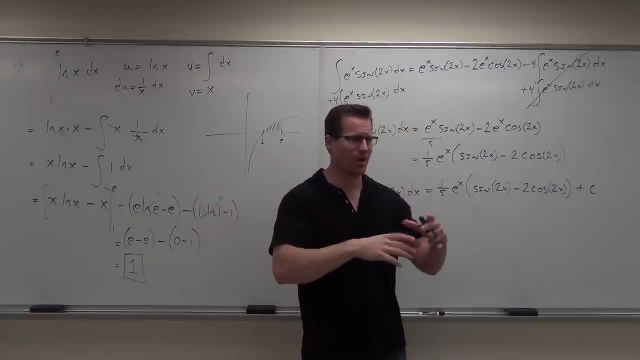 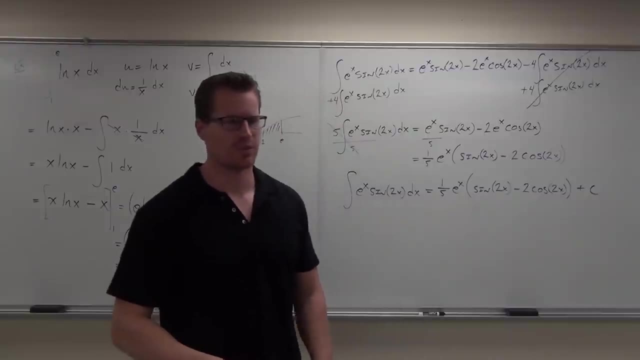 forever. if you find the area under there, it is exactly 1.. I think that's just amazing. I don't know why, but I think that's so cool. Anyway, we can find the integral of ln x now And we can even evaluate it with different integrals. 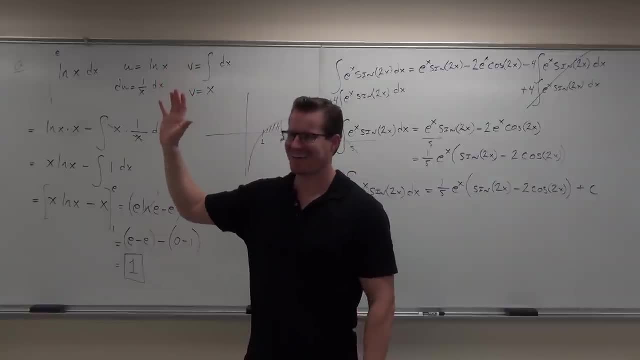 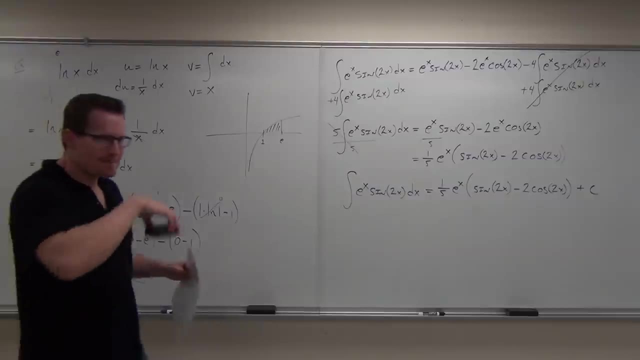 So you'll be okay with that. one Interesting stuff today. That's interesting, It is right, I think. so Now are you ready for the hardest one that we're going to do today? This is going to be ridiculous, all right. 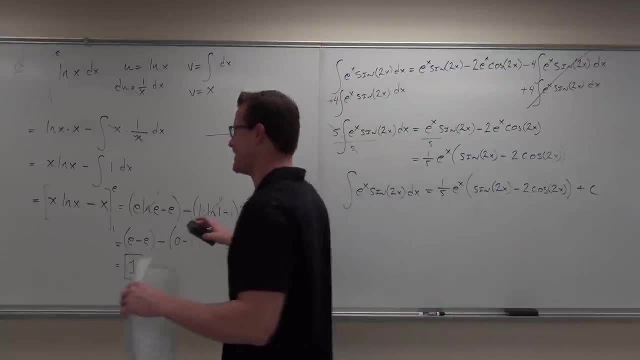 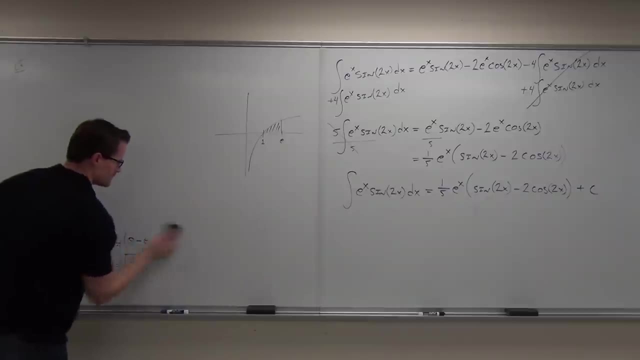 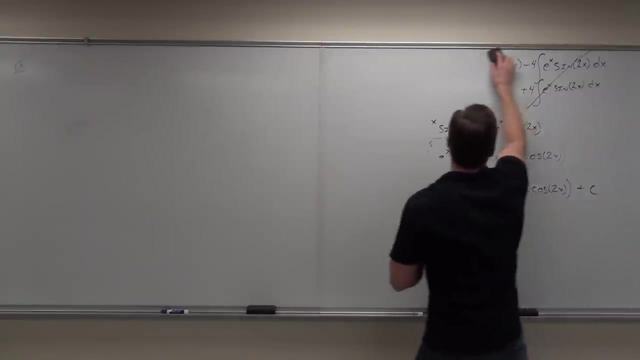 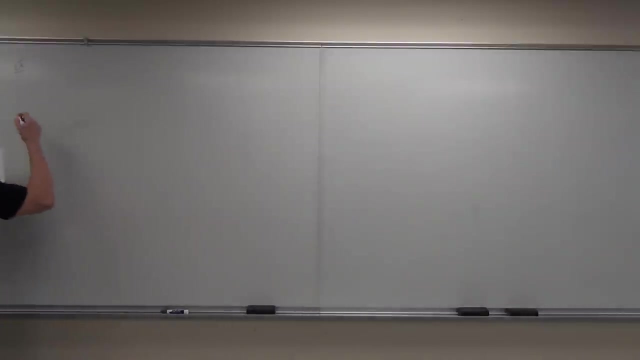 We're going to have a lot of work today. It looks so simple to start with, but it's not going to be Okay. I'm going to add one thing to this problem that's going to make it from easy to hard, okay. 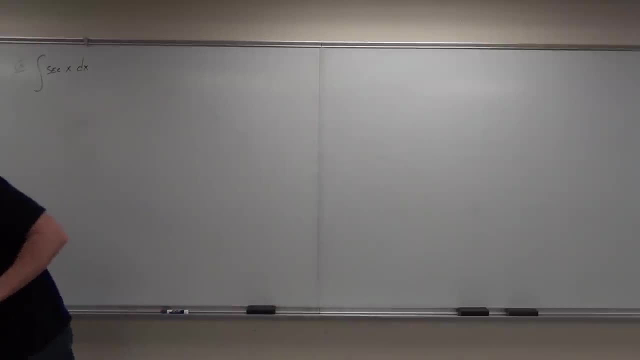 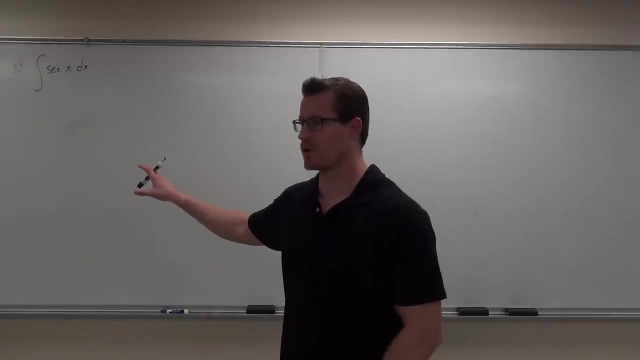 So if I had the integral of secant x, if I had the integral of secant x, that's actually in your integration table, Do you understand? So you look there first. So you wouldn't do anything with this problem except go. okay, this is ln. 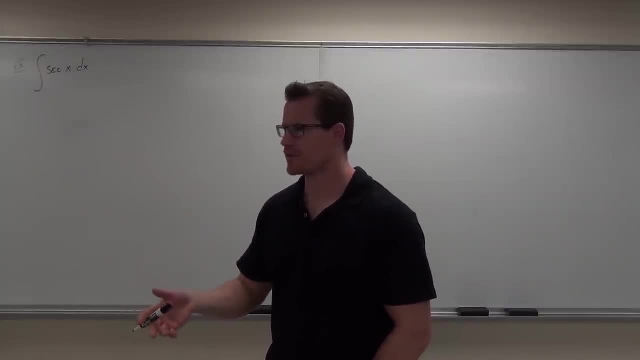 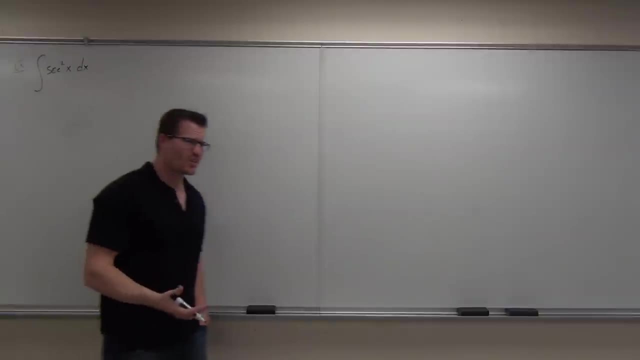 absolute value of secant x plus tangent x plus- I think that's it- plus c. You might want to look that up. That's in your table. If I did this, that's even easier. That's tangent, You're done. 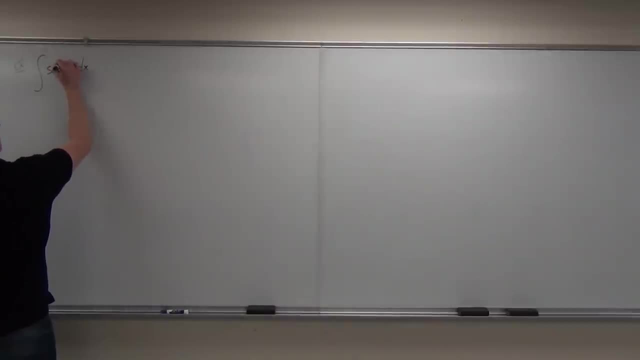 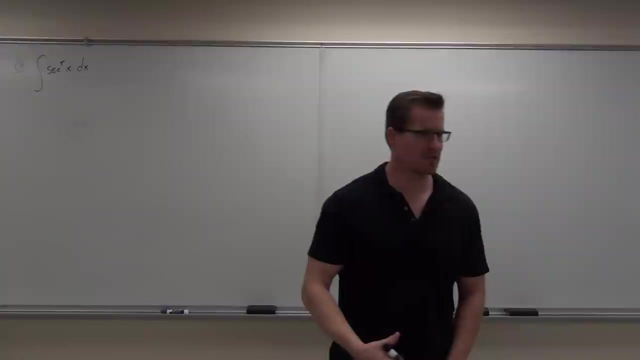 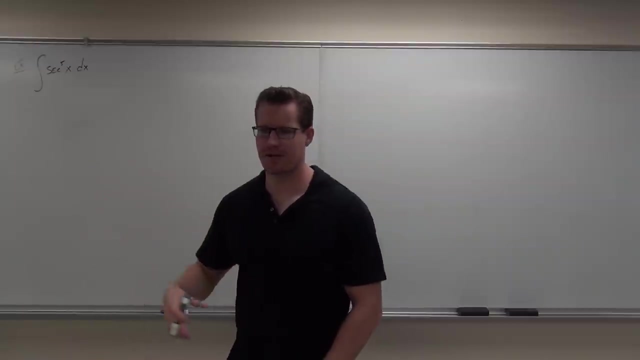 If I did this, we get a problem because that's not in my table. I can't do a substitution because if I pick u equals c, I'm going to get the derivative of secant x, the derivative of secant tangent. That doesn't appear again. so I can't do that. so we're going to have to find out some other way. 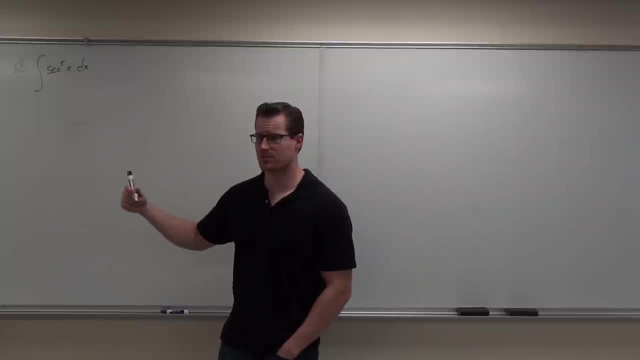 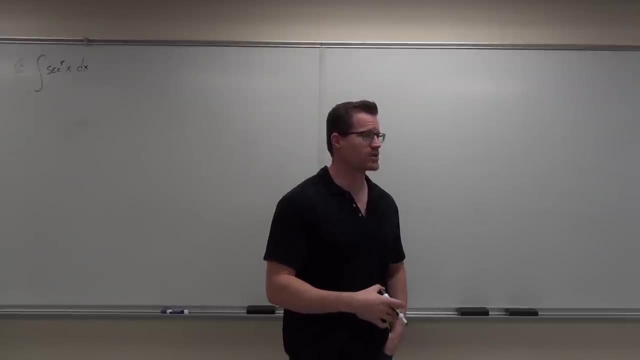 to do these sort of problems secant to the 5th or secant to the 3rd power. I'm going to show you some techniques that we're going to get to a little bit later in section 7.2.. This is kind of like an introduction to some things that we are going to be doing. 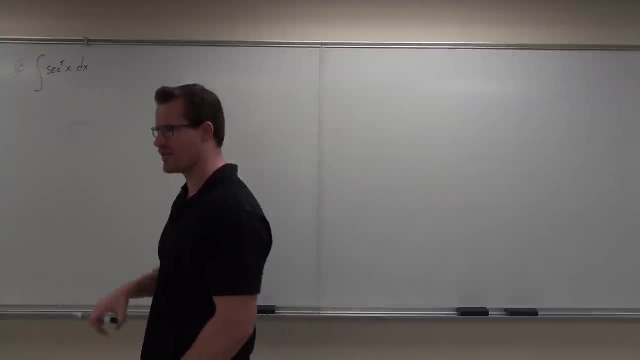 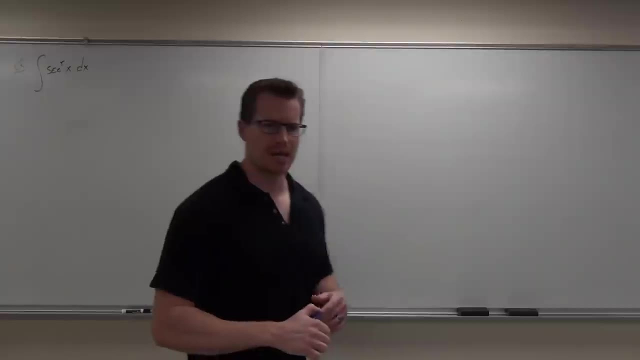 I'll give you some better ideas later, but right now I kind of want to invent something with you. So here's the idea. One idea is: if you don't know the integral right off the bat and you can't use a substitution, integration by parts is kind of defeating you here, because there's really nothing to work with. 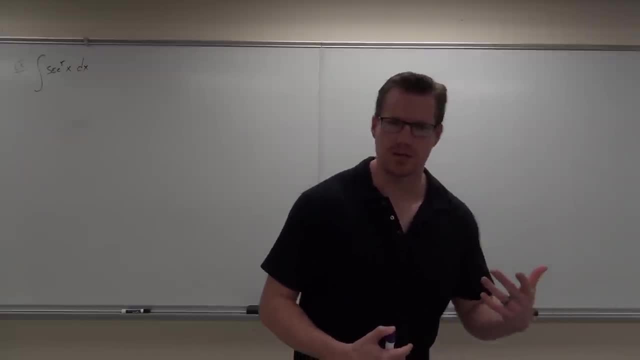 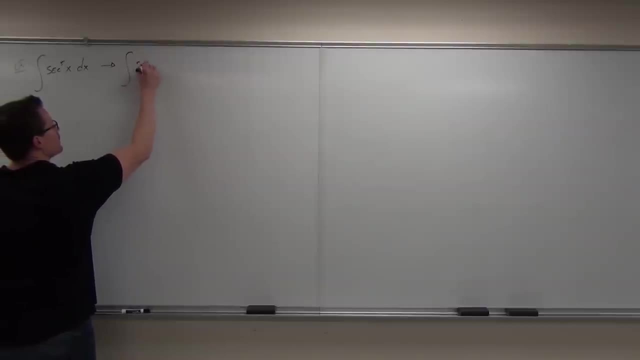 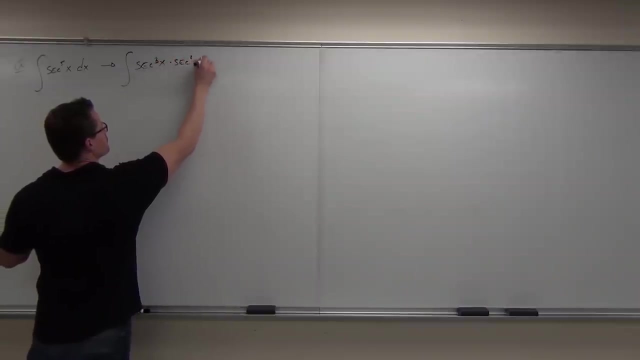 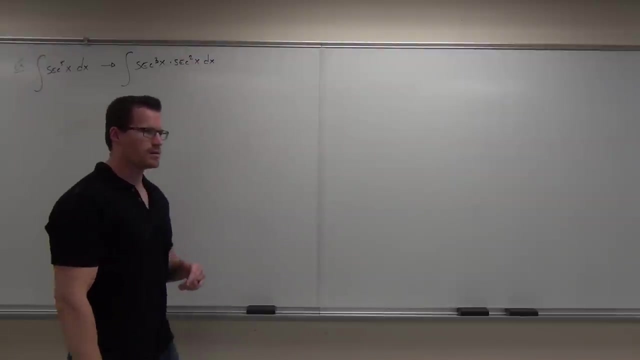 You get back exactly what you have here or make it worse. It's not a good thing. We'll break it up somehow into a part where at least you know how to take the integral of something Like that. Why I'm doing that is: well, I don't know how to take the integral of secant cubed. 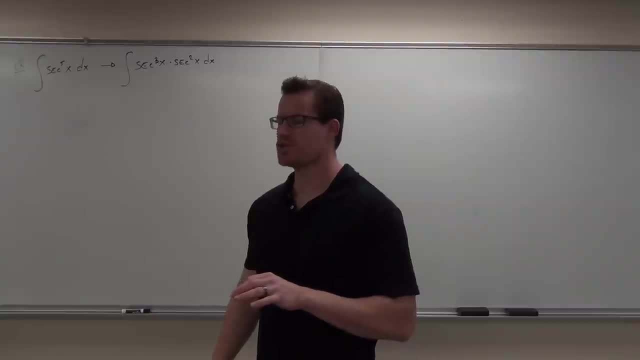 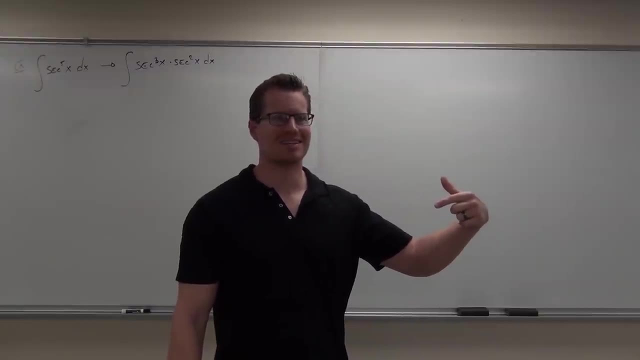 but I do know how to take the integral of secant squared. Does that make sense? What you can't do, you can't break this up as secant times, secant squared, times secant squared and just go: hey, the integral of secant is this times, the integral of secant squared is 10.. 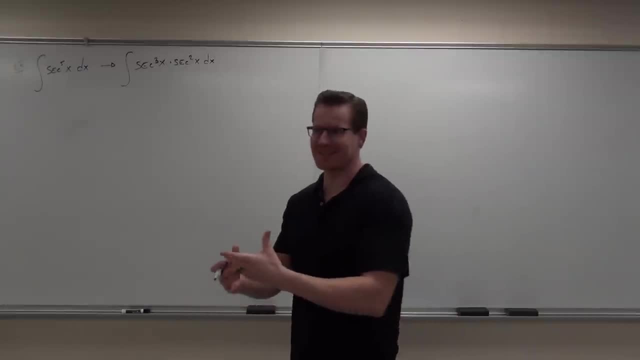 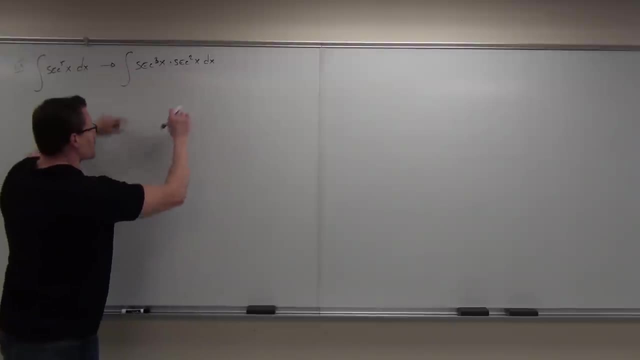 You can't do that, okay, Because that's like a product rule, That's like the whole idea of product means integration by parts. so we can't do that. So only one product, Only one product. Okay, Well, let's start doing this. 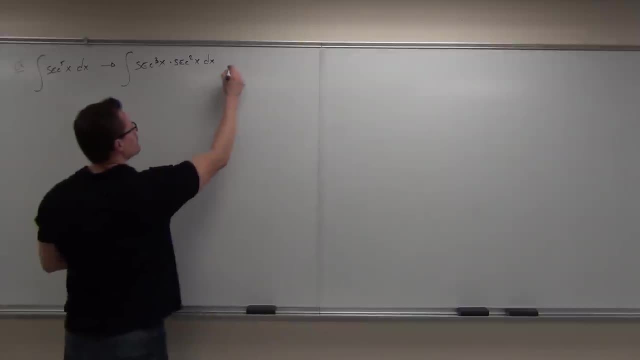 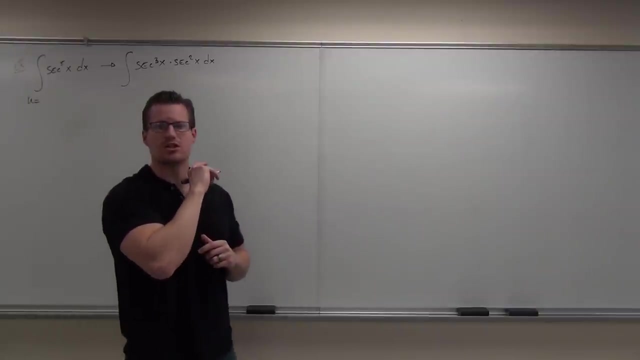 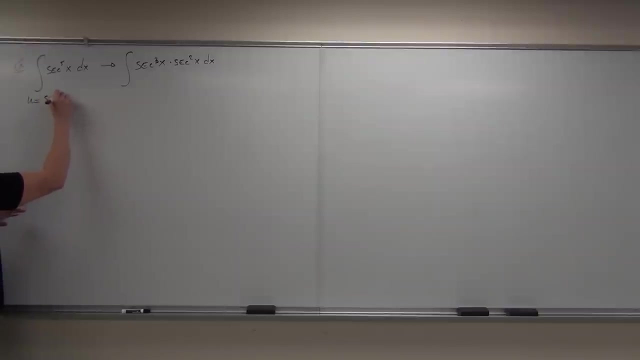 If I do this, I'd probably pick- let's see. let's see what you would pick- Secant cubed, because I don't know how to take the integral of that part. I can take the integral of secant squared, So u equals secant cubed x. Let's do the derivative right now. 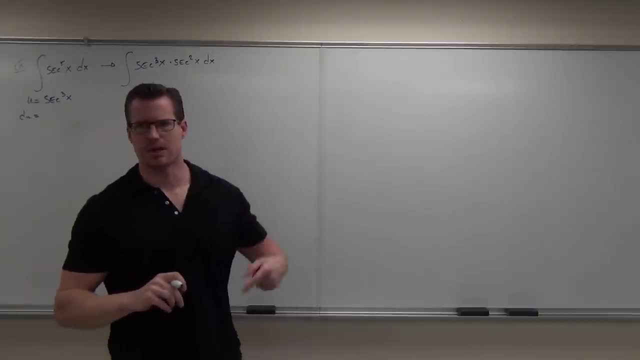 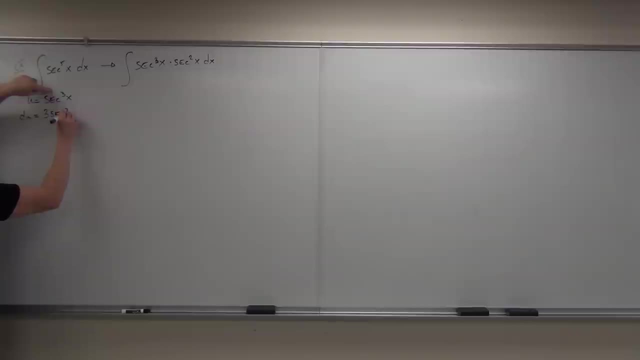 If I do the derivative. I'm going to do the derivatives quick right now because I'm expecting that you guys can do this all the time. okay, The derivative of secant cubed would be 3.. Secant squared x times secant x, tangent x. 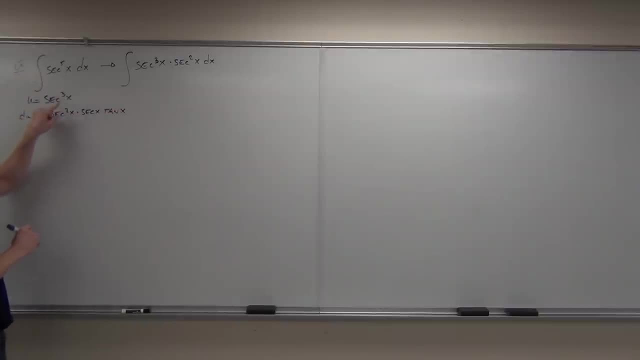 Do you follow that by the chain? rule 3 comes down, becomes a 2, leave the inside alone. Derivative of the inside is secant squared. secant x, tangent x. You guys? okay with that one? Okay, If not, go back and refresh your memory on how to do integral of secant cubed on your own. 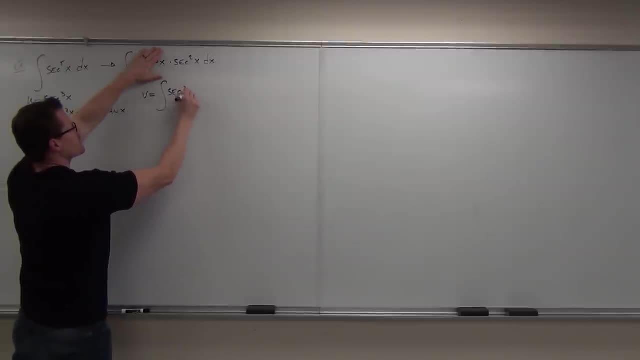 V would be the integral of secant squared. x, dx. This is nice. I broke it up into something I can actually take: the integral of Integral of everybody. What's the integral of secant squared? Can you guys do that? Okay, We're starting. 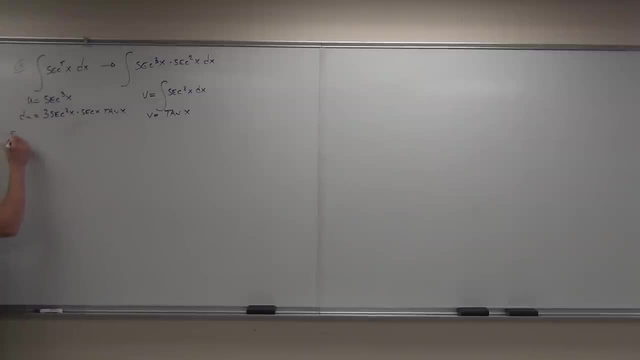 So our first part here is: we know this integral is u times v minus the integral of v du. I've got my dx again: V du, V du. Let's clean this up just a little bit. Instead of secant squared, what am I going to put? 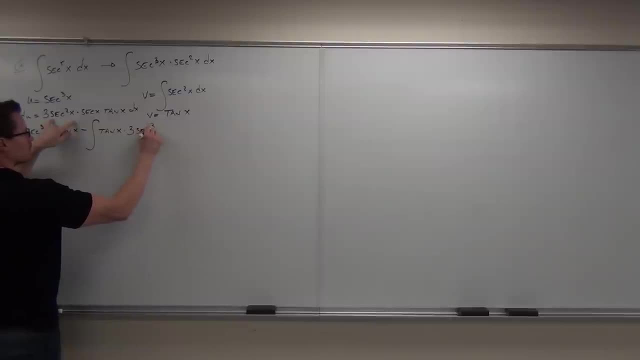 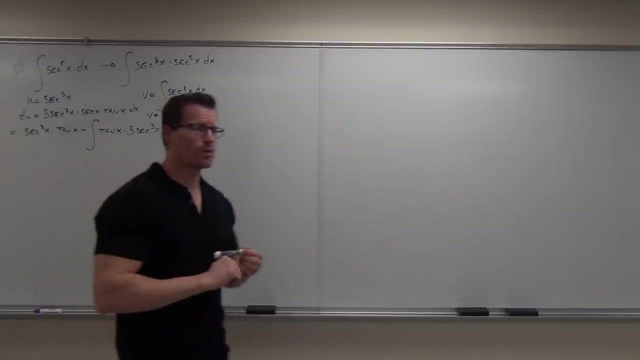 Secant, cubed, Secant. We have lots of writing going on, so I want to make sure you guys are okay on every single step. Are you okay getting secant cubed x times, tangent, x, U times v, Yes or no? 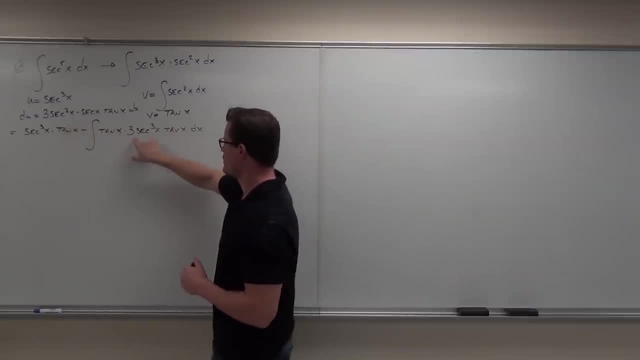 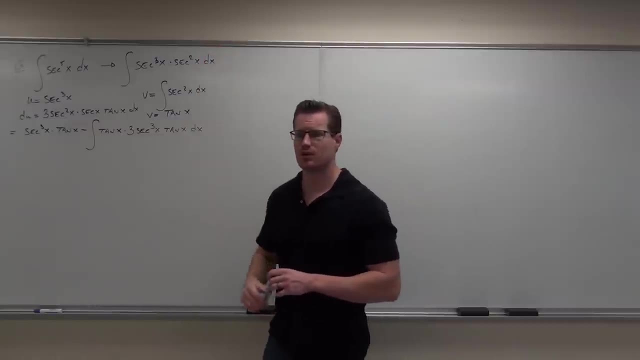 Minus integral of v tan x. This is du. It's 3 secant cubed tan x. and then our dx. You guys feel okay with that one? Okay, Let's clean it up just a little bit. What are we going to do here? you know. 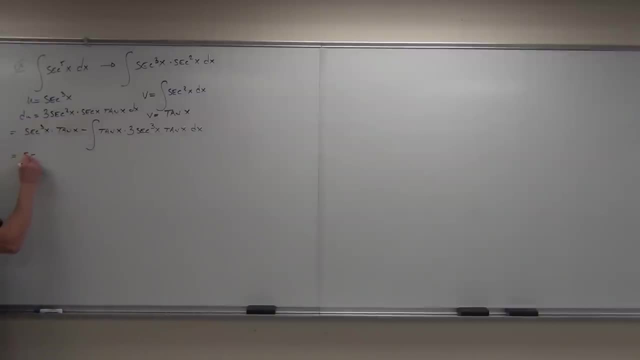 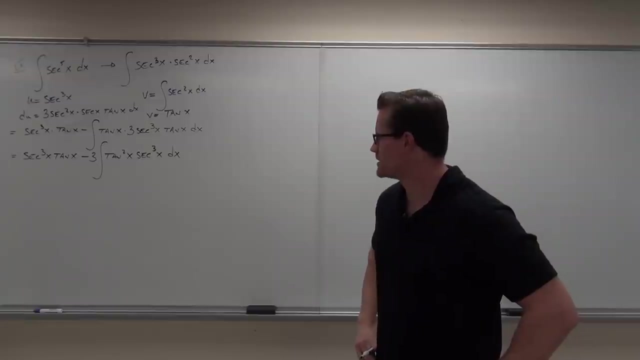 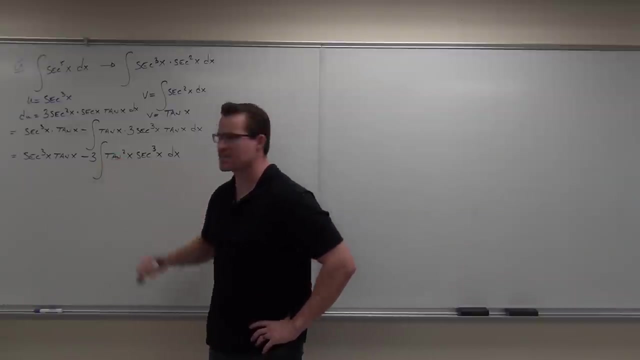 Okay, Three out. What else? Tangent, squared So minus 3. integral of tan. squared x, secant, cubed x dx. Okay, This is fun now. Well, this is fun. What do we do here When you have something like a tangent and a secant? what you're going to see? 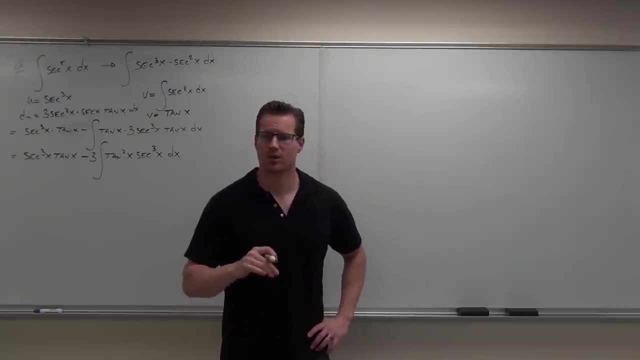 in the next section. that we do is oftentimes we're going to be using identity to change one into the other. For instance, I don't want tangent x and secant x because even if I did integration by parts of that, it's going to be really hard to do. 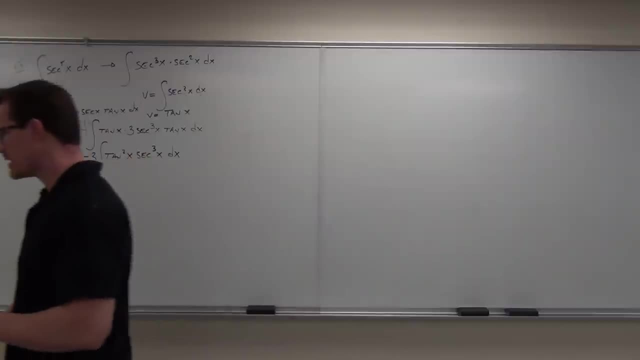 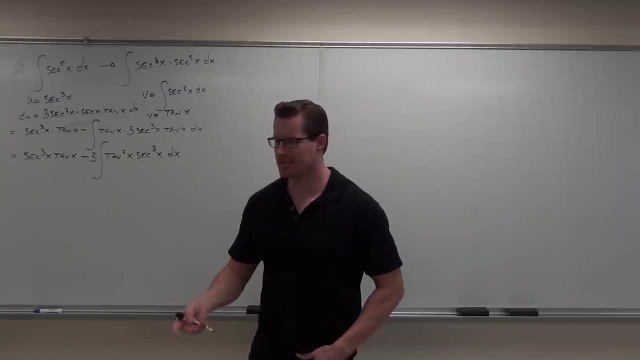 So let's make it easier, or maybe even impossible to do. Let's make it easier, Instead of having tan squared x, we're going to use an identity for that. What you need to know is: you need to know your identities. Have them written down. 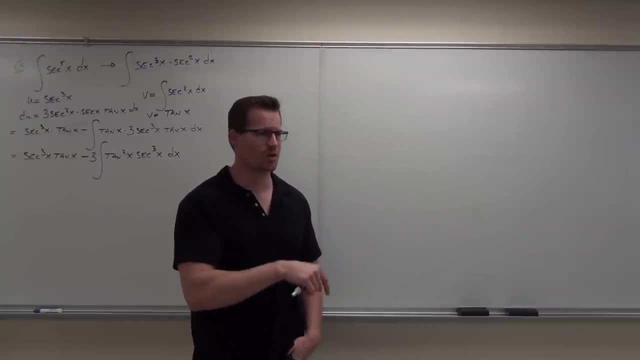 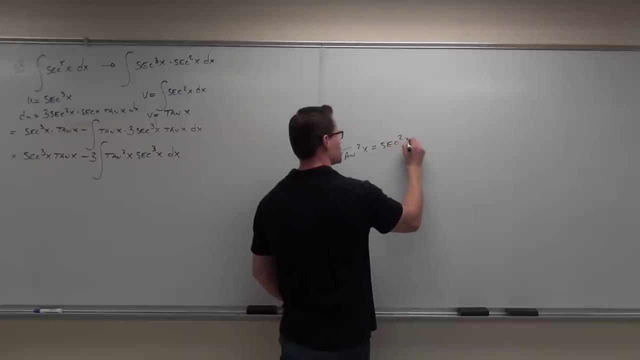 Tan squared x is the same thing as secant squared x minus 1.. Did you know that This is true? So tan squared x is secant squared x minus 1.. Let's use it, because now we can change our tan squared into a secant. 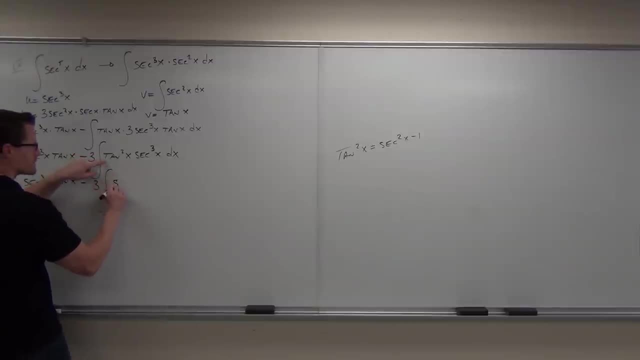 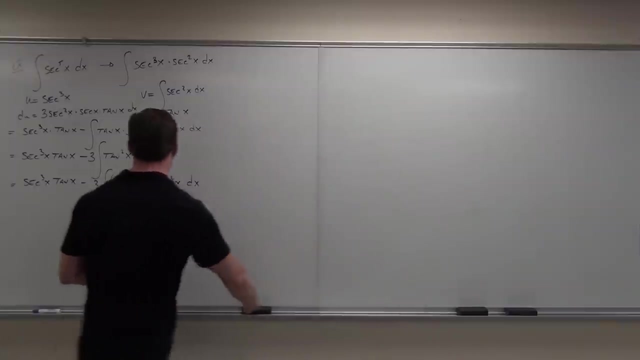 So instead of our tan squared x, we have secant squared x minus 1, and then secant cubed x dx. So true, that's an identity, Use it. Oh wait a second. This is kind of neat. You're going to see something we just dealt with actually. 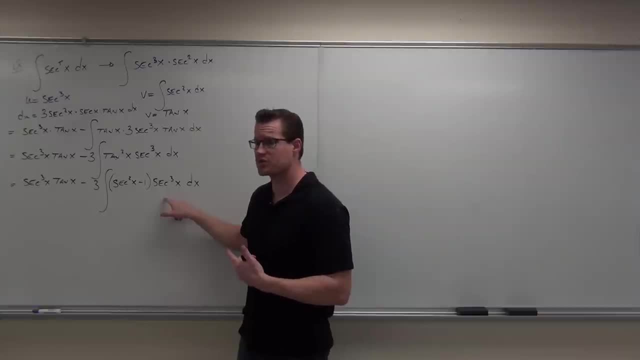 What should I do here? Distribute it? Yeah, I'm going to distribute that, because right now substitution isn't going to work, because if I try This one, I don't get exactly this thing back again. Does that make sense? I'd have a secant tangent again. 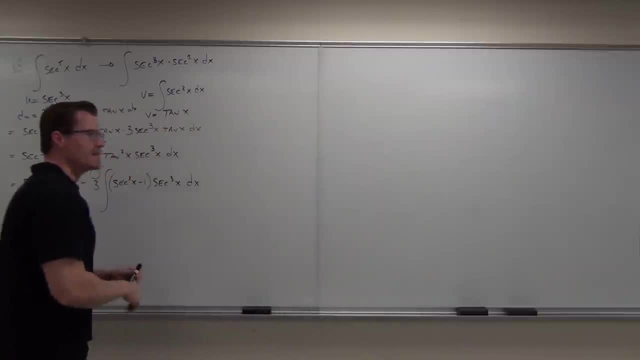 That would be a big problem. I don't want to do that, So let's distribute, And this is the same process that I'm going to teach you in the next section. You're going to do this a lot, So let's distribute this guy. 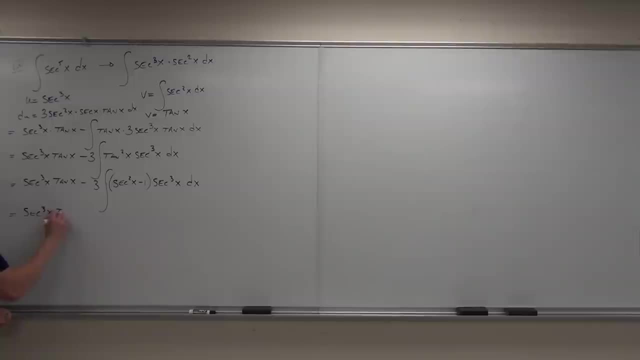 Well, that becomes secant cubed x, tan x minus 3 integral of. Tell me what I get for my integral. Secant to the fifth power of x Minus secant cubed x, dx. Okay, I really do need a show of hands if you are okay with that so far. 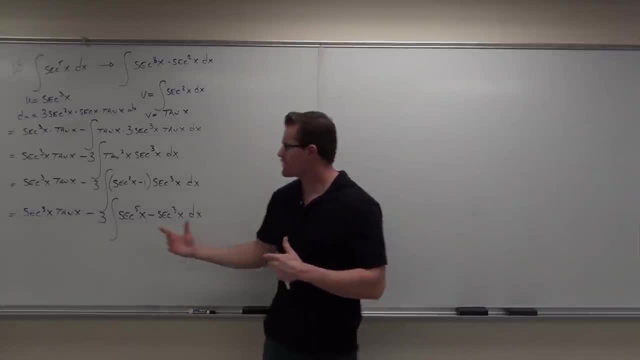 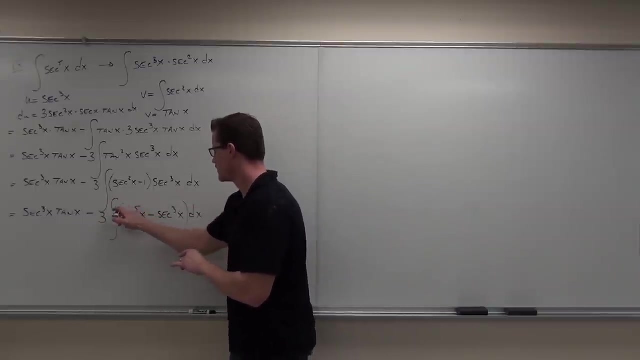 Are we all Cool? What can you do? every time you have integral and subtraction, What can you do? Separate it. Let's separate it Now. watch what we're going to do. Make sure that when you separate this, this minus 3 goes to this whole entire integral. 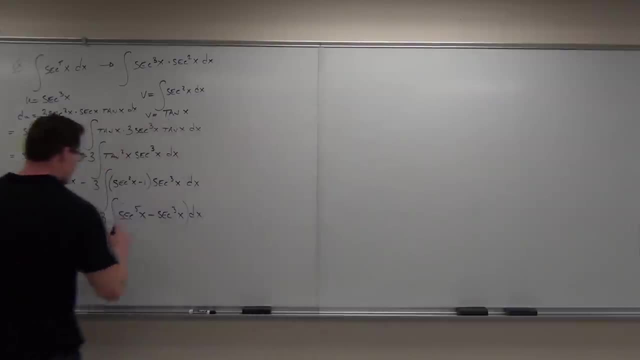 Does that make sense? Yeah, So when we do this, This really should have a bracket here. What we'll get is secant cubed x, tan x minus 3 integral secant to the fifth power, x. Hopefully you're with me on this one. 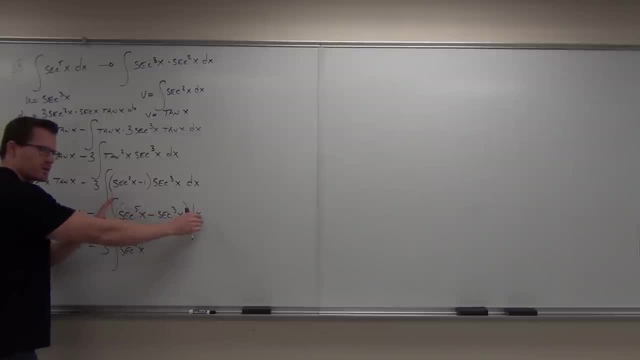 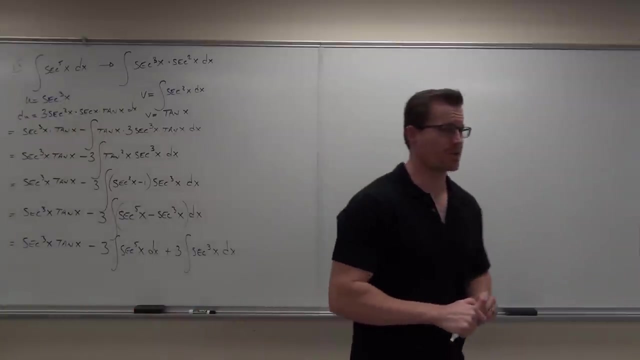 So let me have your eyes on the board here. This would separate into two integrals, correct. It would be minus integral secant cubed. This will make it plus 3 integral secant cubed x. So it's noble, that's equal to mod 2 treat, indeed dx. I want to make sure you're okay with the algebra. it's just algebra right now, but are you okay with it? Yeah, Everybody show of hands if you are. are you okay with Now? is there something good about what we just did? 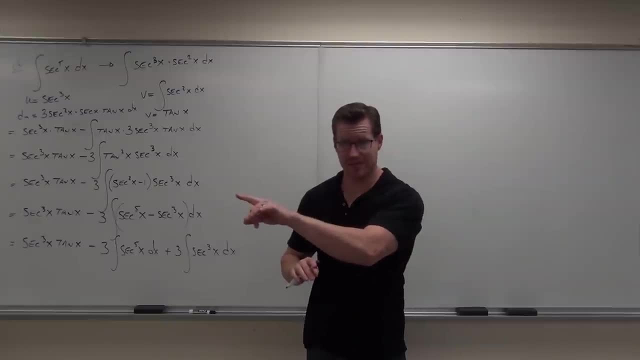 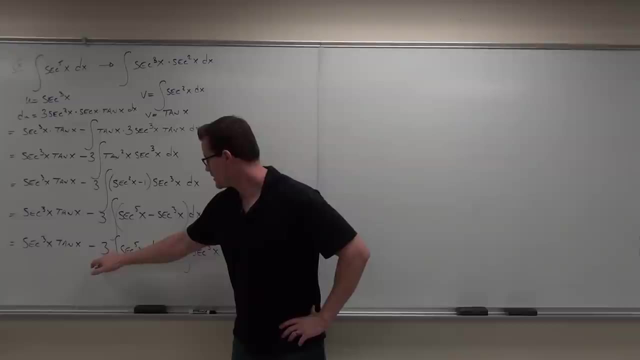 Do you see it? Can you use a track? Say something good about it. what do we have good about it? Give it a compliment. What do we have good about this thing? We got the same thing. Well, can you subtract one of the integrals from the other? 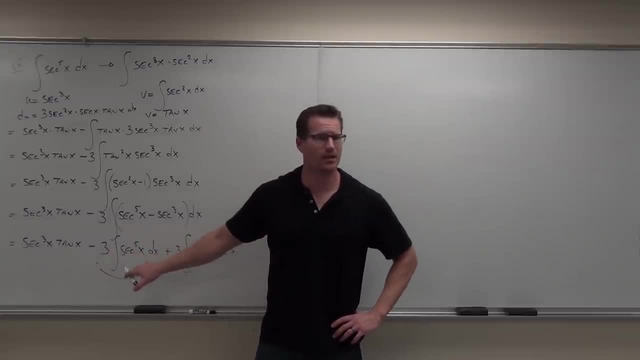 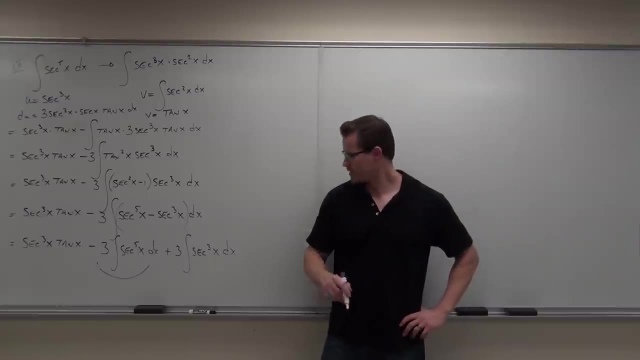 This one. this is great. That's great right now. Why is that great? That's this, That's fantastic, And we're gonna use that in a minute. Tell me something really bad about this: That still has an integral. So, no matter what, we're gonna have to deal with this one. 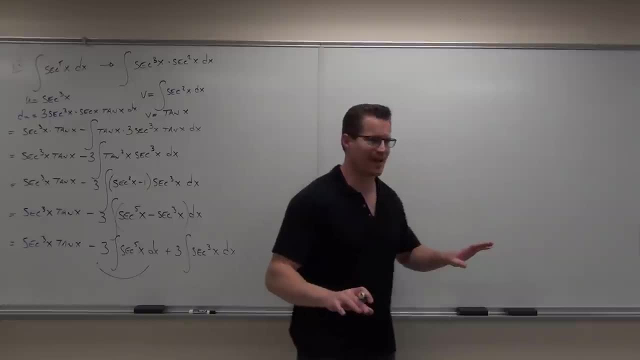 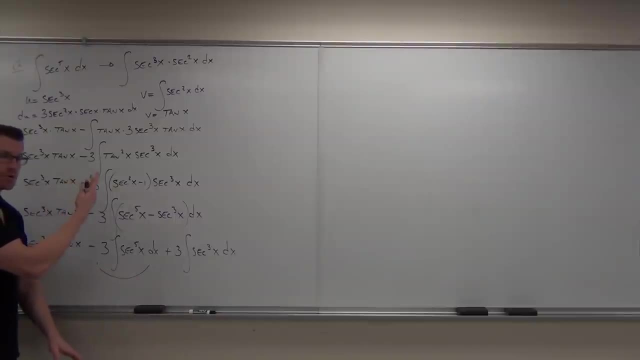 Does that make sense? So what I'm gonna do- this is why this problem's nasty Right now. this would be awesome if there was no integral. If this wasn't here, you would just add that to both sides, You divide by four, and then you're done. 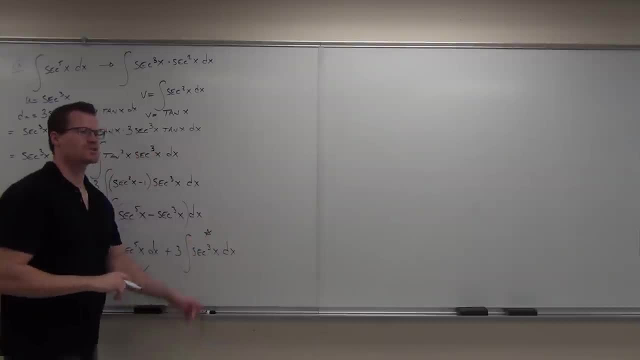 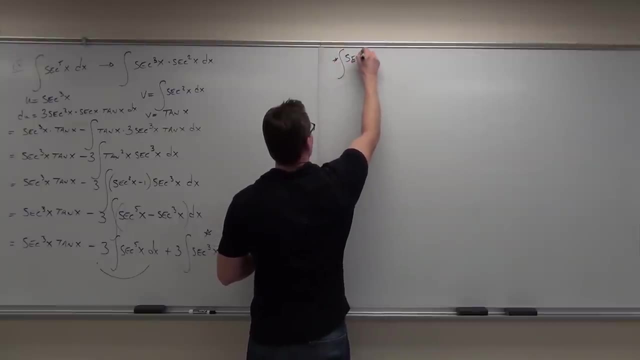 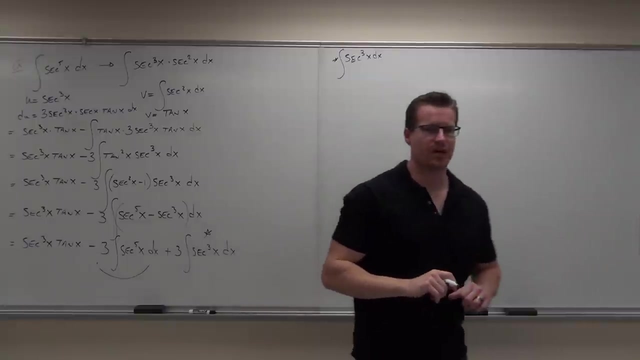 Does that make sense? This, I'm gonna give us a little asterisk. We're gonna have to do this one off to the side Now. integral secant cubed x dx. Do you understand that? that's really similar to this idea. 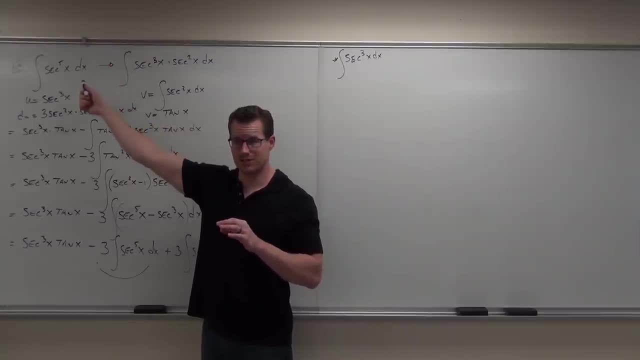 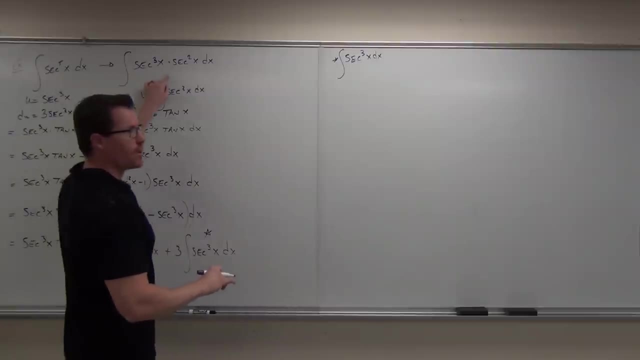 Can I strip off a secant squared Sure? If I can do that, then I'm gonna do the same exact thing I just did, So I'm gonna do this kind of quickly here. but you need to understand, it's the exact same idea, only in this case I'm not gonna have secant cubed. 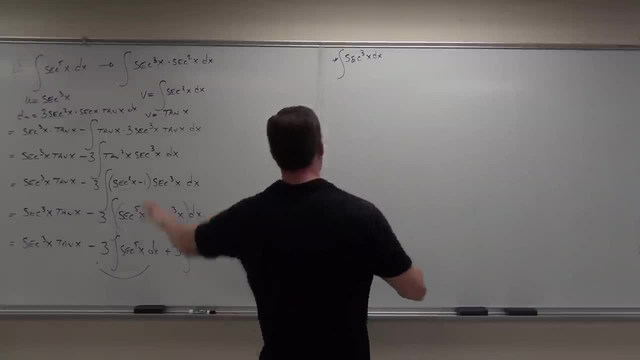 I'll just have secant. That means we won't have to do this process again. We'll get down to here and be able to add our integrals. So we're gonna do this idea twice. You're gonna need a lot of practice right now. 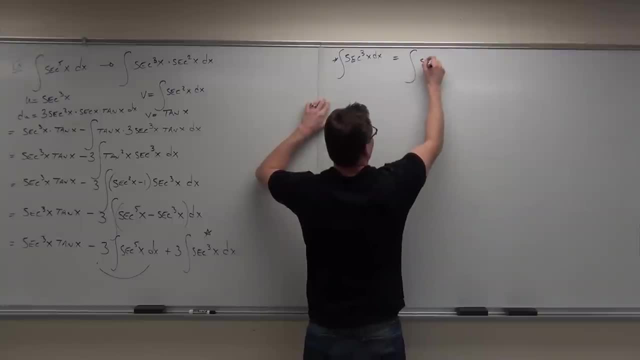 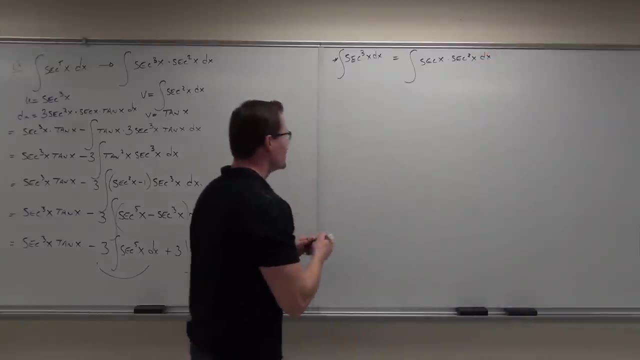 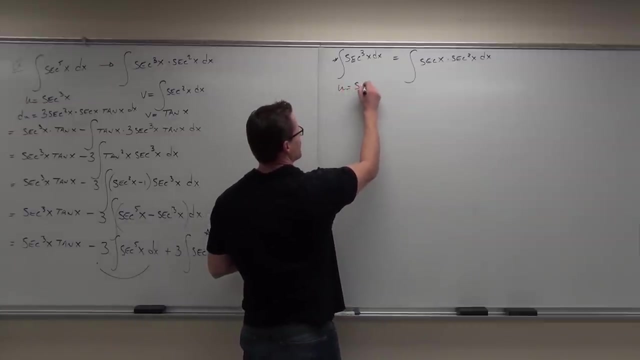 So this becomes integral of secant x times secant squared x- dx. Same thing, Same thing, Same exact idea. Strip off something that you know the integral for, Well, then u equals secant x, The derivative is secant x, tangent x- dx. 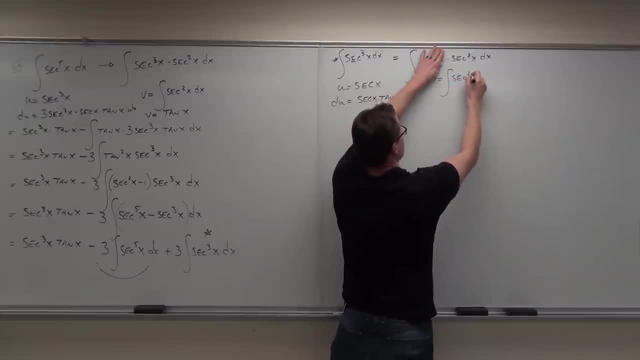 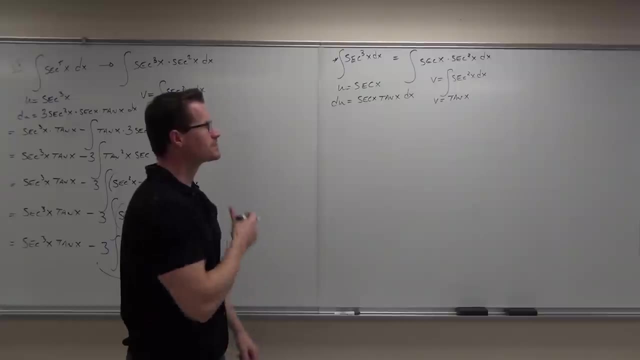 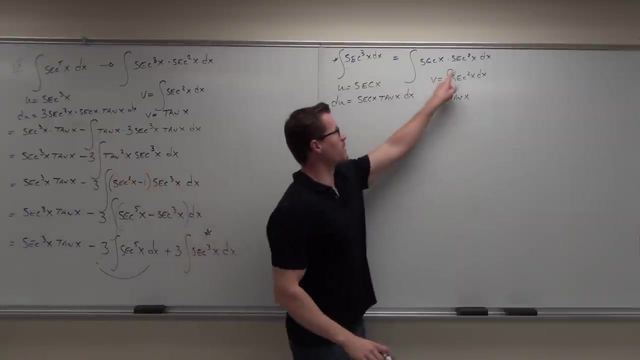 v would be the integral of the rest. secant squared, x, dx, And our v is tan x again. You guys, OK with that one. Do you see the same technique at work that we just did? Strip off the secant squared, Call that your v, integral, your v, No problem. 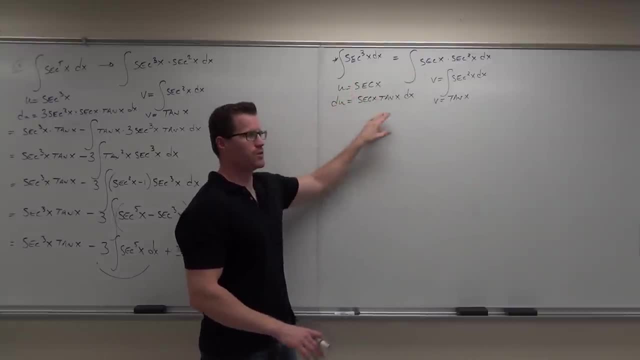 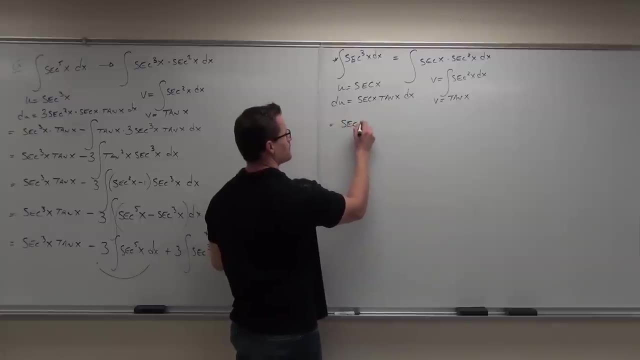 That's easy, This one. call that your u derivative of u. You can all do that. That's secant x, tangent x. Now if we do our integral, that's gonna be u times v minus the integral of v du. 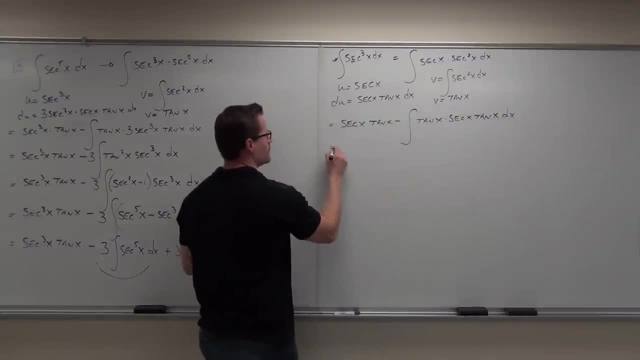 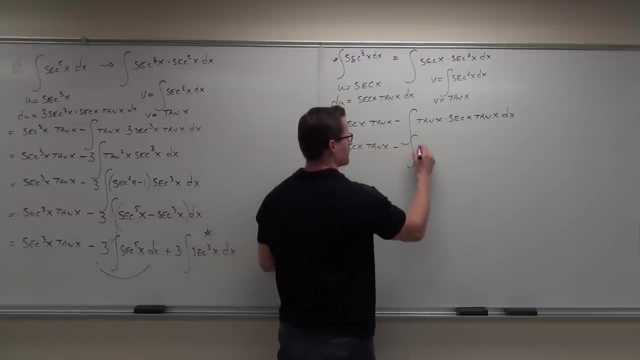 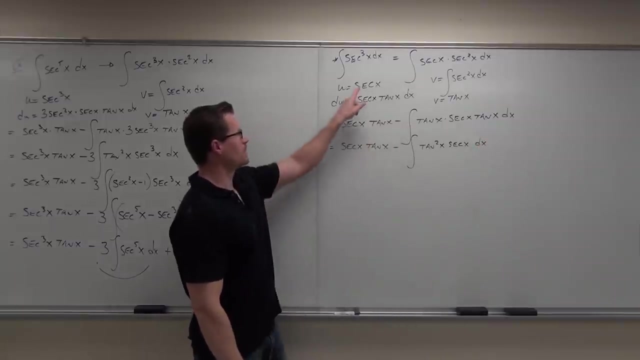 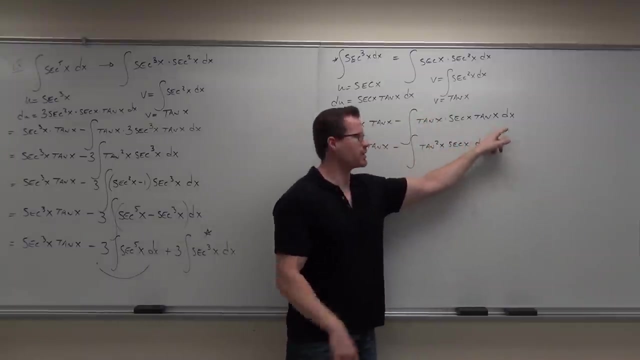 We'll clean it up a little bit. So u times v. got it Minus integral of v. hey, no problem, du. OK, it looks kind of nasty, but we can deal with it. Got that same thing. We'll simplify it a little bit. 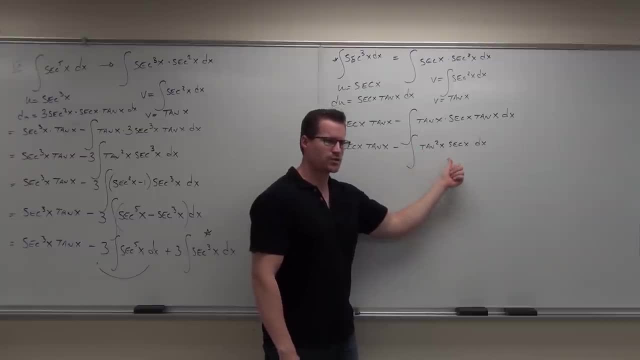 Tan, tan, tan squared. All right. Now this looks a whole lot like that one Very, very similar On. instead of secant to the third, I had secant to the first. I'm gonna use the same identity again. 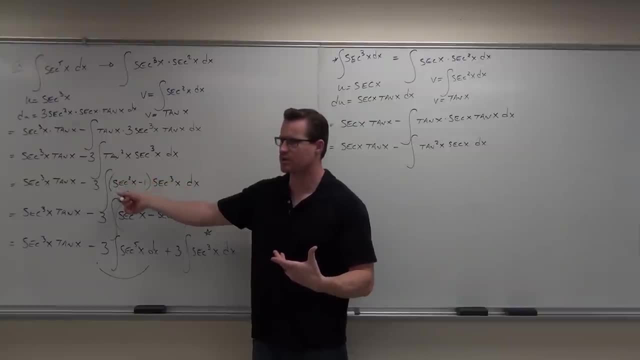 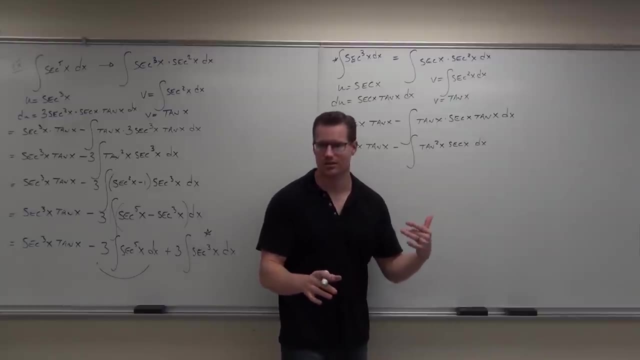 So instead of tan squared, I'm gonna write that as secant squared minus 1.. You guys still with me? Yeah, Are you sure? I don't want to blow you out of the water here? A lot of algebra, a lot of trig here. 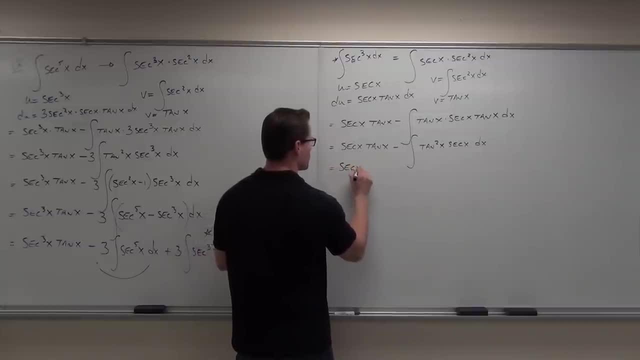 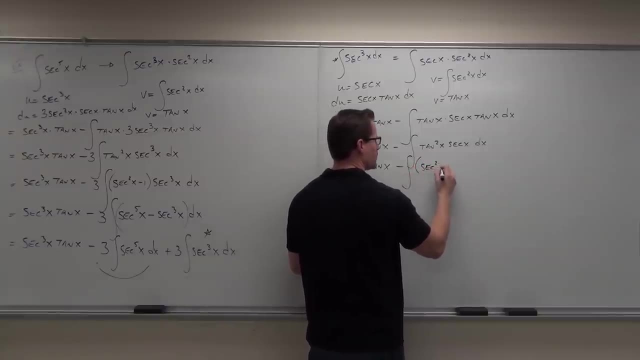 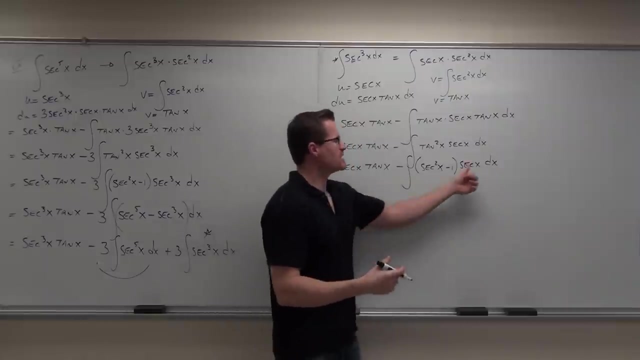 A lot of algebra, a lot of trig. So secant x, tan x, All right. All right, Minus the integral of: yeah, let's call that secant squared x minus 1 times secant x. Do the same idea again. 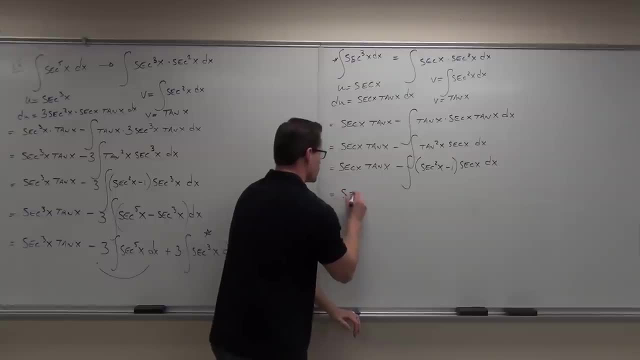 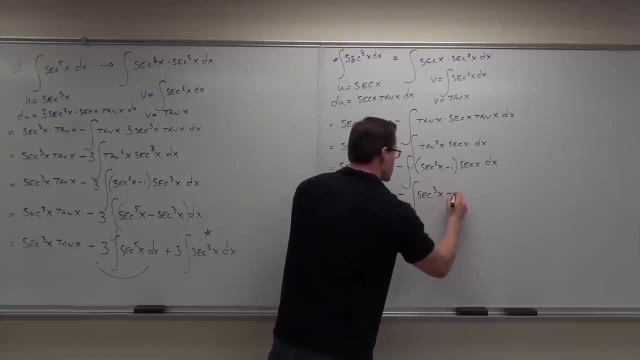 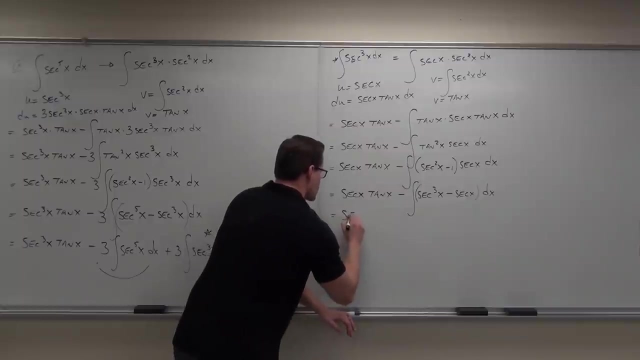 Distribute it again, That'll be secant cubed x minus secant x dx. Do the same thing here That we just did here. Let's split off our integrals again. Well, if we do that, then we got secant x minus. sorry, not minus. 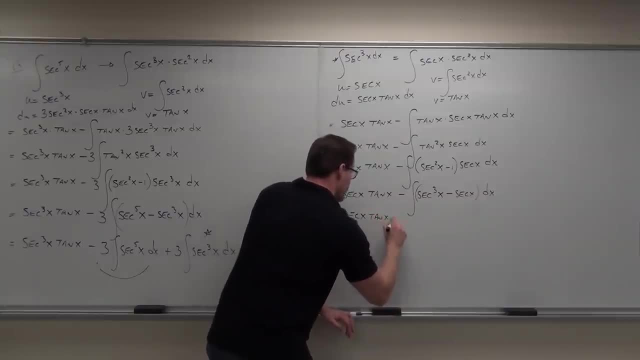 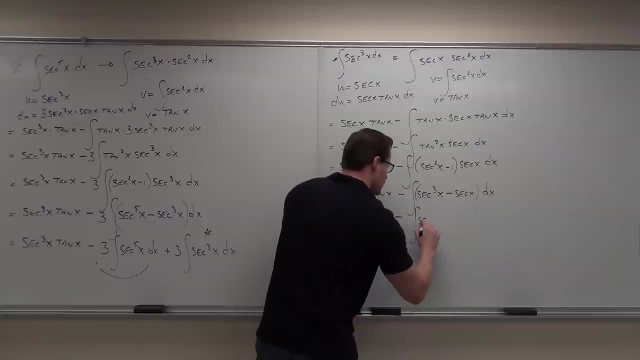 Secant x, tan x, Minus. tell me what I'm gonna have here. What's the next thing? Secant cubed x, dx. Okay, Tell me what the next sign's gonna be. Is it gonna be plus or minus? 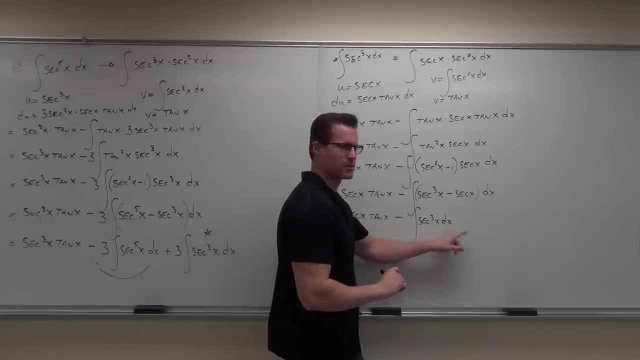 Minus. Do you guys all see why it's gonna be plus? Oh, it's gonna be minus 1.. Remember, we're separating this. This will be integral, minus integral, but it's in brackets, So this minus will distribute. 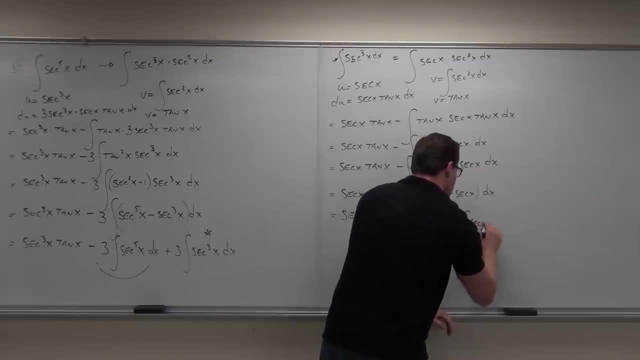 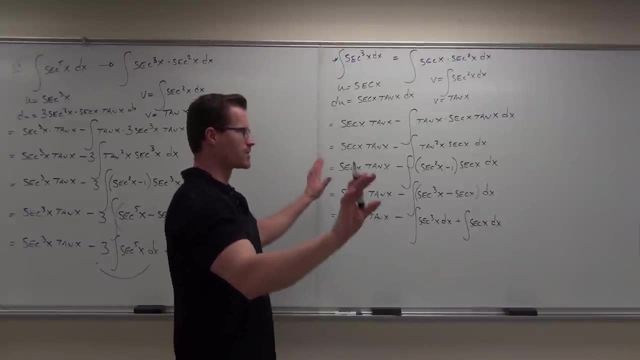 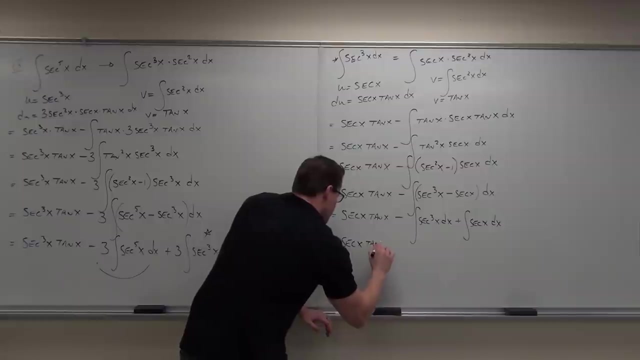 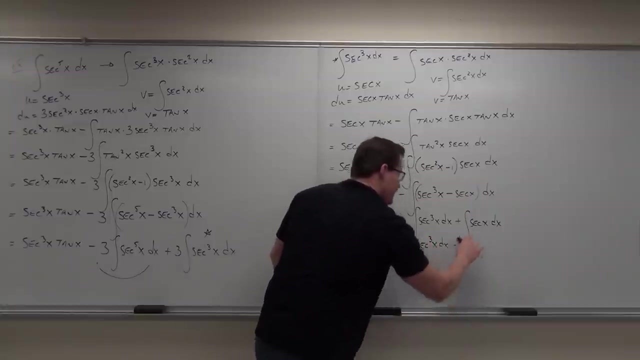 It'll become plus integral. secant x, dx. Oh goodness, Almost there. Let's see, We got secant x, tan x. We got minus Integral of nasty thing we can't get rid of. Now this one, we can actually do that. 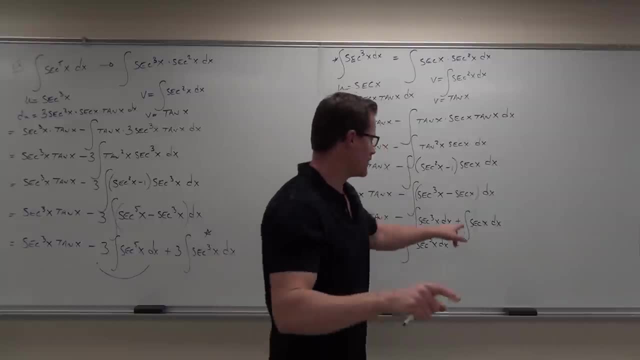 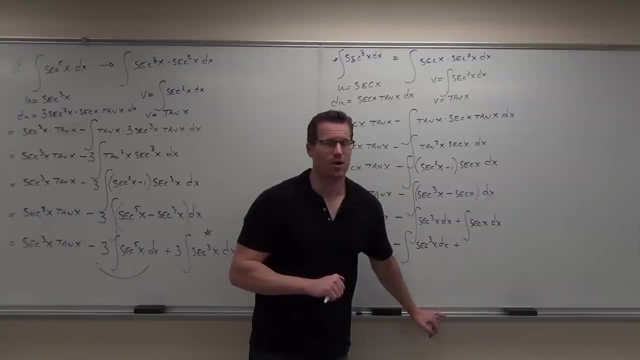 Look back in your notes if you have to. I think I gave it away earlier. but the integral of secant x. Do you know what the integral of secant x is? Natural log of secant x plus tan of x dx. Yes, you're almost right. 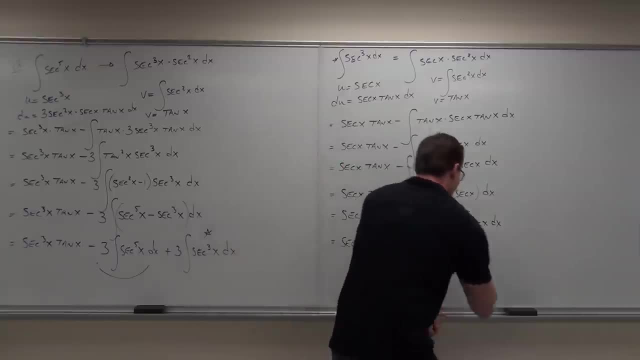 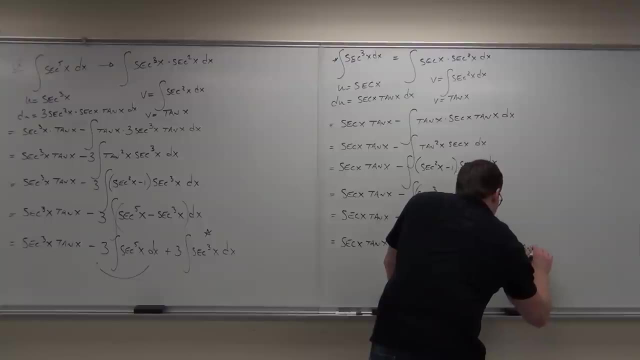 There's one little word you forgot: Absolute power. So the natural log of the absolute power of secant, of x plus tan, of x plus secant. Can you do it? I'm going to refrain from putting the plus c, But yeah, you're right. 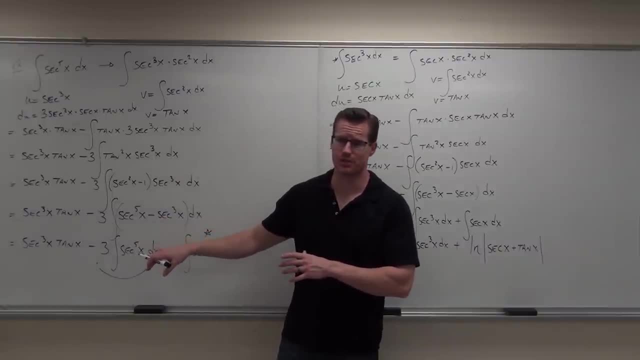 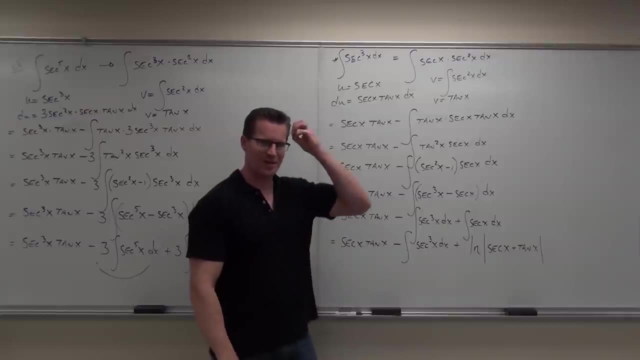 I'm going to refrain from the plus c until I'm completely done with my integral. I don't want that thing hanging around because it's really confusing You guys. OK with that one. Yeah, You sure Have I blown your minds to that yet? 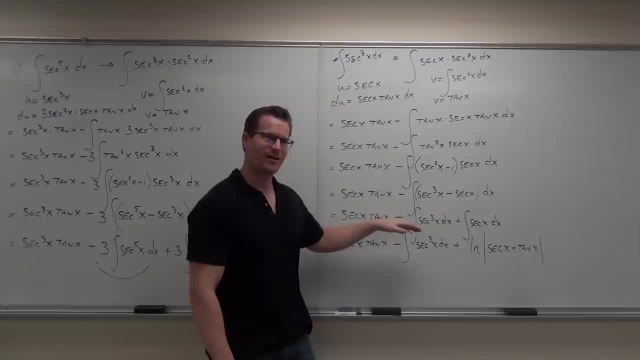 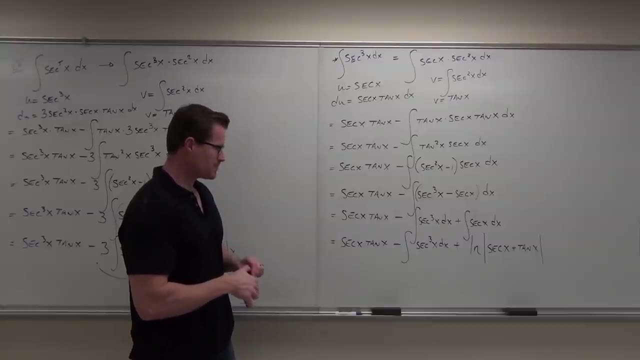 Yeah, What the heck. This is crazy right, We're about 75% of the way done. We're almost done, Almost. Here's what we got. We did basically a problem within a problem. that was just a problem. We did a problem within a problem. that was just almost as hard. 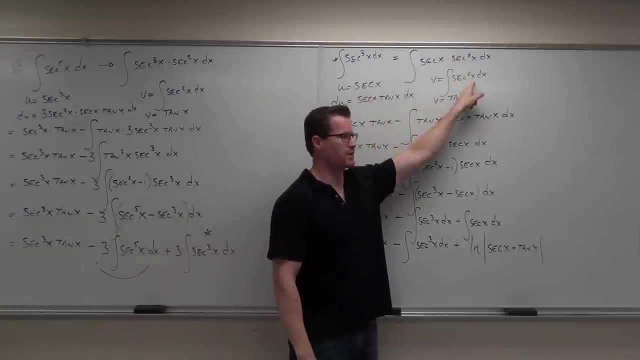 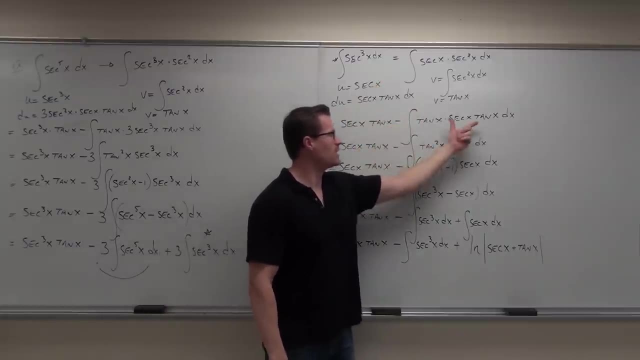 Same exact idea, though: Break off the secant squared, Make that your v, because you can do the integral of that. The problem is tan x. You got u times v minus integral of well vdu, Clean it up Tan squared. 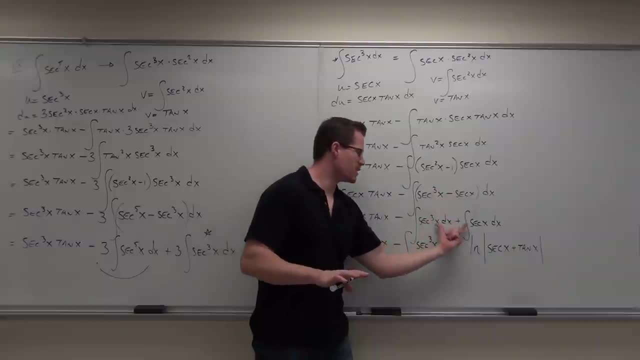 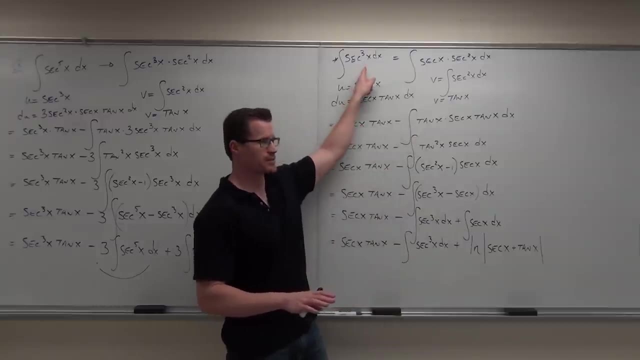 No, no, no. Secant squared minus 1. Distribute, Split it up again. This stays the same. Why do I want that to stay the same? Because it's this, It's this right here. OK, Got to get rid of this in a second. 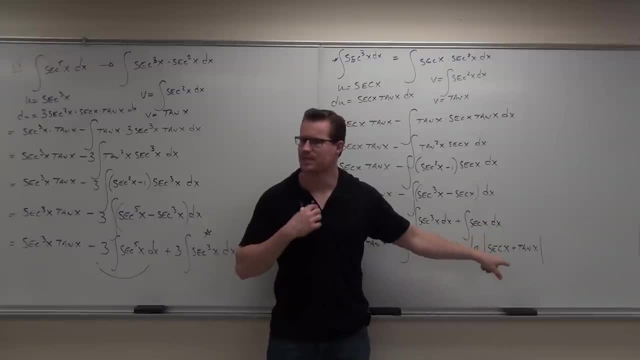 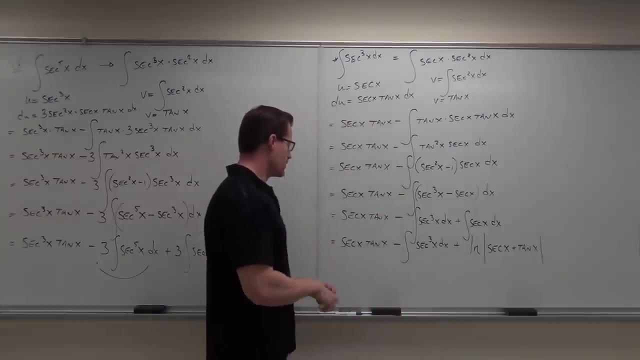 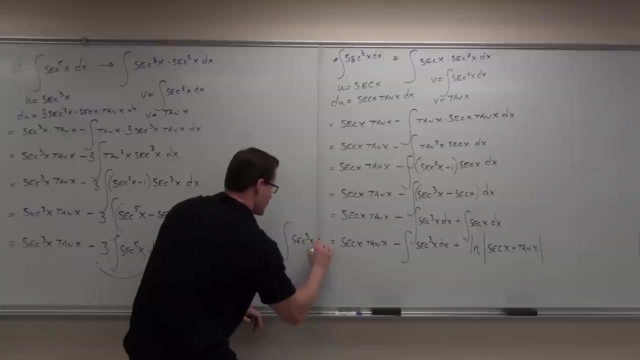 This one. I wanted that because I know the integral That's in my integration table now. That's why we did that in the last chapter. You guys, OK with this so far? Yes, No, Yes, Yes, All right Now, keep in mind, it was this. that's equal to this. 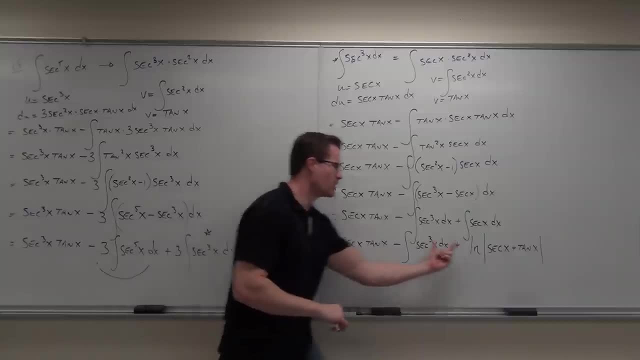 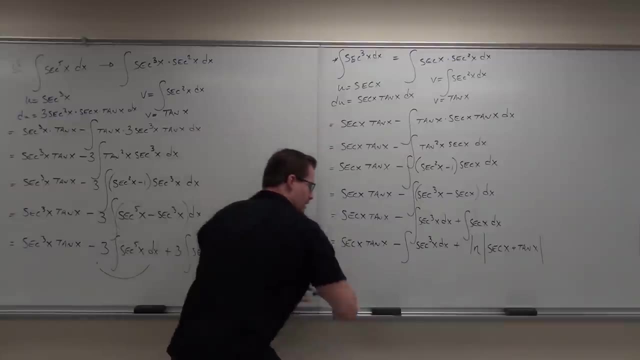 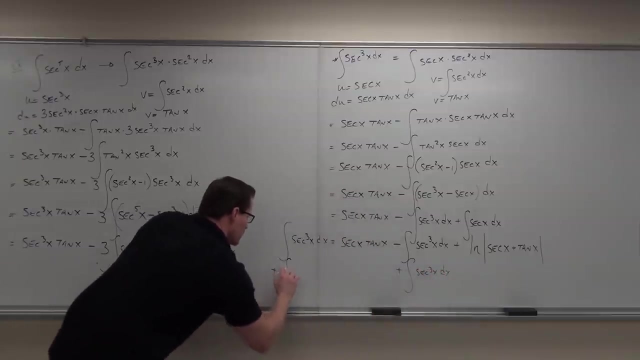 Tell me what I'm going to do next. Notice: no integral, No integral Integral. What am I going to do? Add the integral to the other side. So if I add that, treat this like an equation. Add this integral to both sides. 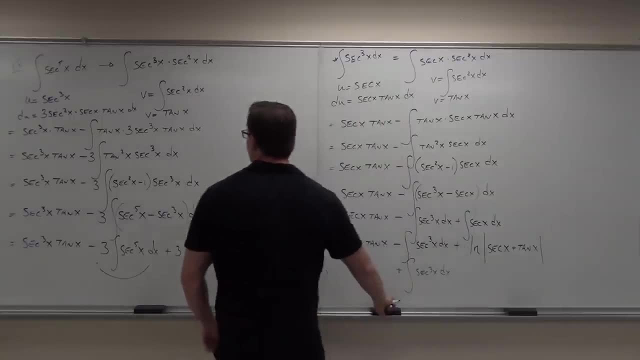 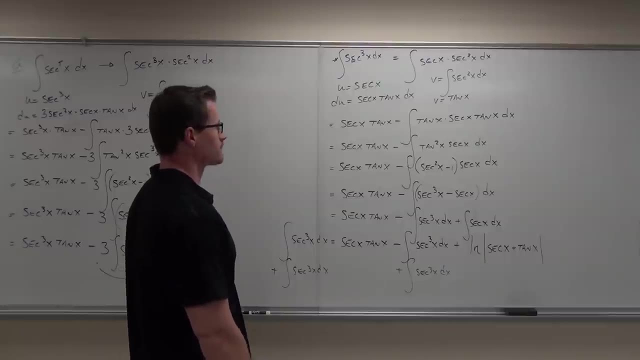 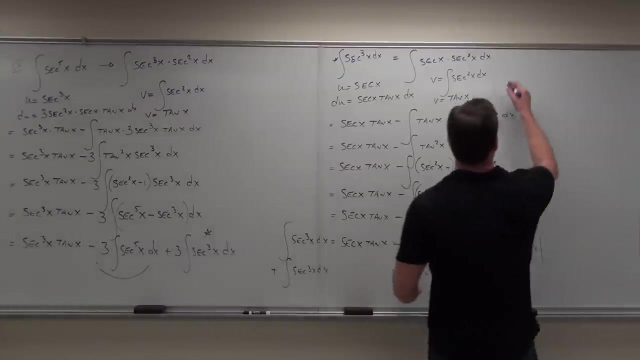 If we do, if we add that, let's see What do you want me to erase? It's going to have to be something The left, I can't see the right. OK, You know what? I think I can write it over here too. 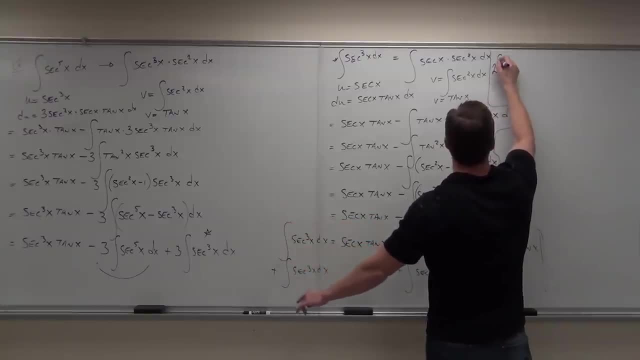 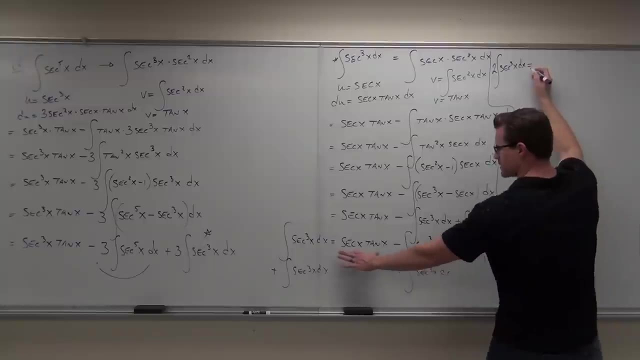 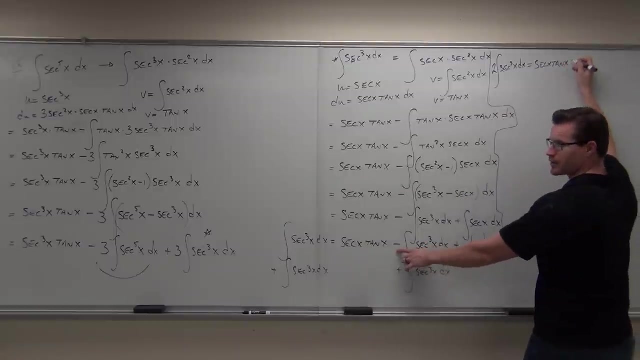 How much is this going to be? Well, 2 integral secant q. How much that's going to equal? is this thing? Is this still here? No, Got rid of it. Is this still here? Yeah, And we're almost done. 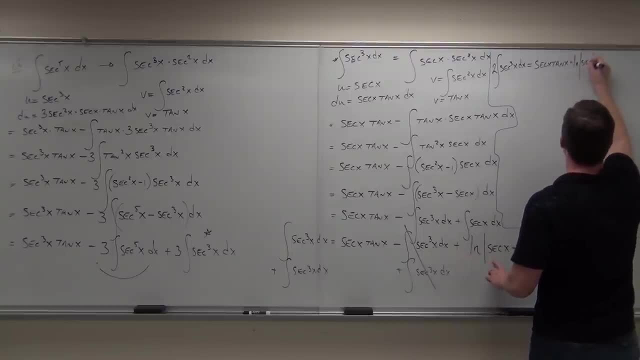 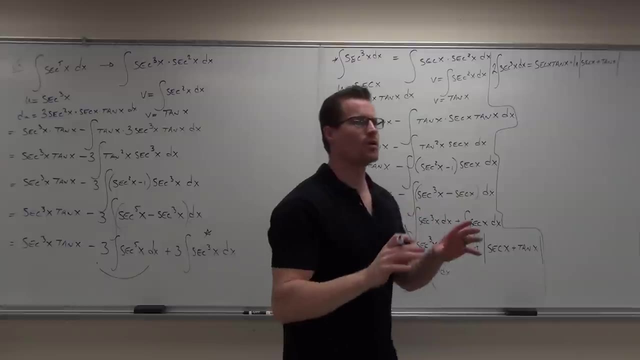 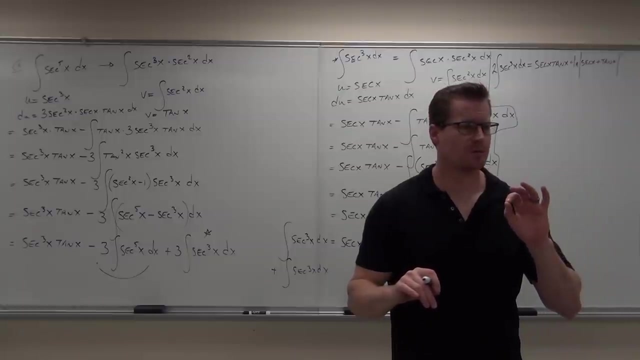 Just stick with it right now. What do we know? Why do we need to divide by 2?? Is that 2 what I want? I want this without the 2.. So, yeah, divide by 2.. Yeah, Without the 2.. 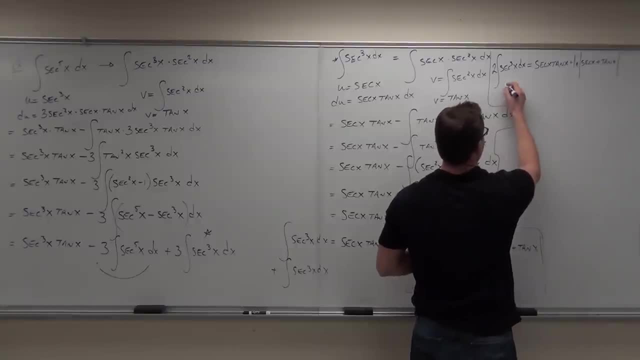 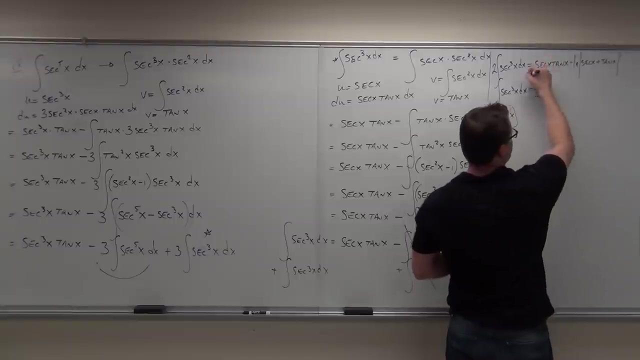 So, yeah, divide by 2.. So we're going to get secant cubed x. dx equals 1 half. You can do a bracket around the whole thing. You can do 1 half. You can do 1 half for each of them. 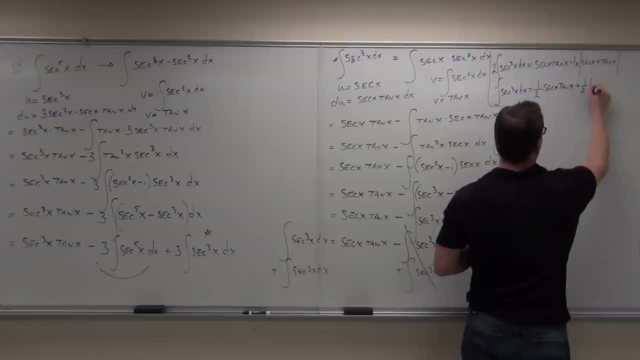 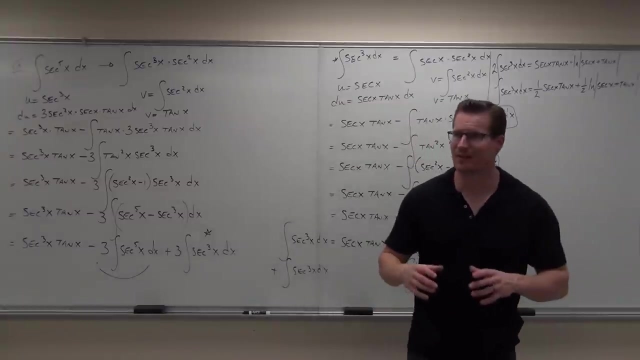 Secant x, tan x plus 1 half ln. absolute value. Secant x plus tan x and absolute value. That would be crazy if my absolute value was. I know maybe your brains are hurting a little bit. What I want to know is: are you OK on just this piece right now? 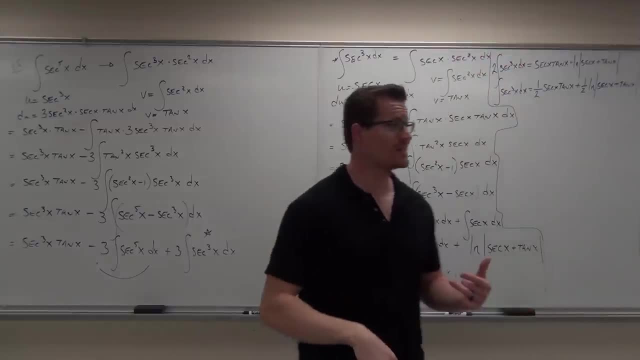 Show of hands, if you are OK. Do you see how it's very similar to the first example we did today? Yeah, Really similar. You get down to one part you can't get rid of. Hey, it matches up. Add it to both sides. 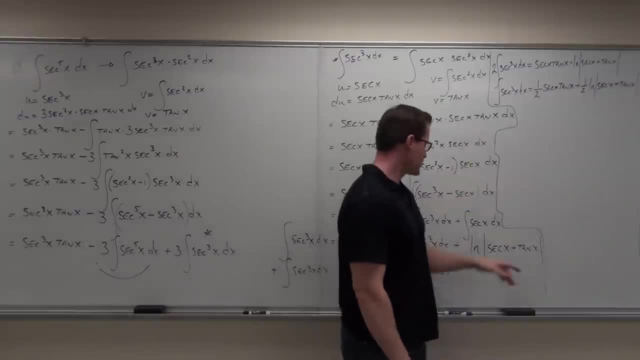 No problem. In this case, 1 plus 1 gives you 2.. Just divide by 2.. This piece is gone. That's great. That's what we want. We have this plus this. Divide by 2. You get 1 half. 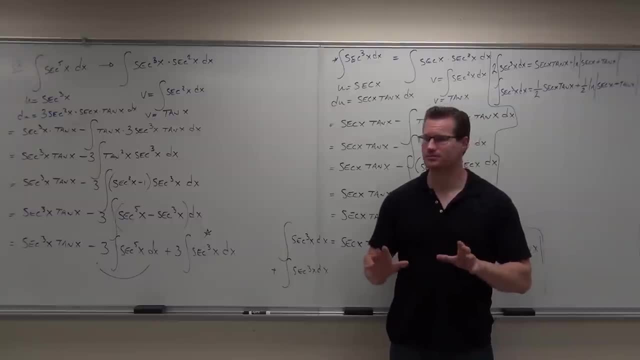 You guys? all right with that one. Now here's the awesome part. We're good to go on this right. This is awesome, This piece. we're going to be good to go. As you pointed out, we're going to be adding this to both sides of our equation. 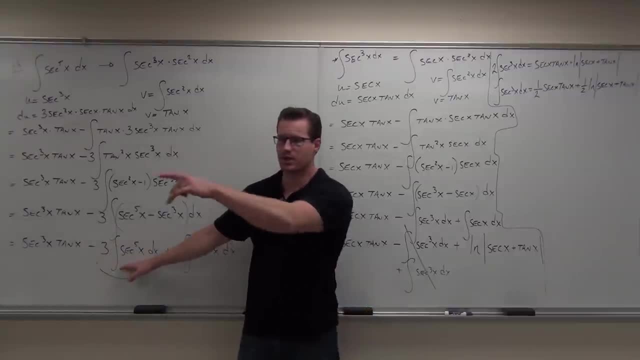 You got me This piece. we now have something for that. So what I'm going to do is I'm going to erase this part. What we know is this: This is 1.. This is 1.. This is 1.. 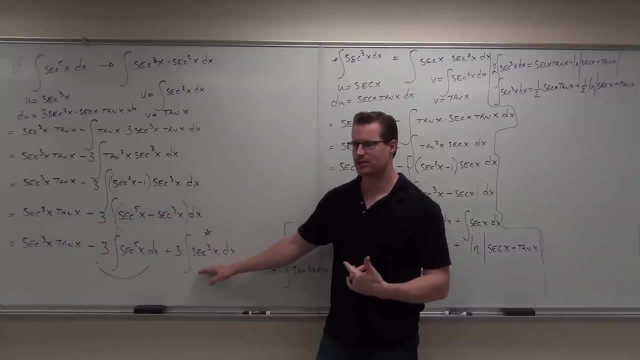 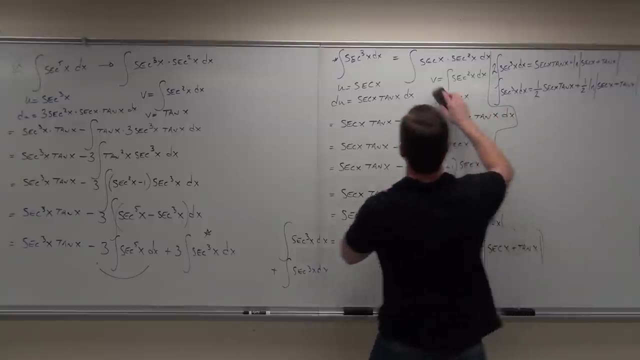 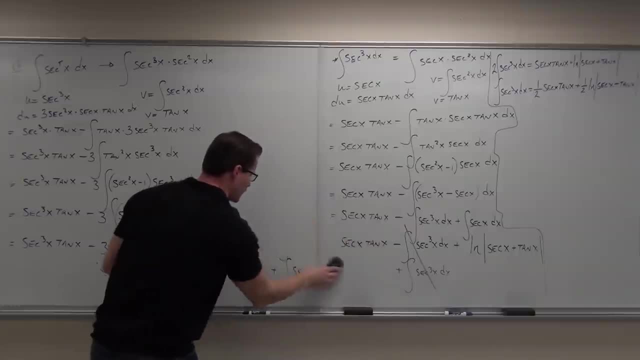 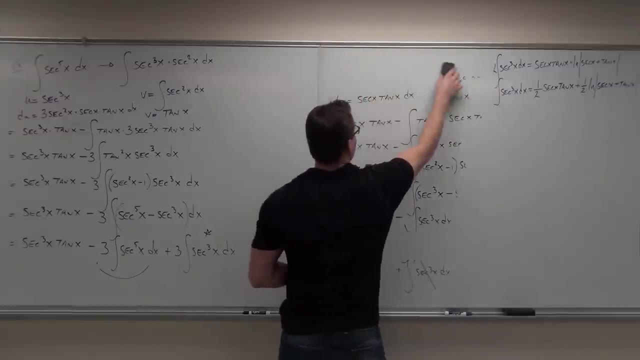 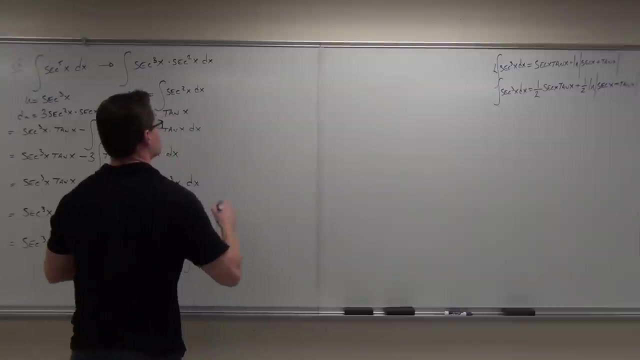 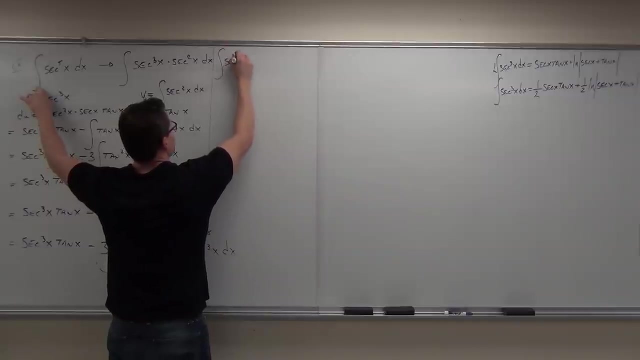 So you guys have any questions on this Iran ratio? give it a little space. Okay, so the integral of secant to the fifth molar- Oh, there's Four- استoras of the power of x, dx is equal to. here's what we know. 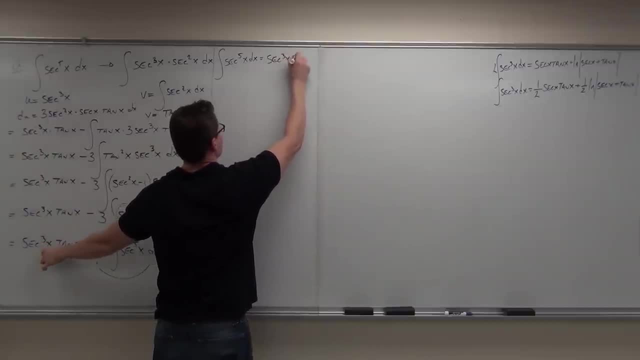 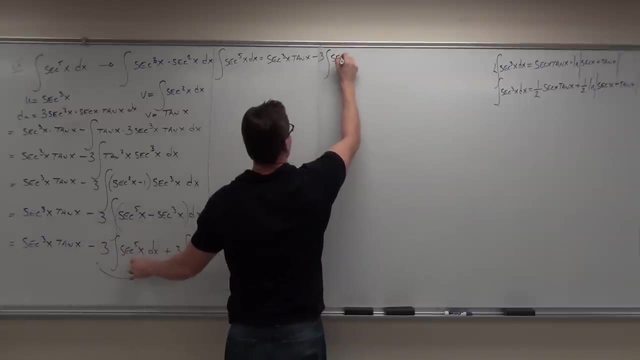 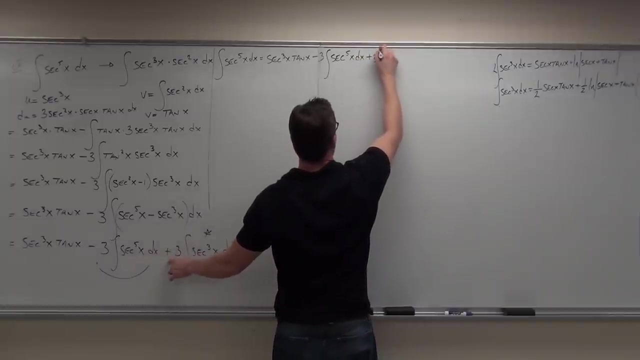 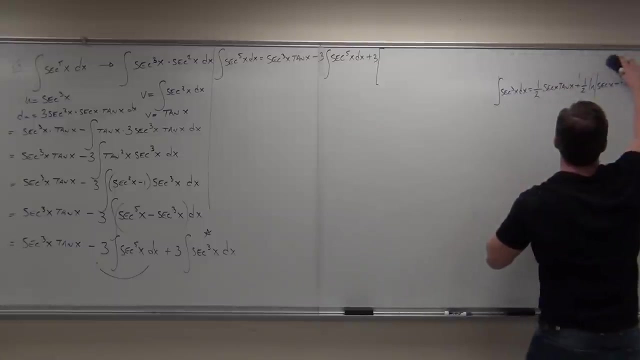 We know it's secant, cubed x, tan x, minus three times the integral of secant. to the fifth again, dx plus three times, plus three times. here's the cool thing, Here's what we know we wanted, plus three times this piece. 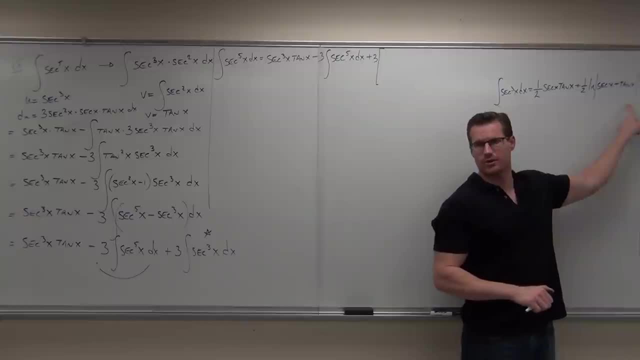 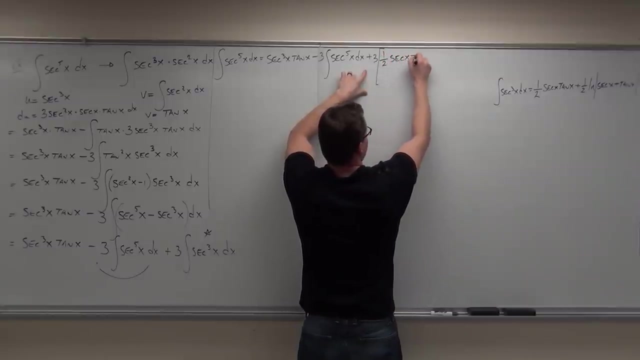 This piece is this whole mess of junk over here. You with me. So instead of three times integral of secant cubed x, we're gonna have three times this whole thing right here. So we're gonna have three times one half secant x, tan x plus one half. 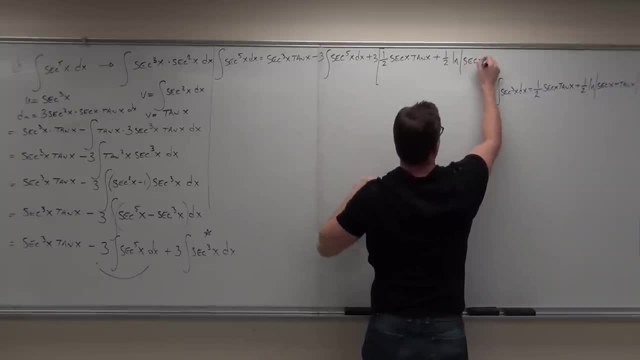 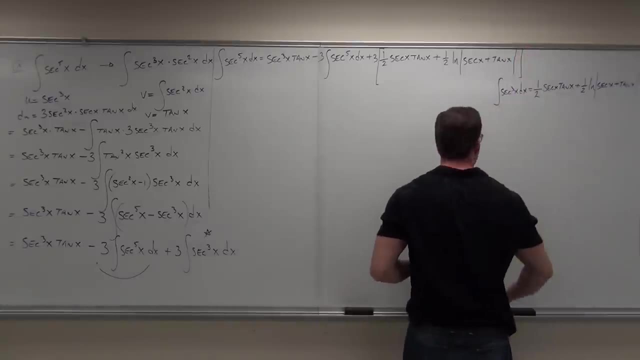 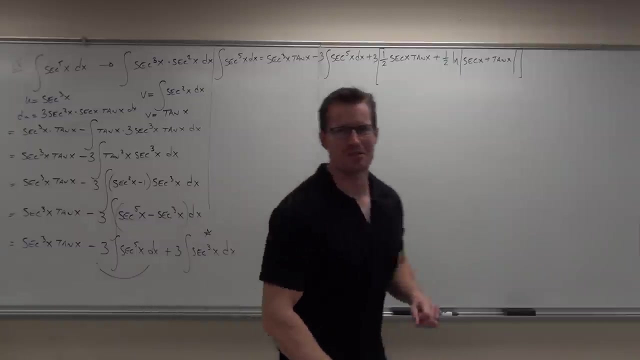 ln, absolute value, secant x plus tan x and absolute value nth bracket. Talk about probably the longest problem you've ever done. huh, You're crazy. We're almost done. almost, We've gotten rid of the integral right. 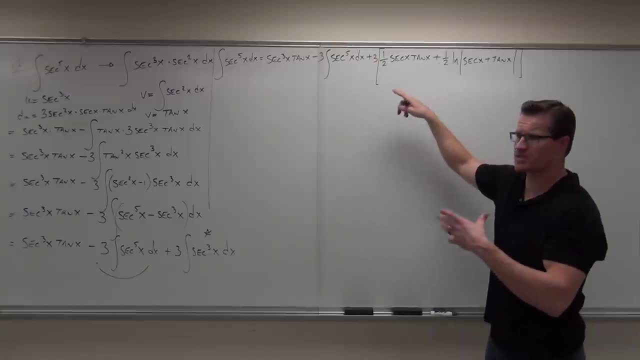 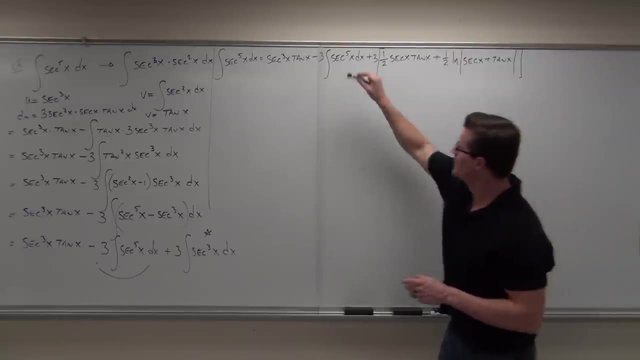 We've gotten rid of the integral, We're gonna have to probably distribute the three to get three halves instead of one half, but that's easy, That's not a problem at all. What are we gonna do next? This is the only integral that we don't like. 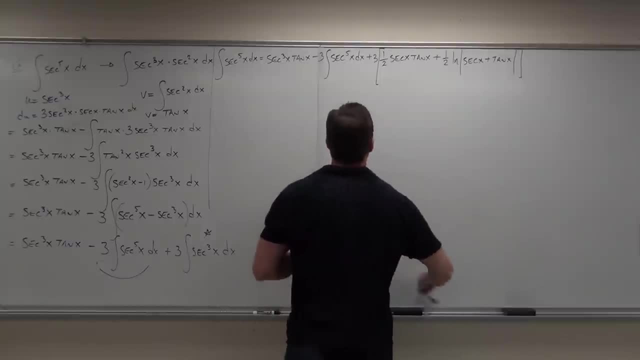 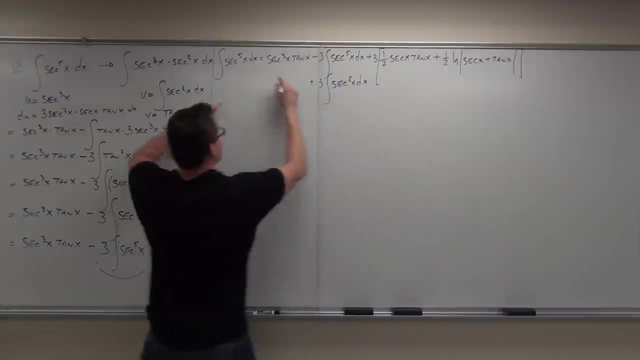 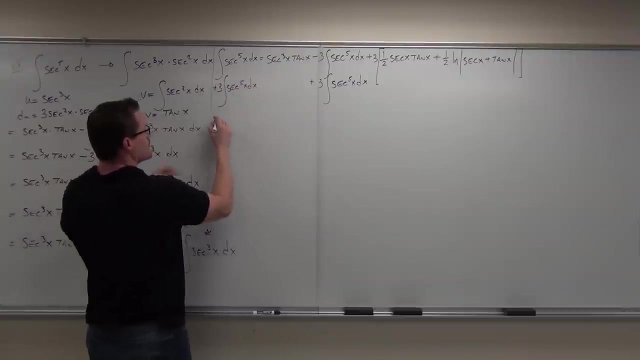 It's already matched up with that one. Just add it to both sides. If we do, if we add three integral secant to the fifth, power, x, dx, it's an equation. Just add it over here, Then I end up getting how much is here? 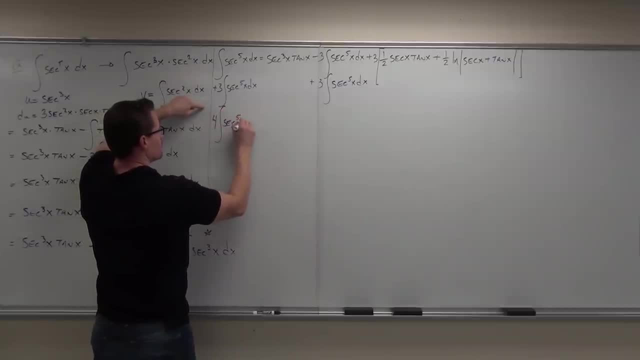 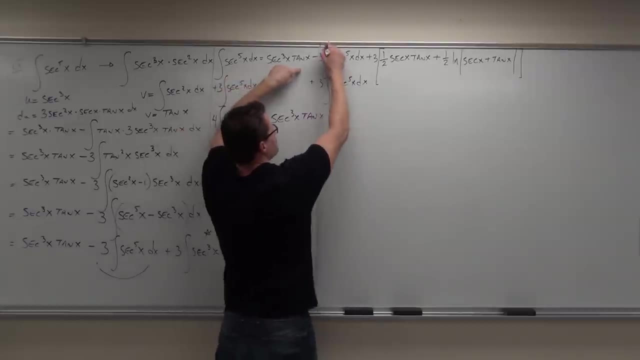 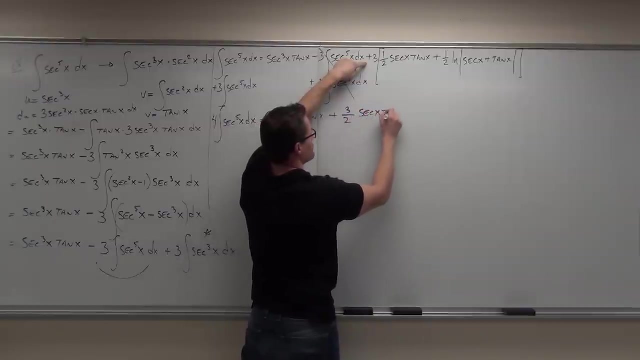 Four secant pi. Four secant pi. Over here I've got secant cubed x. that's right. This is gone. I added it Plus. I'm gonna distribute this: Three halves secant x, tangent x plus three halves. 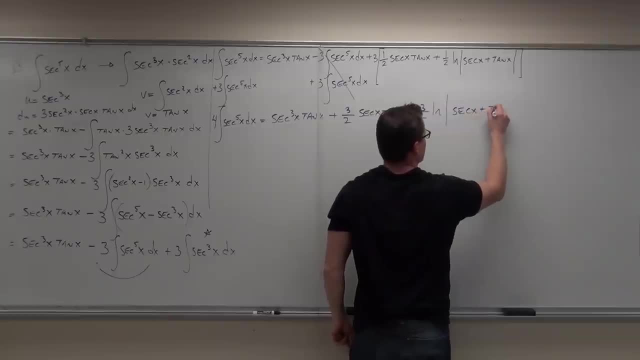 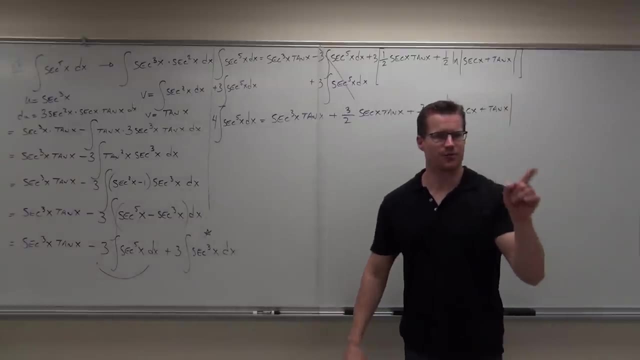 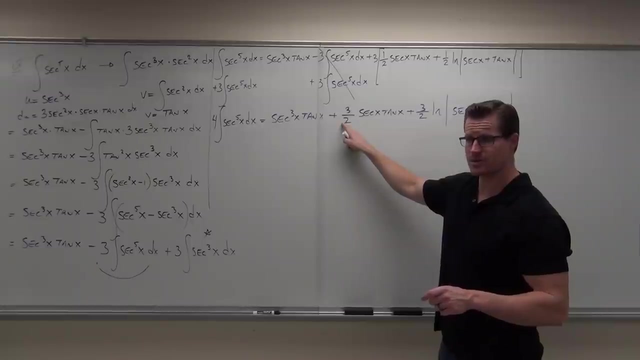 ln. absolute value, secant x plus tangent x. What's the last thing I'm gonna do? Divide everything by four. So this gets divided by four. This is gonna be a one-fourth. This will be a three-eighths. 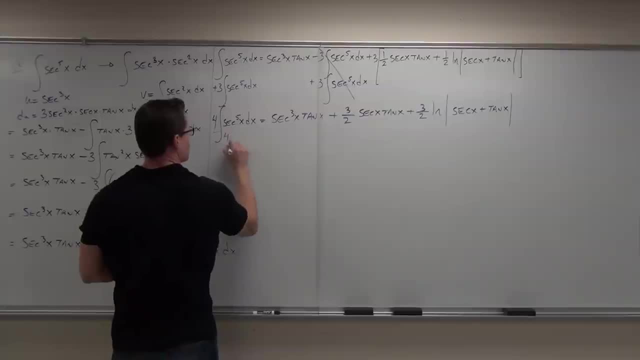 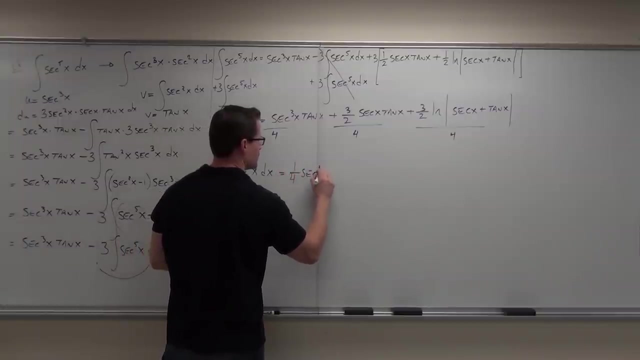 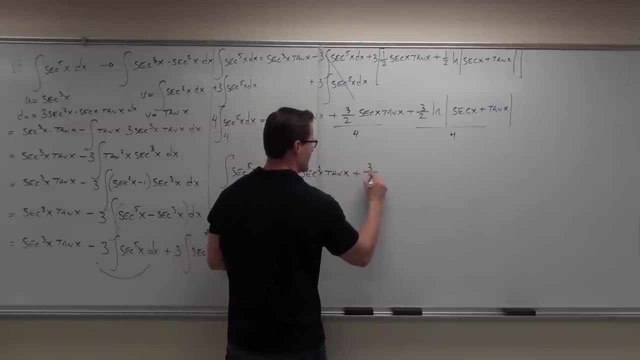 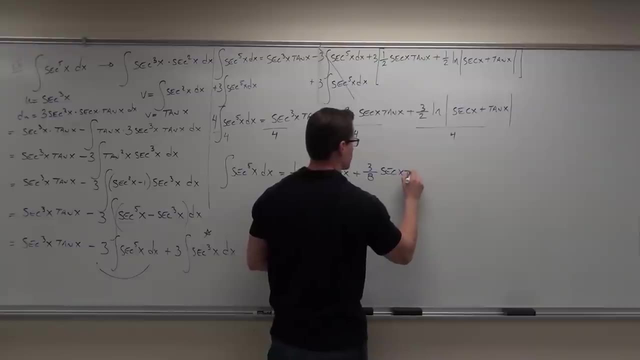 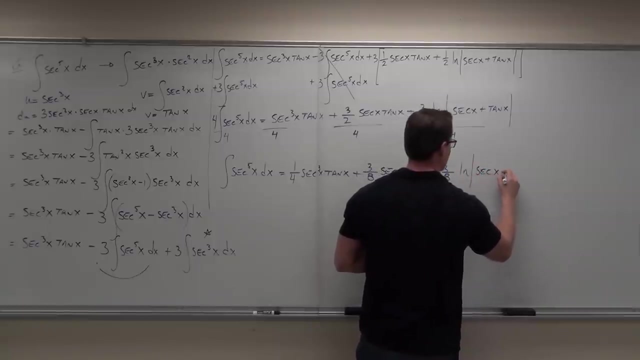 Anytime you divide a fraction like this, just multiply the denominators when you're good, Plus three-eighths. Anytime you divide a fraction like this, just multiply the denominators when you're good: Plus c. gotta have the plus c. 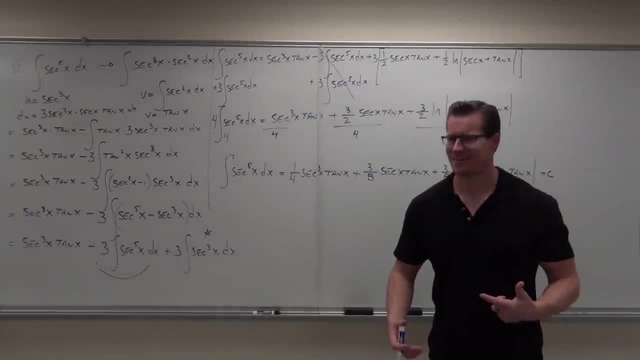 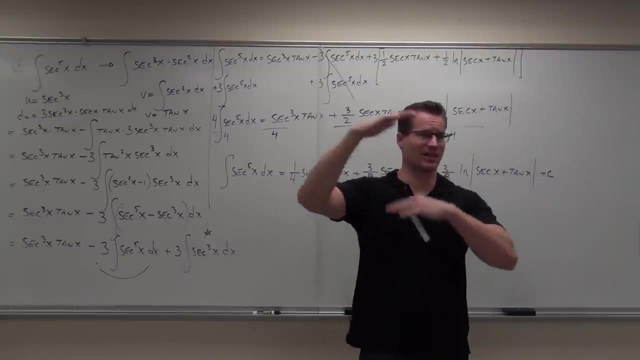 Oh, my goodness, Do you get the idea here? Did I just lose you? I don't wanna lose you, I forgot about it. It's a lot, my goodness. This is like a whole pit on my piece paper. It's an entire page, one entire page. 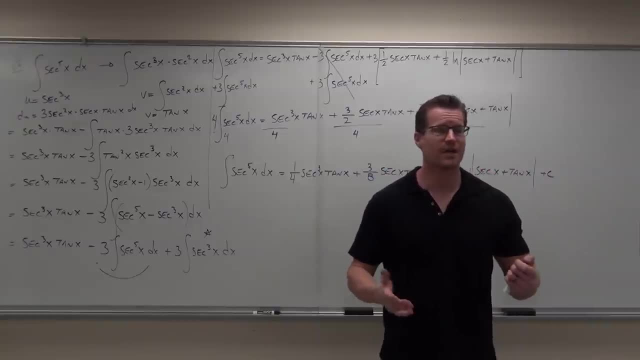 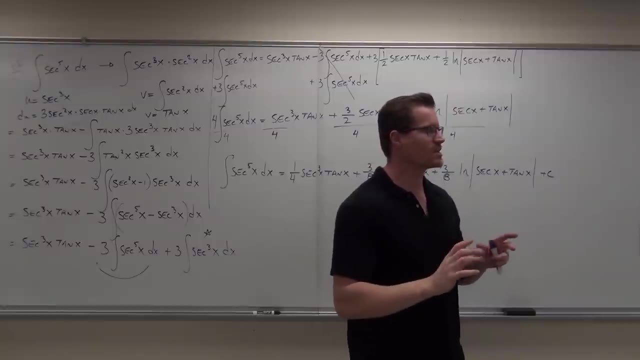 It's just a lot of things going on here. I want to show fans if you can follow it make sense to you. Good, so so that is this. start with something that you can actually take an integral hang on. Start with something. I shake it in below if you can't find it, split it up. 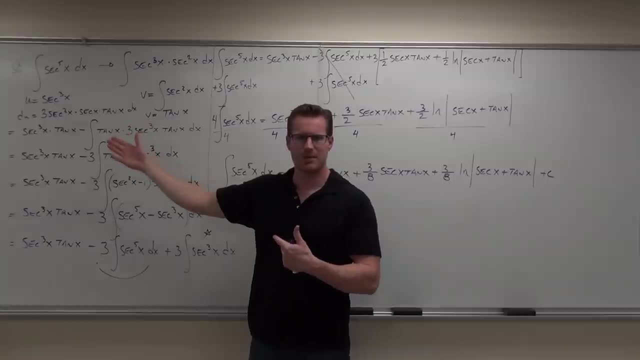 Do that. you roll the piece, then see what you get. if it's trigonometric or something with the exponential or both, Often times you're going to get back a piece that looks exactly what we started with. if you don't have any other integrals, You're good, like we did over here. 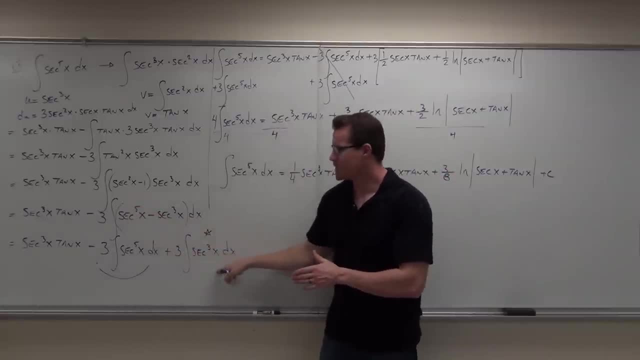 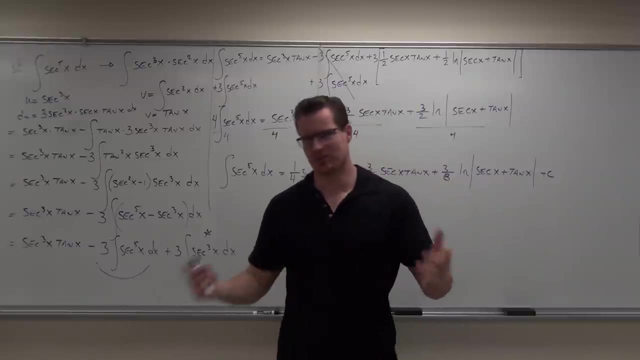 No, there are integrals, no problems, add to both sides. if you do, You might have to do the whole thing again. take care of that integral, then you can ultimately add it to both sides. Divide by your coefficient and you're done. Okay, so the last little bit that we're going to talk about in section 7.1. 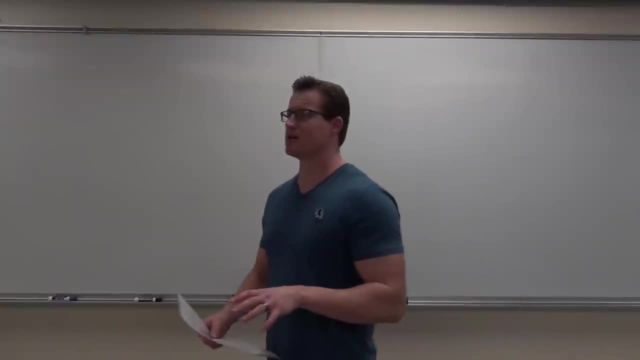 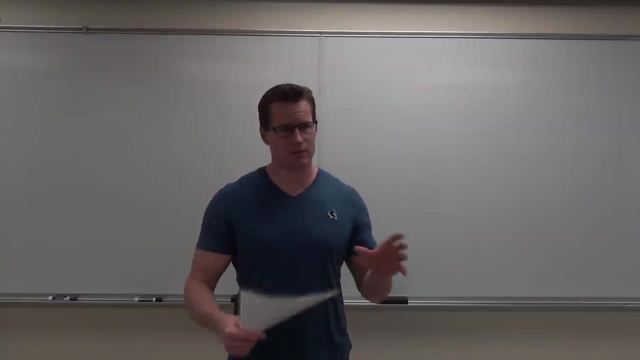 I'm going to invent for you the reduction formula. what this does is when you have like a Sign to some power inside of your integral and we can't take care of it Just by the integration table, we can actually reduce it to a lower power of sine. 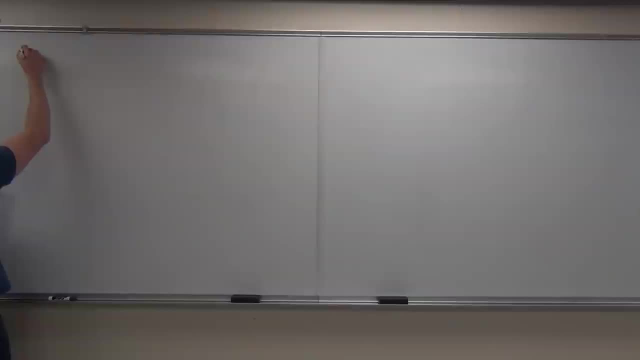 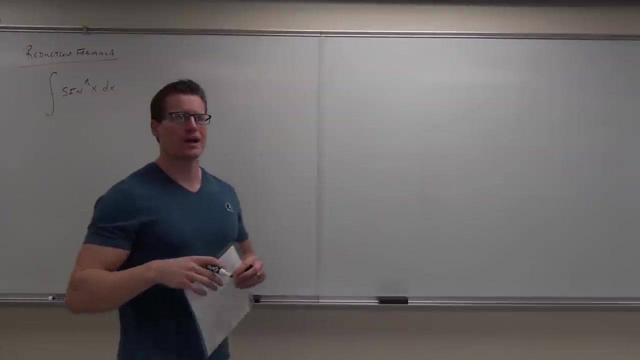 I'm going to show you how to do that right now. so this is called the reduction formula And it starts with this idea: suppose you have some integral with sine to some power, sine to some power Greater than or equal to 2. now, naturally you probably wouldn't use this if you had sine to the first power. 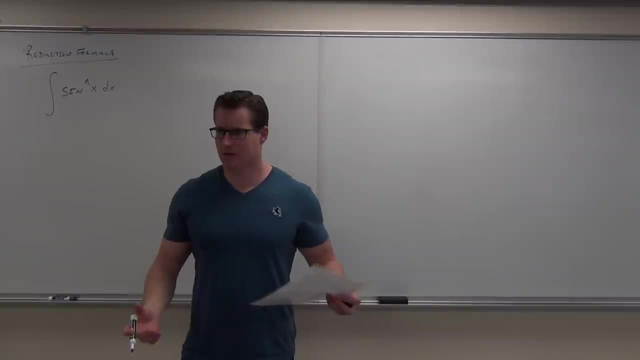 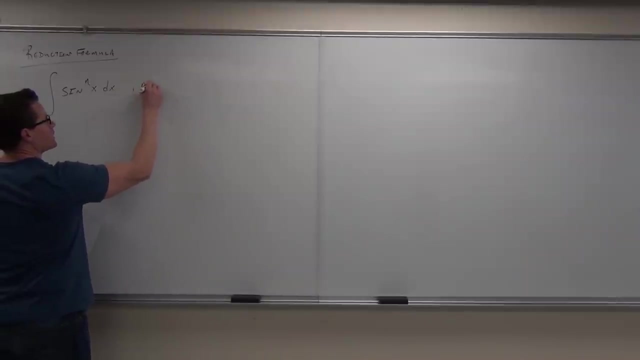 Because what's the integral of sine to the first power? Negative cosine, that's right, It's a negative cosine, that'd be easy, okay. So hopefully you understand that this is going to happen, for n is greater than or equal to 2. So when we don't just have sine, that would be silly to use this well. 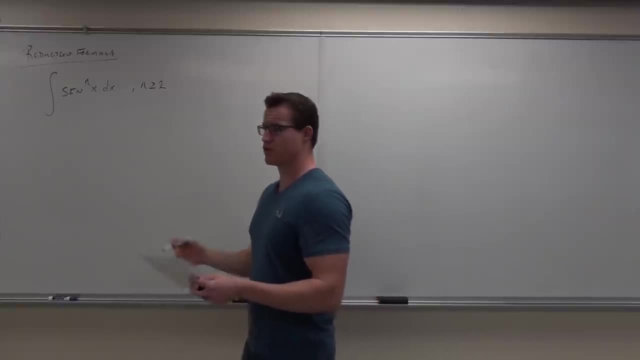 Let's suppose that we do have something, some power greater than or equal to 2. so if you had sine squared x, Well, we probably want to figure out how to, How to do that right, how to find that out, and one way that we're going to do these is with the reduction formula. now, 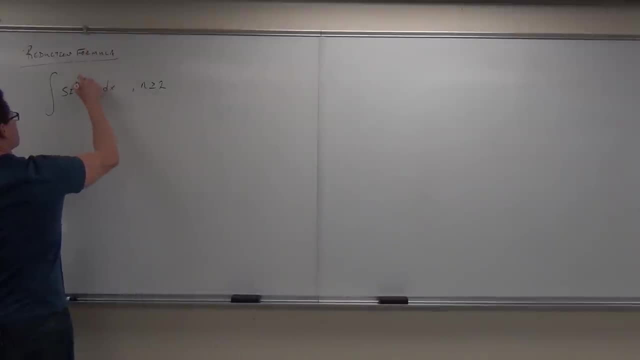 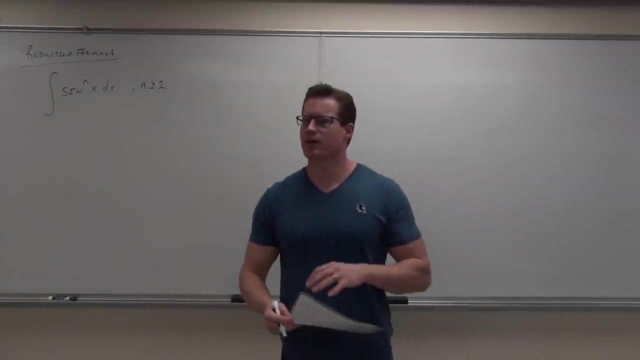 So, basically, what we're going to do is do this problem in general and see what it gives us. so here's an idea. The idea is we want to split this thing up so that we can use integration by parts. a substitution is not going to work. 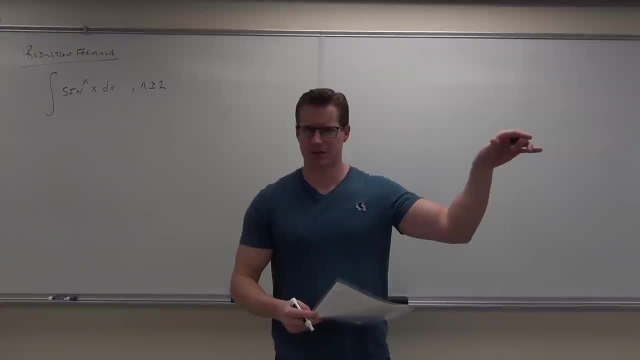 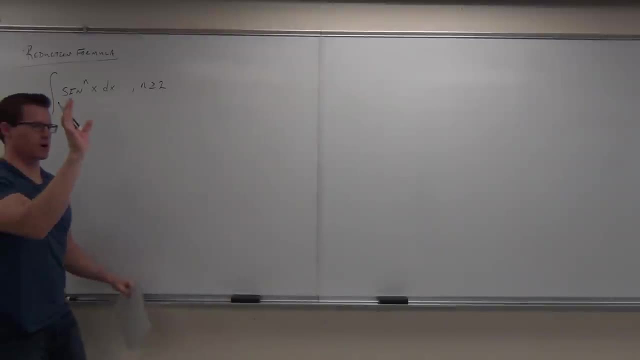 Because we have signs and signs. Does that make sense to you? Are you with me? Is it you? Okay, I'll show you. Here's one thing we're going to do right now. We can't do anything with the problem. There's no substitution. that's going to work, because if I substitute for sine, I get a cosine. does that make sense? 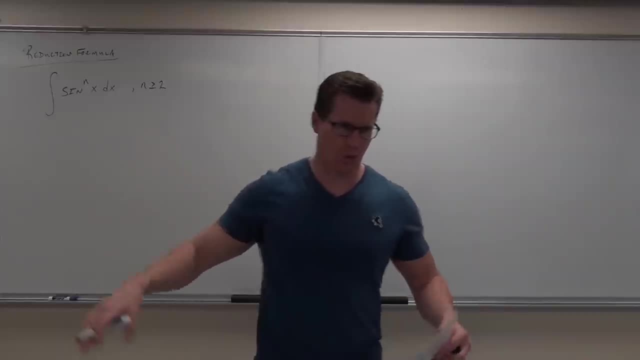 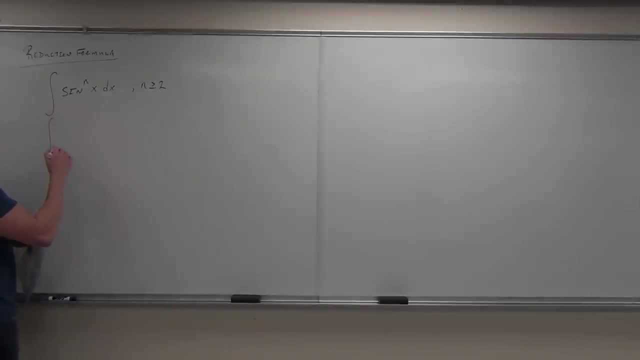 Do you see a cosine up there that a substitution won't work, so let's break off something. now check this out: If I have sine to the nth power, well, Let's split off one power of sine. if I do that, then I get sine to the n minus 1 power. 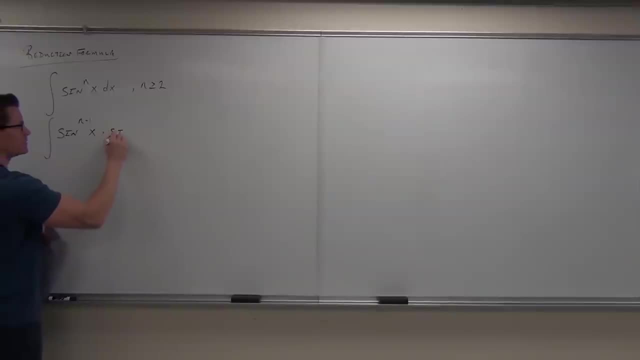 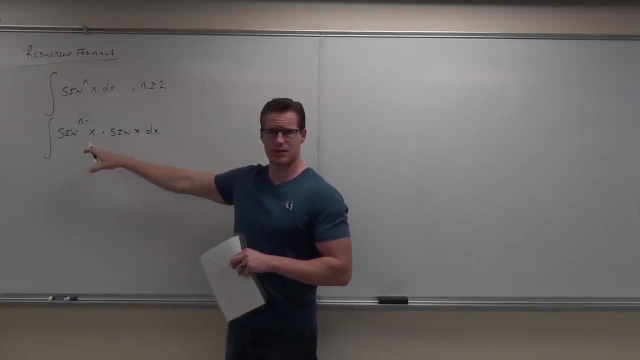 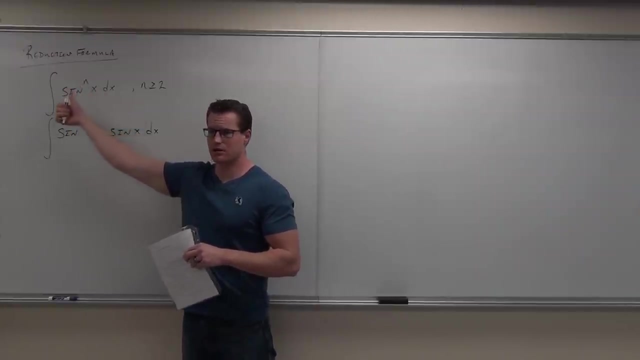 times sine to the first power. I need you to verify for me that this is equivalent to this. You guys with me on that one. Remember: when you multiply common bases, you add exponents. so n minus 1 plus 1 gives us our n. Does that make sense? 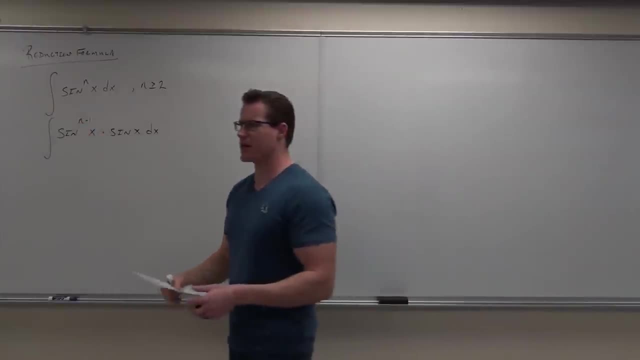 Here's what I mean about a substitution not working right now. if you couldn't visualize this in your head, visualize it now. If I try to do a substitution for sine, what's the derivative of sine cosine? It's not sine. so this is a problem. 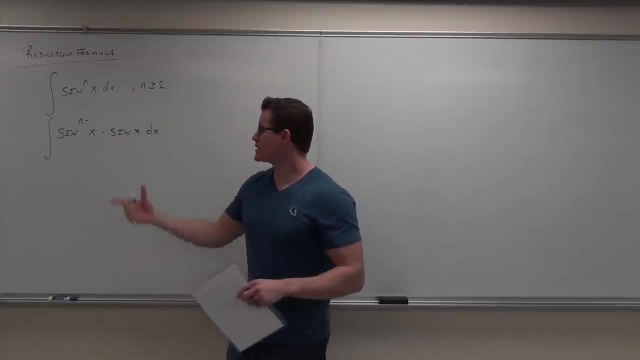 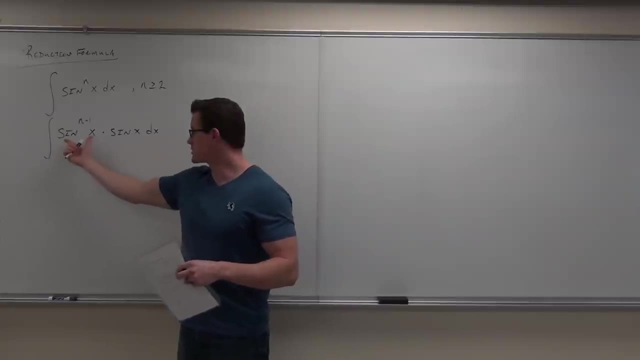 So what we're going to do now is: well, let's go through the whole process. Does this fit our integration table exactly? Not even close. Will a substitution work? We just talked about that. No, No, because the derivative of this is cosine, not sine. that doesn't work. 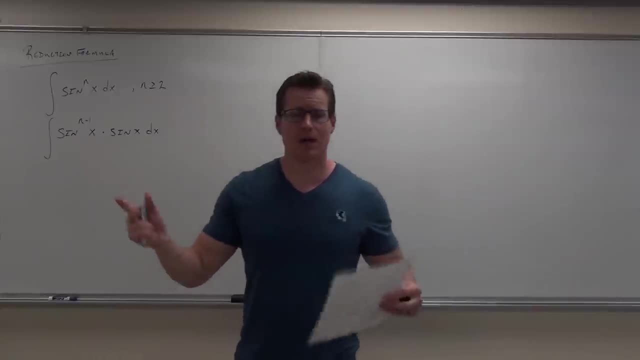 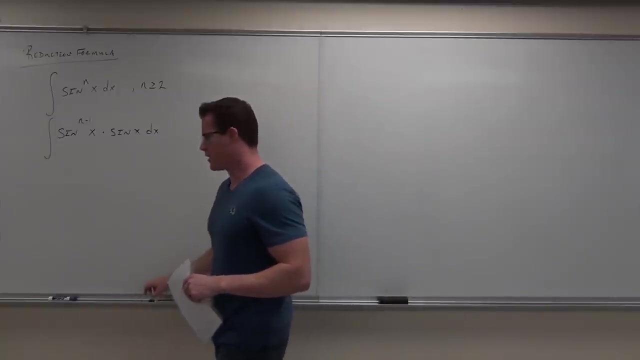 So we're going to have to use Minimal parts. We have to Now remember when you're doing integration by parts- and some of you haven't had very much practice- I know it's a brand new section and you haven't ever done it before- When you're doing integration by parts. 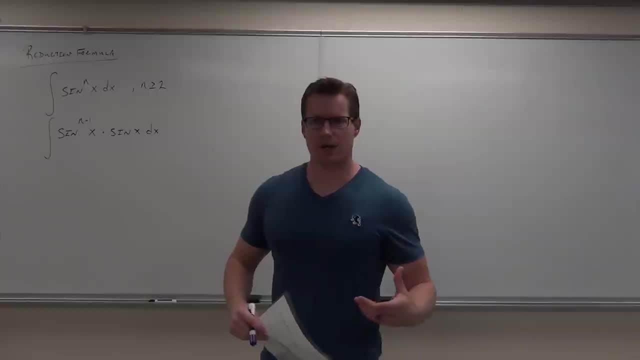 You might have to do it a few times. It's not a one and done all the time. okay, Especially if you have something like what you saw in the math lab: T cubed e to the t. You're doing that. You're having four integrals there. 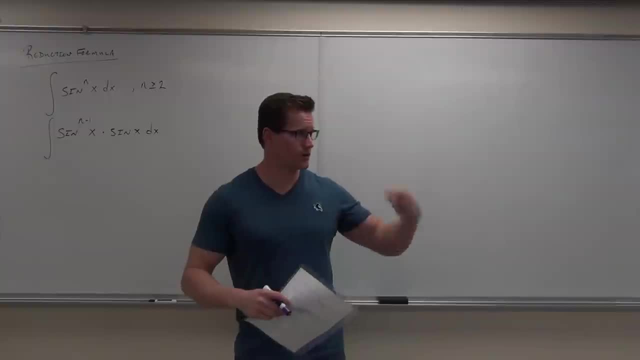 You're going to do it three times: integration by parts, three times. So it's often times you have to do it more than once. Well, here and the way you pick it, You pick it so that one of two things happens. One thing has to happen: You have to be able to do the integral of v. 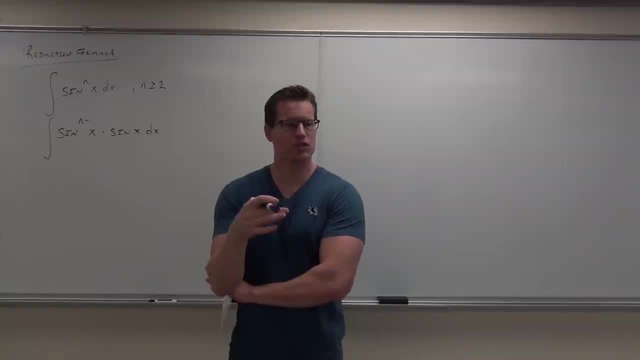 Does that make sense? You have to be able to integrate that, And That's what we're looking for is secondary Is that the derivative of the? u becomes easier. It doesn't grow, it gets smaller, power wise. Okay, those are the two big things you're looking for. 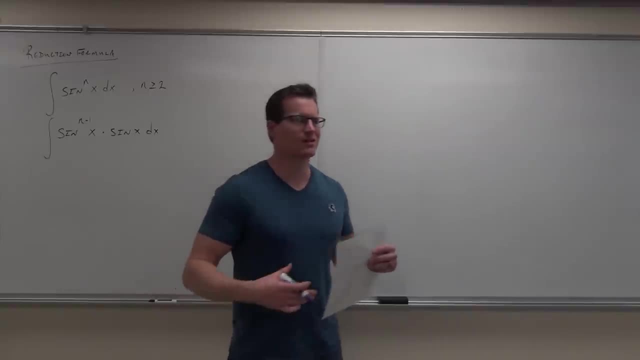 So here let's look at it Now. here nothing's going to get better. Okay, nothing's going to get easier as far as the derivative goes, Because sine, just like cosine or any other trig function, it recycles. So we're not looking to make the derivative any easier. 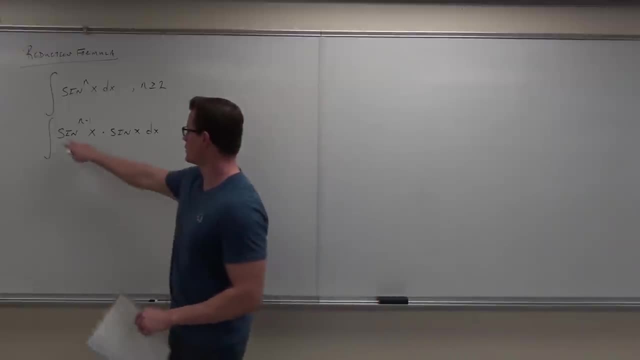 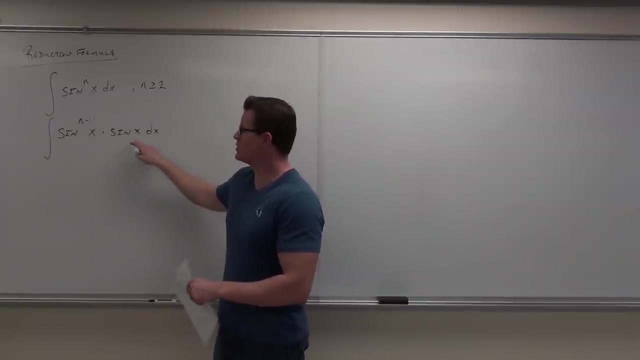 What we'll be looking for is something we can take the integral of. Can you take the integral of this? No, It still has a power to it. Can you take the integral of this? No, Then u's going to be this thing, v's going to be this thing. 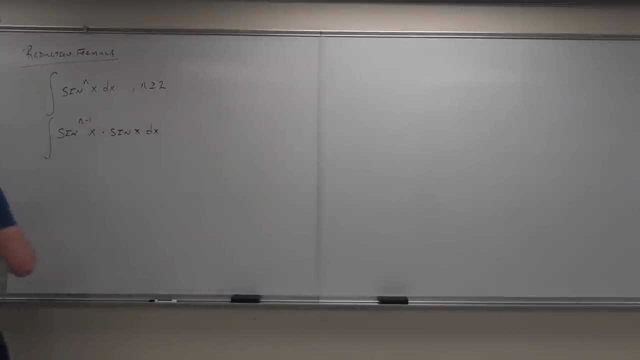 Does that make sense? Yep, Okay, so u equals sine to the n minus one of x, And v equals the integral. Remember how we do integration by parts? Yeah, We cover this thing up. v is the entire rest of the thing. It includes the integral. It includes whatever else you have. 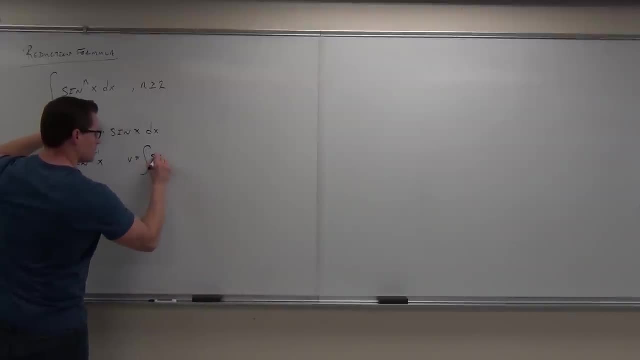 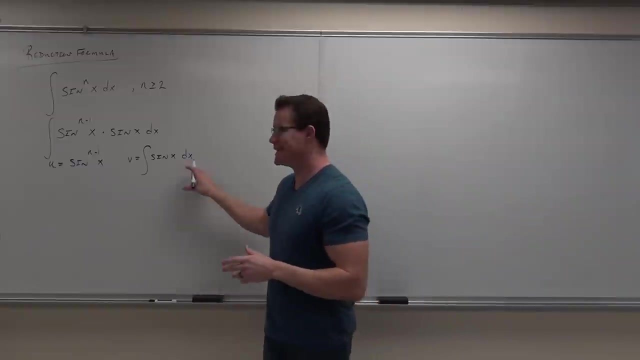 That's horrible looking. Including the dx. Some of y'all are getting kind of sloppy on some of your integrals. You're not putting the dx, You're missing stuff. You're not putting the dx over here or the du. Make sure you have those little pieces. That's kind of important. 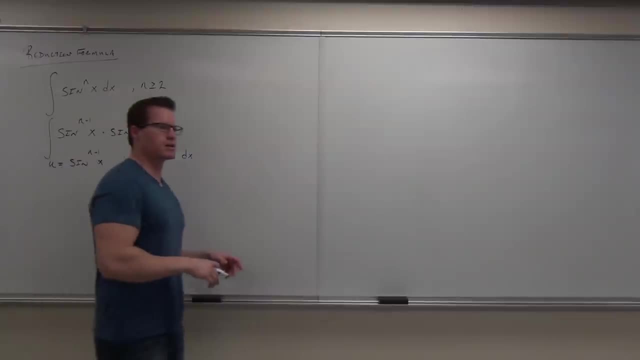 Okay, So next thing we do: Why don't you tell me What's the next thing that we do? We do the derivative, The derivative. Okay, so du equals, Look at how this derivative is going to work. The power is n minus one, You with me. This involves what? 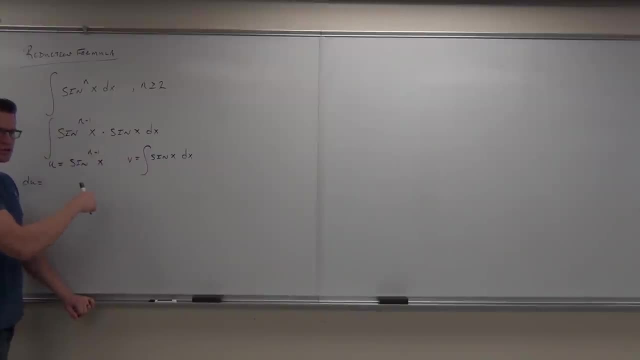 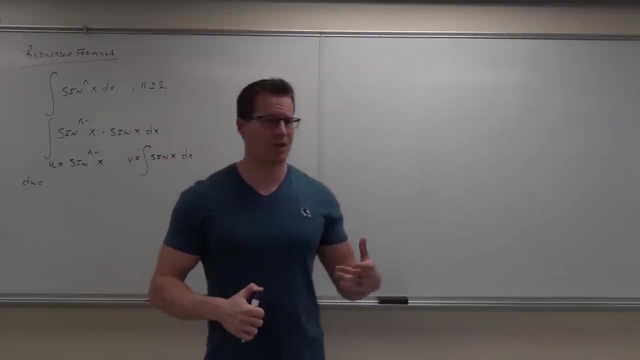 It's going to be a chain rule. That's a chain rule. It's a power rule. Power rule is a chain rule. So power rule says: Watch carefully, Remember. we're just proving this, So you're not going to have to ever do this proof. I'm going to create a formula for you, for you to use. 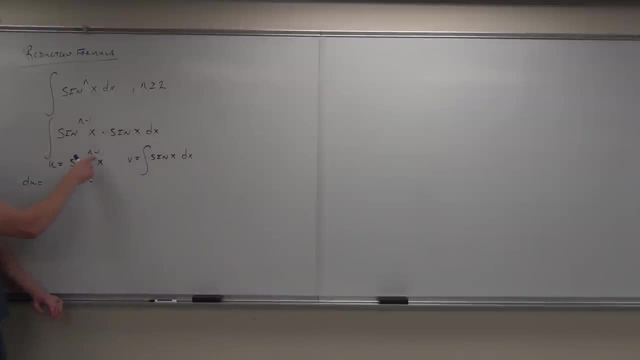 Which is kind of nice, But I want you to follow it at least. So the chain rule or power rule says: You bring this down, You leave the inside alone. You subtract one from this And then you multiply by the derivative of the inside, Which is cosine x, dx. 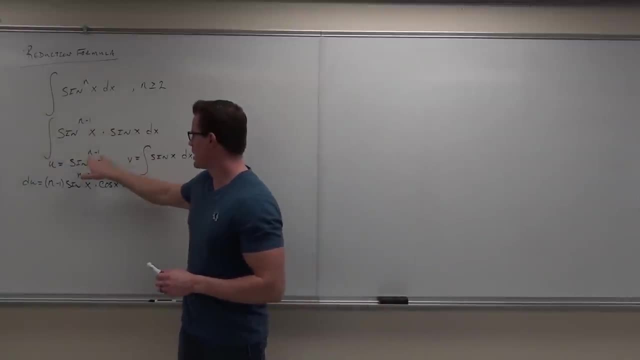 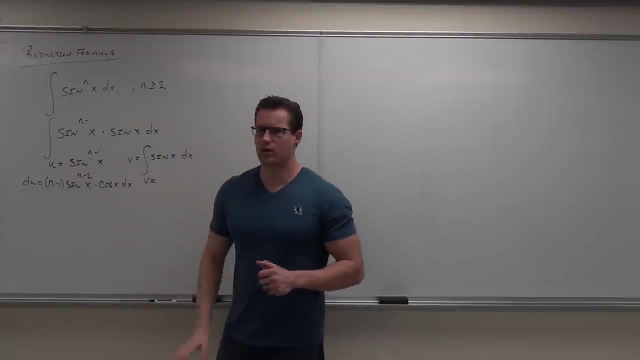 It's just the chain rule. It says: you bring down the power Got it, You subtract one from the power Got it, Multiply by derivative of the inside. We're good to go Show your hands if you feel okay with that derivative. Awesome. Now integral of What's the integral of sine x. 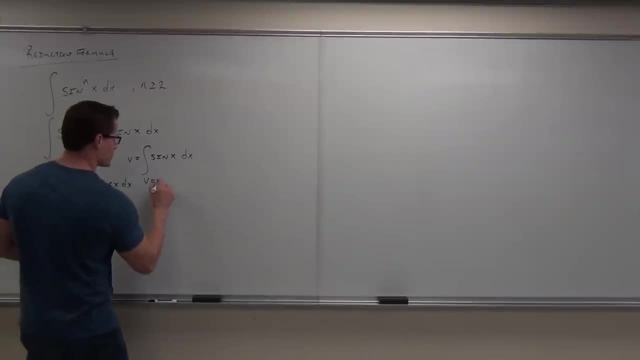 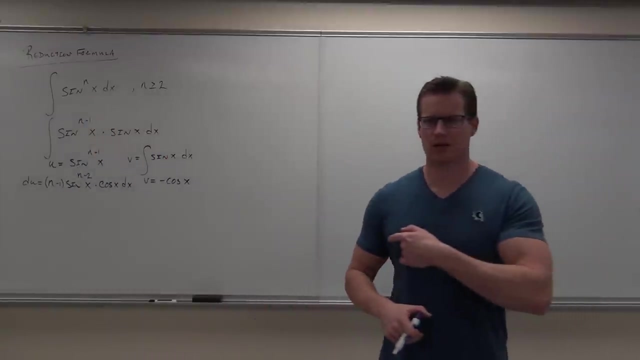 Negative cosine x. How much Negative cosine x? Negative cosine x? Okay, Let's see what this does for us. So we've just performed the- What was it called? again The whole process. What is this? Integration by parts, Integration by parts. Okay, so we're just doing integration by parts. 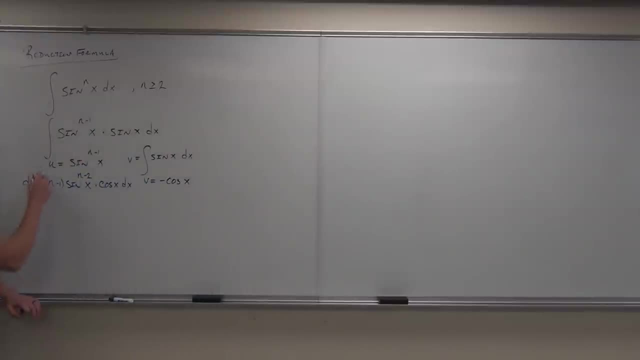 Let's write out what it is. We know. integration by parts says: Once you picked your u and you found your v, The integral equals u v minus integral of v du. Or, in our case, u times v minus the integral of v du. Where this whole thing is my du. 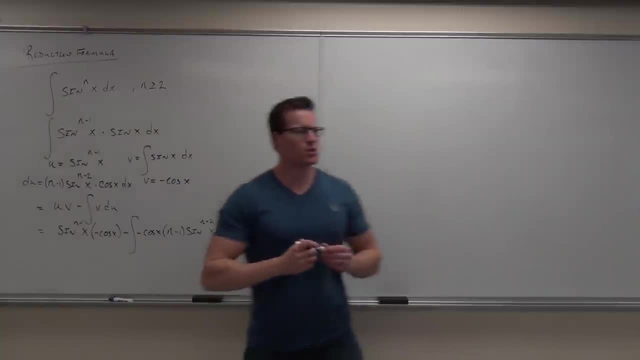 I'm going to clean it up in just a little bit, But I want to make sure you guys are okay with this. Do you see where everything's coming from? We've got our u times, our v. Got that Minus, no problem. Integral of. Here's our v. 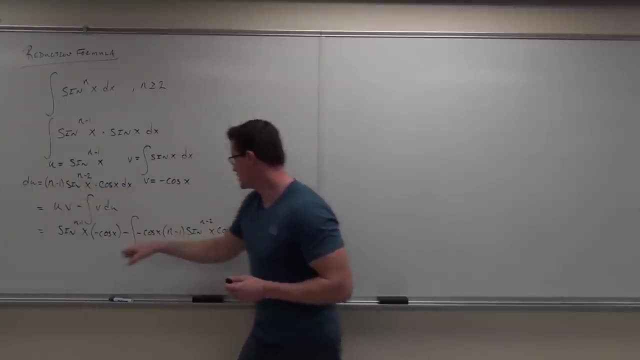 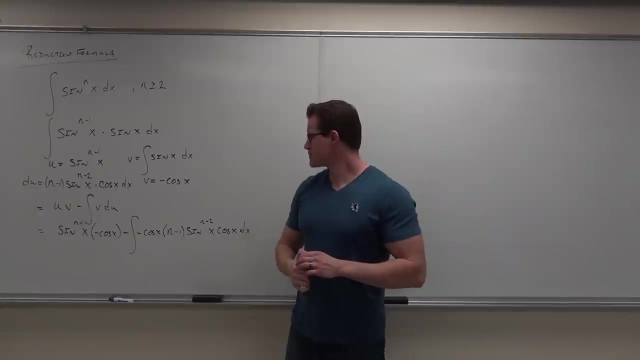 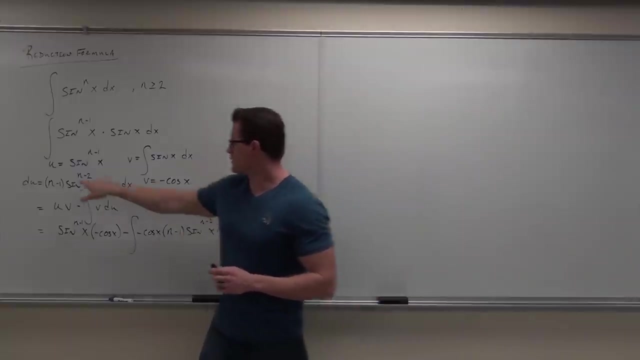 And then this whole mess of junk is du. So we've got exactly the same thing. Show your hands, if you feel, okay with that one Question. So we've got v equals and then Say what? now The? u goes here, We have that. Whatever v is, Whatever you solve for. 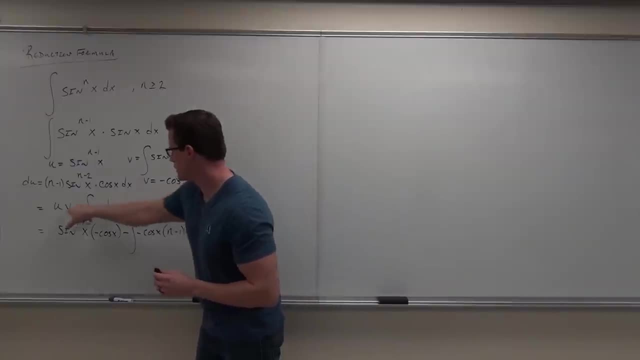 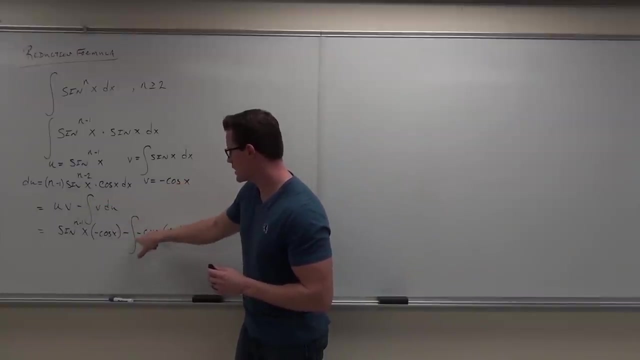 We don't need this, We need this. The v follows that up. So v goes here. This is this: Minus minus, Integral integral. Plug this thing in again, So negative cosine x, And then du is this whole mess of junk. That's right here. Does that make sense? 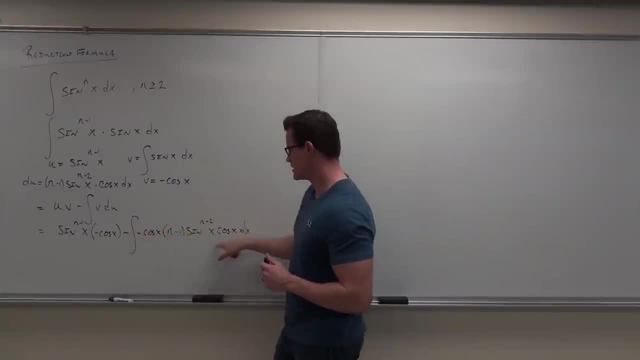 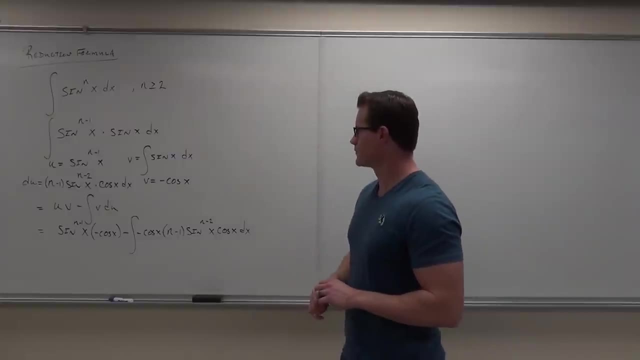 So look at this again: Here's v, Here's du, Here's v And here's du. That's what's going on. We should find the indefinite integral of sine x. We don't have to put negative cosine x plus c. No, the plus c is going to be one constant at the very end of this thing. 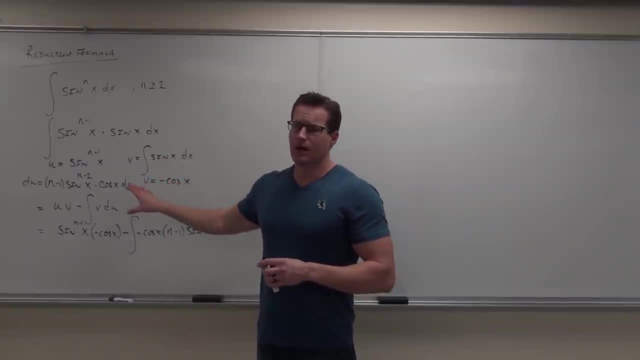 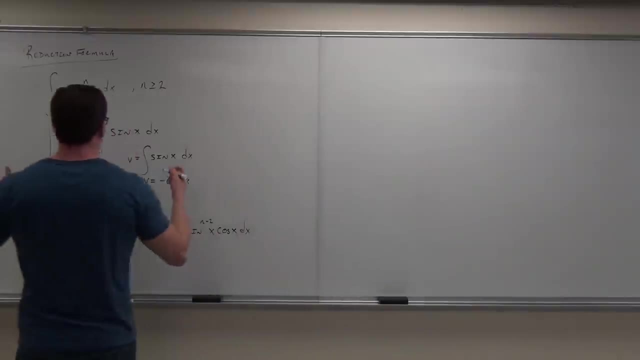 This is just a temporary deal that we're doing okay. In fact, some people show this a little bit differently. Some people show it like this: They say, well, Because remember, it's u dv right, So they show this as dv equals this. And then they go: Well, let's get rid of the D, Let's make this V. 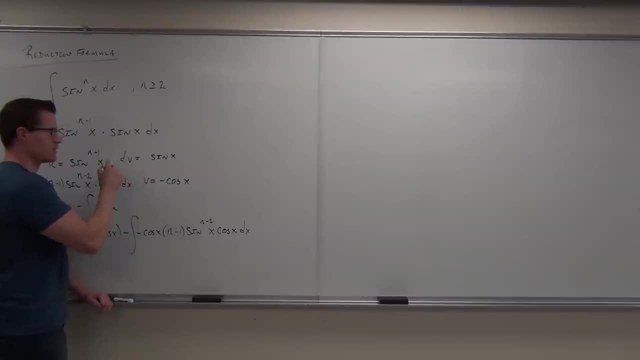 Well, that's the derivative of V, correct? How do you undo a derivative? They integrate everything. We just ignore this. Integral of DV would be V, Integral of this is, So we kind of skip that little part just to make it easy. 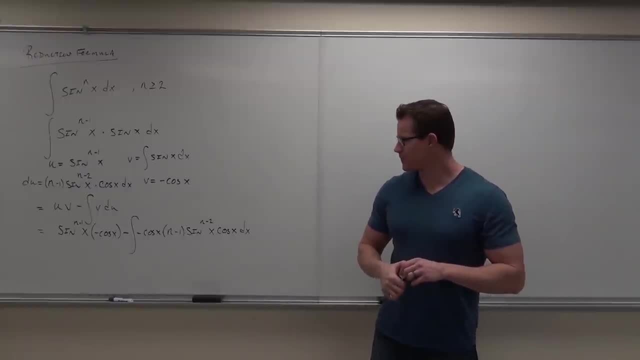 It's easier to write a question: Shouldn't the cosine at the end of V be negative? No, because we're taking a derivative right. So the derivative of sine is positive cosine, The integral of sine is negative cosine. That's where we got that from. 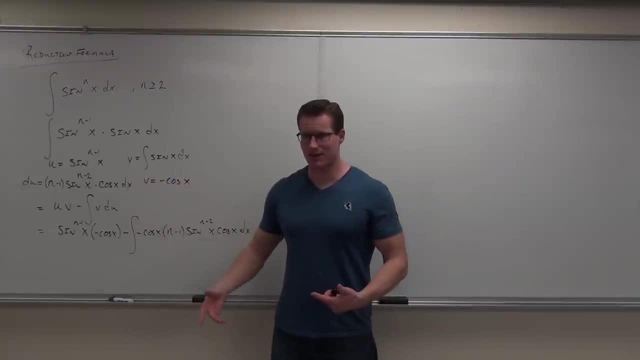 But the derivative of sine is not negative cosine, It's positive cosine. Get them straight in your head. Okay, we've got to have those right, And some of you made that mistake on your last test. We've got to get these things right. 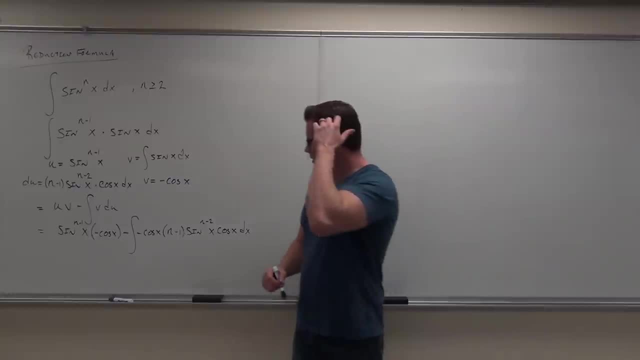 You guys all clear with this one. I'm going to clean it up just a little bit. So what we're going to clean up is we're going to do Probably, pull the negative out front. Negative sine to the n minus 1x cosine x. 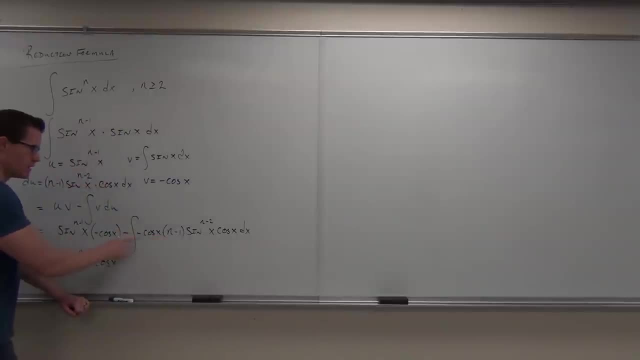 Tell me what happens here. What happens It does, because minus and negative, that's going to become a plus. Also, one of these things is a constant. What is it? Cosine x is not a constant. That is a constant. 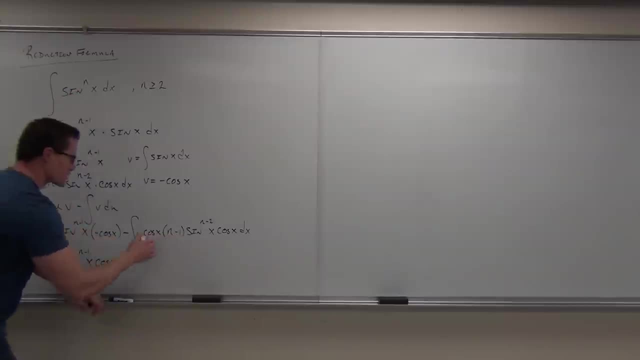 Yeah, n minus 1.. That's going to be a number right. It actually comes right from here, So we're going to have plus n minus 1. Integral Also. let's clean this up a little bit. I've got a cosine x. 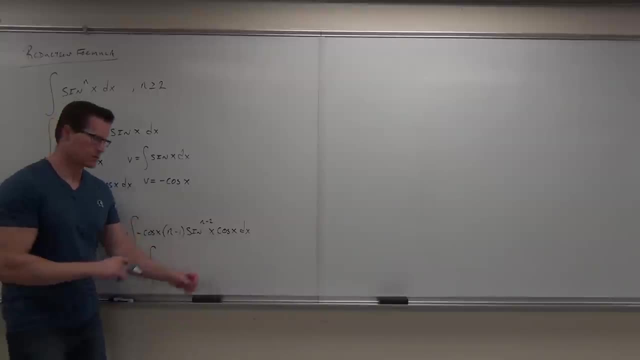 I've got a cosine x That becomes- Let's see what we've done- Negative comes out. That should be easy. This becomes a plus, No problem. This is a constant Pull out in front of your integral Cosine x. 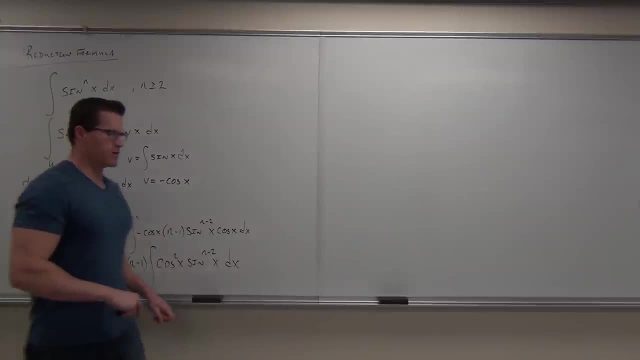 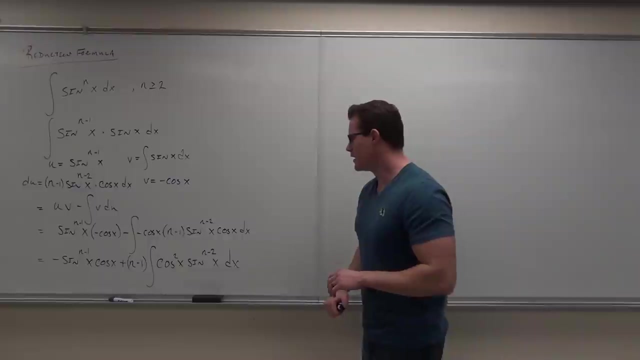 Cosine x is cosine squared x, and then sine to the n minus 2 power of x. I'm not sure if you're okay with that one. Are you still okay? Okay, It's just a little bit of algebra that we've done. 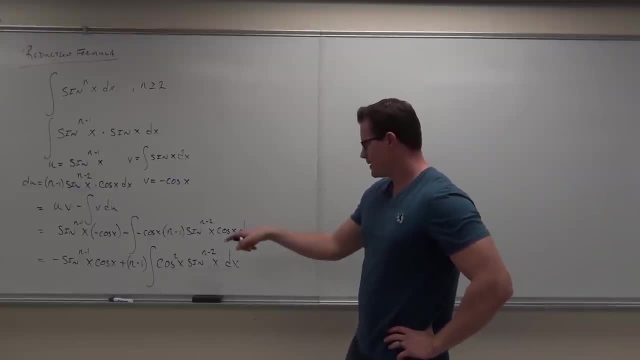 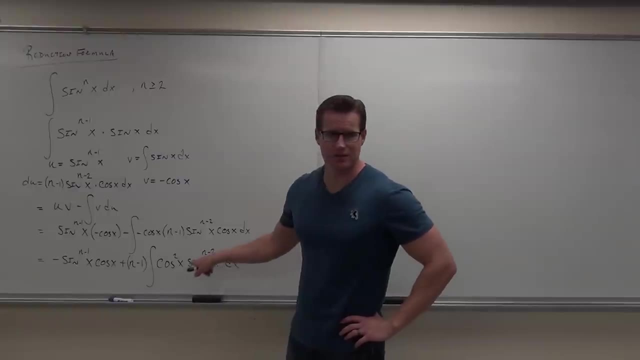 Now here's the deal. Oh man, This right here is a problem, because if we do a substitution with either of them, it's not going to get rid of the entire thing. We don't even know what that power is. 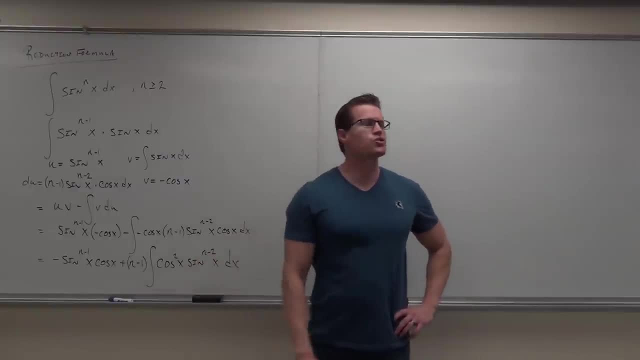 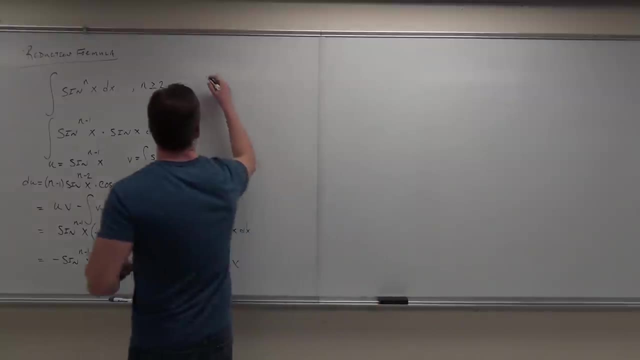 Are you with me? So what we're going to do is we're going to trick the problem a little bit. We're going to call this something different. We're going to call this using one of our identities. Remember that identity. It's Pythagorean identity for sine and cosine. 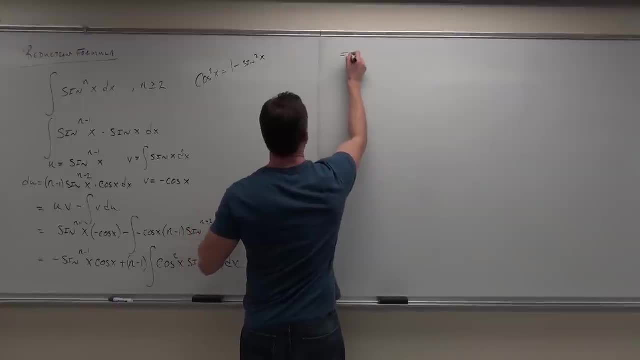 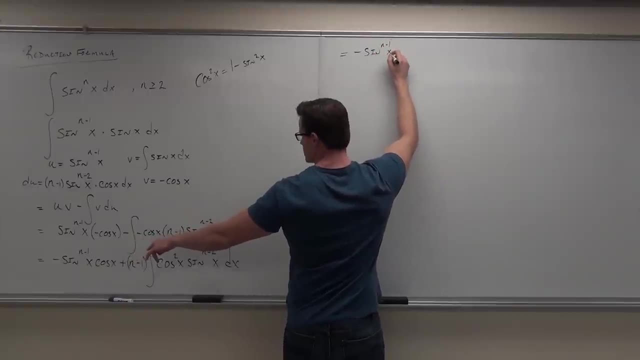 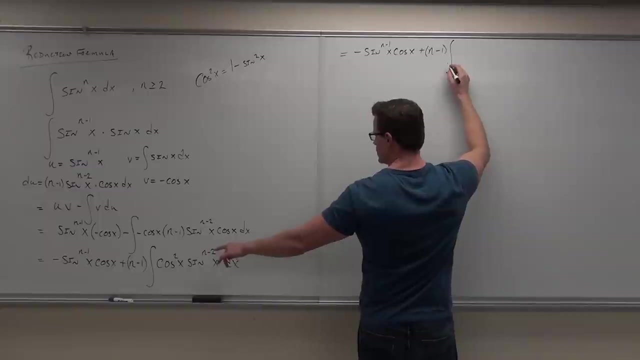 So here we go. We know that this thing equals negative sine n minus 1 of x times cosine x plus n minus 1 minus 1 minus x times cosine x plus 1.. What are the other two things as well? Okay, So cosine squared. 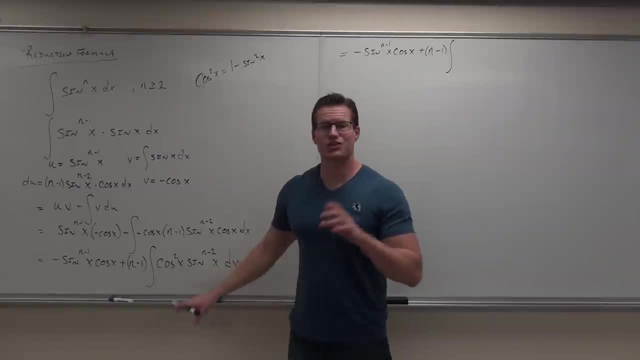 No, no, no, no. Let's not do cosine squared. What we're going to do here is we're going to replace that with sine. So we have sines and sines, and you're going to see why in just a little bit. 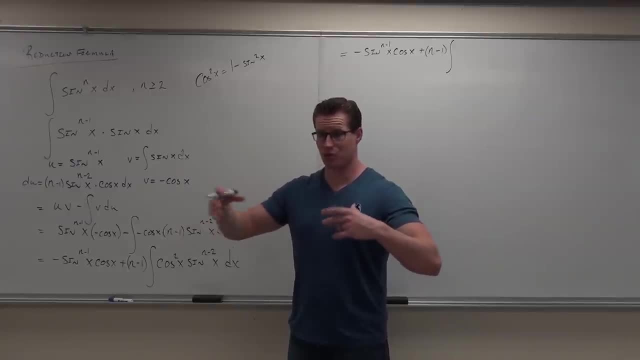 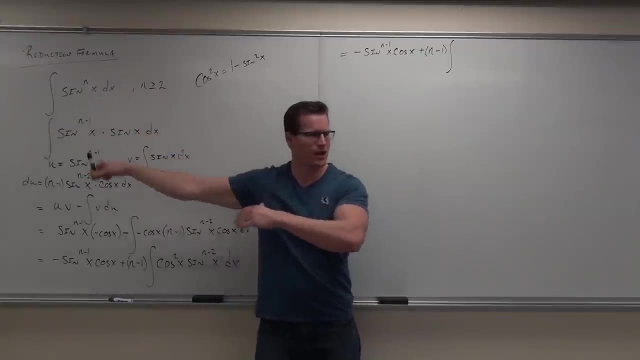 Remember that You've done some of these integrals, probably in your homework, where you have to make it down. Remember adding the integral to both sides. We get the integral back again. You're going to see that here in just a minute. 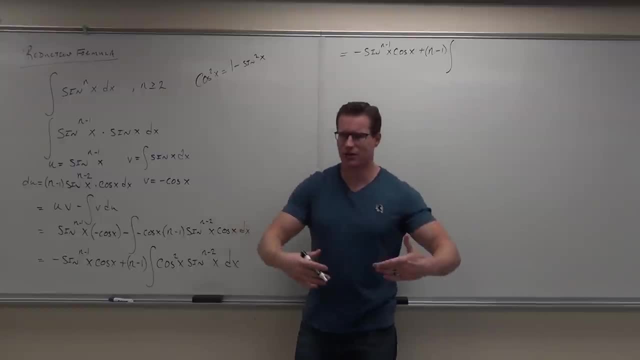 We're going to get this integral back again. Remember what happens when we do that. When these things recycle, like sine and cosine does, When they recycle, you go, oh man, No, just add it to both sides and you're good to go. 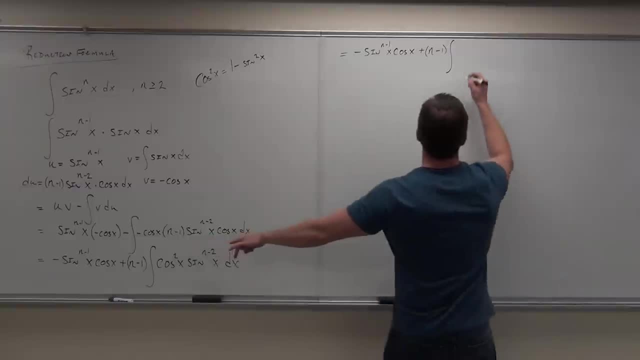 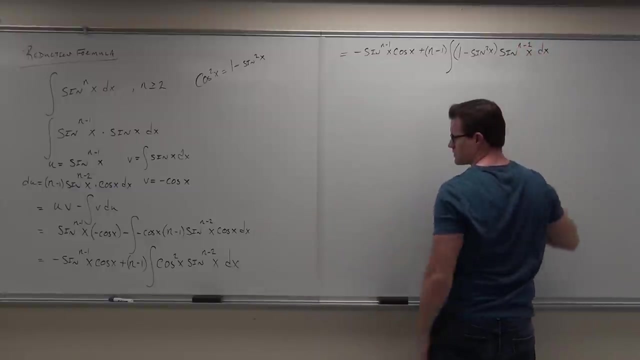 You follow. So we're going to do that in just a minute. So cosine squared. now let's change it. This is going to be 1 minus sine, squared times sine to the n minus 2 power of x dx. Let me know if I've missed anything. 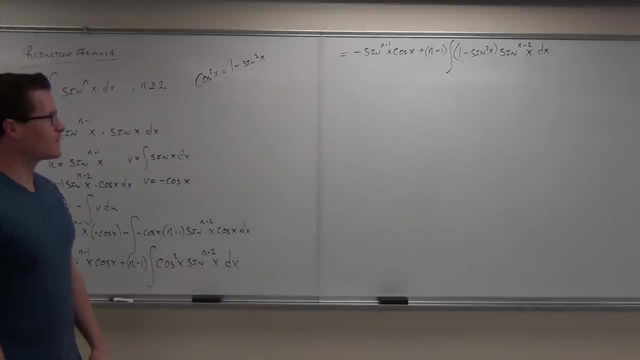 I've written a lot of stuff. Hopefully I haven't Y'all still okay, Yeah, Okay, tell you what the next thing we're going to do. The next thing we're going to do is we're going to distribute this. 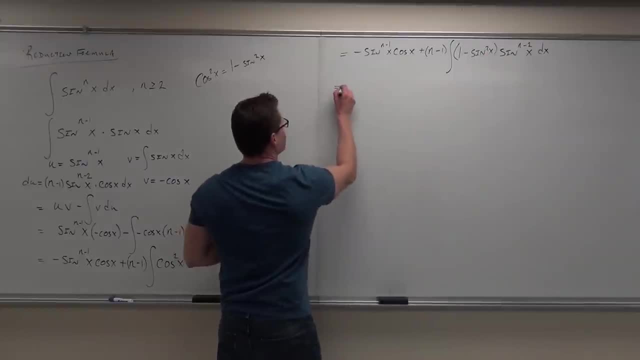 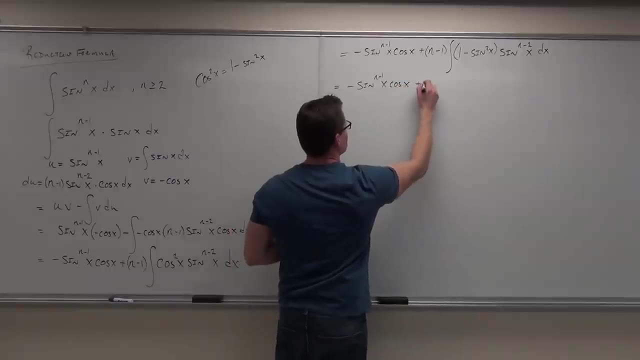 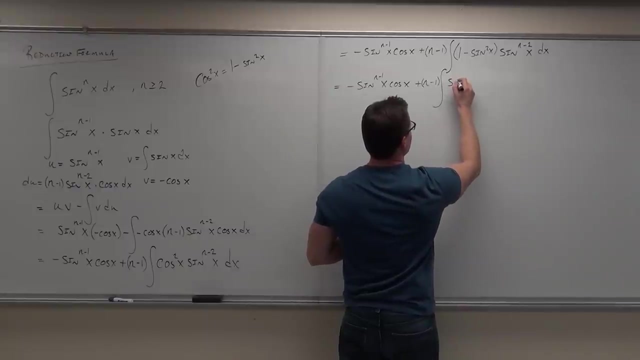 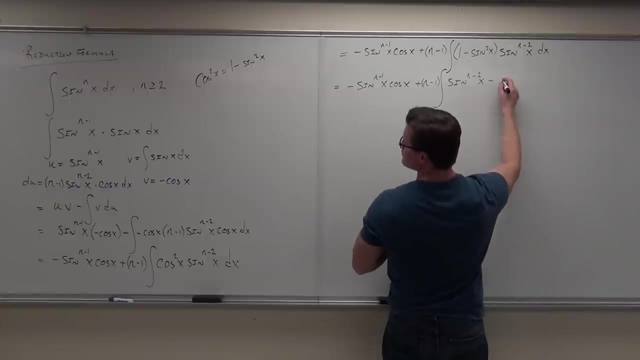 because I don't like this right now. I'm going to distribute this, So we're going to have. What's that going to become when I distribute this? Sine squared x to the n minus 2.. Sine squared x to the n minus 2.. 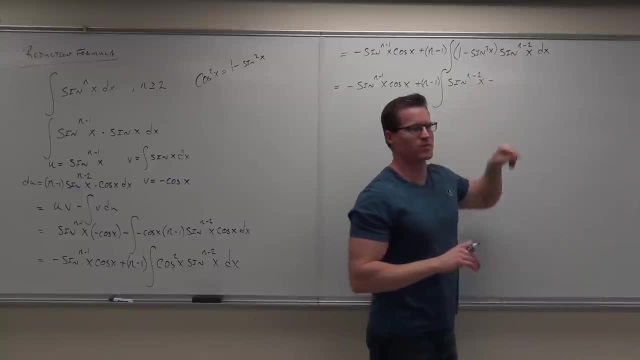 Sine squared x to the n minus 2.. What do you do when you have x bones being multiplied? What do you do? Sine, squared x to the n minus 2.. Let's just add them. How much are you going to get? 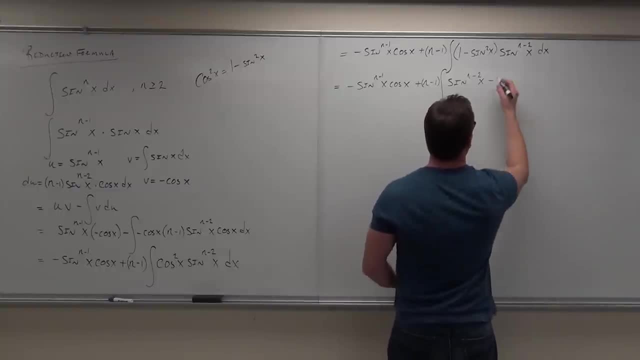 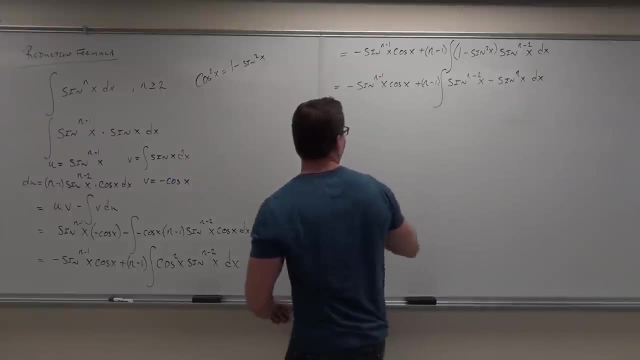 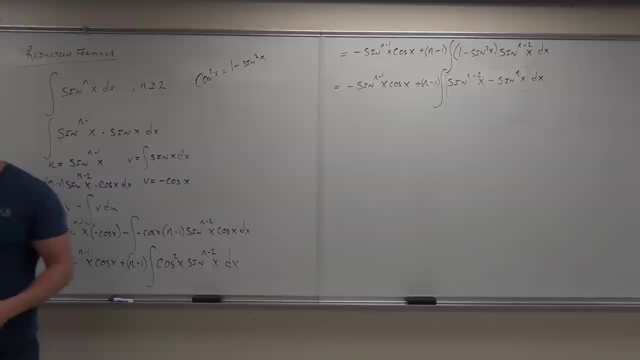 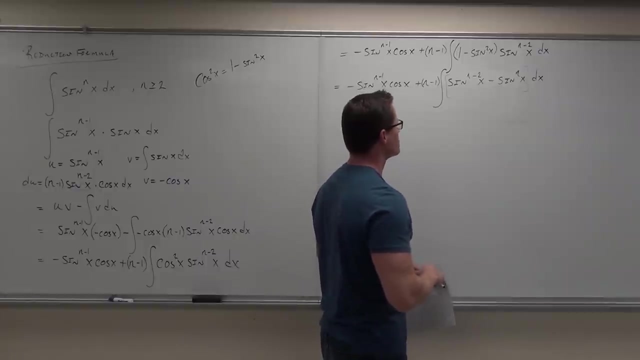 Okay, Okay, and remember, this is in here. I'm going to make sure I'm on my right track here. Okay, You still okay with that so far? Yeah, We are almost to the point where we can start back to the side. 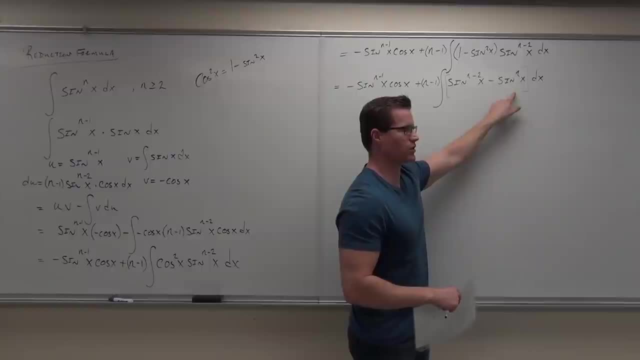 You see, we have it right here, right, But this is wrapped up in this integral, So we're going to split This integral. just one big thing that you need to notice: This is n minus 1 times this entire integral. 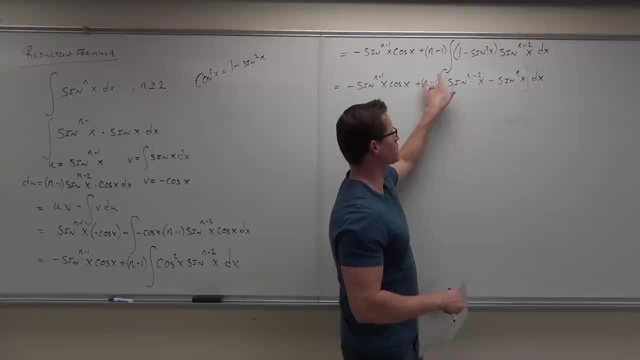 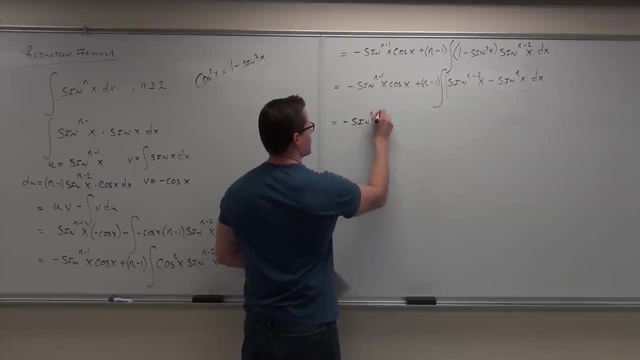 Does that make sense? Which means, if I split this up, it goes to not only the first one, it also goes to the second one. Is that clear? So when I do that, we'll get okay. negative sine n minus 1 of x. 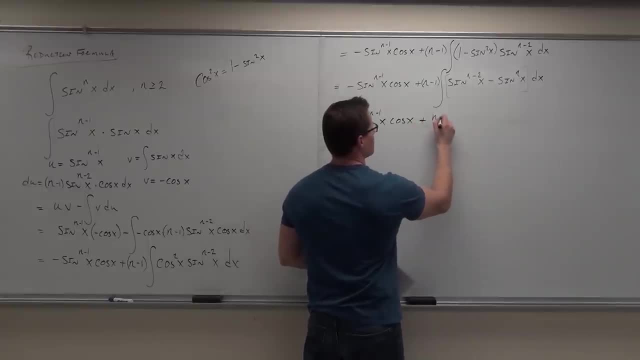 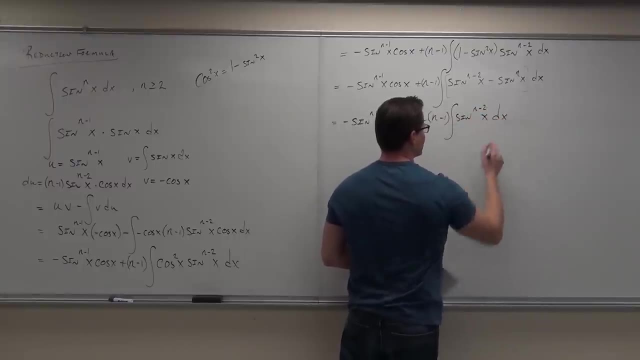 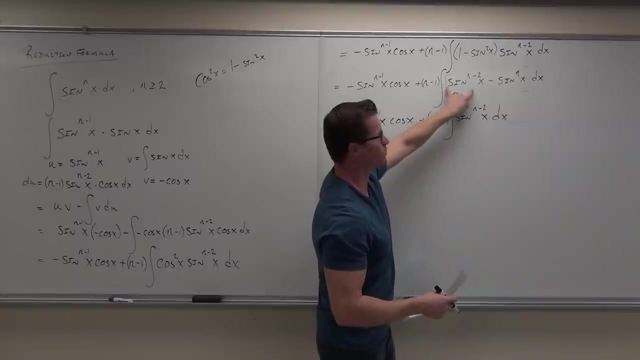 cosine x: nothing changes. plus n minus 1 times the integral of sine n minus 2x dx. Don't forget that dx. Here's what happens. So this: it's basically just like you dropped the parentheses because you're distributing this to this first integral, no problem. 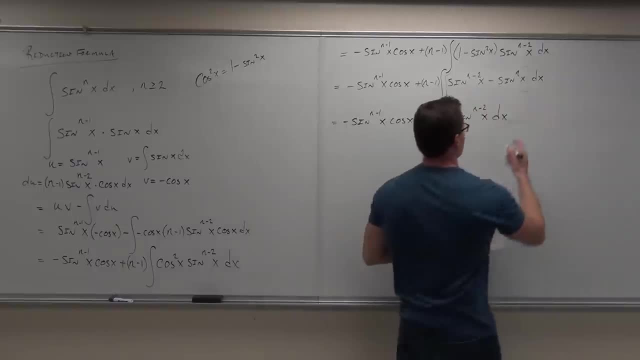 What's the next thing I'm going to write? Minus, Not integral. N minus 1.. N minus 1, yes, In parentheses, Then integral. what's in the integral Sine 2x, Sine of what? 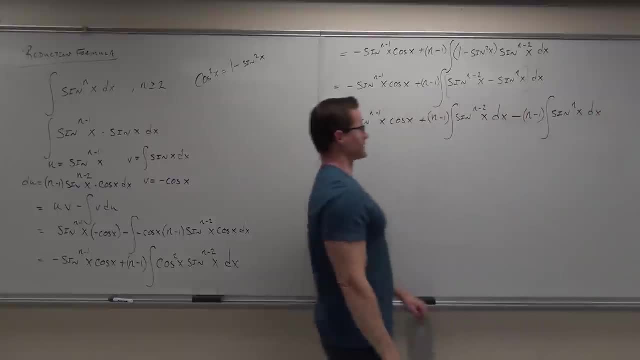 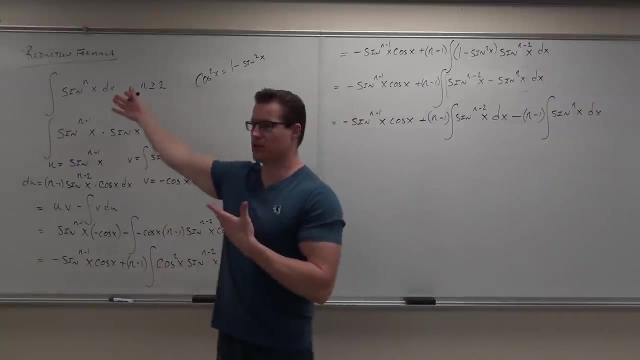 I mean x. yeah, That's it. Oh, now this is cool. It's weird, right? We're doing this in general. We didn't start with anything, Any number, Nothing, That's. this is kind of neat. 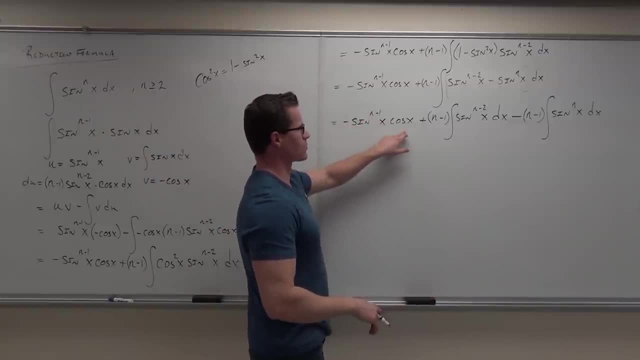 So we've worked this all the way down. We now have this. there's no integral there. Here we got an integral, but that's okay. we're creating a formula. okay, This part. What is this part? The beginning: 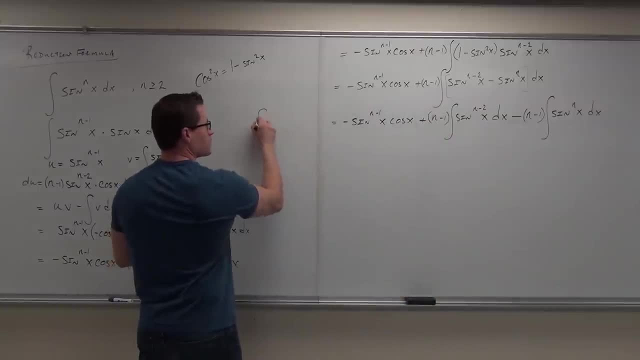 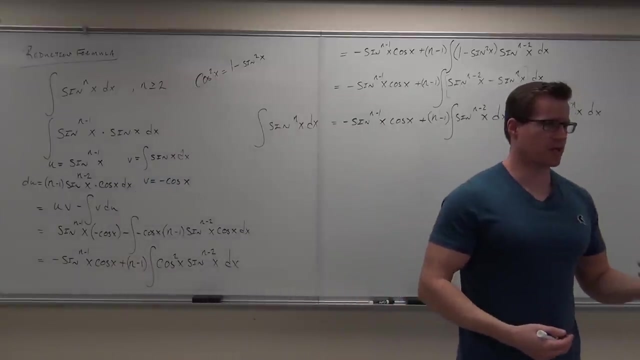 It's what we started with. Yeah, it recycles One, two Recycles Okay. so every time you've seen this before- I think we've seen it like three or four times now in this class, Because I want you to get used to it. 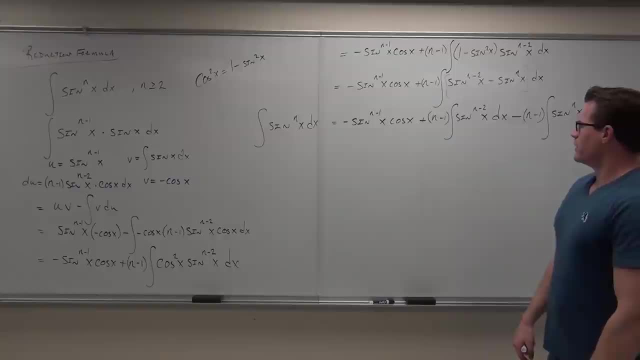 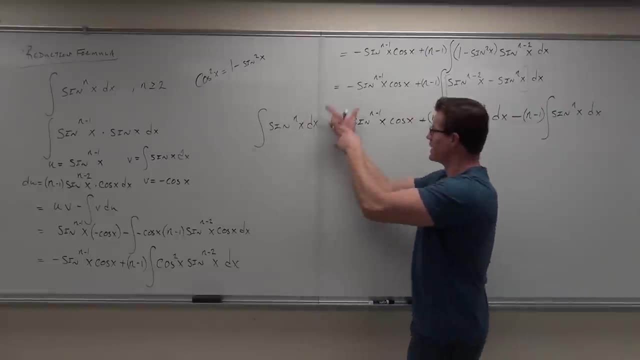 This stuff happens Especially on your type of homework that you're going to be doing. What do we do to get rid of this piece? Add it to both sides. It's an equation. This we have proven that it equals this entire mess of garbage. 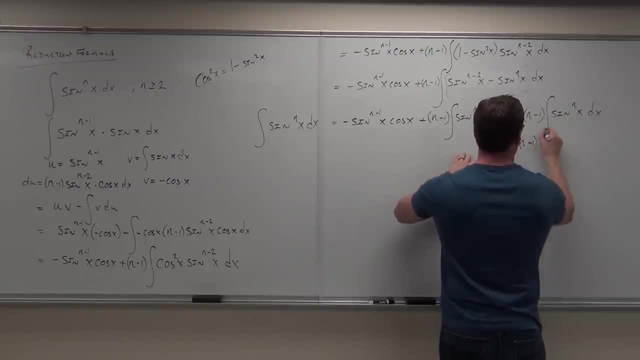 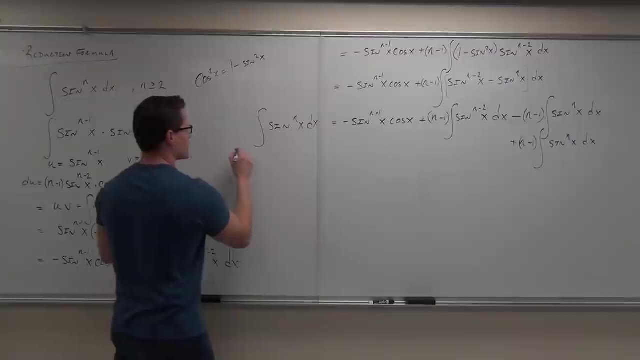 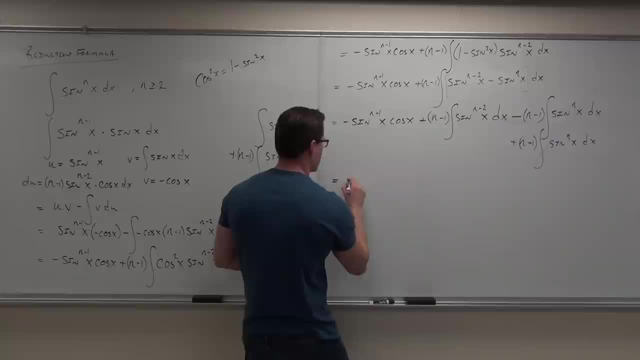 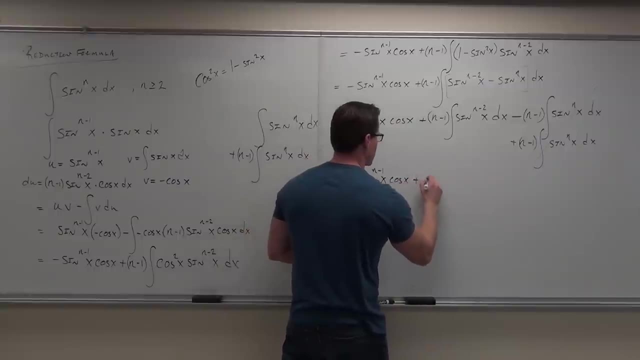 Yeah, Yeah, Yeah, Yeah. Let's think about what happens. Let's do the right side first. On the right hand side, this entire thing is gone. We have negative sine to the n minus 1 power of x, cosine x plus n minus 1 integral sine. 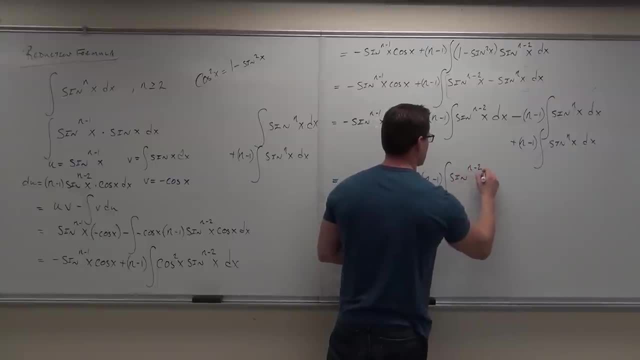 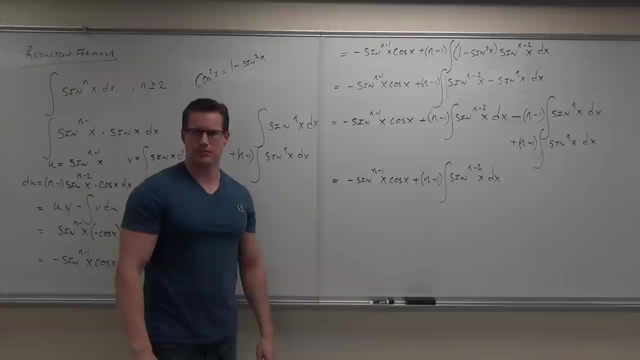 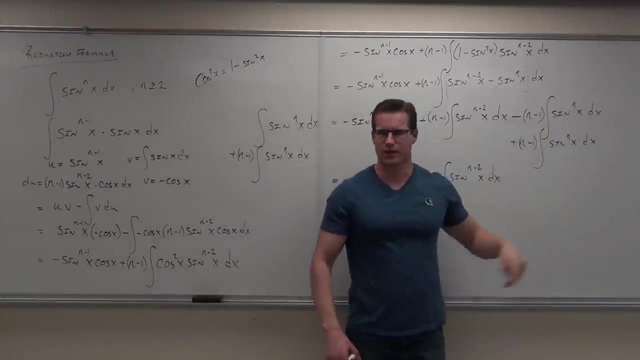 to the n minus 2 power of x dx power. This is gone, You guys? alright with that one? Yeah, Yes, no, yes, no, You sure This is all the same right, All the same, we just added this to both sides. 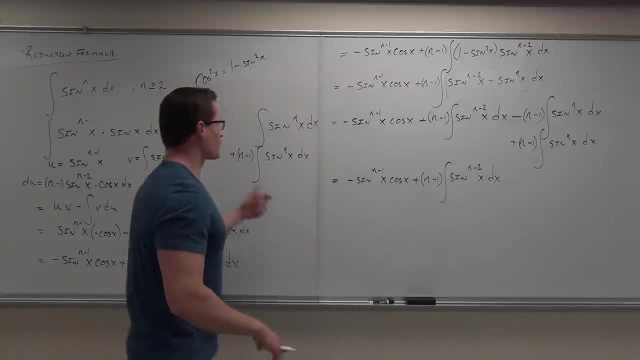 therefore, it is gonzo simplified. Now over here. this is the interesting one. How many integrals are here Two? This is just here. How many are here One? So the number up front is one, correct One? 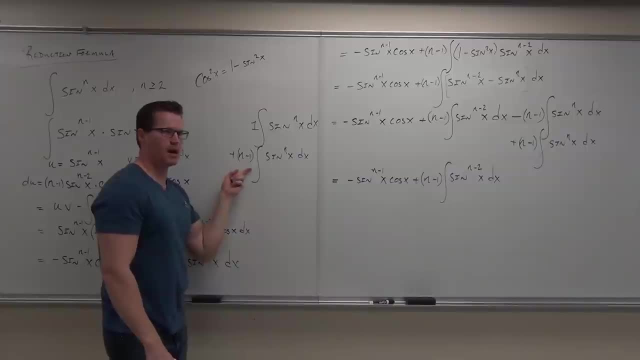 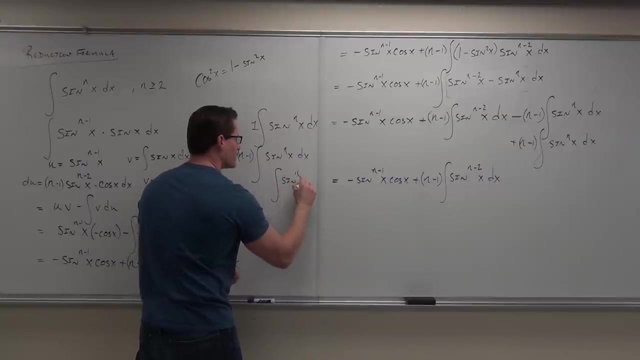 How many are here? N minus one. Add them. What's one plus N minus one N? So then I'll write it in black so we can see the difference here, So that we know N times this integral equals this stuff. 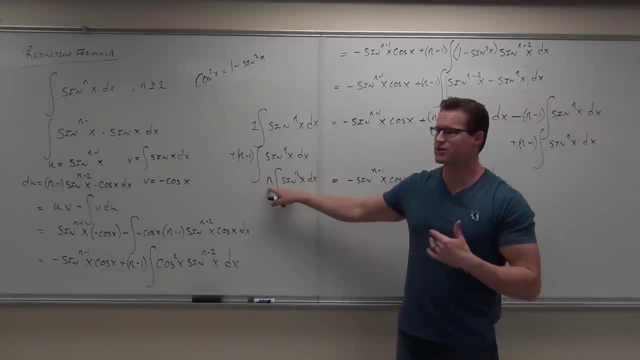 Now, every time before when we've had a number out front. remember, N is just a number, It's like two or three or four or five or six or seven. What do we do with that? We divide. 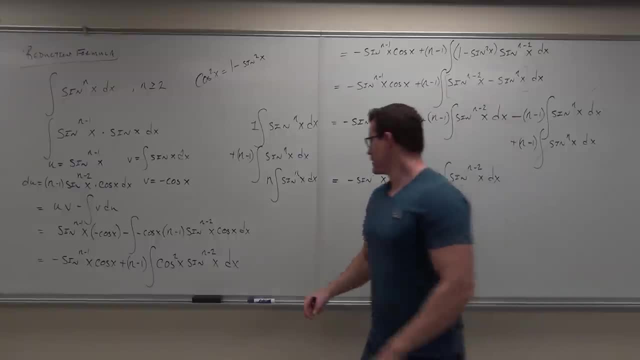 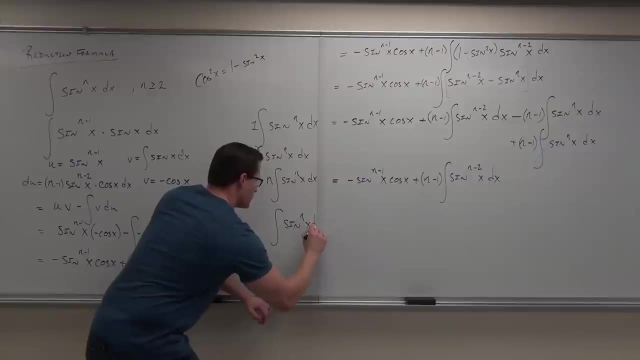 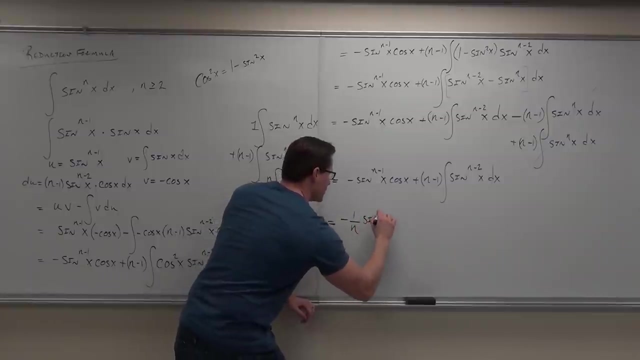 If it was three, we divide by three. If it's N, just divide by three, Divide by N. So if we divide by N, what we end up getting is negative 1 over N sine to the N minus 1 of X cosine X. 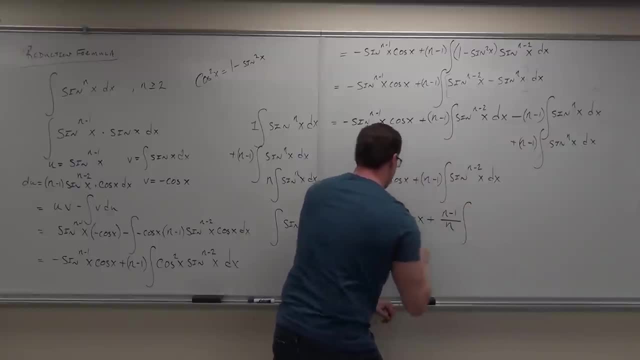 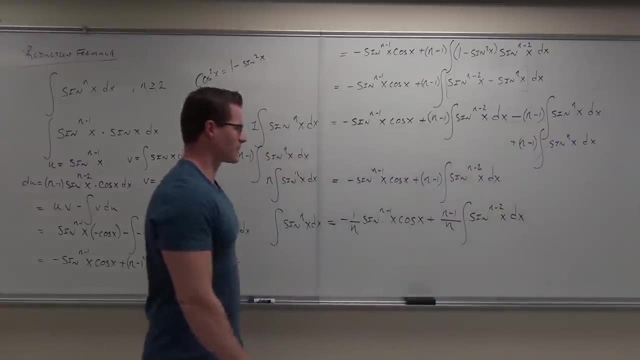 plus N minus 1 over N times the integral sine N minus 2 of X, dx. Of course plus C, because we're talking about an integral, But that will come at the very end. Let's make sure I did it right. 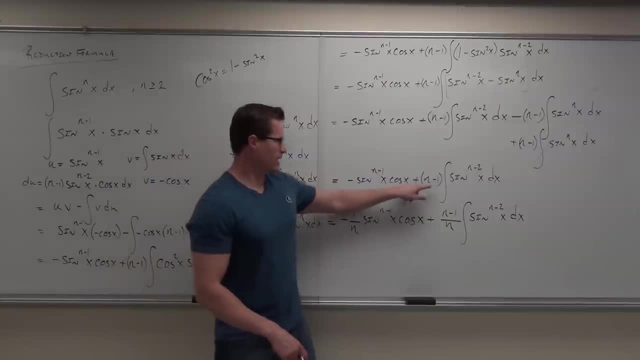 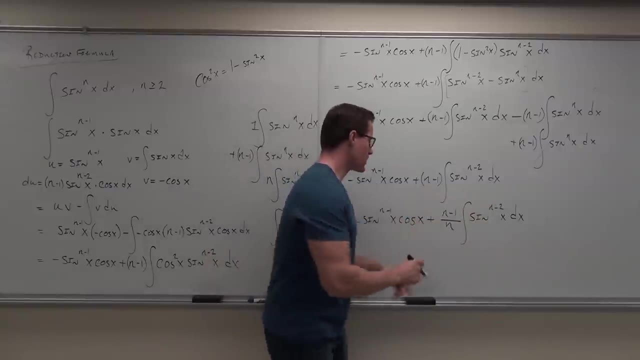 Do you guys see where the 1 over N is coming from? Divided by N, Here we have N minus 1.. Well, now we're dividing it by N. There's only two terms: This one and that one. This right here, this is the reduction formula for sine. 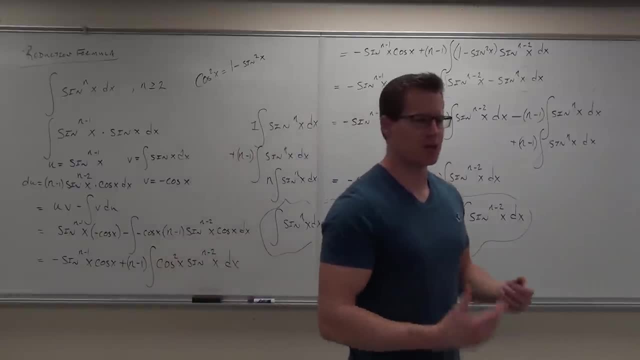 Now, if you're thinking that's a lot harder than just doing the problem, It's really not. I'm going to show you. Do you want to see an example of how this stuff works? I'm going to have to erase the board, though. 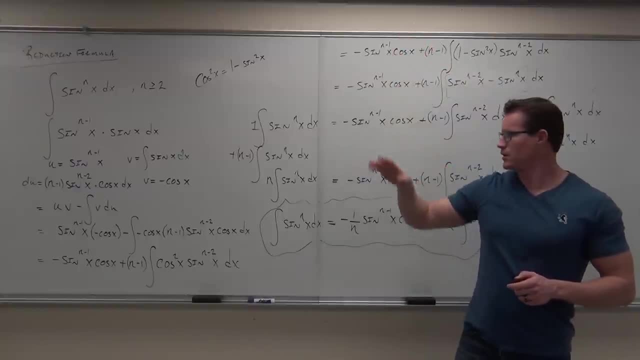 So show of hands if you feel OK with the proof. Oh wait, Just do it. I'm just going to erase this side. Are you guys OK with getting this far? Yeah, It doesn't make sense on how we got that far. 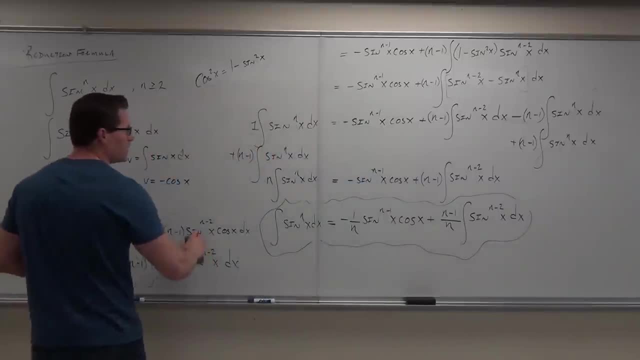 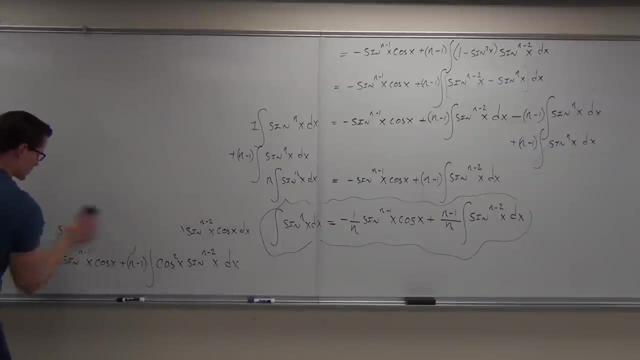 You just have to use it. I just want to make sense to you where it came from, that it wasn't just magic, OK. So reduction formula. I'm only going to give you one example on how this actually works. I think one example will make it very clear on how it works. 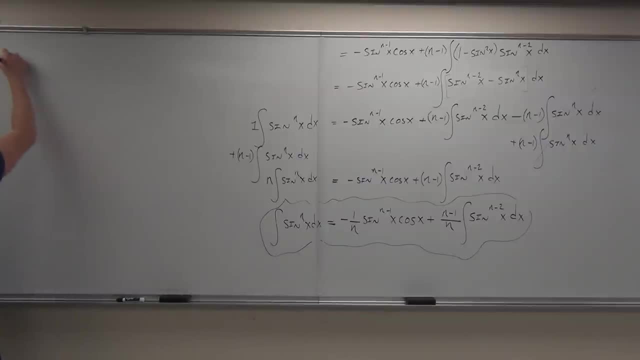 So here you go, Isn't it kind of a cool little proof, though It's interesting, right? It's a really nice little proof. Add it to both sides: if you've been practicing to buy, You're good to go. Kind of neat. 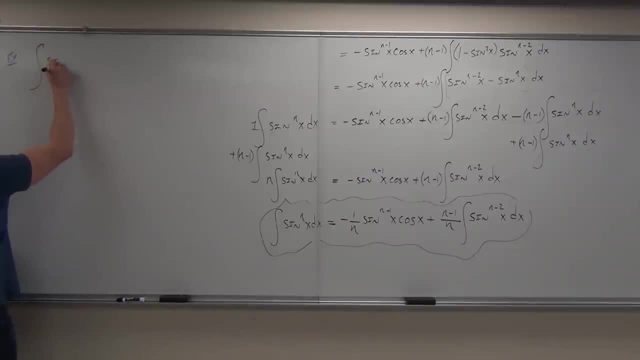 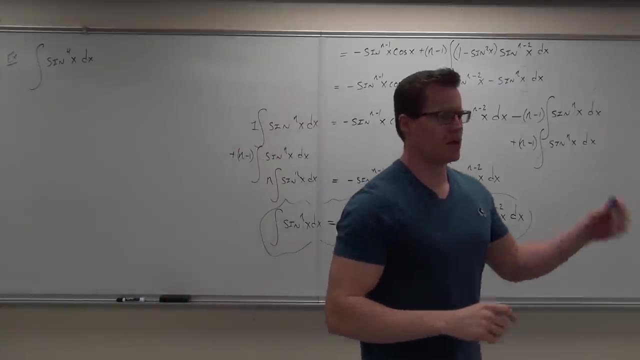 And what this allows you to do is this: If you've got an integral of sine to the fourth power of x dx- sine to the fourth power of x dx- you start thinking: wait a minute, How in the world am I going to do that problem? 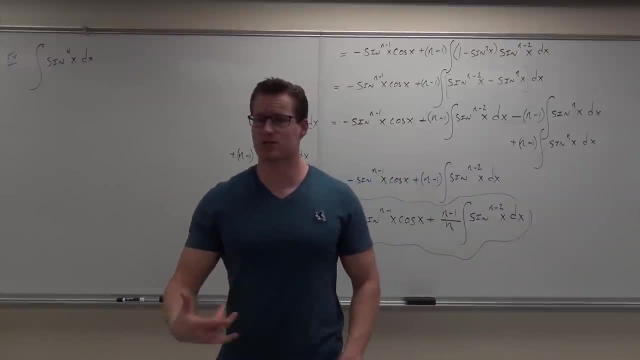 I don't know. I mean, does it fit the integration table the way it is right now? Does it? No, Will a substitution work? No, No, Remember, if I pick sine, the derivative of cosine, it's not up there. 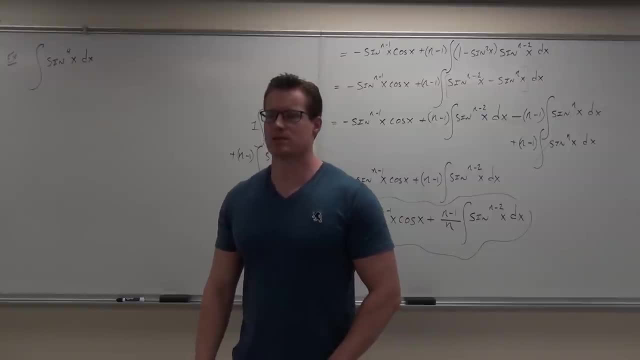 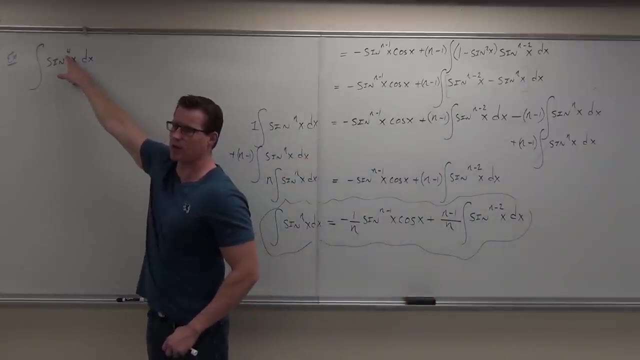 So that would be a problem. Integration of five parts: will it work? Yes, Yes, it will, But we've proven that we can actually do this every single time we have any power greater than 1, or greater than or equal to 2.. 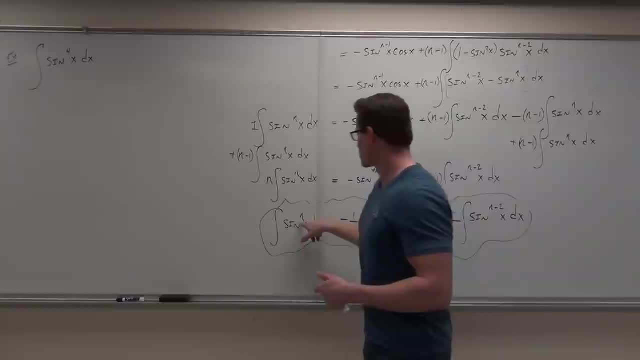 We'll check it out. Here's how it works. What's your n? 4.. So this is sine to the fourth, So our n would be 4.. Here's how you work it. It's really nice What this integral is going to equal. let's read it. 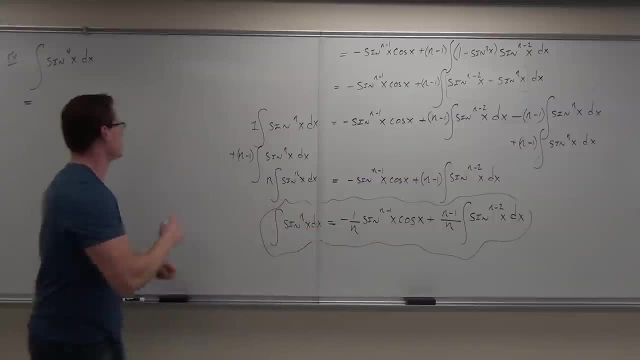 It's going to be negative 1 over what? 4.. Negative 1 over 4.. What's the next thing I write, Sine, Sine of. where are you getting the 3 from 4 minus 1.. Right there. 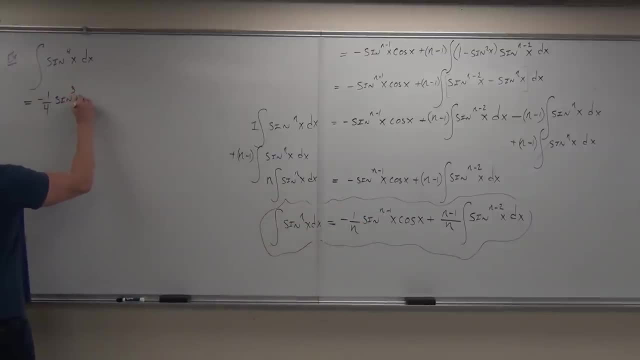 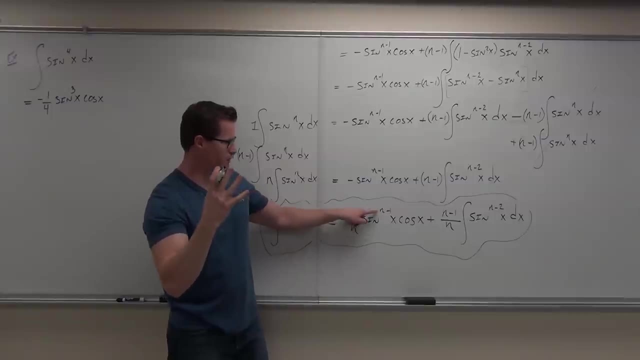 4 minus 1. x cosine x. So let's see: n was 4.. So negative 1 over 4.. Got it Sine to: the 4 minus 1 is 3. x cosine x. Then we're going to put a plus. 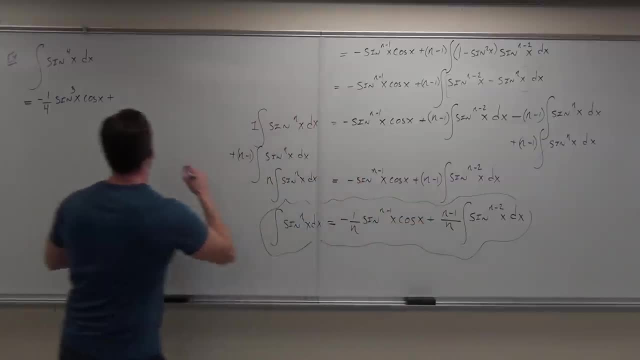 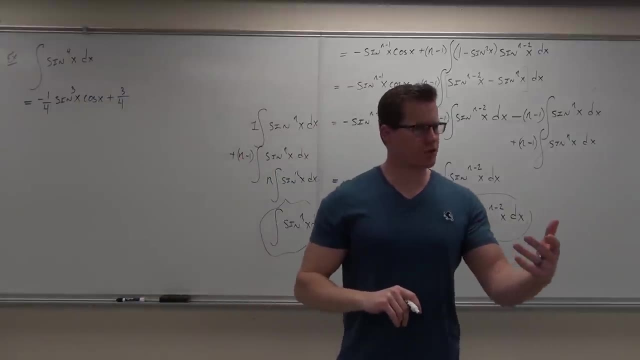 Again, n is 4.. So n minus 1, that's 3 over 4.. What's the next thing we have? It's an integral. It's an integral. You're still going to have an integral. That's why it's called the reduction formula. 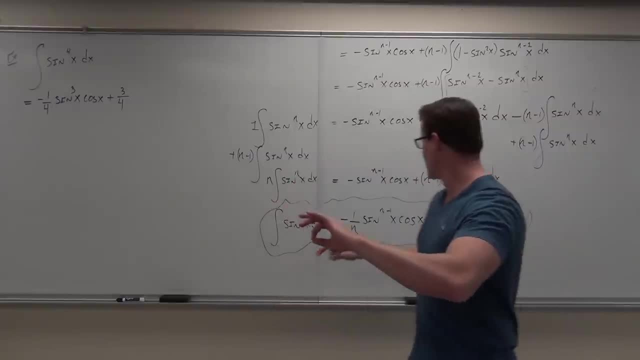 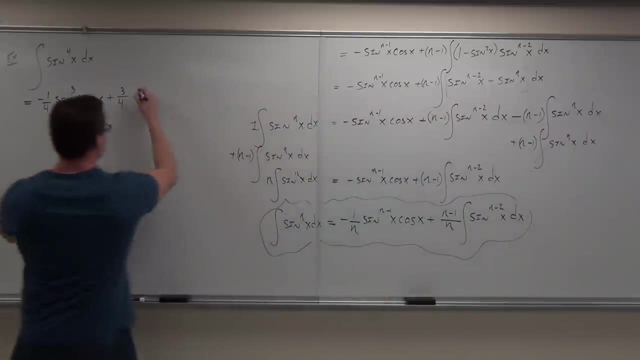 because it's going to reduce the power of the sine by 2 every time. Do you see that? By 2.. So instead of having sine to the fourth, now we're going to have an integral. It says of sine Square. 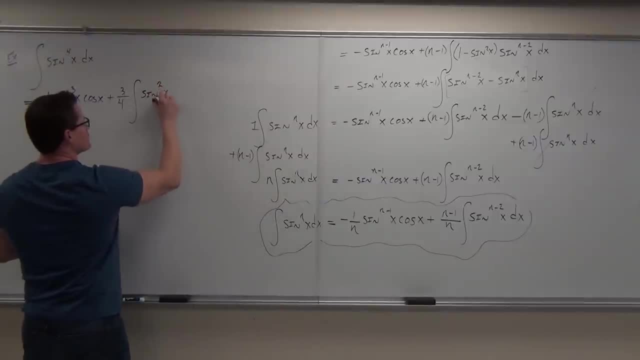 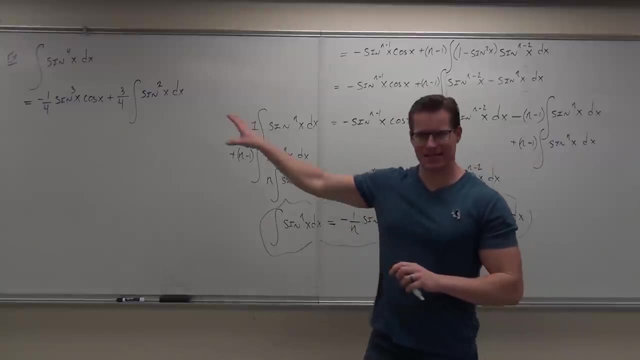 Good Yeah, n is 4.. 4 minus 2 is 2.. And it just made it a little bit better. Isn't that kind of nice? Is it easy for you? It's just a formula, So it's kind of nice. 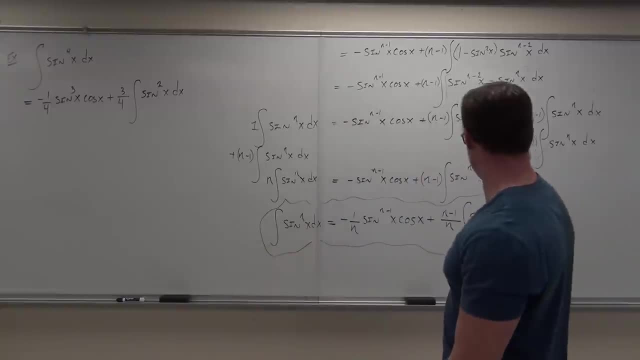 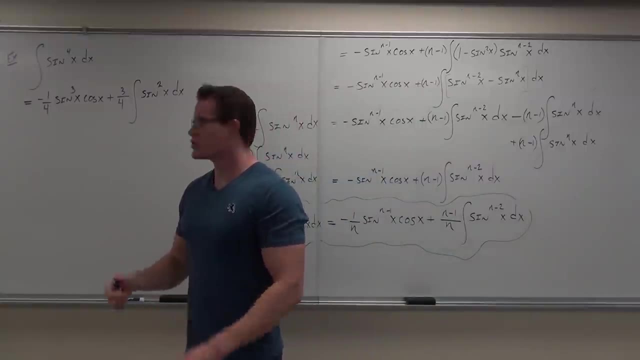 That way you don't have to waste a lot of time on integration by parts. Make sure I got that right. Questions. So then, once we get the integral of that, we can still keep going by plugging in. That's the question. 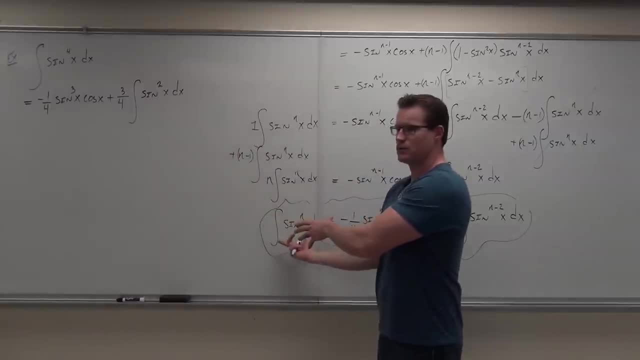 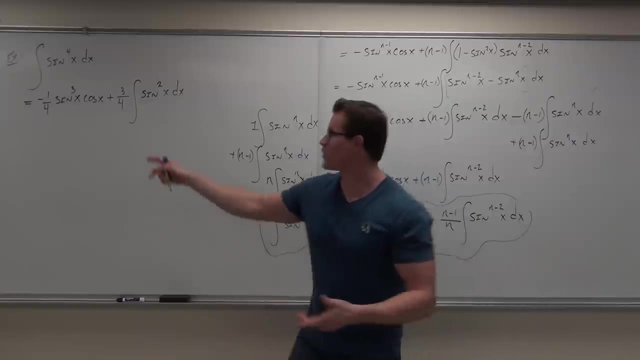 Does this now fit this model? Shoot, just do it again. As long as the n is greater than 2,, greater than or equal to 2,, and this is 1,, you're good to go. So if this is a power 3,. 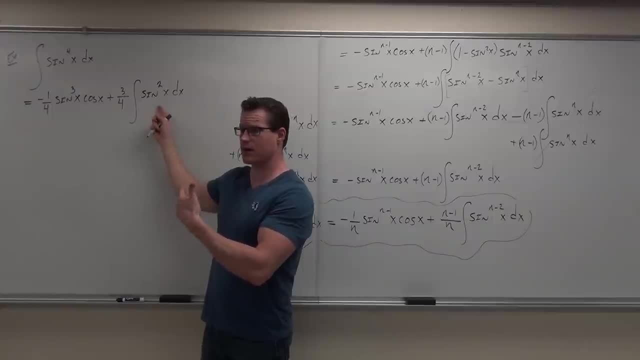 you'd be done right now, because you'd have the integral of just sine to the first right. The integral of sine is just negative cosine a. You're done. So what we do is just do this one more time, So we rewrite everything. 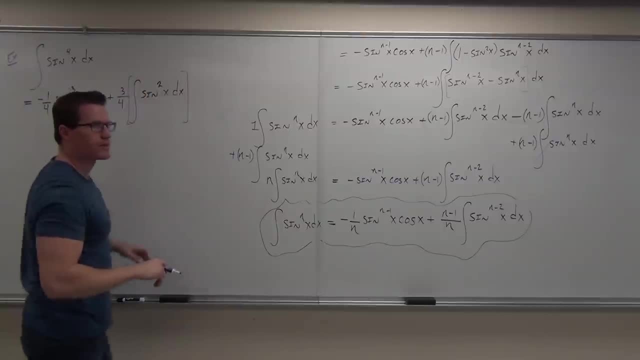 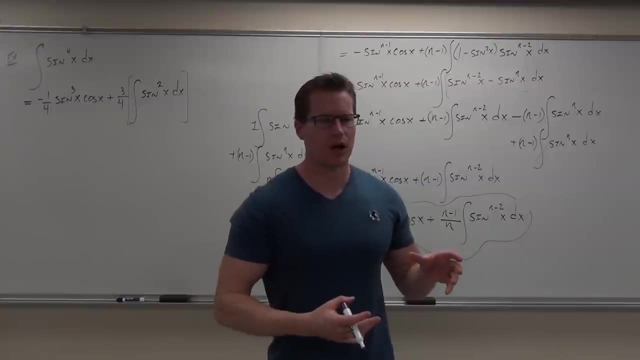 It's just this little piece. Remember, this is in a bracket. Some of you are in the very bad habit of not writing parentheses. Parenthetical expressions in mathematics are absolutely crucial. It allows you to distribute, It allows you to see what's being multiplied. 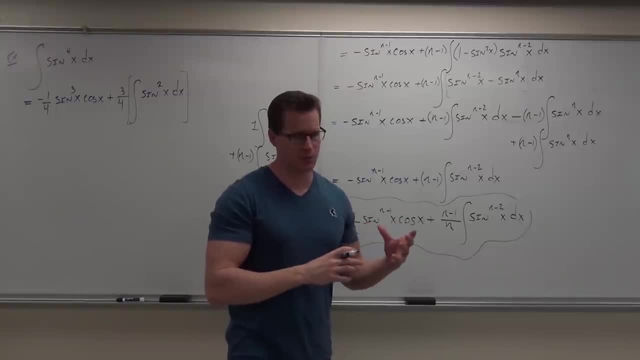 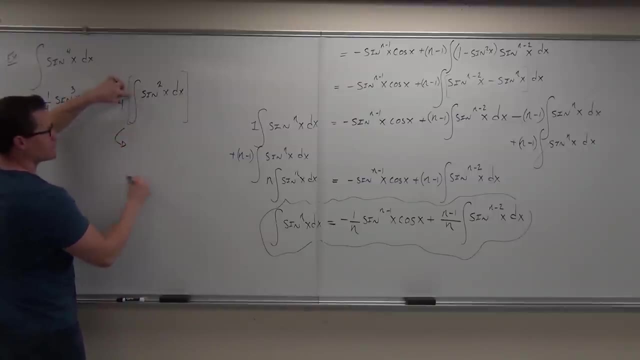 order, operations-wise, what's being added and subtracted and not being multiplied. okay, So they're very important. So when we have this thing, when we do this, this little segment, well we can do the same thing. Just be real careful that you know. 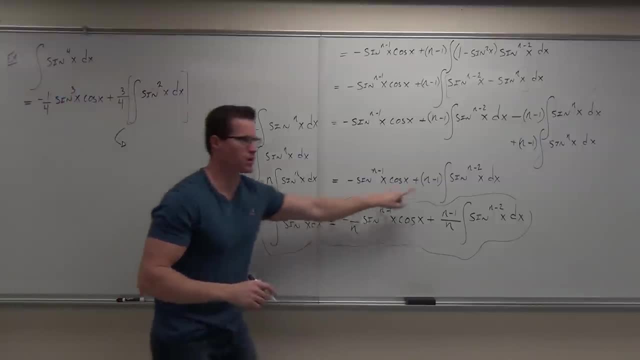 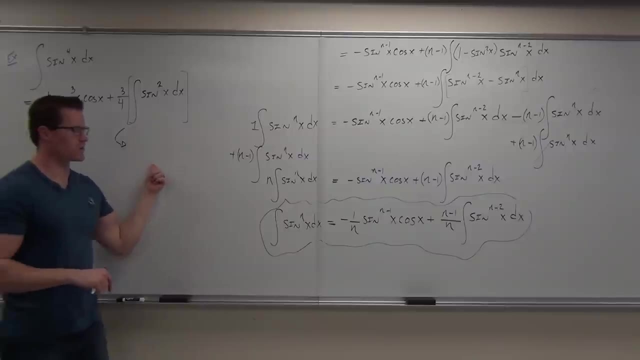 this positive 3 fourths is going to distribute across both of these terms. Does that make sense? That's huge. So for us, let's do it. Why don't you do it? Just do this little piece sine squared x. 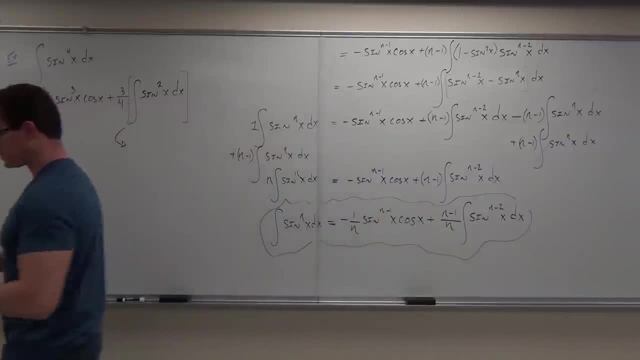 Do it just like that. okay, Just write out what that little piece is. Okay. what's our n? again, people, Negative 1, south. What's our n? 2. Oh, 2.. Let's plug in the 2. 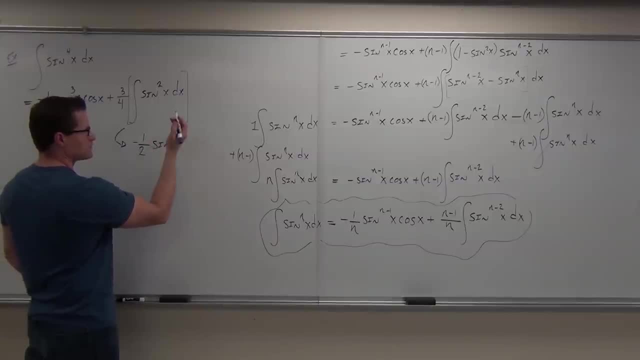 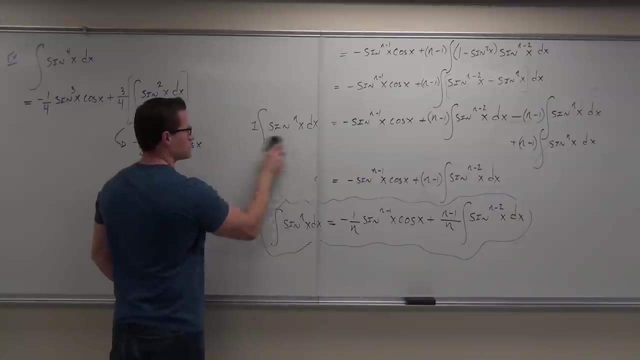 everywhere you see the n Yeah, 2 minus 1 is 1.. That's cool, Cosine x. I have to erase this part now. Plus plus Okay, 2 minus 1, that's 1 over 2. integral of: 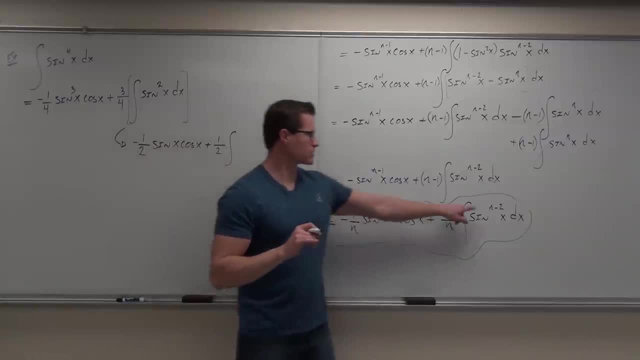 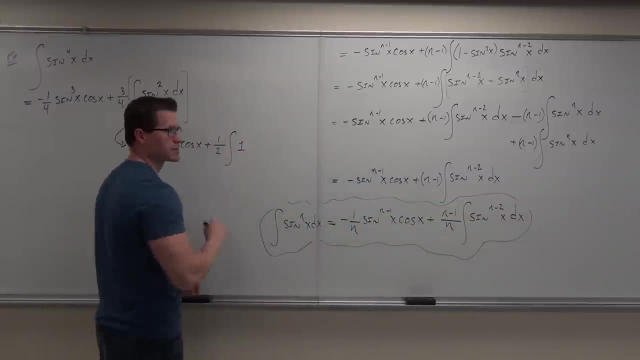 Please be careful when you do this. How much is What's our n? 2.. 2 minus 2? 0.. What's anything to the 0 power 1.. Don't you be putting a sine there? that doesn't make any sense at all. 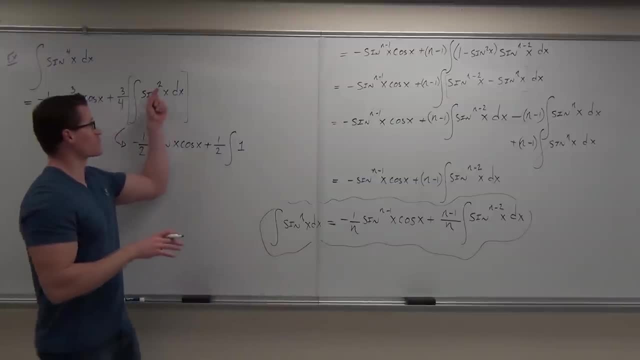 If you put sine, then this would have had to be a 3.. Does that make sense? Yeah, Hello, yes, no, Yes, Sine, some of you. it doesn't make sense. I can tell in your eyes. 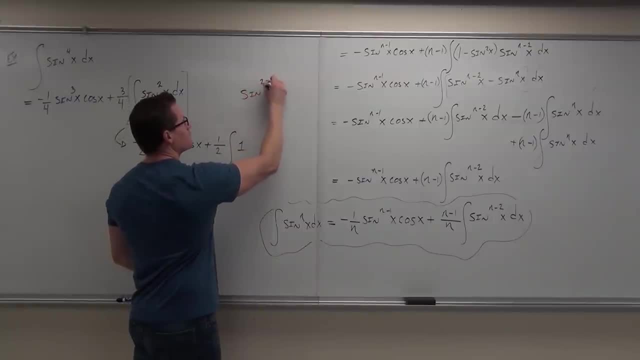 2 minus 2? 0.. Anything to the 0? 1.. dx, You don't even really need the 1 there, I'm just going to write it down: 2 minus 2? 0. 0.. 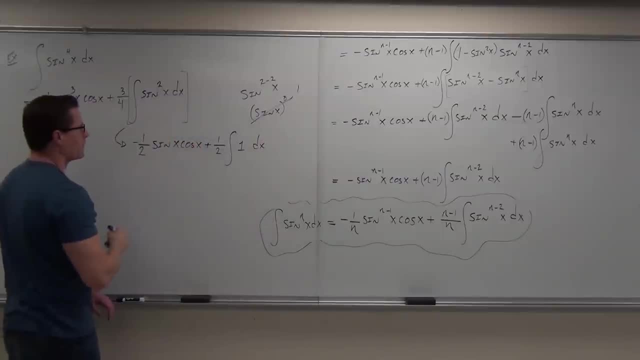 1. dx. You don't even really need the 1 there, But we can have it. So this would become negative: 1 half sine x, cosine x plus 1 half. Hey, what's the integral of 1? n. 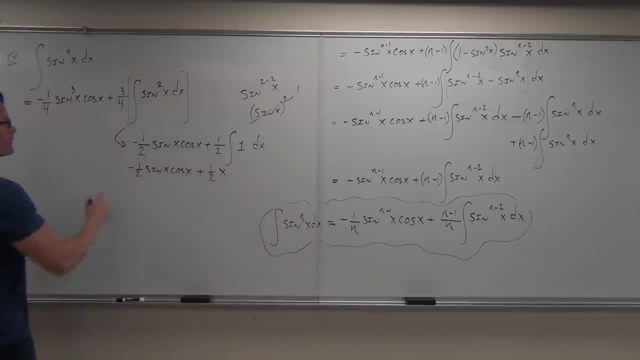 There we go Now. just keep in mind that this whole thing- there's a 3 fourths in front of it and a plus in front of that and a cosine x and a sine to the third power of x and a negative 1 fourth. 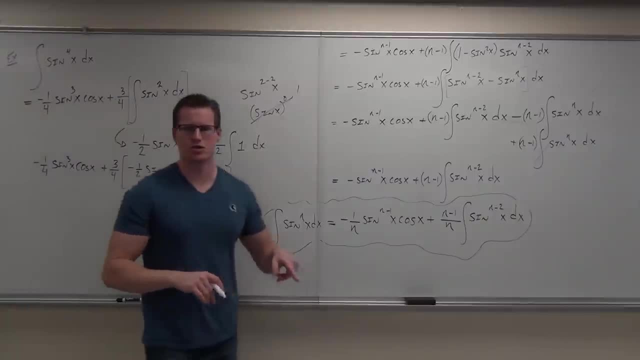 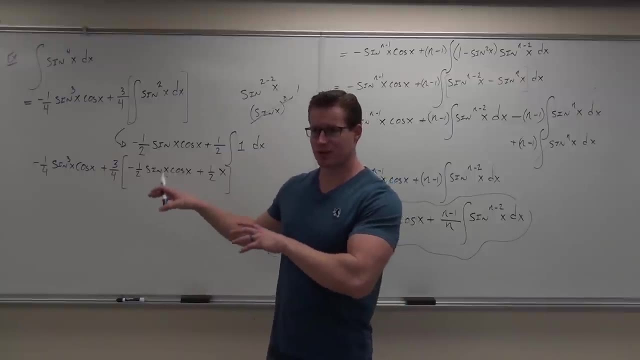 This has to distribute, which is not a problem. You just can't lose it. You can't lose track of it, because that would be a problem. Quick head nod, if you're okay with that so far. Do you see how much faster this makes integration by parts?